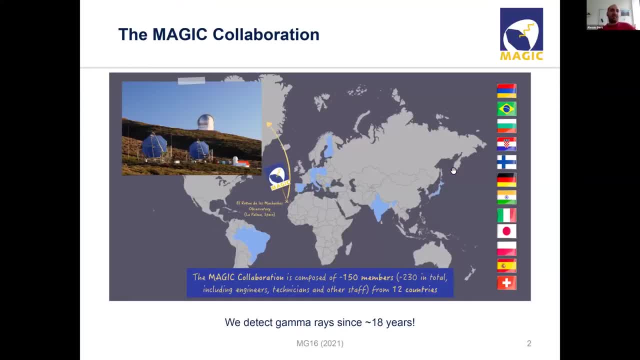 at in other conferences. So, starting a bit presenting the magic collaboration, We are basically running two Jericho telescopes of 17 meter diameters in the islands of La Palma, So we are more or less 150 people, and taking into account also technicians, engineers. 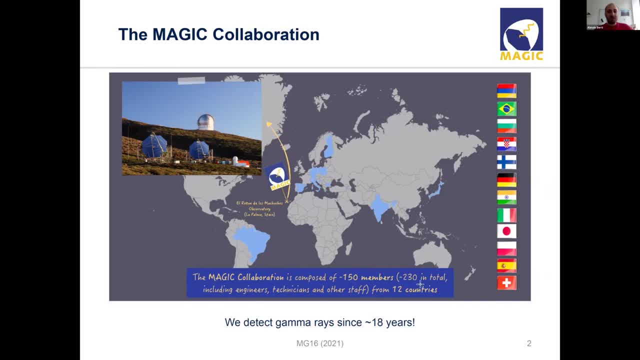 and so on other stuff. We are more than 200 people from 12 countries And basically we are running this telescope since more or less 18 years. Well, basically the first telescope since 18 years. then the second telescope was added later in 2009.. So a little bit less. 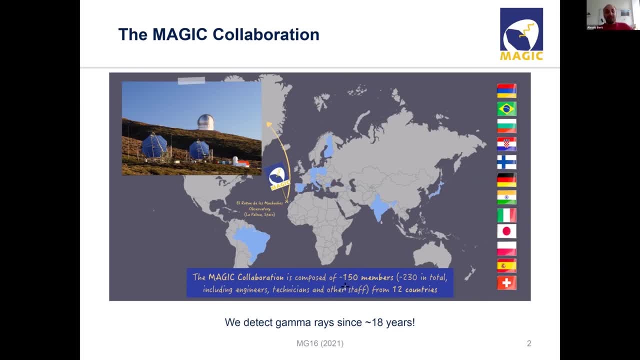 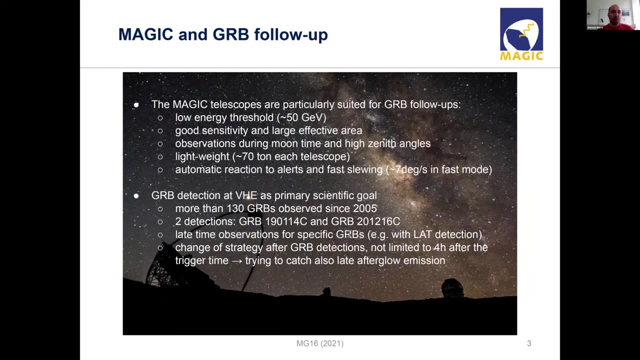 it is running since a little less time. We of course have a quite extensive follow-up program for GRBs because our telescopes are quite suited for the follow-up of GRBs, Starting from the fact that we have a low energy threshold because we have a large reflector, So also the energy threshold that we have is quite low around. 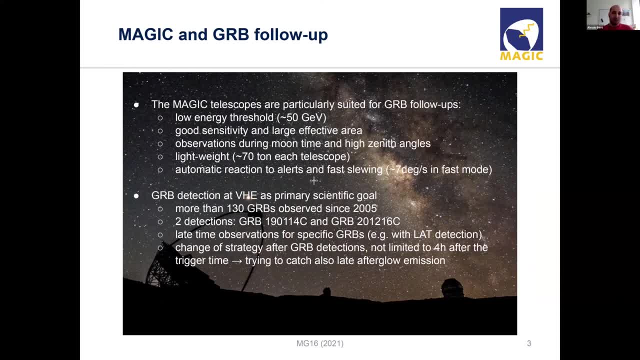 at the zenith And we have also an additional trigger system which is called the sum trigger, which allow us also to go down to around 30 GV in threshold, again in zenith, And this is of course very good for GRBs, which are quite distant sources where the effect of the extra galactic. 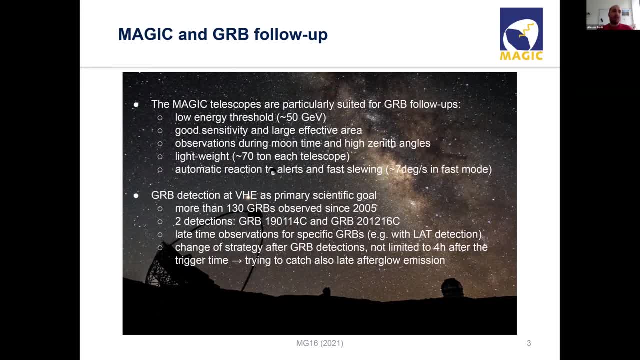 background light absorption is quite, quite strong. We have also good sensitivity, also for small time scales and large effective areas, So we can collect many photons in order to perform, for example, spectral and temporal temporal studies of GRBs. We also have worked quite a lot in order. 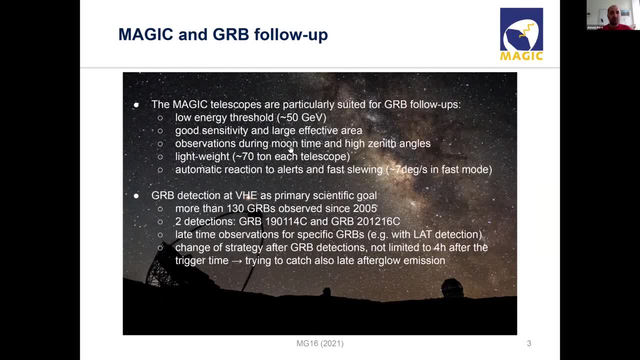 to observe during moon time, even strong moonlight and at high zenith angles, And this is because we want to increase our duty cycles and also because GRBs they come. of course, we don't know where and when they will appear, So we need to be prepared in every situation, And so the telescopes should. 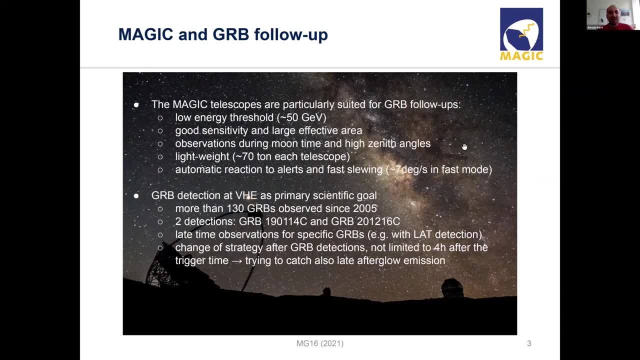 observe under any possible conditions that we, that we can think of. And finally, they are quite lightweight. Well, 70 tons per each telescope, but let's say this is quite lightweight for a spherical telescope And for GRB alerts, but not only for GRB alerts, also for neutrino alerts, for 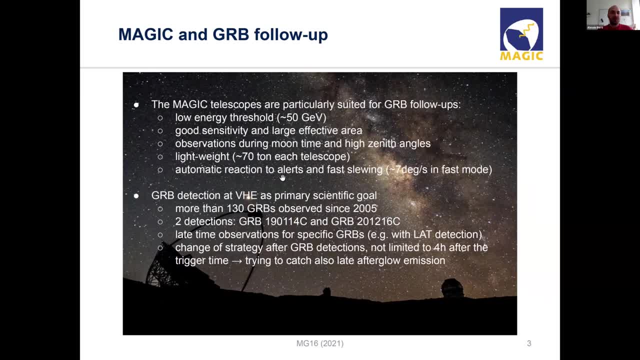 example, we have a full automatic reaction when we receive these alerts where you use also these fastest viewing where a telescope can do with a speed of around seven degrees per second in fast mode, Of course, one of the primary scientific goals that MAGIC always had since the telescope. 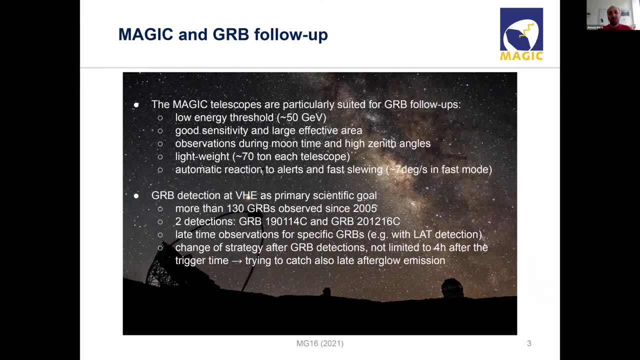 were designed was the detection of GRBs at various energies, And currently we have more than 130 GRBs- actually almost 140 GRBs- observed since 2005.. And we had until now two detections: One is the famous GRB 1914C and the most recent one last December, GRB 2012-16C. 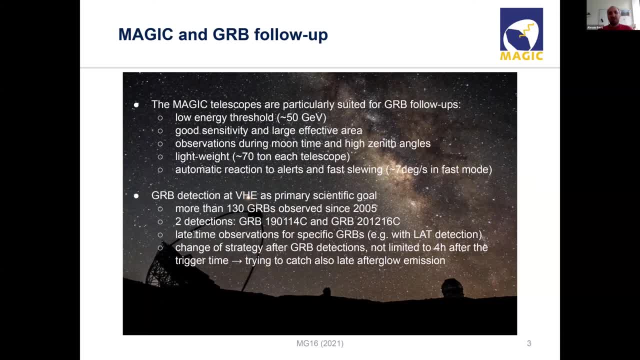 And of course we during the years, looking also at the different results appearing, we also refined and changed a bit the follow-up strategy for GRBs, So, for example, including late-time observation for specific GRBs, So for example the one with a lot detection, because we know that they have these. 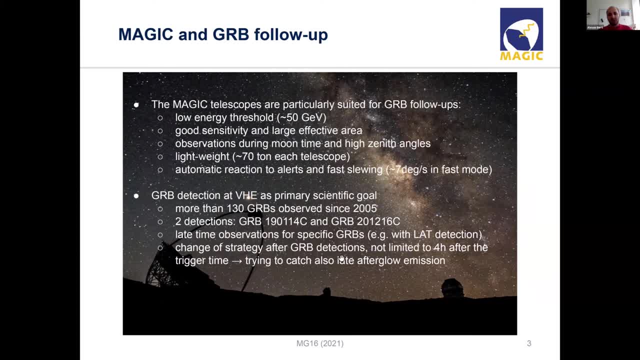 extended emission in the afterglow And also, yeah, not limiting the observation to the first four hours after the trigger time. And this is because now we know that we could have- we can have also very energy emission in the deep afterglow of GRBs. So 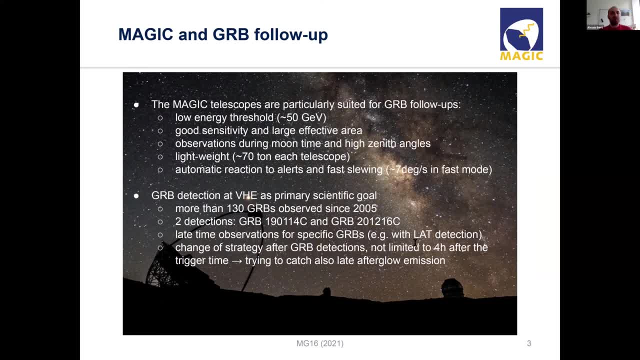 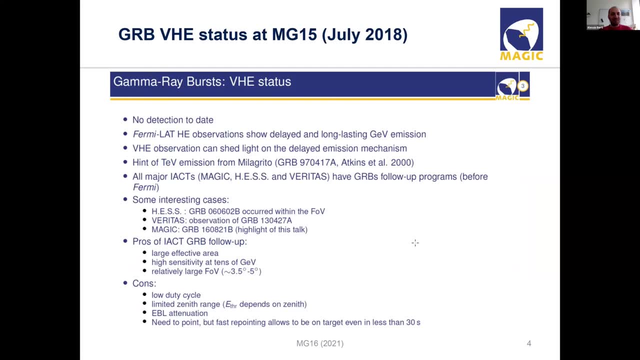 we need to take into account this fact And so, therefore, we changed our follow-up strategy. So this was a bit since I participated to the Marseille Grossman, also in 2018, where I was presenting a similar talk- This, basically, there was the status of GRB- very energy. 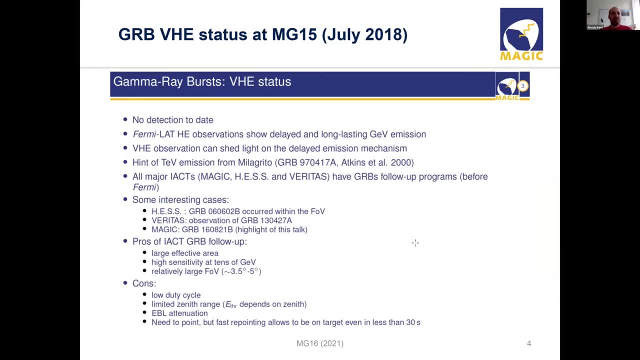 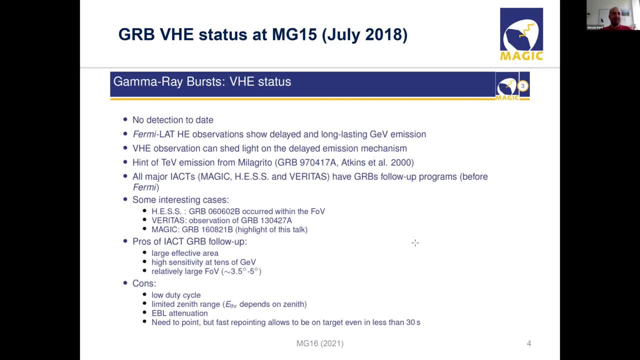 We already knew that from Fermilat we had this delayed and long lasting GEV emission And of course, what we we wanted to do with the very energy observation was to shed light on the possible delayed emission mechanism and know if there is very energy emission, and so on. 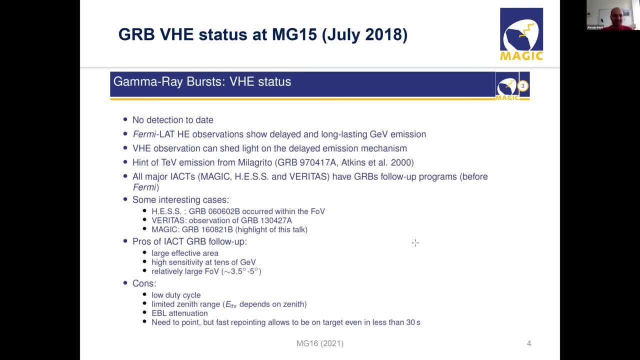 We had these hints in the 90s from Milagrito and, of course, all the major GSTs. So not only MAGIC, but also Hess and Veritas. And, of course, all the major GSTs. So not only MAGIC, but also Hess and Veritas. 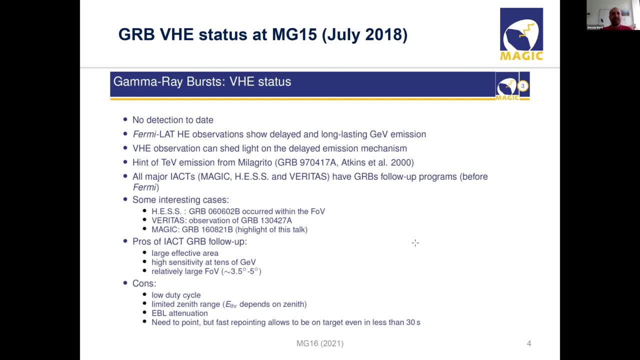 And, of course, all the major GSTs, So not only MAGIC, but also Hess and Veritas, Of course had, and they currently have, GRB follow-up programs dedicated to the search of very energy emission from GRBs, and this, of course, we will hear more. 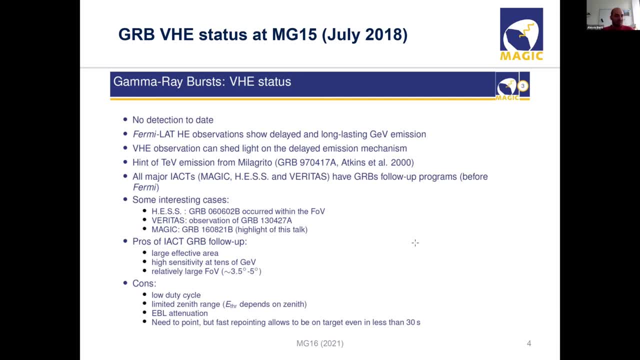 about in the next talks. There were some interesting cases, but of course, yeah, there was no firm detection. There was, for example, this interesting hint on this short, GRB 160821b, which is basically, basically will tell you a bit about in the next slides, But, yeah, no strong confirmation. 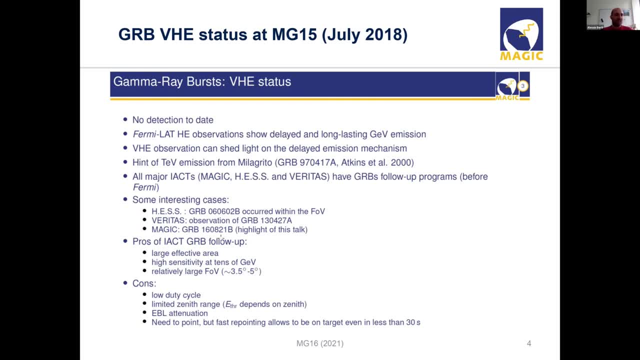 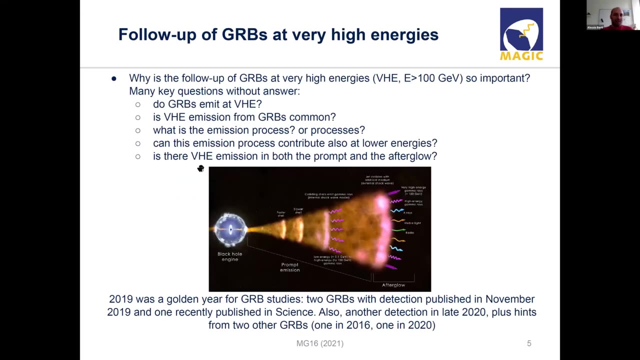 of very energy signal from gamma reverse, And here, of course, some pros and cons of the, of the follow-up of GRBs with the, with the EACTs, which basically I already pointed out some, some of them in the previous slide, So why we are following up GRBs at very energies. I think this is: 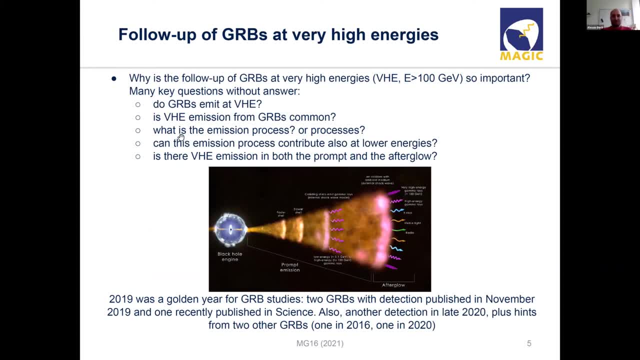 common for all the EACTs. So first we want to know if GRBs actually emit at very energy, If this very energy is somehow common, so present in all GRBs, If it is energetically relevant how it compares with other emission processes in GRBs, Understanding what is the emission process. 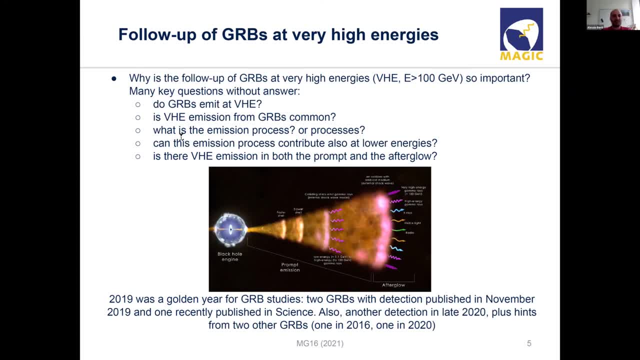 or processes- you know, it is not said that there is just one process that can produce emission for GRBs at a very energy range- And if this emission process, for example, could contribute also to lower energies, for example in the lat energy band. And another interesting question which let's say partially is without answer, is if very energy emission can be. 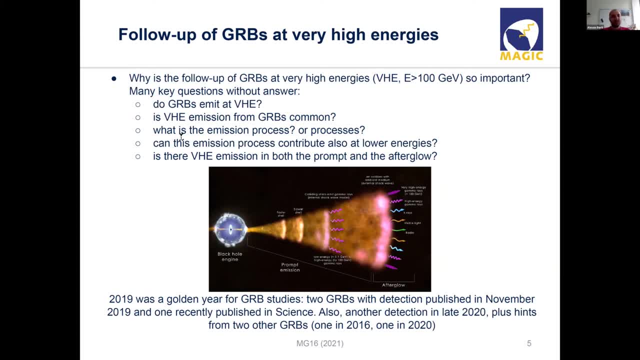 present in both the prompt and afterglow phases of GRBs, So before 2019. I think all of you know that we did an analysis of the EACTs and we have many clues in order to answer this question. But yeah, 2019. 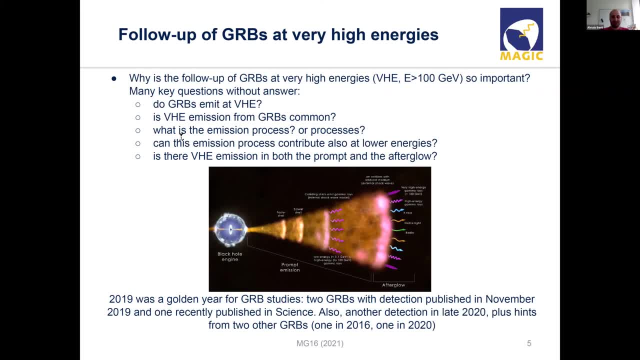 actually, at the end, turned out to to be a quite golden year for GRB studies. We had two GRBs with detection- GRB 1901-14C and GRB 1807-20B, which were published in November 2019.. And then another. 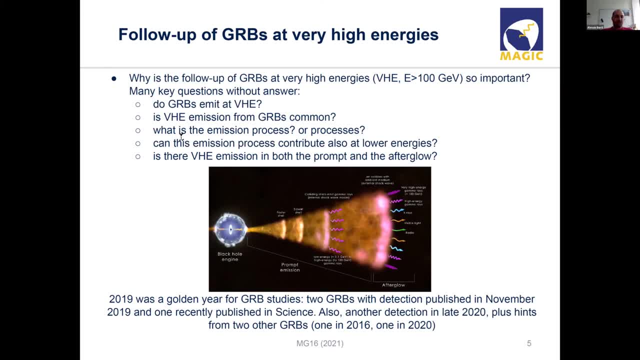 one, GRB 1908-29A, which was instead recently published in Science. So one detected by MAGIC and two by HESS. Then also, as I said before, there was another detection in late 2020, in December, again by MAGIC, And then other hints from two other GRBs, one in 2016 and one in 2020, which I will 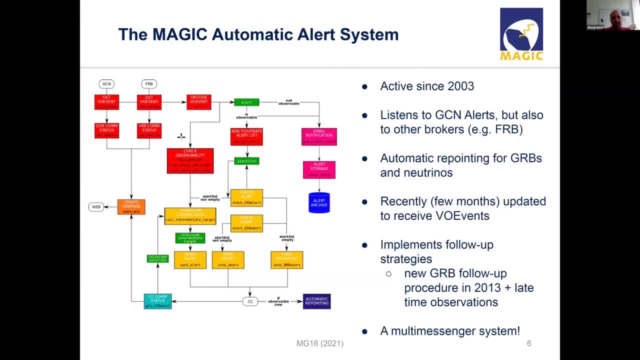 mention later. So, in as I said before regarding the follow-up of GRBs, we have this automatic alert system, which is active basically since MAGIC was born As a mono-telescope which is basically listening to the GCN alerts, but also to other brokers, for 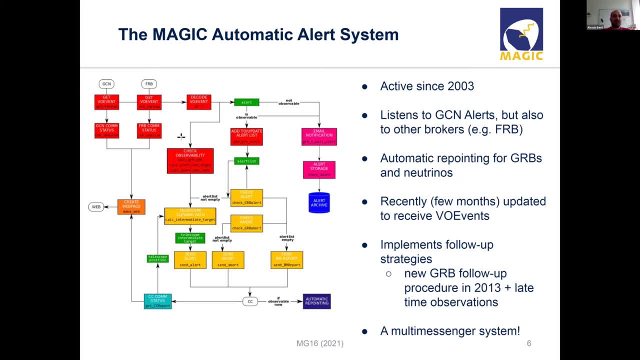 example, the ones, the one delivering fast radio burst alerts And of course we we have the automatic repointing for GRB neutrinos in place. And recently there was this update- since few months actually- where we are receiving the, the alerts in the so-called VOE event format. 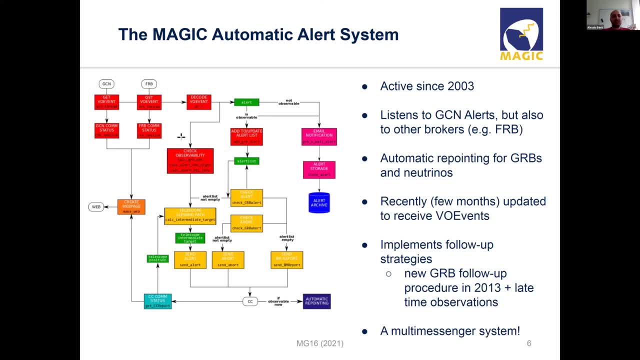 which, in the basically, should be the standard format for delivering transit alerts among the community. And, of course, this system is the one that is actually implementing the follow-up strategies And, since 2013, we have this updated GRB follow-up procedure, which, basically, was updated in order to 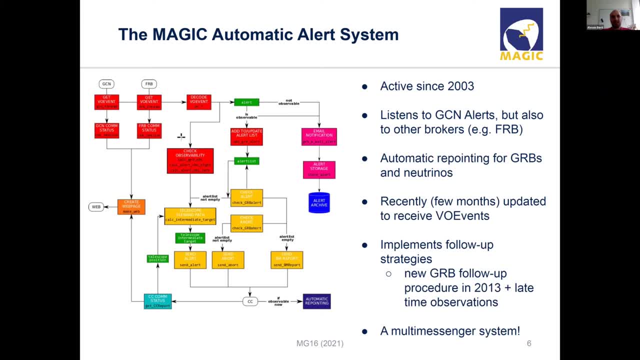 reduce a minimum the possible issues during this automatic repointing, for example, issues related to the data acquisition system, And also we implemented the so-called late time observations, So we don't receive only GRBs and neutrino others, but also, for example, gravitational wave. 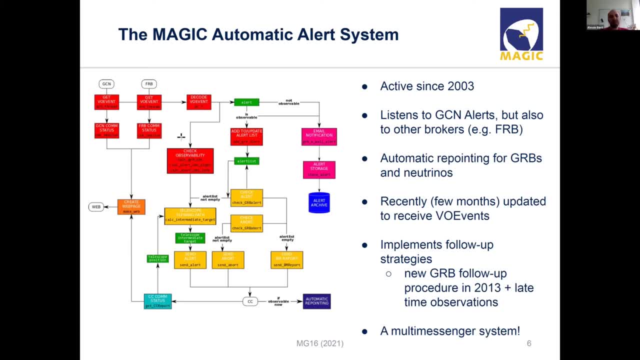 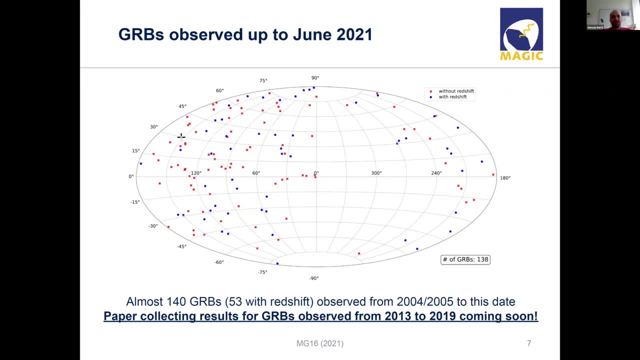 artists. So this is somehow a multi-messenger system. So this is a sky map which is showing basically the, the location of the GRBs for follow-up, followed by MAGIC, since the beginning, so 2004-ero and 2005.. The one with the red cross are the ones with this radar. 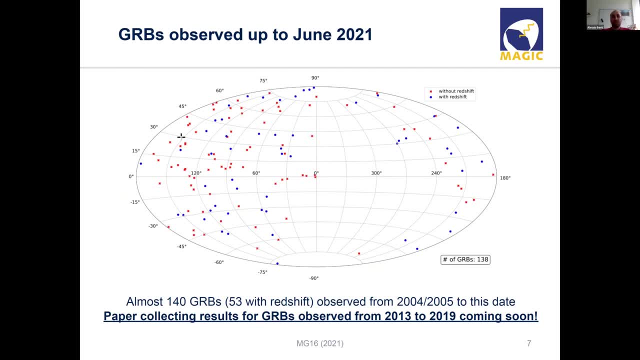 Later on. for example, we do a lot of radio interference as we will process in theworthy weather it depends with without redshift, while the blue points are those with the redshift and we have a total of around 140 grbs, of which 53 have redshift and of course, as i said, among these grbs we have only two. 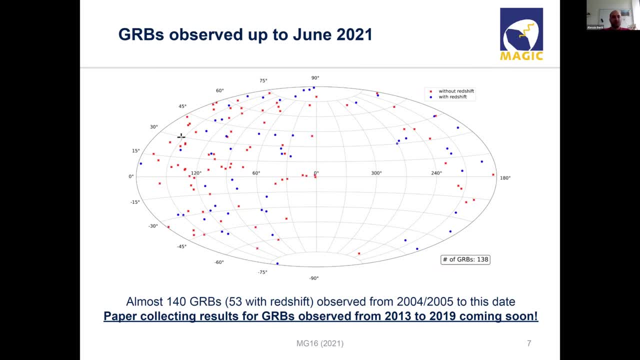 detections and two with the strong hints, but of course also for those grbs which we observed and on which we have upper limits on the very energy emission. of course they can give important informations and important constraints on, for example, on the emission models, and so we are. 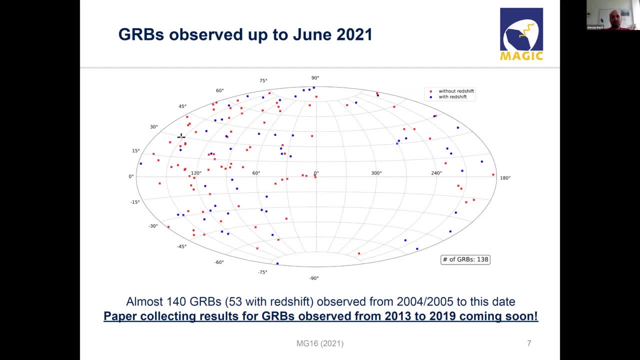 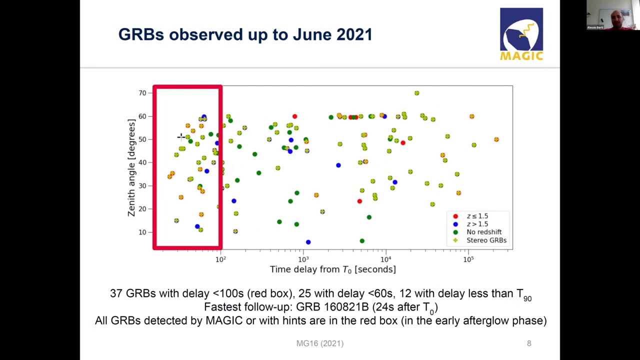 currently working since quite some time on this paper, which is collecting the results for the grbs observed by magic from 2013 to 2019, and this should come soon. this plot is instead. i want to show you a bit the the delay with which we observe the, the grbs. 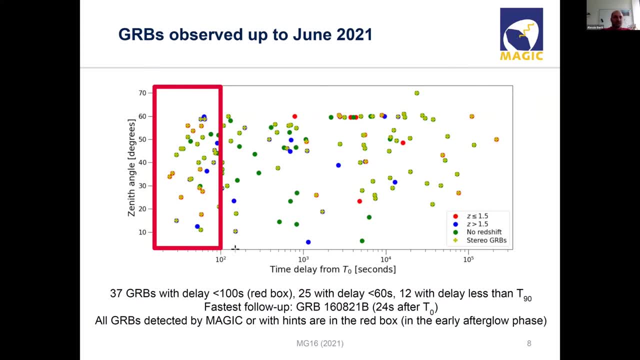 in this red box. basically, i am showing the grbs that we could follow up with a delay less than 100 second and the. the number of grbs in this case is 37. we have instead 25 with a delay less than than than one minute and 12 with the with. 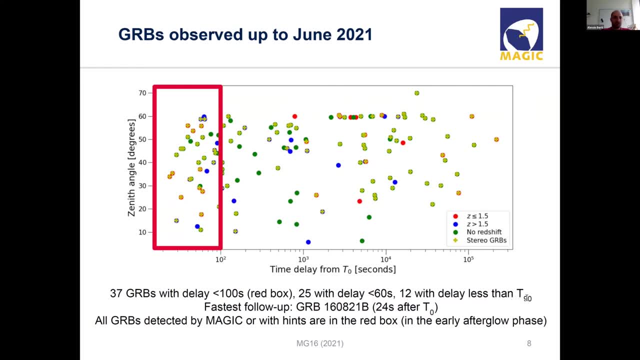 delay which is less than than the duration of the burst. of course this is not telling that we observed you in the prompt, because we know that in some cases t90 is not a good proxy for the for the duration of the prompt emission phase of of gamma ray burst. 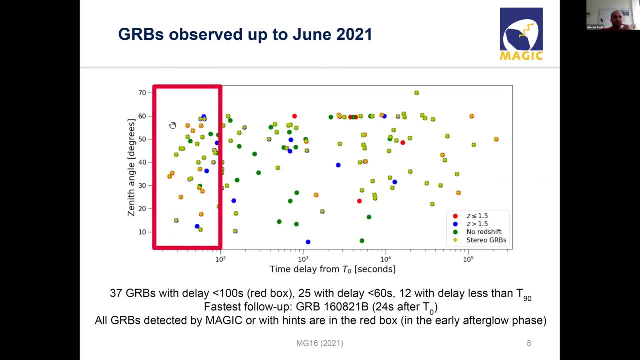 so of course we magic, we are trying to to fill up this red box as much as possible in order, for example, to try to catch the prompt emission, the early afterglow emission and, of course, the afterglow emission. But, as I said before, we have also GRBs followed up at quite late times because we want 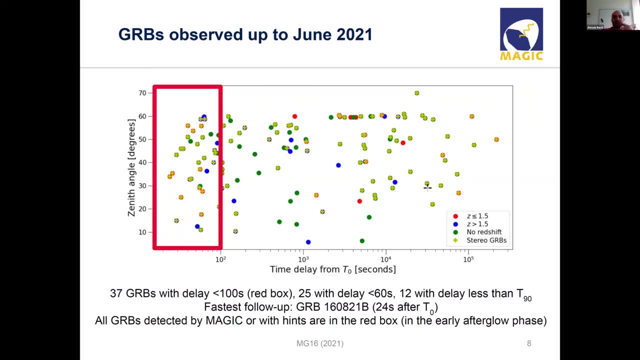 also to try to detect, for example, afterglow emission in the deep afterglow, so quite far away from the onset of the GRB. And just to mention that for the fastest follow-up we have this GRB 160821B, which was followed up 24 seconds after the trigger time of the GRB. 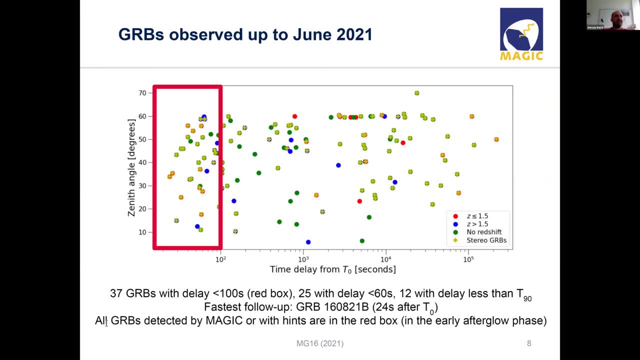 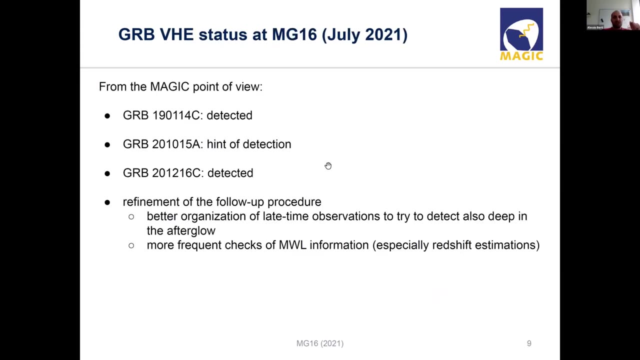 And yeah, just another thing to mention is that all the GRBs which were detected by magic or for which we found some hint of signal, are in the red box, so basically in the early afterglow phase of the GRB. So before I showed you the 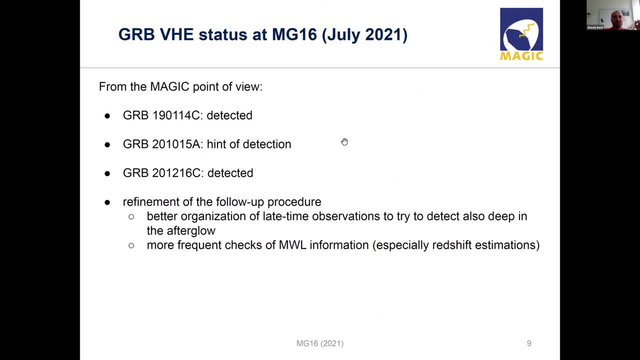 Very Energy status for GRB searches. before at the video: Marcel Grossman meeting in 2018.. This is instead the Very Energy status at this meeting. so Marcel Grossman 2021.. We have a detection from GRB 190114C, a hint of detection from GRB 201015A. 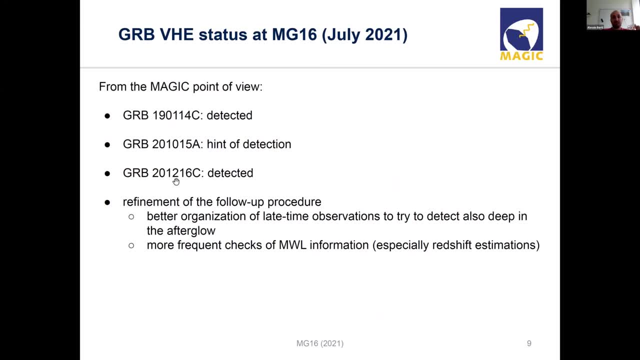 and another detection from GRB jiang持ickenrong 10.4.. from GRB 2012-16C and all these GRBs are long GRBs and, of course, as I said before, but just to stress a bit, we had a refinement of the flow-out procedure after the detection by 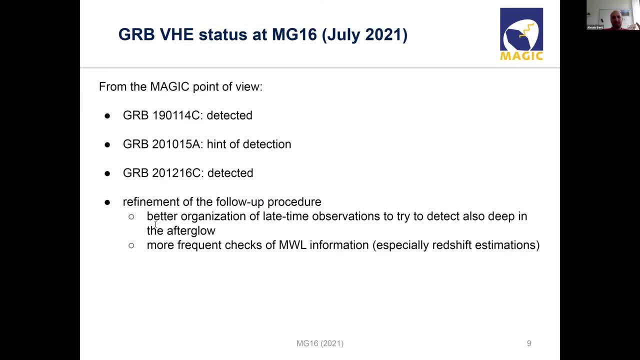 MAGIC, but also the ones by HESS, where we have a better organization of the late-time observation in order to try detect also deep in the afterglow, and then also more frequent checks of the multi-wavelength information that we receive, for example from the GCN circulars, especially. 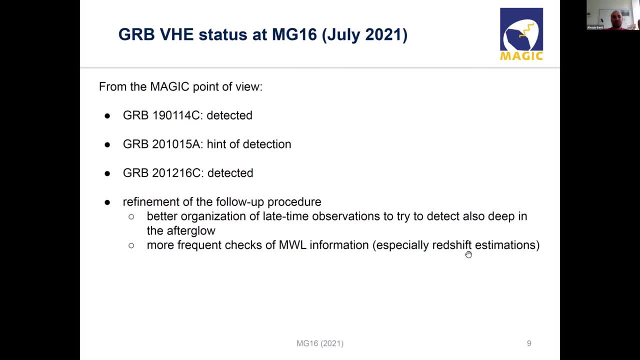 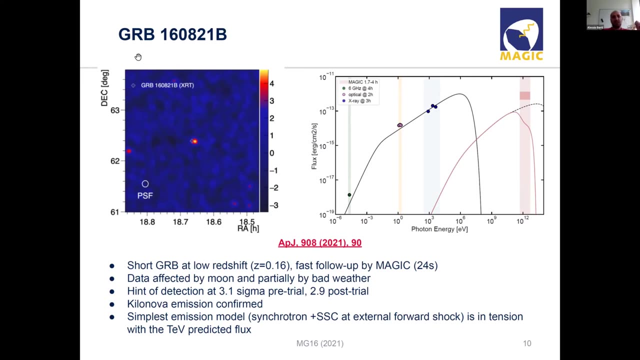 those on the redshift estimations, because we are looking for all the interesting multi-wavelength information to know when and if to follow up the GRBs. basically, As I mentioned before, we had a strong hint of detection from this short GRB, 160821B, and 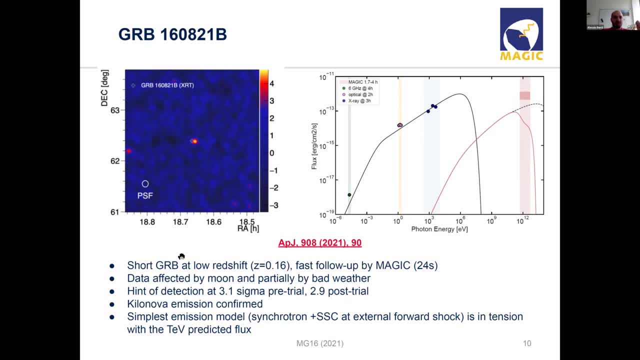 these were quite interesting GRBs. so, as I said, it was a short GRB at quite low redshift, 0.16, and we had a quite fast follow-up by MAGIC, with a delay of only 24 seconds after the onset of the GRB. 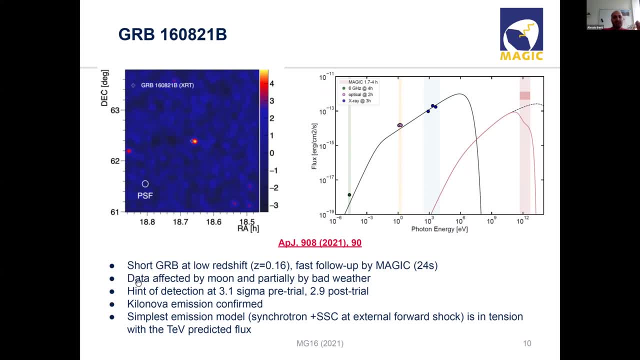 We were a bit unlucky with the weather because the data was affected by moon, so the data is affected by moonlight and also partially by wet weather. in the first part of the observation We had, considering this data, a hint of detection at the level of 3.1 sigma pre-trial, which 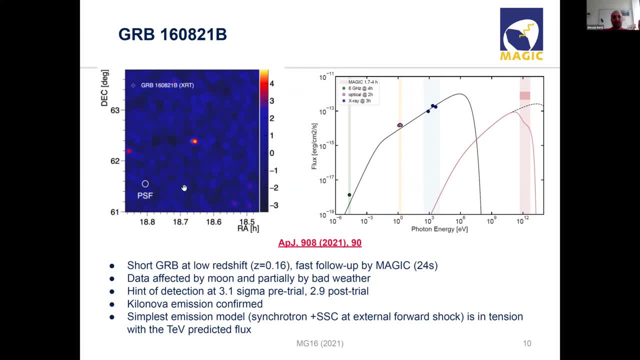 is going down to 2.9 post-trial and this is also interesting, this GRB, because it is one of the few short GRBs with also a kilonova emission confirmed. so, as you know, these short GRBs could be- can be accomplished. 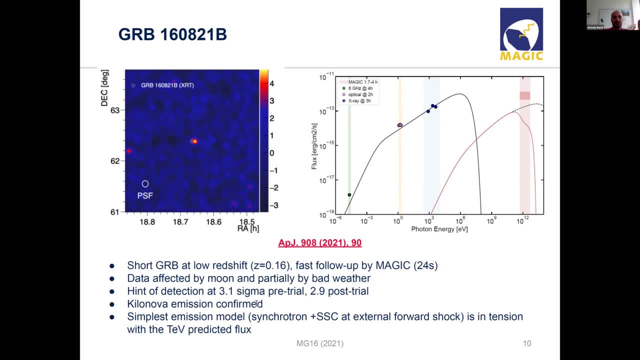 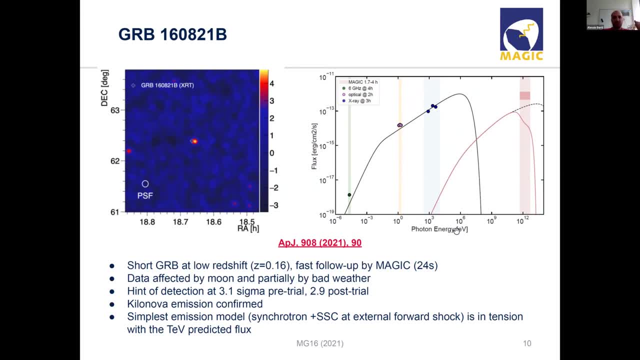 Kilo Nova emission, which was, for example, observed also for this Bionic Neutron Star merger in August 2017.. And what we did with this hint of detection was also to try to model the multi-wavelength data, in particular the radio optical X-ray and also the MAGIC data, with a simple emission. 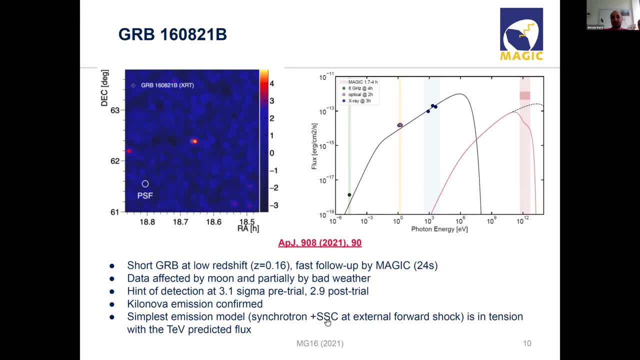 model which is basically considering the short GRB 160821B, the synchrotron and the synchrotron self-compton and external forward shock. but as you can see a bit from this plot, where we have this indicative flux level, from magic, this model is a bit in. 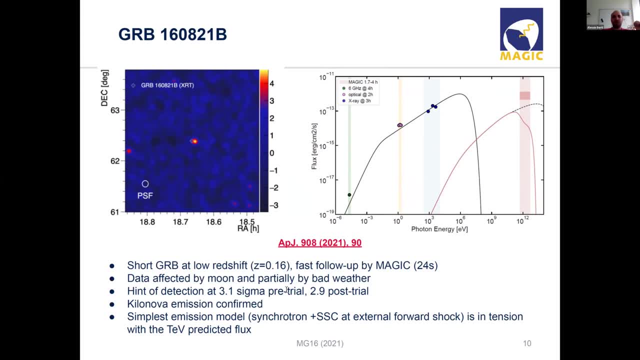 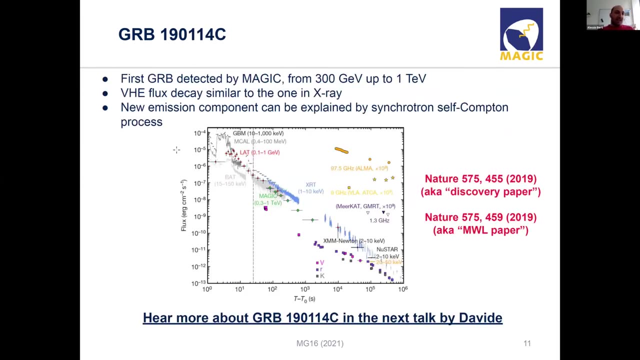 tension with the TV predicted flux. so at least in this case it could be that the emission process could be something different, at least with the standard parameters of the synchrotron self-compton model. and finally, another highlight, from which you will hear more about in the next talk by Davide, is GRB190114C, which is the first GRB detected. 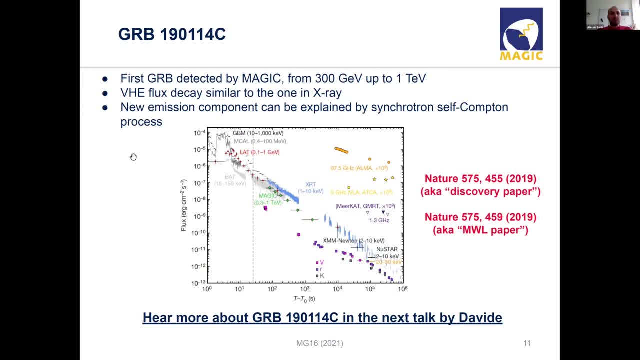 by magic from 300 GV up to 1 TV, in which, basically, if you look at this multiwell line curve, we could see a flux decay which is similar to the one in the x-ray. and starting from this fact and also looking at the energies of the photons, 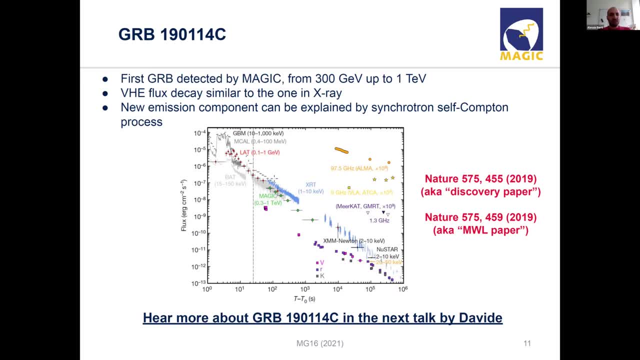 detected by magic, comparing it with the so-called synchrotron burn-off limit, so the maximum energy that photons can reach if they are produced by synchrotron, in this case by electrons. from this we found that the data from this GRB can be described by a new emission component. 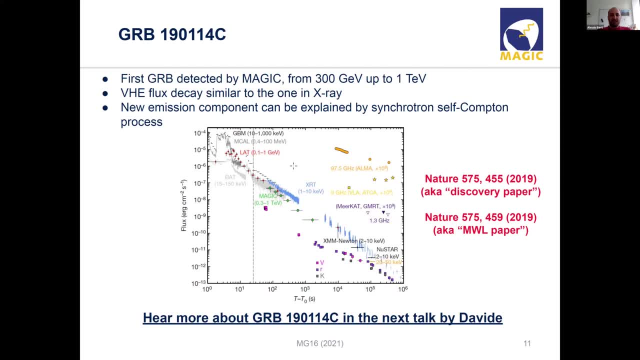 in which we have one component, which is the usual synchrotron emission in the afterglow, but in order to explain the TV emission, we need to add a new component which instead can be explained by the so-called synchrotron self-compton process. 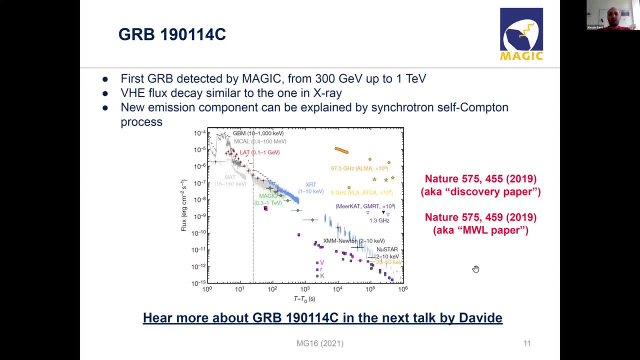 and for this you can have a look, of course, at the two papers. one is more focusing more on the detection by magic, while the other one is also considering all the multiwell lane data taken on this GRB and doing, of course, the modelling, so basically discussing all these. 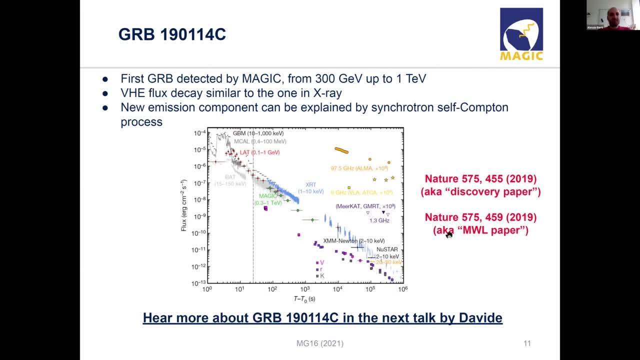 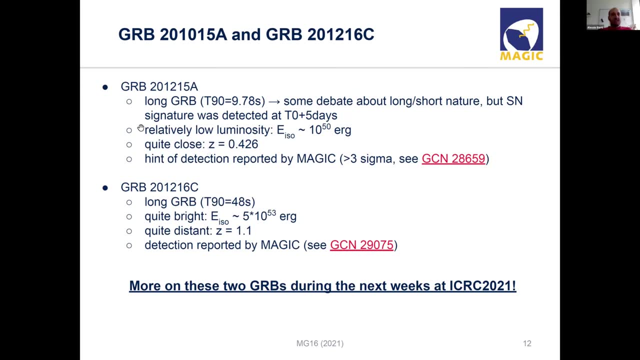 a new emission component in the after love of this GRB. Sorry, one minute. okay, almost finished. so, as i said, we have also these hints from two other GRB. this is one is where jRB20 12-15 a, which is a long GRB2.. 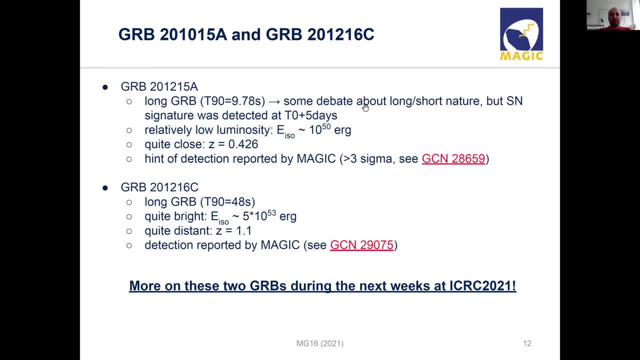 which actually at the beginning, when it was detected, we had there was some debate about its long or short nature, but at the end there was a supernova signature which was detected starting from five days after the onset, which is also this. gb is also quite low luminosity, only, let's say, 10. 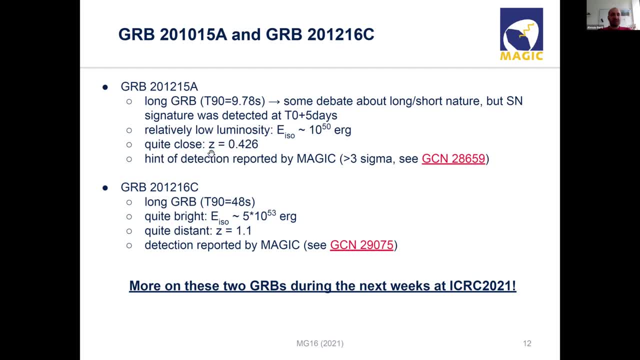 to the 50 ergs and quite close. basically, the ratio is very similar to the one of grb1914c and, as i said, we have a hint of detection reported by magic at a level of more than three sigma. and then, as i said, we had this other detection on grb201216c, which is again a long grb. 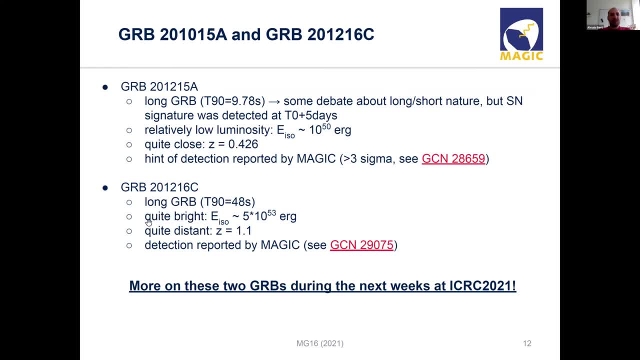 which instead was quite bright. but one of, i think, the most interesting fact about this grb is also that it is quite distant. so at redshift 1.1- and this will make it- is the most distant source detected by ESCTs And of course we have the detection reported by MAGIC. 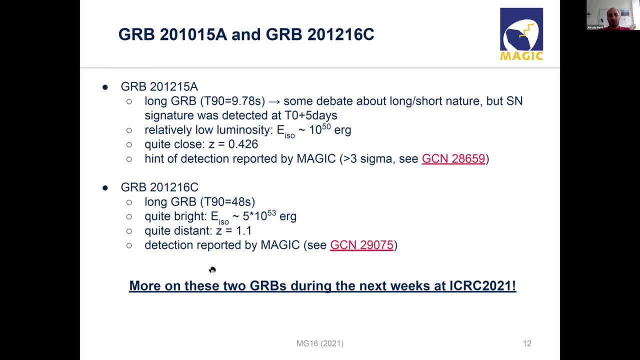 so you can have a look at the GCN And if you want to know more about these two GRBs, I invite you to. if you are participating to the next ICRC, which is starting next week, you will find talks with more details. 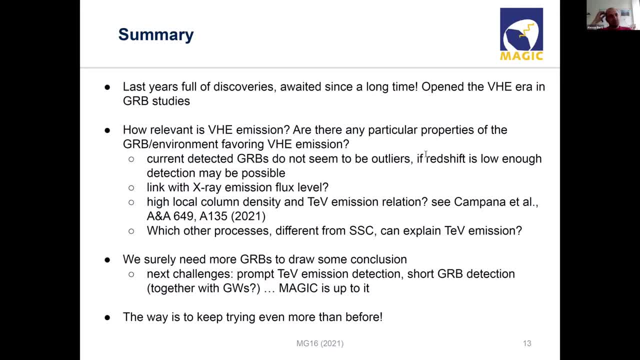 about these two GRBs, And so this leads me to the summary of my talk. So, as you could see, the last years were full of discoveries And these were quite awaited. this is a long time, And we really opened the very energy of GRB studies. 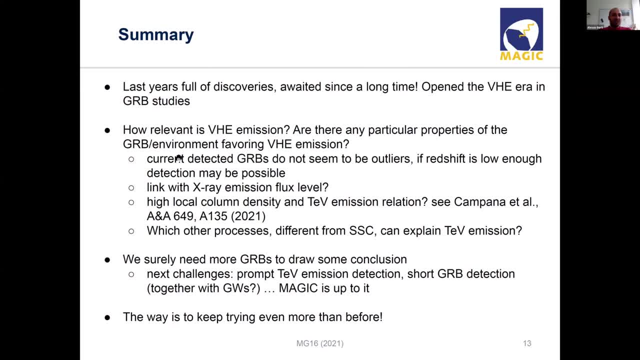 And yeah, basically we could at least partially answer to the questions that I showed in one of the first slides regarding the very energy emissions. So it seems that the current data GRBs do not seem to be outliers among the population of data GRBs, for example by SWIFT and Fermi and so on. 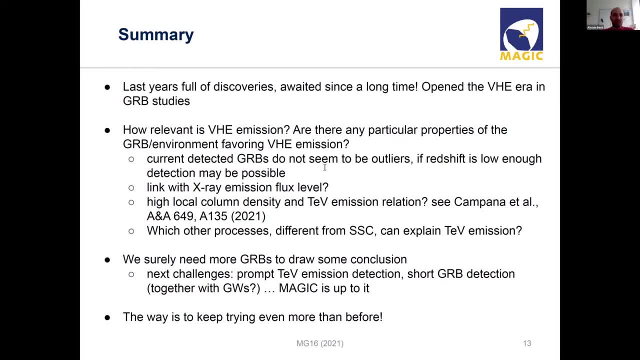 So if redshift is low enough, detection may be possible. We saw that there is a link with the X-ray emission flux level and in general with the temporal decay in X-rays and the TV emission. then there have been recently some papers trying to link. 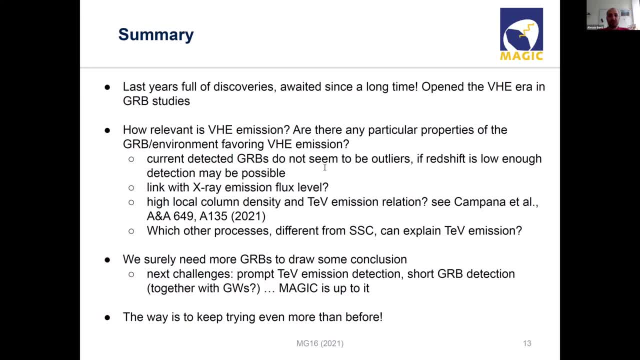 the high local column density and the TV emission, And I leave you here a reference where you can go and check one of such papers. And then, of course, most of these GRBs. they could have been explained with the synchrotron self-compton but possibly other processes. 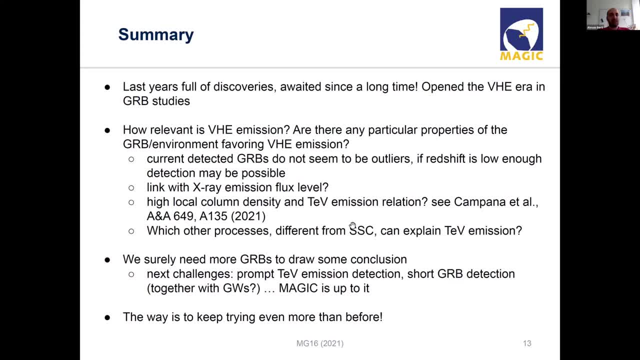 can explain the emission. so this is also an open point And in order to understand more about this, we should really need the more GRBs. to draw some conclusions. And about the next challenges, I want just to report, of course, the one about the prompt TV emission detection. This will be another breakthrough in this field. Also, another one will be the detection of short GRBs, maybe together with the gravitational waves. Okay, we know that the next observational run by LIGO, Virgo and Chagra will be in the future. 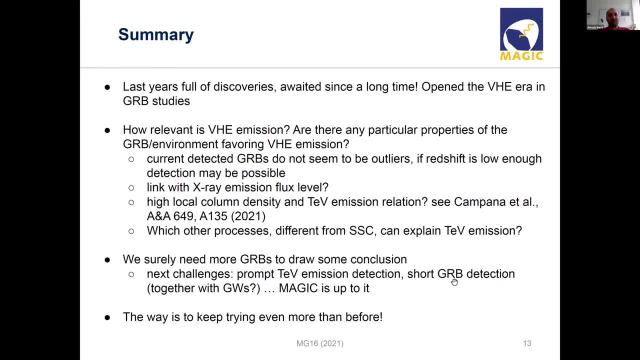 We start the next year, but, yeah, this will be also another breakthrough in this field. And, of course, magic is up to these challenges, thanks, for example, to the fastest viewing that it has. And of course, the way is to keep trying. 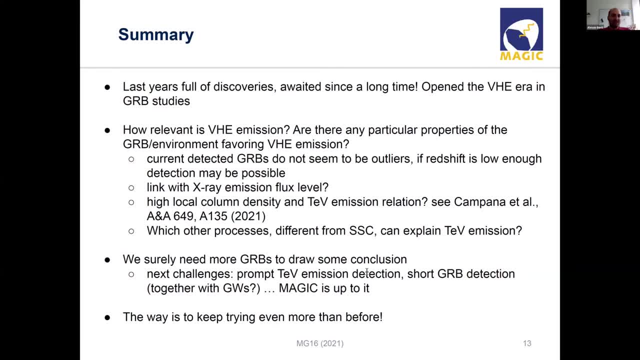 even more than before. So we saw that keeping trying for several years at the end paid off, And so I am sure that keep trying even more will pay off also in the future. And with this I think I'm done. Thank you. 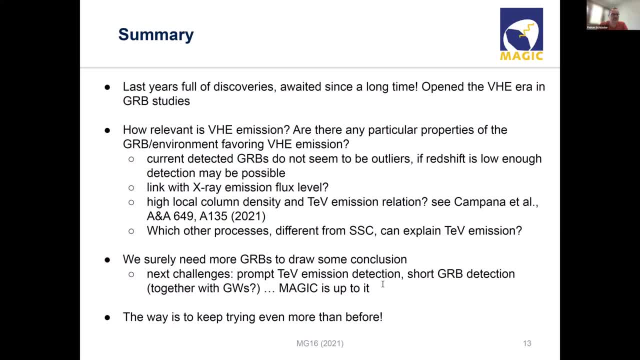 Thank you very much. I am open to questions. Thanks a lot, Alessio. We are a bit short on time, So if there's an urgent question, please go ahead. Okay, Giovanni, please go ahead. Yes, very quick one on the slide read: 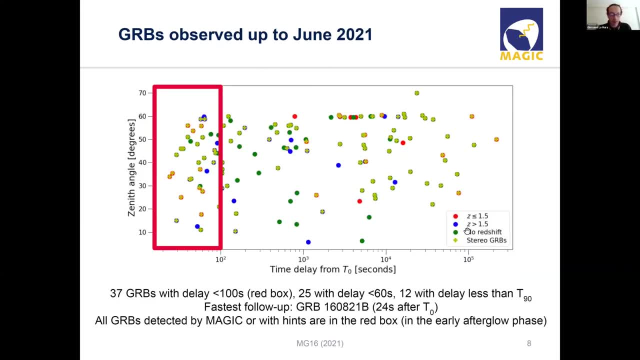 I just wonder whether you have a public repository of the timing of observations or you are planning to have one for the collection of all the follow-up observations of GRBs. OK, You mean only about the timing. So the delay? Well, Yes, the time at which GRBs have been followed up. 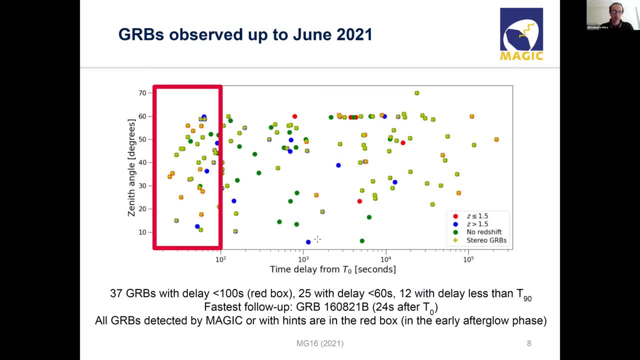 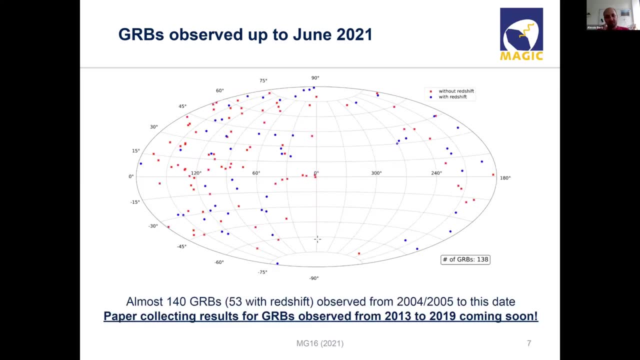 because that might be important for the estimates of detectability. OK So, A full catalog? I think not, But as I mentioned here in slide seven, we have this paper on which we are working on, which is collecting these GRBs from 2013 to 2019,. 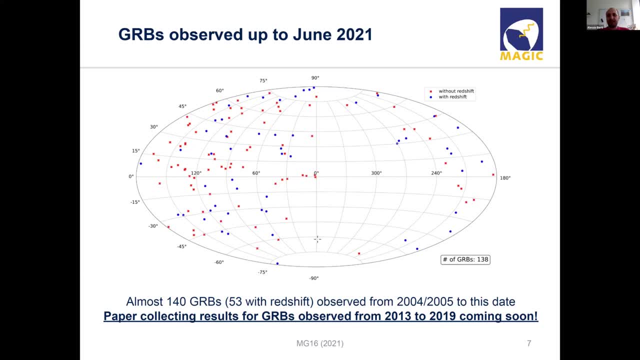 in which, of course, all this information about the delay and let's say how fast we could react, and so on will be surely present, at least for these GRBs- For past GRBs, we could think about what to do with this information. 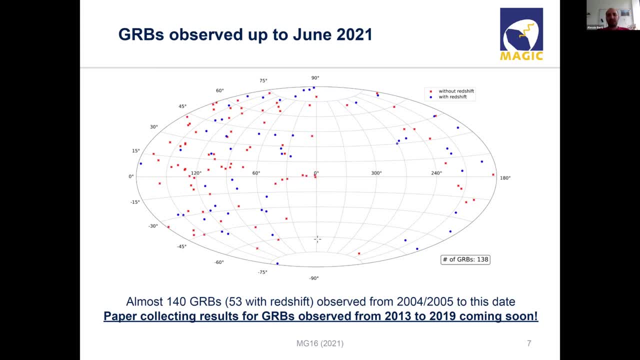 Because, as you said, this will be important also, for example, for the next generation Cherykov telescope. So I am thinking about LST, I think probably that's also what we are thinking about. So, yeah, And for instruments as well. 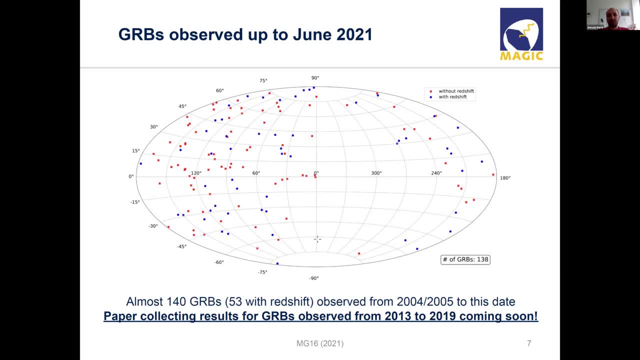 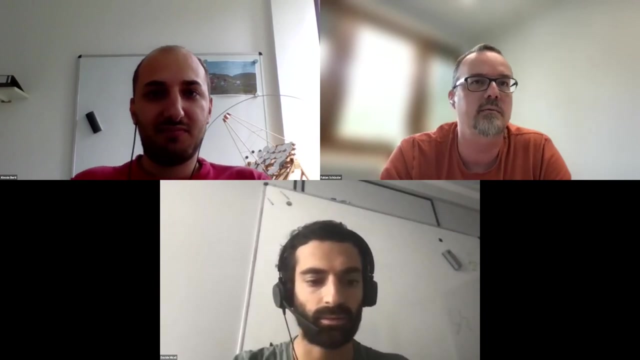 Yeah, of course. So, yeah, this could be an idea on how to use these, let's say, statistics that we have about the follow-ups. Yeah, Thank you. OK, Thanks a lot, We have to move on. Davide will report on the golden GRB detected by MAGIC190114C. 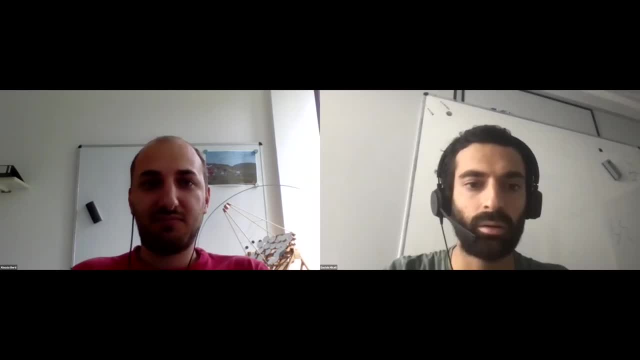 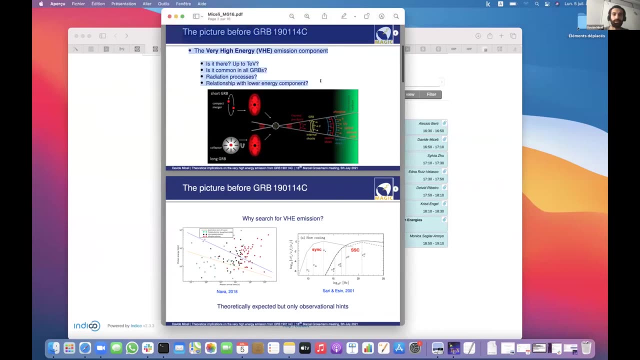 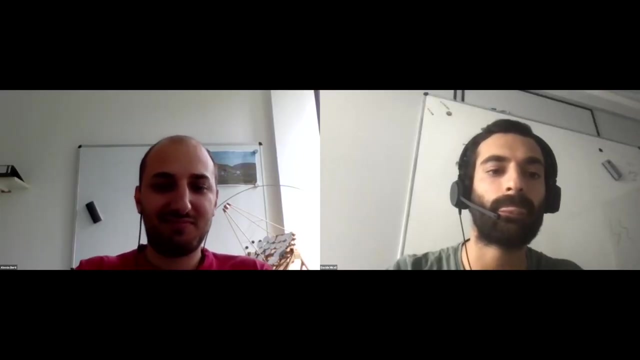 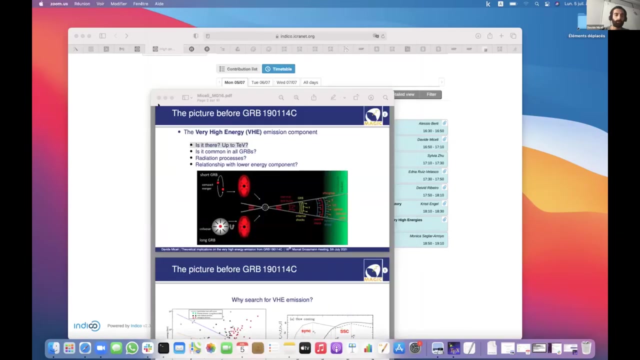 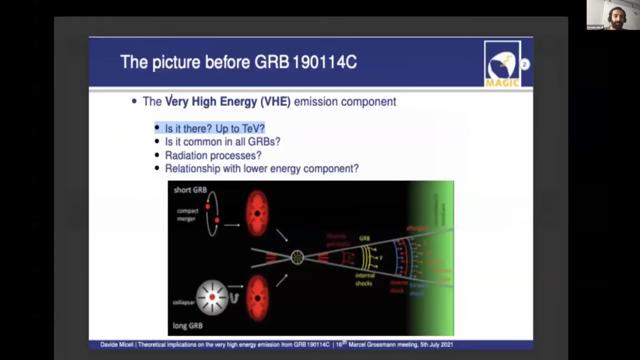 Yes, OK, Can you see my screen? Yes, I will put now, Whoop, I will put to full screen. Sorry, I have a problem. Oh, no, And okay, now you should see full screen. Yes, Yes, please go ahead. 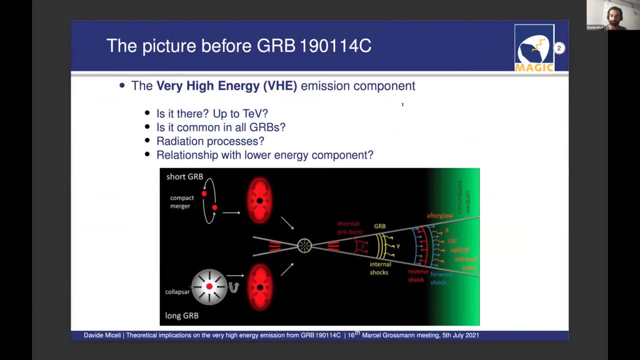 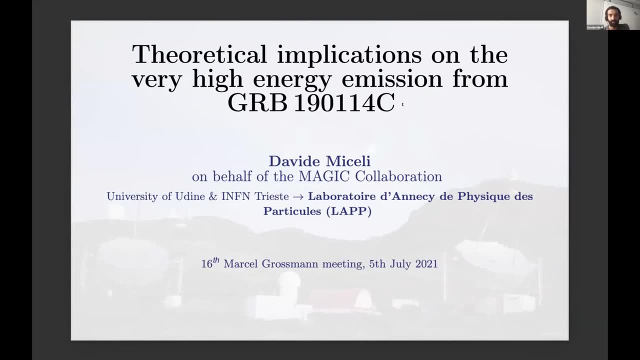 Okay, So, yes, so good afternoon or good night or good morning to everybody. This talk will be devoted to the study on the magic dataset that have been derived from the observation of gamma-ray burst 1901-14C. I will focus this talk on the conclusion. 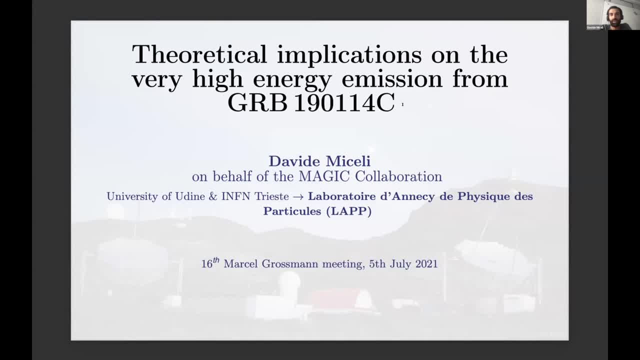 that could have been derived from the TEV datasets and also on the physical implication that have been derived also considering the magic dataset together with the lower emission at the multi-wavelength band. So if we do a little step back in time, before 1901,. 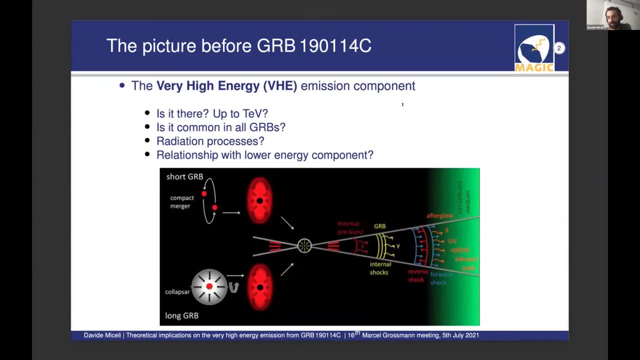 before 14 January of 2019,, as also Alessio talking in the previous presentation, the situation from the GLB side was very, very different from the current one. So the lack of observational, observational proofs from the very high energy side. 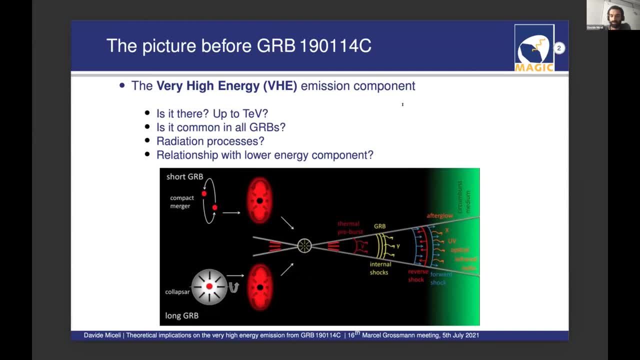 despite a very, very nice model, was presenting the gamma-ray burst emission in the lower energy bands and the very high energy components. So we had open several questions about the very high energy components. So it was not clear if this component was there And even if the extension of this component 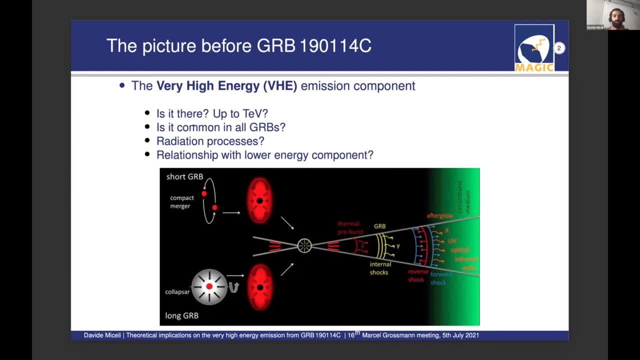 it would be a reach that the TV energies- And there was also discussion about how much this component could be considered common in gamma-ray bursts and debates on the possible radiation processes responsible for these components And also, together with that, the relationship that this kind of component could have. 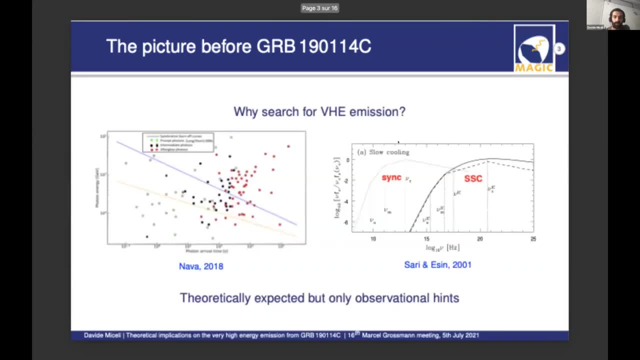 with the lower energy emissions, And from both the observational, theoretical point of view, is it indeed true that there were several studies which point towards the idea that this very high energy emission was indeed present? The Fermilat photons could hardly be reconciled with the synchrotron emission. 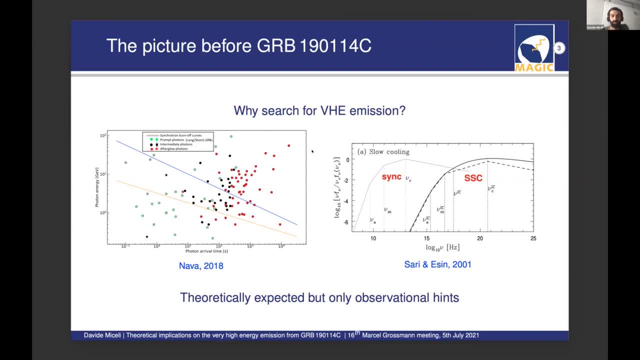 that was seen to be the promising, the likely radiation mechanism responsible to describe the emission in from radio up to x-rays, And these photons observed could explain very difficult, with difficulties, considering the synchrotron emission And from the theoretical point of view. 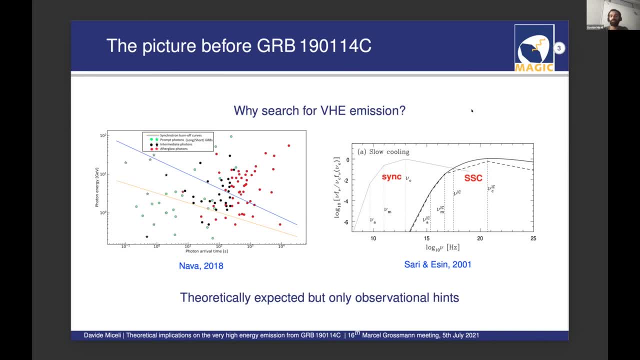 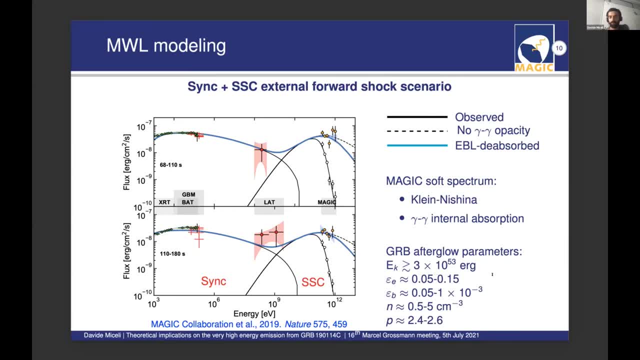 could explain very difficultly with difficulties considering the synchrotron self-compton. could explain very difficultly with difficulties considering the synchrotron self-compton. fill in the typical range which was used for old modeling of the data from the radio up to X-ray. 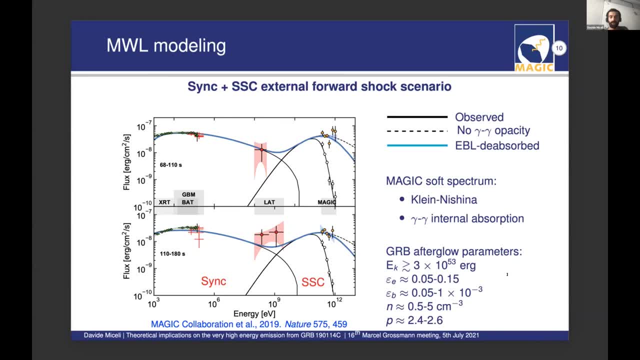 And these results also point towards the idea and the possibility that this synchrotron self-compton component, this TV emission that we have seen, could be somewhat universal, so somewhat typical to several gamma ray bursts and common and therefore we could increase more the detection. 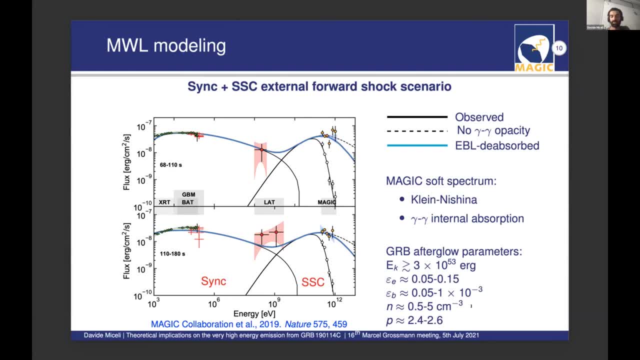 in the future, And this actually was happening, since now the number of gamma ray bursts is increasing. Moreover, what we can derive from this modeling, as we can see here from rough estimation, the power emitted in the TV range is more or less at the same level of the power. 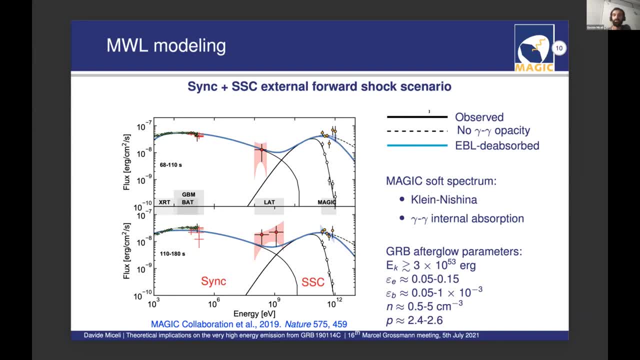 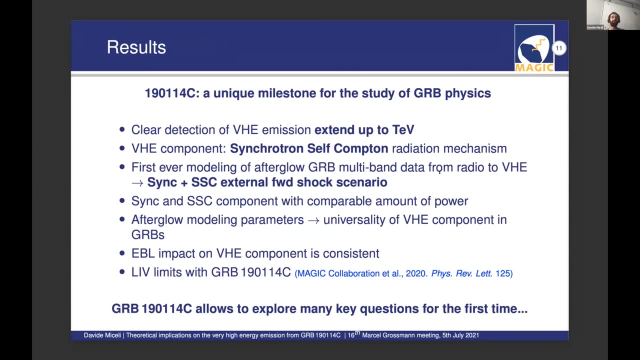 emitted by the synchrotron component And therefore again, we 190114C results were a unique milestone for the study of gamma ray bursts and it gave us the possibility to point and to explore for a first time several important questions on gamma ray bursts. 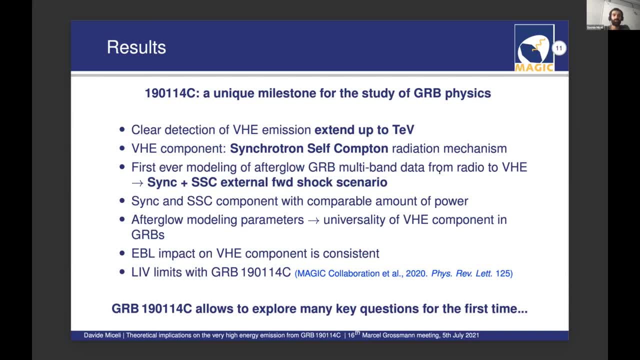 In particular it was part of the- was detected a very high energy emission extending up to the TEV range, and the radiation mechanism which, for this GRB, was explaining consistently the behavior of the very high energy component is the synchrotron self-compton. 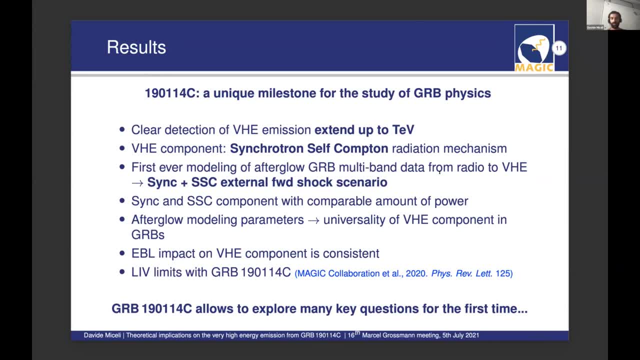 which has also the powerful effect, together with the synchrotron emission, to explain the afterglow of the gamma ray burst in a multi-wavelength approach for the first time, so collecting all the data from the radio up to very high energy, assuming the external forward shock scenario. 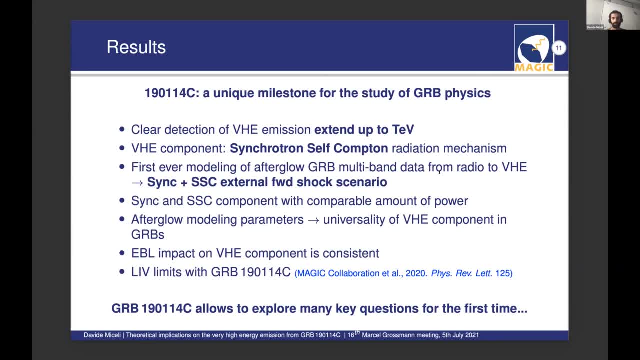 From the physical interpretation of the results. what we have seen is that the synchrotron and synchrotron self-compton component present a similar amount of energy radiated, and the afterglow parameters point towards the idea that a universal 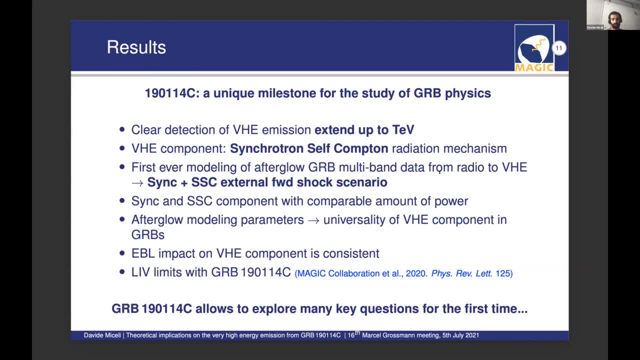 very high energy component could be present in gamma ray burst. Some side studies also shown, as I've seen, the impact of the extragalactic background light on the very high energy, especially when going up to the TEV. and also just to say that the gamma ray data sets of 1901-14C- 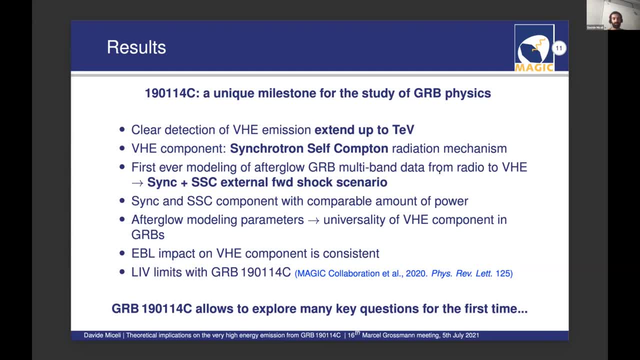 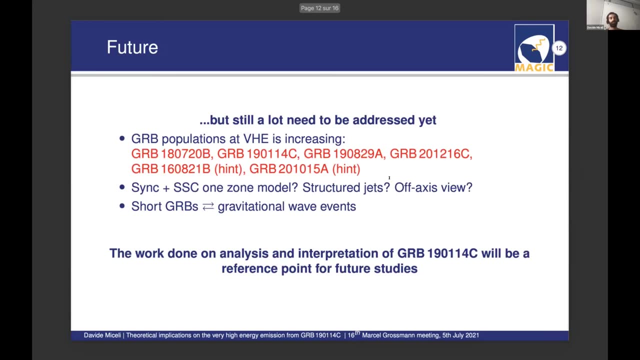 was also used to derive limits on the Lorentz invariant violations and the metric. A collaboration has also published a paper concerning these results And anyway, as also mentioned before and as we will mention in the next talk also, a lot of things are still not addressed. 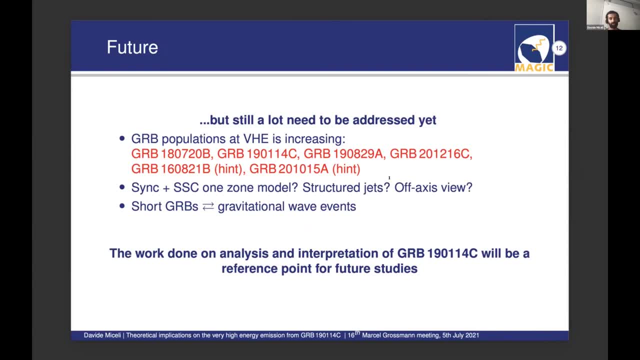 And in fact the gamma ray burst population is increasing. Currently there are four gamma ray bursts detected and two with hint of detection And, in this new context, the work which was done for the interpretation of 1901-14C. 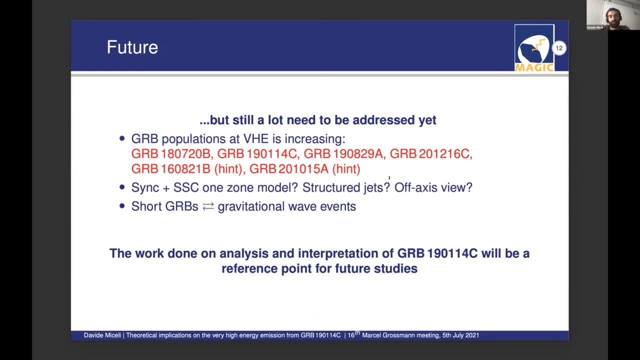 could be seen as a reference point, a reference starting point for the future studies that will be surely, and are already published, on these new events and, we hope, also for the future one that will be detected by the current and future instruments, These events, 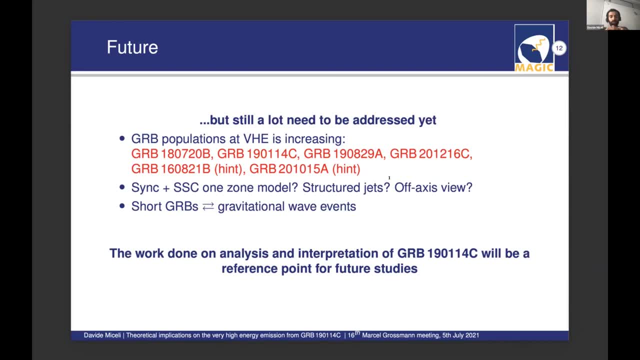 these new events could also be important to explore in more detail the theoretical models which currently are thought to explain these very high energy components. So is the synchrotron plus synchrotron self-compton emission in one zone model valid to explain all the emission? 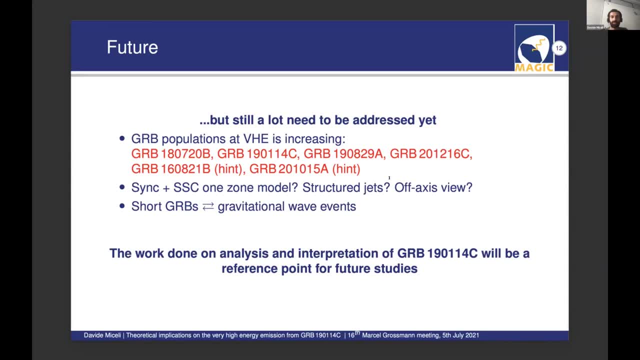 or should we claim for some more sophisticated structure like the structured jets? or we should take into account also the effect of the viewing angle. This is something that will be surely part of the discussion for the future. detection of and analysis, interpretation of gamma ray bursts. 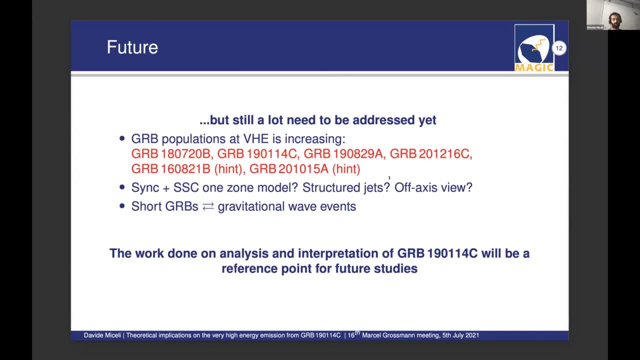 And yes, I also mentioned, as also in the other talk was mentioned before, the important relationship that connect the gamma ray bursts with gravitational wave and this could give important information from the sides of the physics of gamma ray bursts. and this could give important information from the sides of the physics of gamma ray bursts. 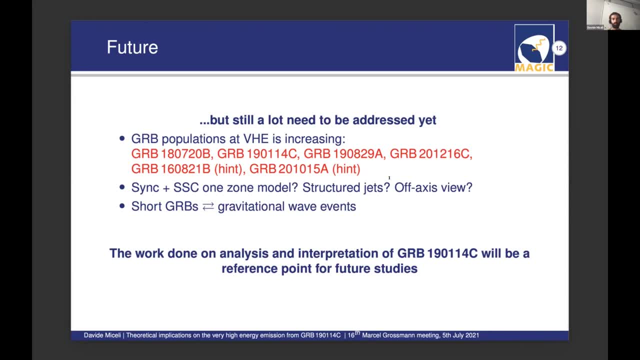 not only on the interpretation of the very energy emission component, but also on the connection of their progenitors. And so this is the end of my talk And if you have comment of question, please. Thanks a lot, Davide. Is there an urgent question by somebody in the audience? 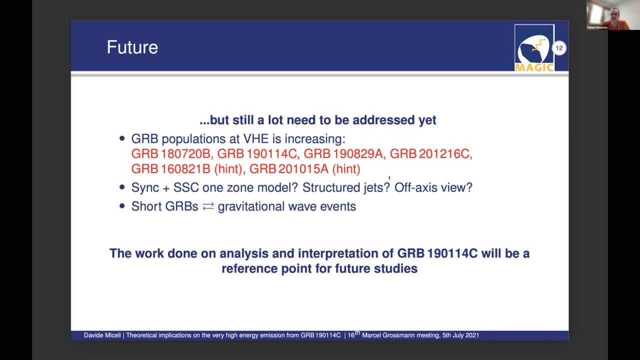 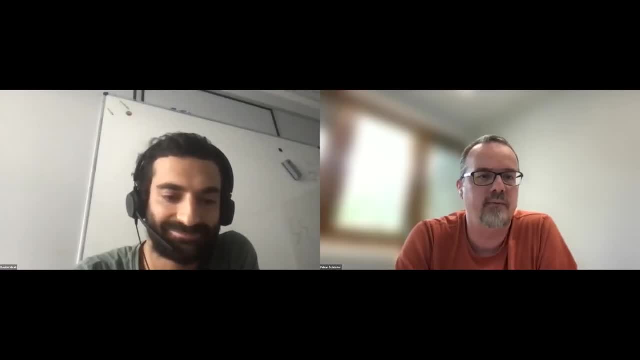 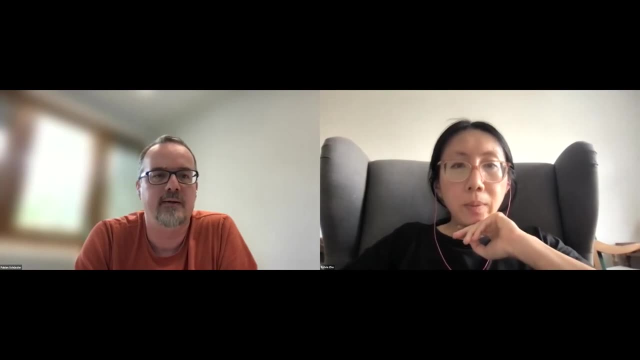 I don't see any raised hands, Then in the interest of time, let's just move on. Thanks a lot, Davide. You're welcome. Very interesting, Silvia. can you report on the HES-GRB program? Hello? 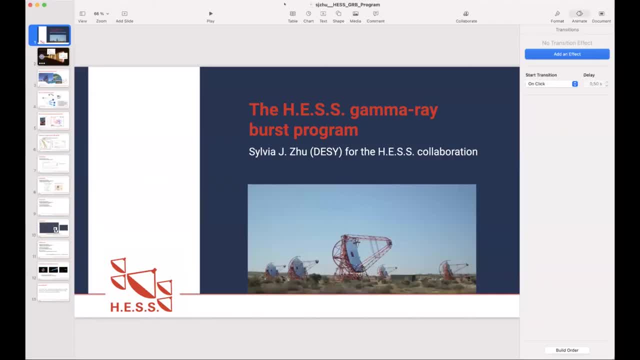 Let's see Sharing screen. Luckily, I think I'm going to be slightly under time, so hopefully that will be okay for everyone. That's very helpful. All right, Hold on a second, All right? Okay, I'm just going to start talking. 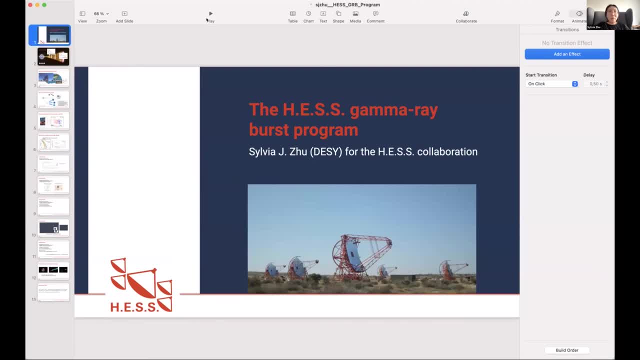 Hi everyone. I hope you're all having a good time. Yeah, I'm here to talk about and just summarize the HES-GRB program, And many thanks to Alessio and Davide who have given really great overviews. 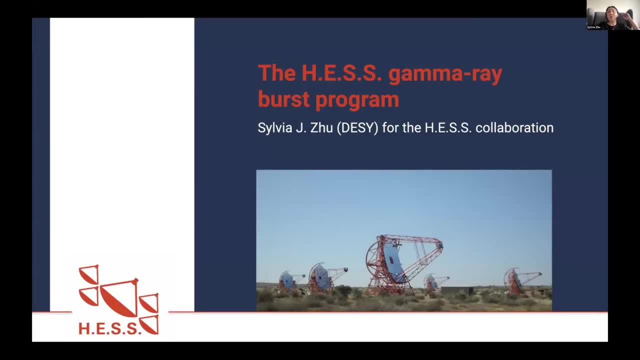 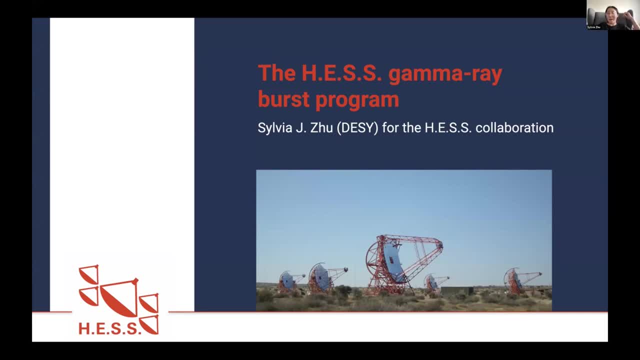 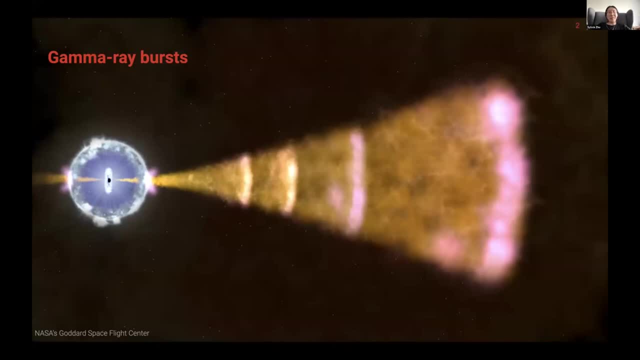 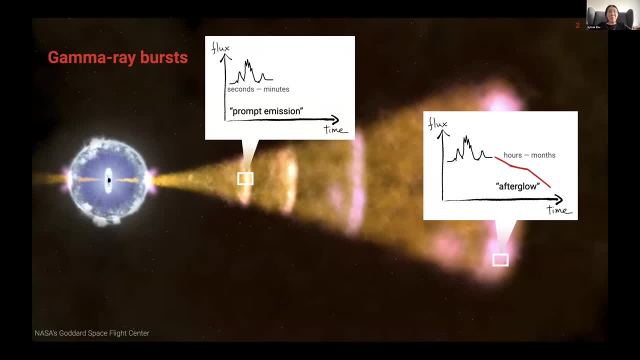 I believe I've seen a version of it already in Alessio's talk, But basically, right, when we talk about GRBs, we talk about prompt submission that is lasting for seconds to minutes, and then we talk about afterglow emission that could be observable for hours. 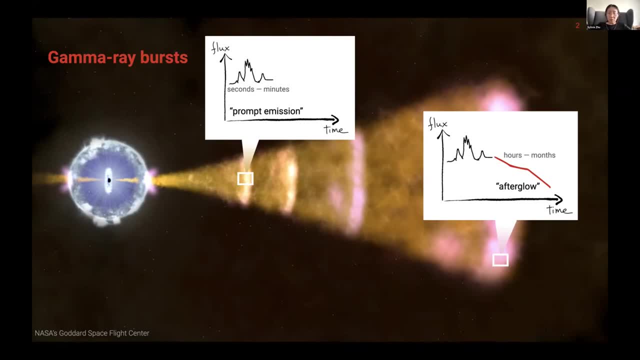 to months afterwards, Of course, when we were talking about VHE observations, of GRBs for – it's perhaps natural to expect that we should be looking earlier, so focusing on the prompt submission, perhaps, perhaps, or the early afterglow, and so this is a natural assumption to make and this 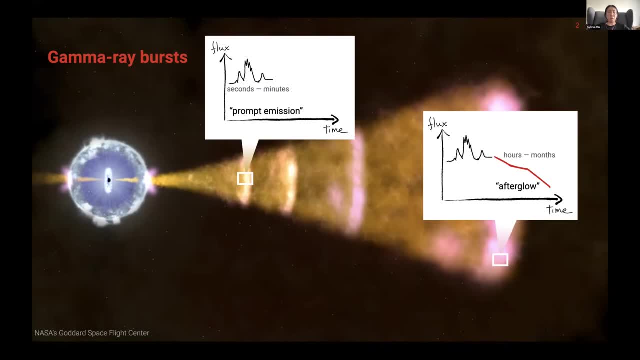 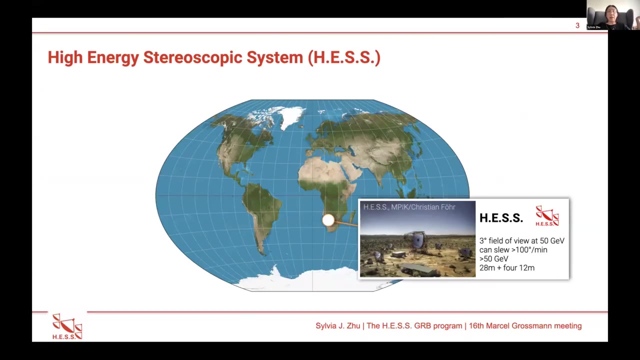 is something that I think all of the VHE instruments were making. As was mentioned before, MAGIC has only recently started to look at GRBs after four hours, and HESS has done a similar thing. So HESS is short for the High Energy Stereoscopic System. 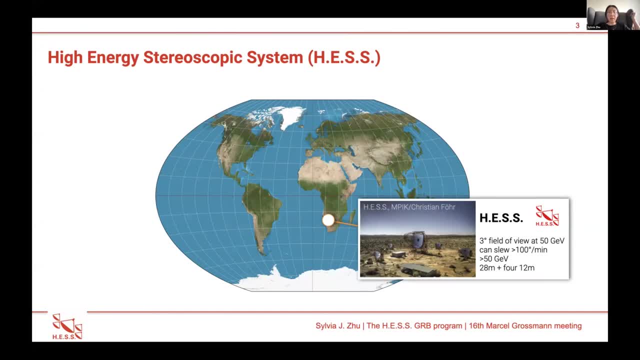 It is a set of five telescopes in Namibia and it's currently the only set of IACTs in the south and the southern hemisphere, which is great because it has a complementary view of the sky as MAGIC and VERITAS. These five telescopes consist of four smaller ones that have a higher energy range and 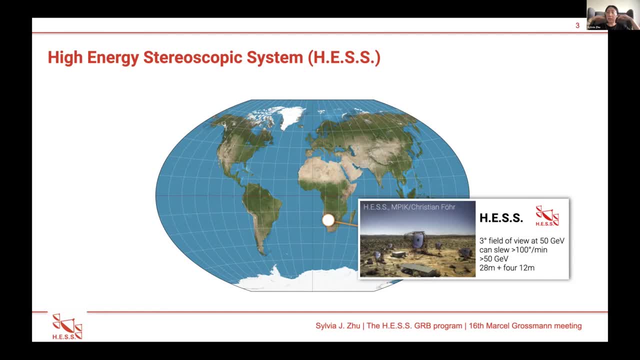 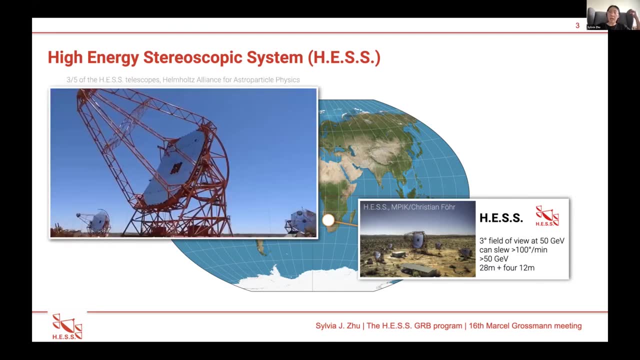 then a 28-meter one, the largest one, CT5, that has a lower energy range. It can go down to some tens of GeV, And while the HESS telescopes are not as agile as the super-agile MAGIC telescopes, I think 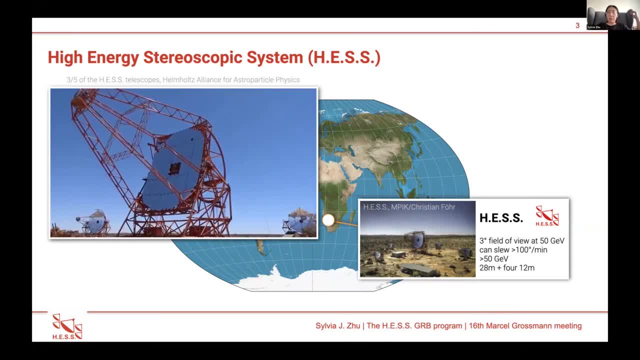 we still do pretty well. So here you see a video of- I believe this is in real time- of the enormous monstrosity of steel CT5, slewing pretty quickly And this so, as was mentioned before, this fast, rapid slewing is important because, of course, IACTs don't have 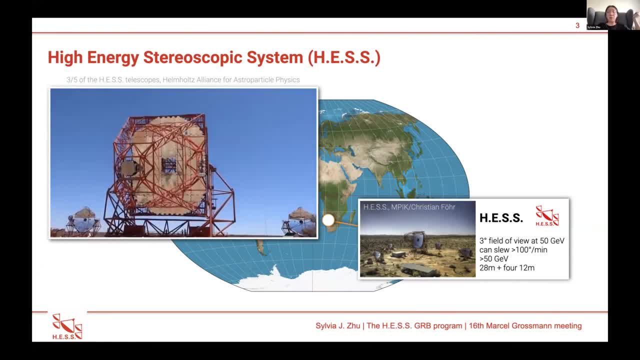 very large fields of view. right, We have fields of view that are about a few degrees radius, which means we don't see a large part of the sky. Well, we see a patch of the sky at any time. We do not see large fractions of the sky. 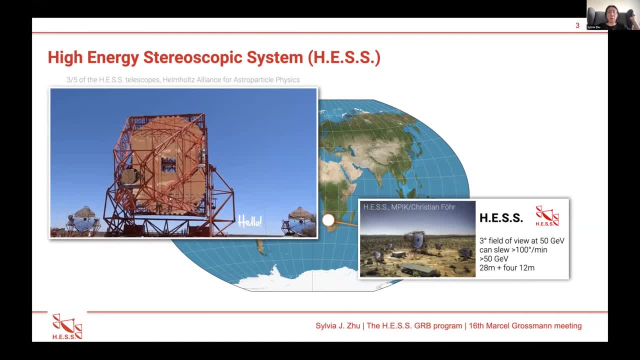 This means that we depend on other instruments, on large field of view instruments, to actually detect things for the most part, or to detect transients and then communicate those detections in some way to us so that we can observe them and repoint to the parts of the sky that they're. 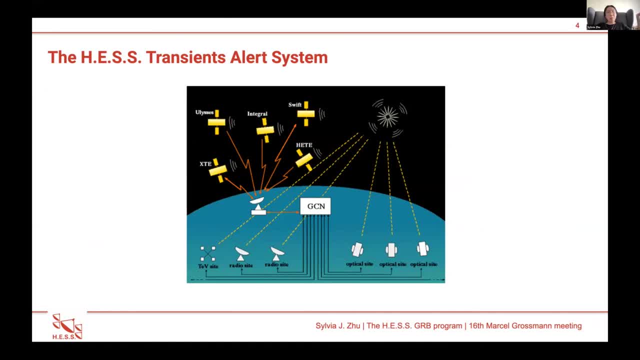 in. So just a quick summary of how the HESS Transient Alert System works. Actually, right now, what you're seeing is an image. if you go to the GCN website, you can see this rather old diagram of how the GCN system works. 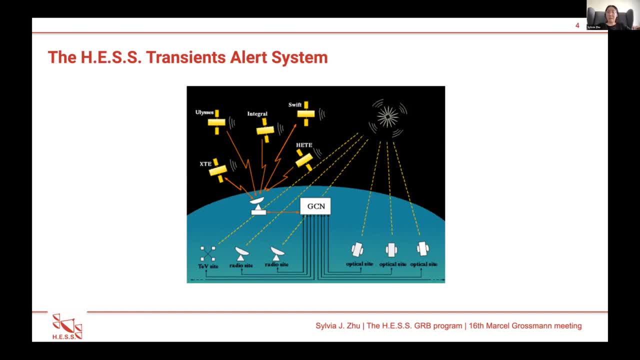 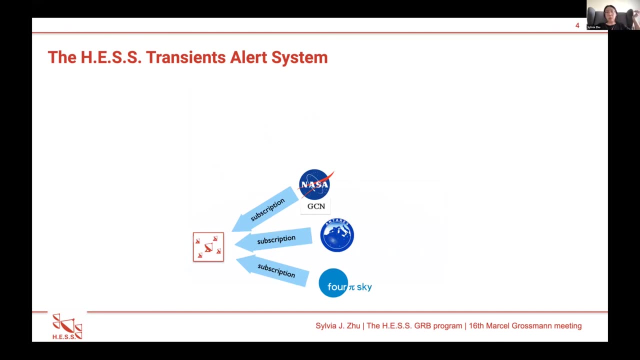 And up there we have some satellites, including ones that are no longer running, but also ones that are still up, And at the bottom we have, for instance, a TEV site, And this TEV site could be HESS. So HESS, of course, gets GCN notices or has a subscription to GCN notices. 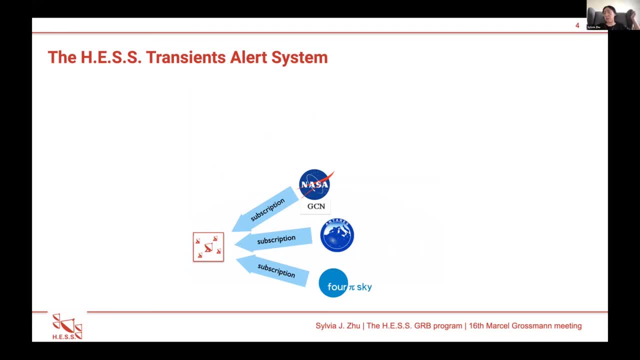 And so when these notices come in, for GRBs, for instance, or other types of transients, then the HESS Transient Alert System can make the decision whether or not to observe and, as well, informs the people, informs the humans, to make decisions about whether or not to. 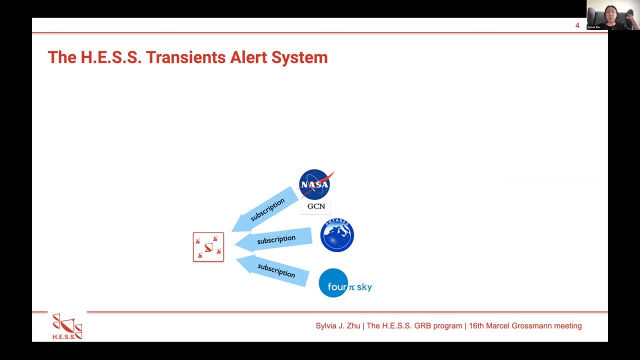 observe. Besides GCN notices, HESS is also subscribed to GCCN. Oh yeah, And so they can send notices to other observatories like Antares, as well as other brokers like 4Pi Sky, And HESS also receives direct notices from IceCube. 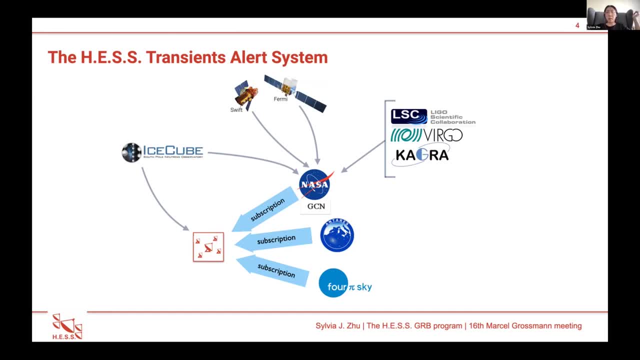 And as well IceCube, of course, along with other electromagnetic observatories, as well as the gravitational wave observatories, send their notices through GCNs, And so, through all of this, we have multiple ways of getting information about transients being detected. 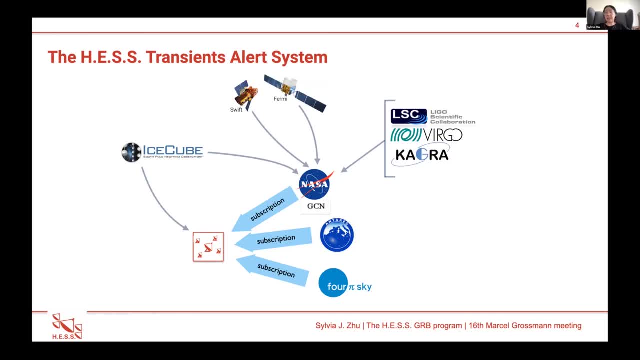 And, of course, this is not just GRBs. This is many different sciences, This is many different systems. This is many different systems. This is not just GRBs. This is many different science cases. The HESS Transient Alert System: it's a fully automated system which is necessary because 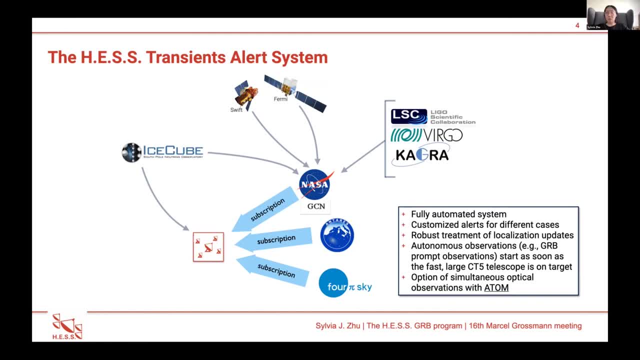 transients, and especially transients at these timescales you need to make fast reactions, So you want to automate everything as much as possible. In addition, the alerts are fully customizable for the different cases, And this is not only different science cases, because you want to treat your gravitational 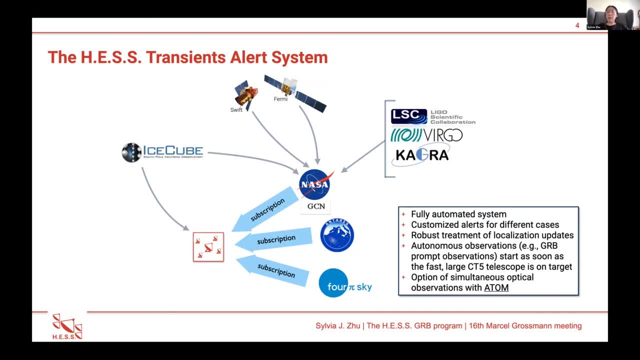 waves differently from your fast radio bursts, but it's also customized for different or customizable for different systems. So you want to make sure that you're not just alerting telescopes because maybe you want to treat SWIFT-BAT differently than you treat Fermi-GDM. 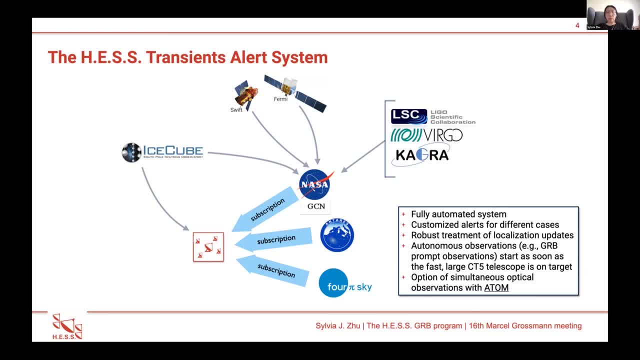 We also have a robust way of treating localization updates. So for some of these telescopes and some of these observatories, the localization changes over time and we are able to react to that and treat that in the proper way. So we talked about- so I mentioned before- about how it's reasonable to assume that you 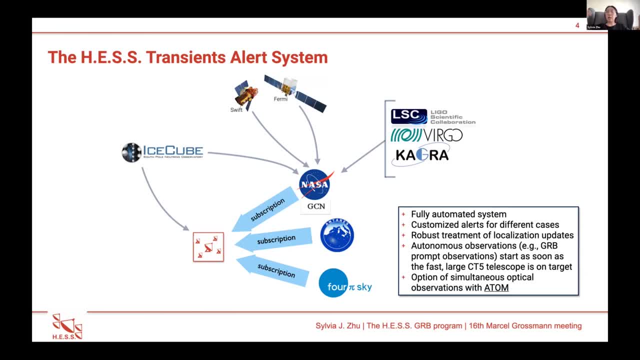 want your observations to start as early as possible, So of course you also want autonomous observations, so you want the array to move automatically, And this occurs, for instance, for GRB prompt observations, and these can start as soon as the fast and large CT5 telescope is on target. 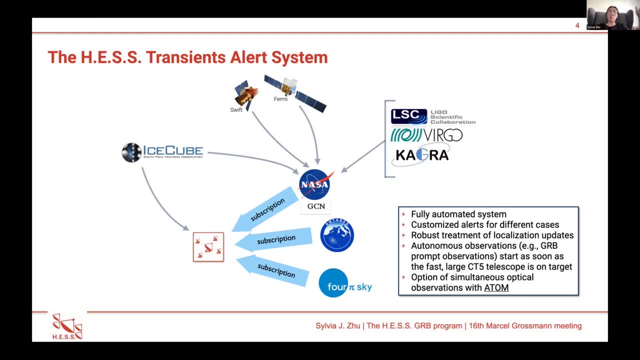 So this means that if we're doing something else, the array is looking at its normal target. we get a prompt GRB trigger, then the array immediately slews and as soon as CT5, which moves the fastest, is on target, regardless of what the other telescopes are doing, we 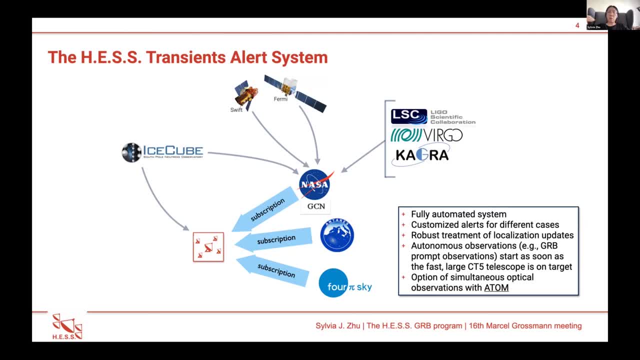 start taking data. So this makes us more streamlined, more efficient and just using the time as best as we can. And at the HESS site there's also a completely automated autonomous robotic telescope, ATOM, And with ATOM we also have the option then for depending on what observations we're. 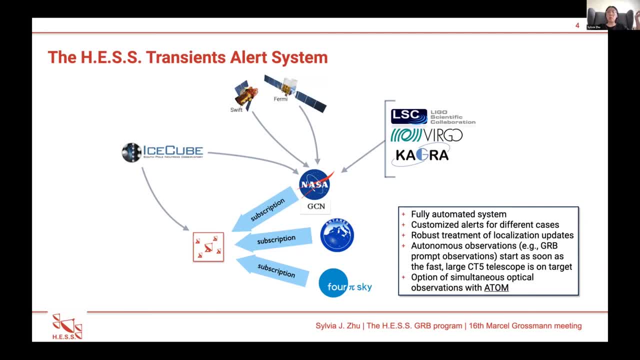 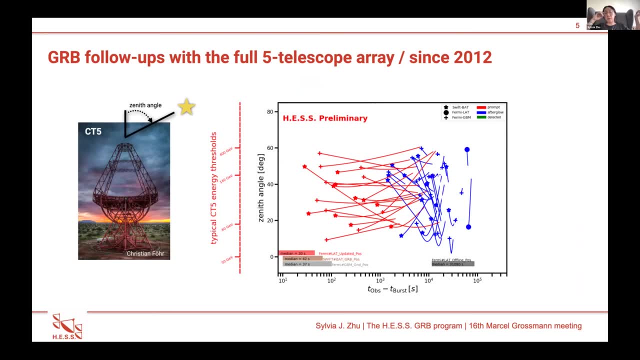 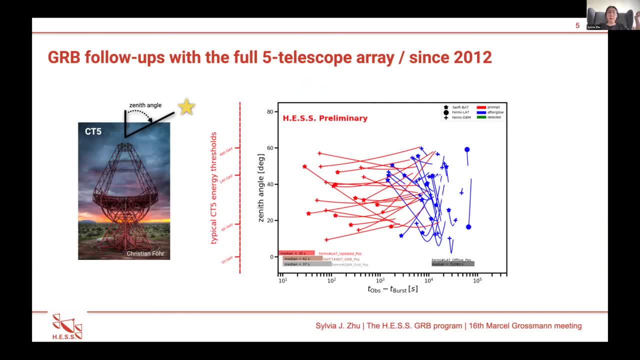 This is the full five telescope array. This is the full five telescope array, And what you're seeing here is a plot of all the GRBs that HESS has followed up since then with the full five telescope array And the different let's see. no, yeah, 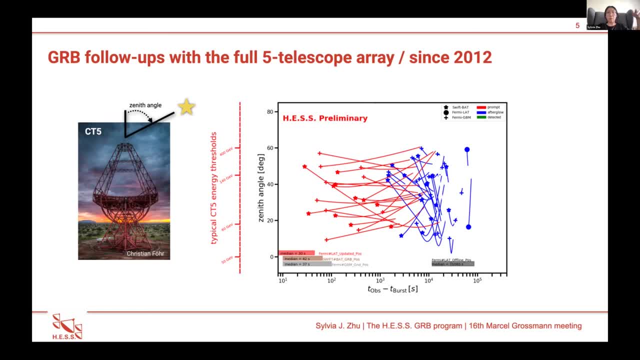 So the vertical axis is the zenith angle of the GRB, which is just the angle from the vertical, And of course, when you have a lower zenith angle it's more directly overhead And so you can probe it down to lower energies. 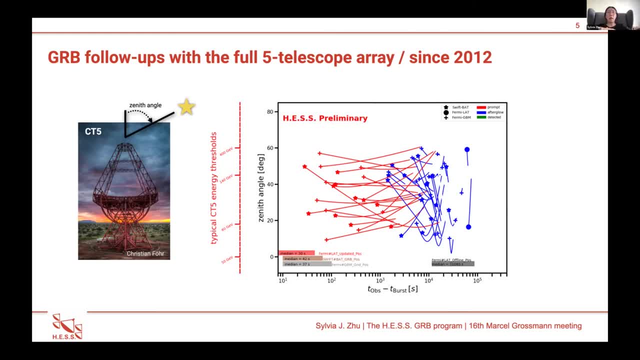 You have a higher zenith angle, Then you can- only you can go. you can't go down as low in energy. What you're seeing here are GRBs that are have were followed up by HESS in these years, And the stars are swift bat GRBs. 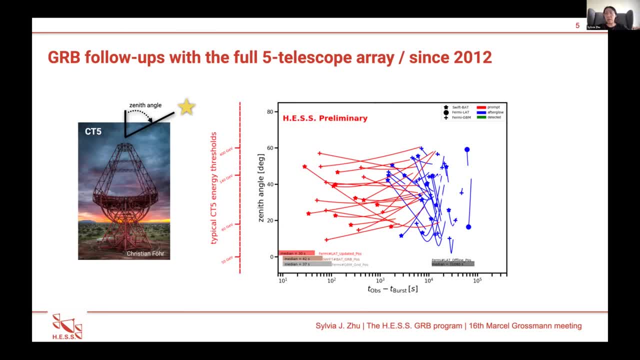 The crosses are Fermi-GBM GRBs, The circles are Fermi-LAT GRBs And most of our about- I think about 60% to 80%, depending on the definition of our GRBs that we follow up- are bat GRBs. 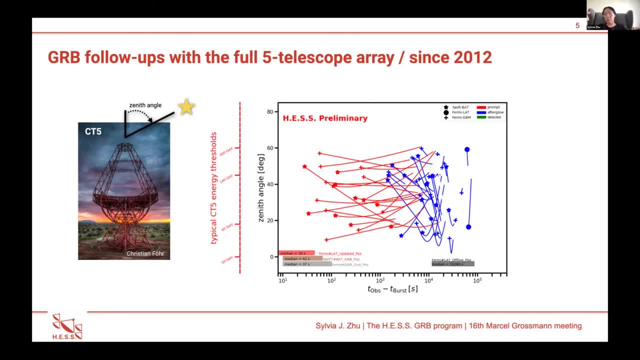 And we also follow up GRBs by other instruments as well. But these are just the main ones. the let's see the red points and lines just show how the zenith angle changes over time for prompt alerts. So these are so. so this is slightly different from the typical GRB definition of prompt. 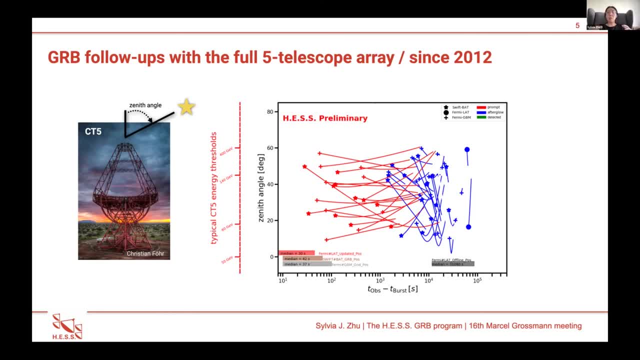 versus afterglow Prompt essentially just means autonomous reaction. So the red are the GRBs for which we had autonomous reactions. The blue are the GRBs for which we had some manual decisions later, because maybe at that point, maybe at you know, you want to make some more. 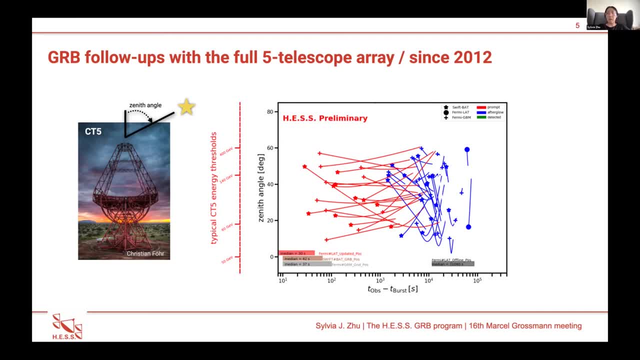 Information based on what other GCNs have come in um until that time. So, of course, this was what it looked like up until mid 2018.. And then we suddenly got a couple of VHE GRBs and life is great now and we are all. 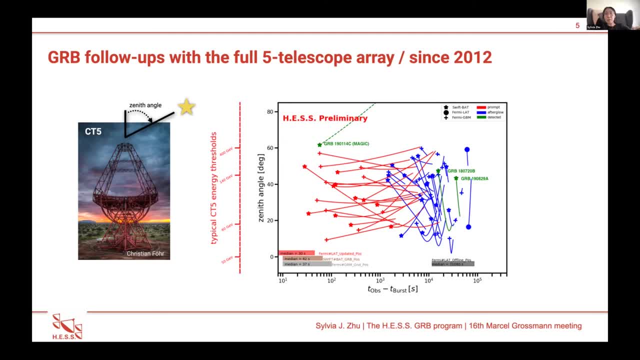 celebrating in VHE GRB world. Um, the first GRB that was detected by Hess, uh, was 1807-20B, this green one on the right, Um, and let's see, Yes, Yep, And then, uh, we also have 1901-14C on the top left, which unfortunately, was, uh, under. 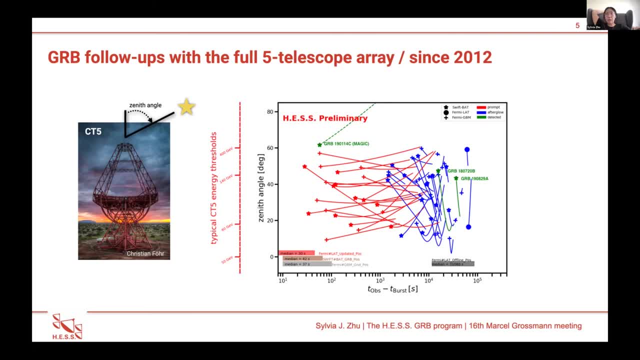 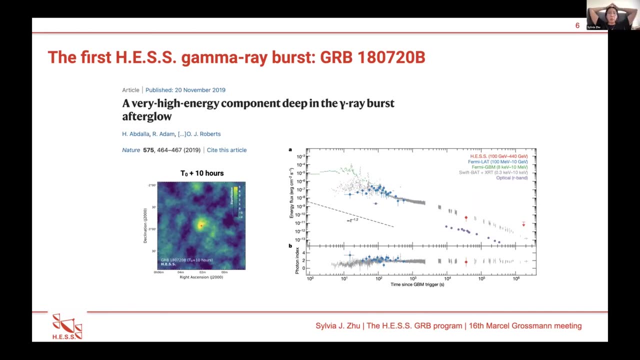 moonlight conditions that were too bright for us. Um, and then we have the marvelous 1908-29A, which, uh, Edna is going to talk about next. So just briefly summarizing, or just reminding everyone about 1807-20B: um, this is a GRB. 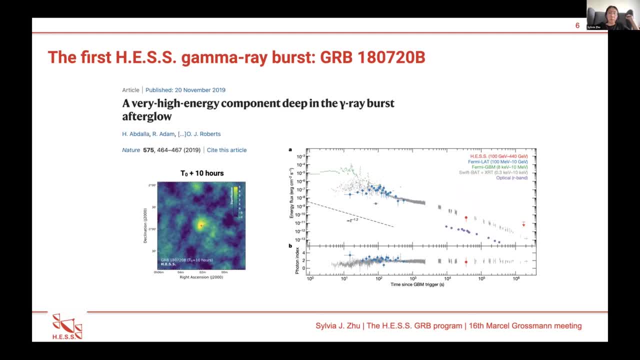 for which we had observations starting at around 10 hours after the GRB occurred. And with these Uh, with these observations of I think it was a few hours long, we were able to get a five Sigma results. And this was extraordinary because you don't necessarily expect a uh VHE detection at 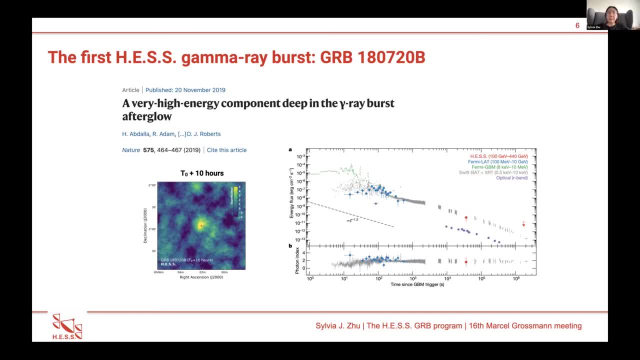 10 hours after the GRB first began, after things have really slowed down On the right, here you see a multi-wavelength light curve. Uh, this is the energy flux light curve, uh, for different instruments. And in the blue you have Fermilat, in the gray you have a swift bat, and then later, 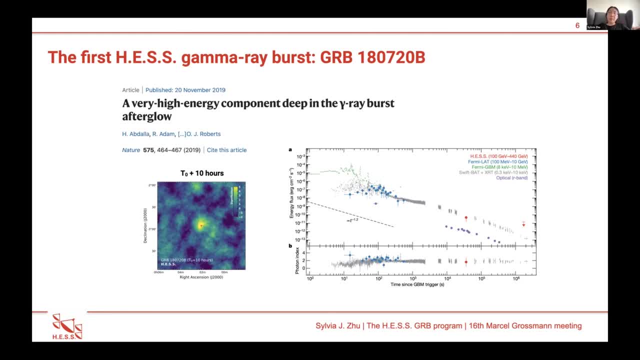 Swift XRT and in the red you have Hess And it was already interesting to notice that even with this uh sort of uh five Sigma results. that's the uh at the time of the Hess observations, the energy flux in the 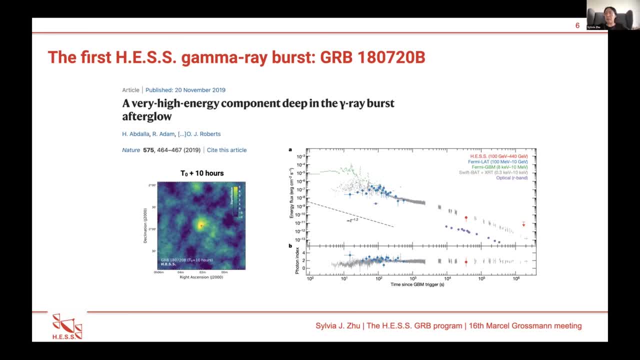 Hess energy band seemed to be similar to the energy flux in the Swift energy band. And then, if you look at the photon index, which is the lower panel, um, again comparing Latin blue, Swift in gray and Hess in red, the photon indices were all hovering around. 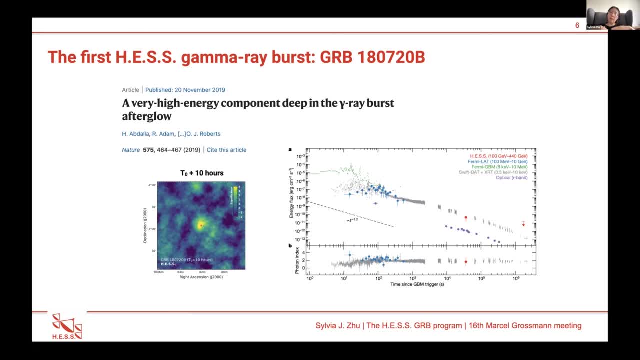 two again being cut: um, which is not necessarily expensive. Now this is another thing that can be Expensive For GRBs. If you have, um- yeah, not necessarily expected for GRBs in general- Um, but of course, then you could immediately say, well, but your Hess error bars are enormous. 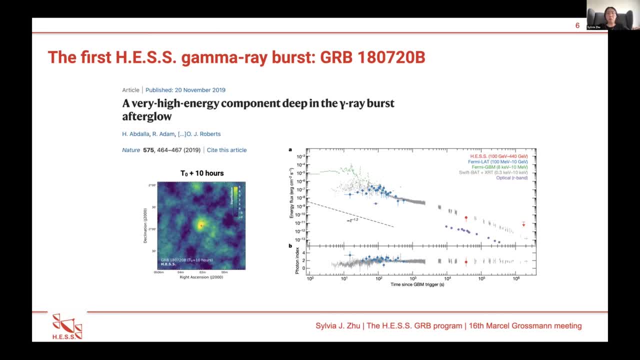 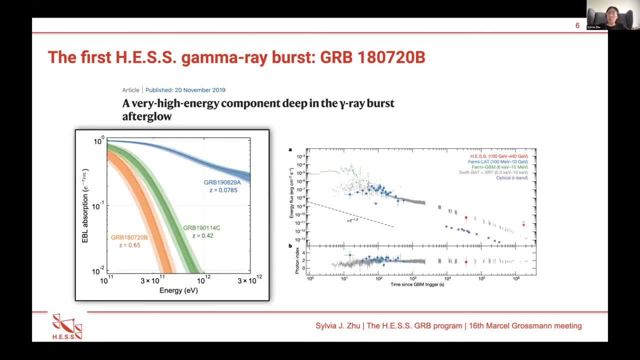 and yes there has error bars, or fairly large, And partly is because this was only a five segment detection, So we're limited by the number of photons we have Um but as well because GRB 18,, oh 7,, 20 B at a redshift of 0.65, um is the far that 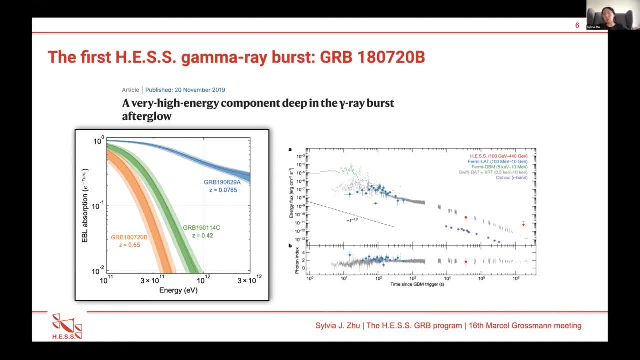 was the farthest one of the public GRB, So, uh, three-point, So, uh, this is the greatest point in the entire thing, but it's not, uh, the most important thing published VHE GRBs so far. And so, because of that, because of its distance, it was more. 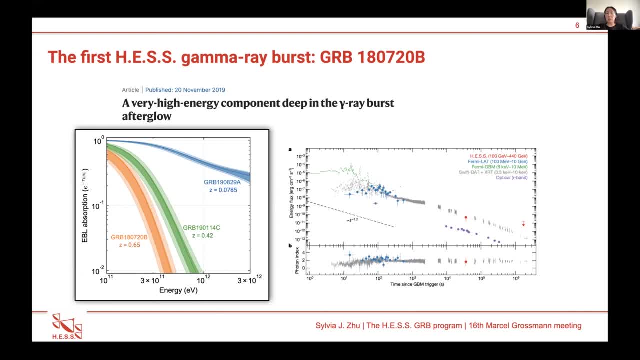 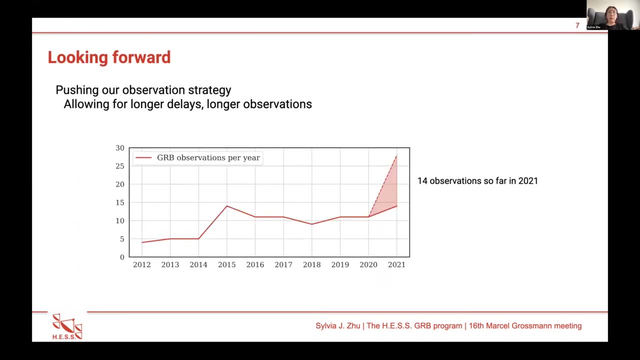 it was more affected by the EBL attenuation than the other GRBs are, And so what we really were looking for was a really close by GRB. We got lucky. 190829A- Again, stay tuned for Edna's talk next. Do not go away. So looking forward, what are we doing to do better in the future? 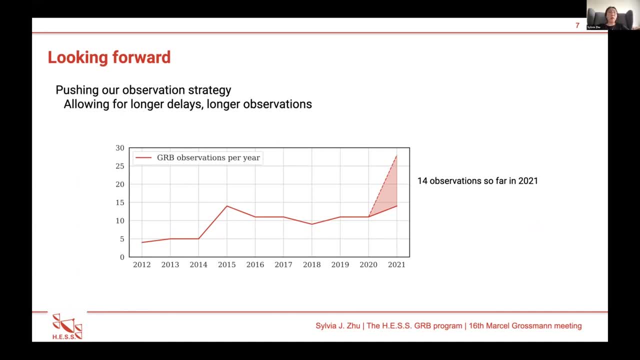 So one thing that I think we're all doing now is to push our observation strategy more, And what does that mean For us? it means we're allowing for much longer delays, as well as taking longer observations of individual GRBs. So what you see here is a plot of the number of 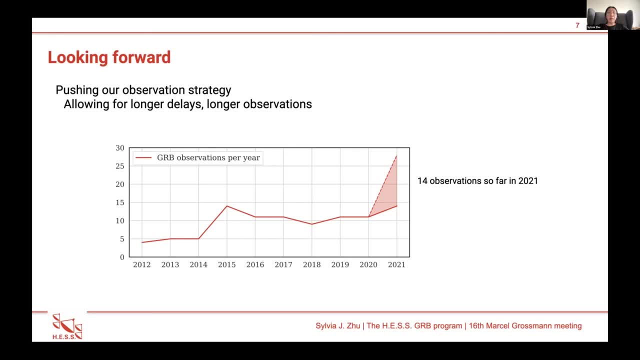 GRB observations we conducted per year And you can see that after things kind of leveled off for a bit, we went after on average 10 GRBs per year until this last year, So in 2021, so far 2021 is. 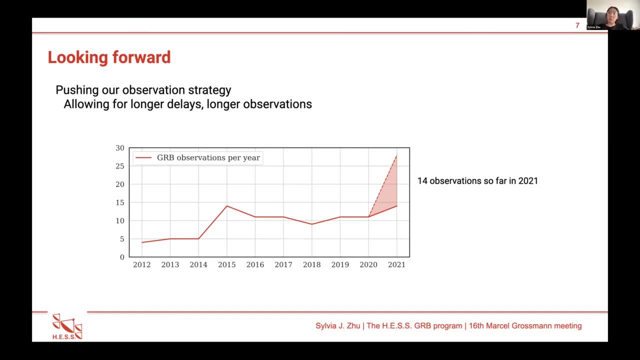 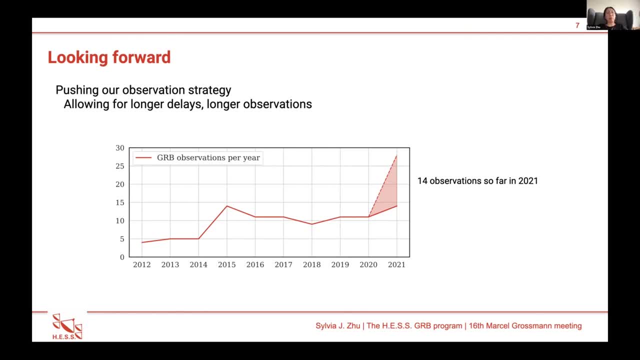 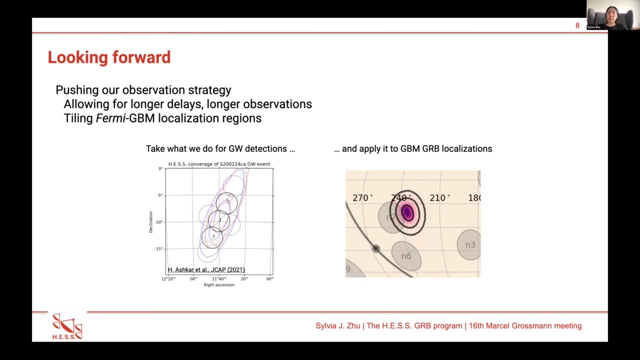 this year And, yeah, and we're still working on analyzing the data for all of these, of course, But hopefully we'll get some interesting results out whenever we can. Another thing is, as I mentioned before, we want to utilize these different telescopes or these different GRB. 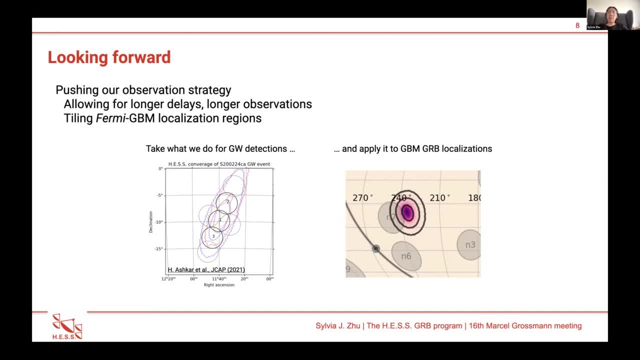 detectors, for instance, And the best way to do that is to use these different telescopes And the best way that we can. So this means taking something like the Fermi-GVM localization regions and tiling them. So currently, what we do for gravitational wave detections is to tile the 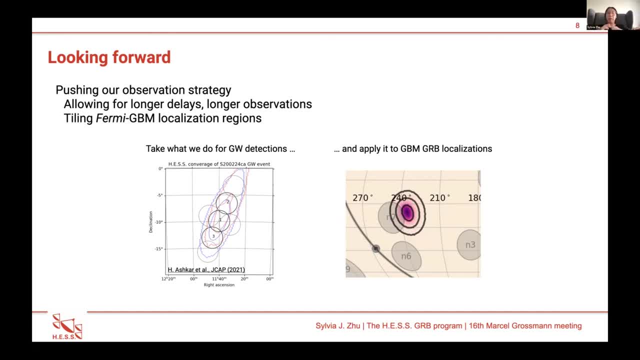 localization region to try to cover as much of the probability as possible, because these are localizations with very large uncertainties. This is also true for GVM-GRB localizations And so, because these are of similar size, a lot of times we have adopted this or are adopting this. 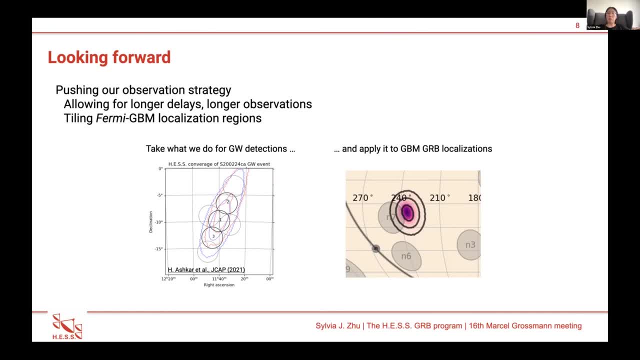 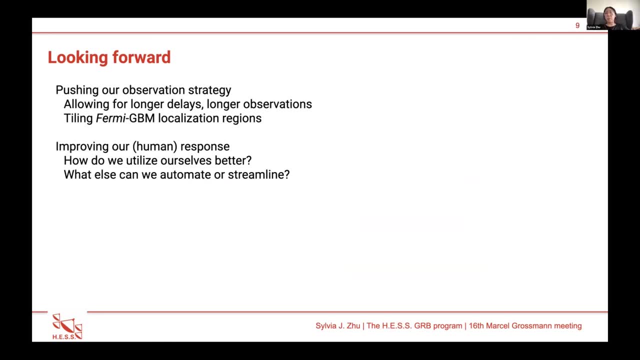 tiling maneuver in order to have a better chance of observing the true position for GVM-GRBs. And, of course, the questions we're all asking ourselves is: how can we improve our own human response, How do we utilize ourselves better And what else can we do to automate or streamline? 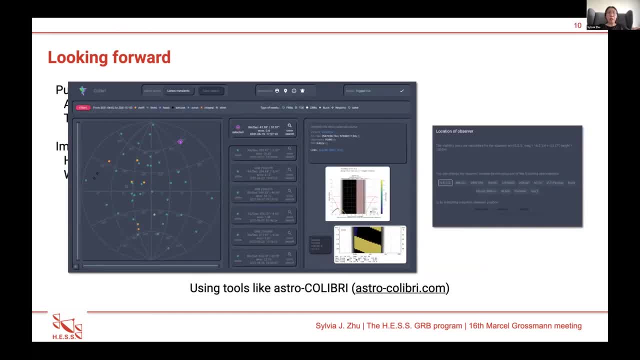 other things. And as an example, here we are using tools like Astro Colibri, which is not a part of the HESS collaboration but has overlapping interests. So if you want to check out this tool, you can see that it has a record of recent transients, not just. 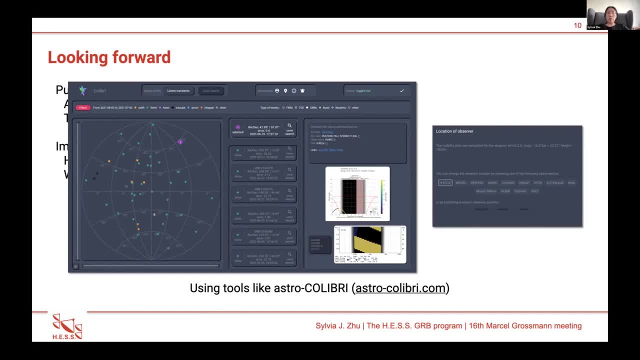 GRBs, And when you click on a transient, you can see, for instance, the visibility at the site that you're interested in, And you can specify what site you're at, either one of these preset telescope facilities or with your own custom observer position. 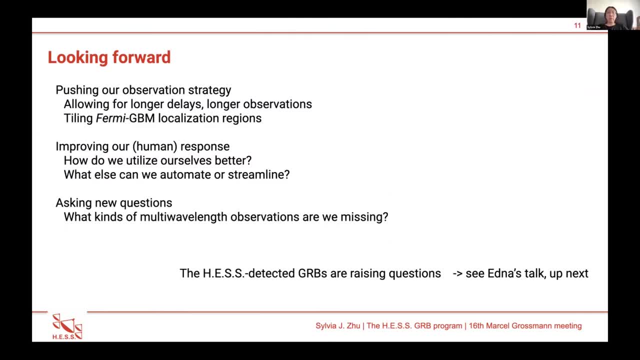 And, of course, now we're asking new questions. So, from an observational point of view, what kinds of multi-wavelength observations are we missing? Is there an energy range where we need more observations? How do we go about getting it And how do we use it as best as we can, Because currently the HESS-detected GRBs are raising? 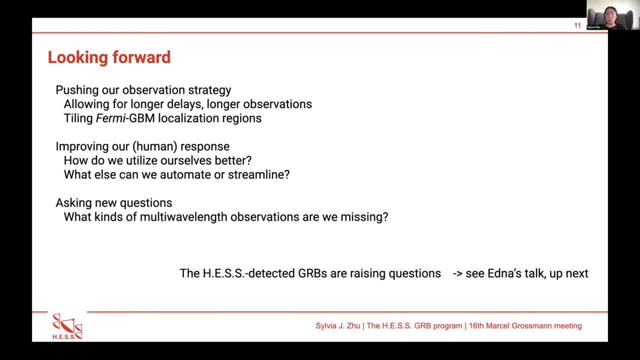 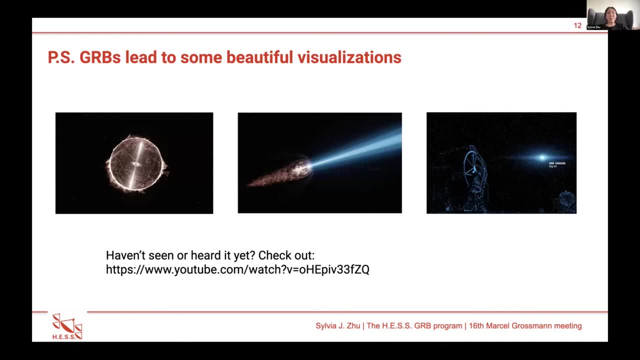 big questions, And this is again seeing Edna's talk up next where she will talk more about it, And I'm almost done. Just a little side note: GRBs can also lead to some beautiful visualizations, So what you see here are screenshots from a recent outreach project. that sort of was at the interface. 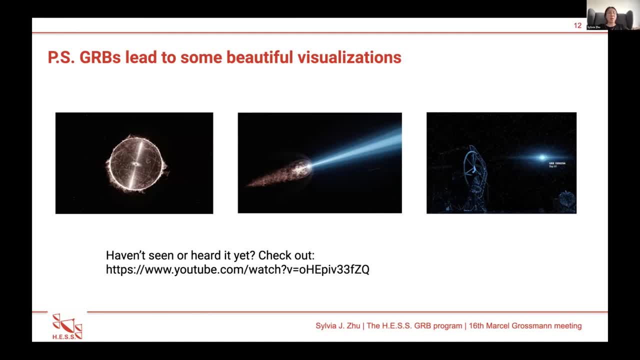 between art and science. So these are not just artists' impressions, but these are actually simulations, particle simulations of what GRB jets collapse, stars, what the jetted emission, what all these things look like And, as well, we have a really nice soundtrack composed by an electronic artist to go with it. 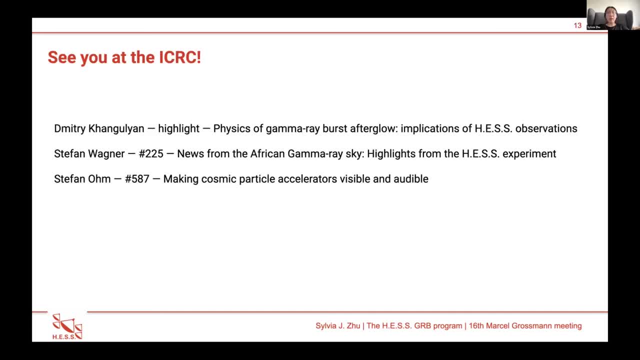 So if you're interested, please check out this YouTube link. And, as a last advertisement, we are going to be discussing a few of these things at the ICRC, So Mitya Kangoulian has a project that's going to be a real challenge for us. And it's going to be the first ever virtual-based installation of a satellite. So this is the IGRC. So Mitya Kangoulian has a project that's going to be a real challenge for us And it's going to be the first ever virtual-based installation of a satellite. 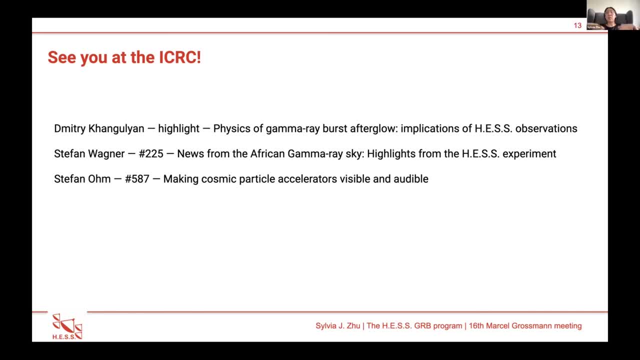 And it's going to be the first ever virtual-based installation of a satellite. In a highlight talk we'll be discussing sort of overall physics of gamma-ray burst afterglows and implications of the Hess observations. in particular, Stefan Wagner, our spokesperson, will be giving an overview and summary from the recent highlights from the Hess experiments. 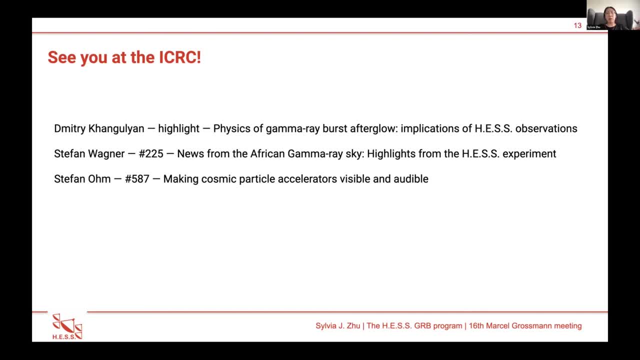 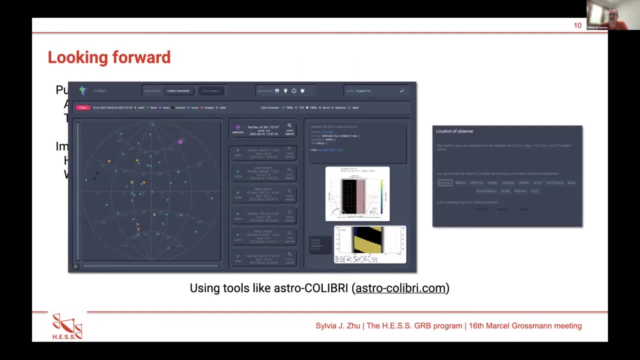 And if you're interested in the pretty pictures, Stefan Ohm has a contribution on how these artistic videos are created, And that's it. I have no summary slide. This is it. Thanks a lot, Silvia. Thanks a lot for the advertisement of Astro Colibri. 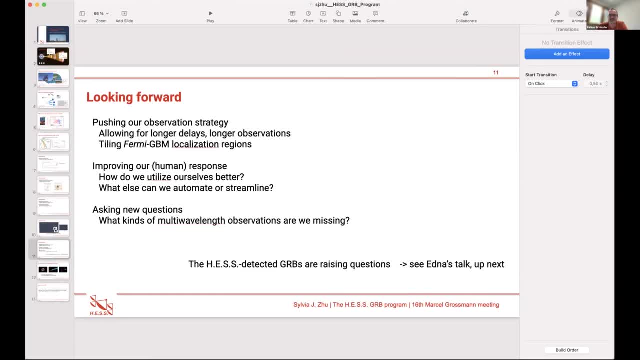 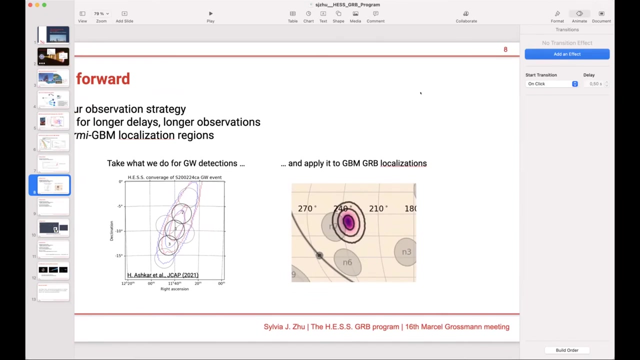 Other questions. I have one, if I can, Fabian Sure go ahead. Silvia, can you show again the slides about the tiling Yep? Okay, So let's say the LIGO-Virgo had the probability map included. 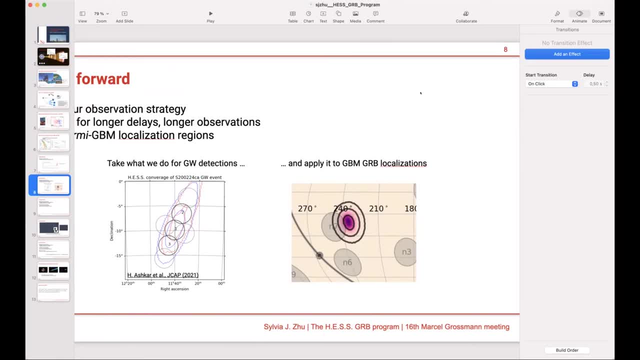 For the GBM-GRB localization. do you know whether they are releasing the same information? So, where you are starting to tile from their center And then you go, what is the strategy that you adopt to tile the GBM locations? Right? So actually, I saw Eric Burns showed up so he can probably give you more details. 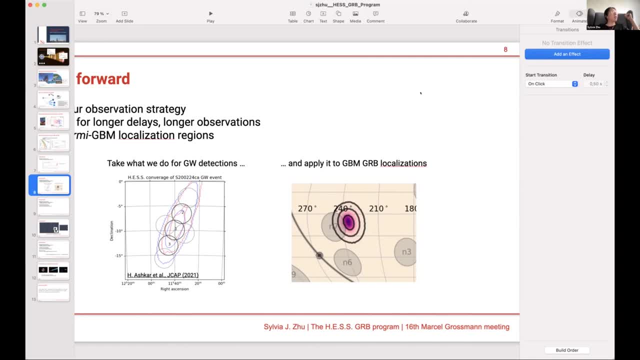 But as far as I know, I believe there's. So there's the automated, the RoboBA now, I think, which does essentially what the human births advocate used to do: to get the on-the-ground, human-in-the-loop GBM localization positions. 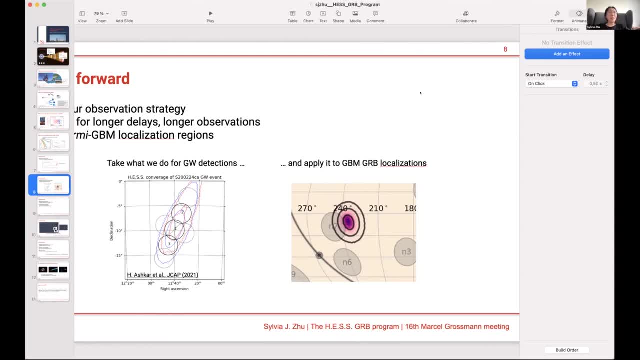 And so that happens on a latency of, I think, 10 to 30 minutes, or something like that, after the births began or after the births occurred, just to wait for the full data to downlink. And then they do provide this healpix map linked from GCN notice, I think. 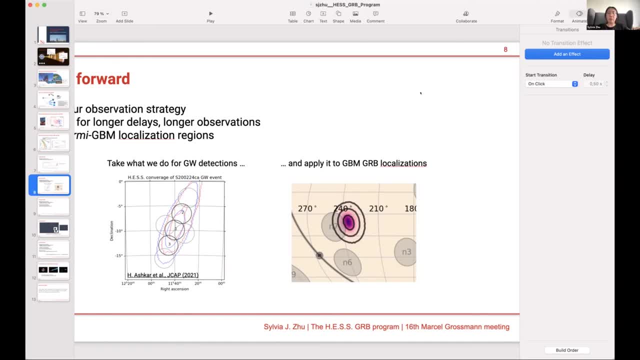 From the last GCN notice that is sent out if it's available, And then we just use. we just download this healpix map and then apply the same kind of strategy. And there are different strategies where we apply. but we basically say, considering where this is, what the zenith angle is and how it's moving across our field of view, how do we maximize the probability we cover? 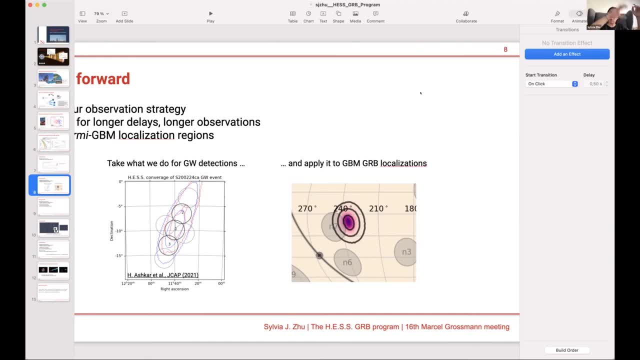 And yeah, usually basically that's it Okay. So basically this starts at the center and then it kind of goes around. The question was really, let's say, simple in this way. So thanks that you answered it properly and correctly and what I wanted to hear. 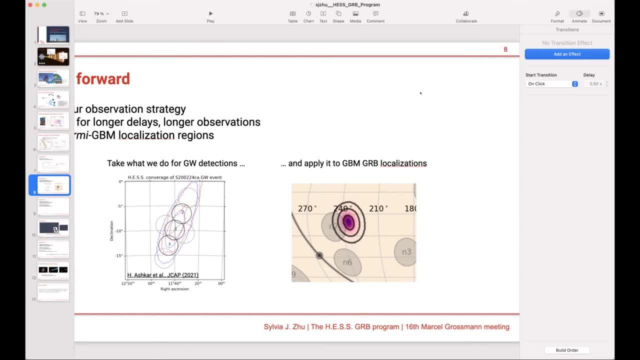 But then the GBM has not just the location error, the statistical one, as you know very well. there is some systematic error. So you are searching for the larger error box. Yes, So the and again, Eric should correct me if I'm wrong. 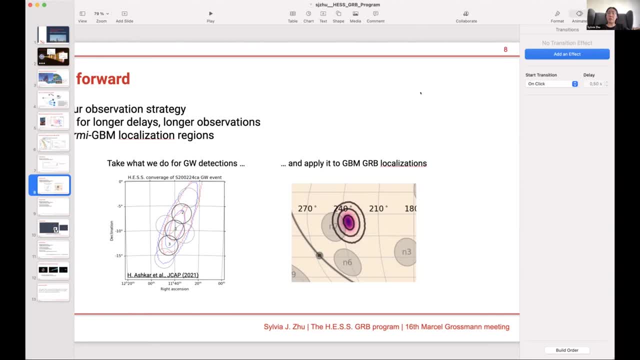 But the final, the full healpix maps, also include the systematic uncertainties folded in. So when you're looking at the healpix maps, you're getting statistical and systematic combined, And so this is why we are focusing on these maps rather than just the single points. you know, the localization center which, and then looking at just which, only gives you sort of information about statistical uncertainties. 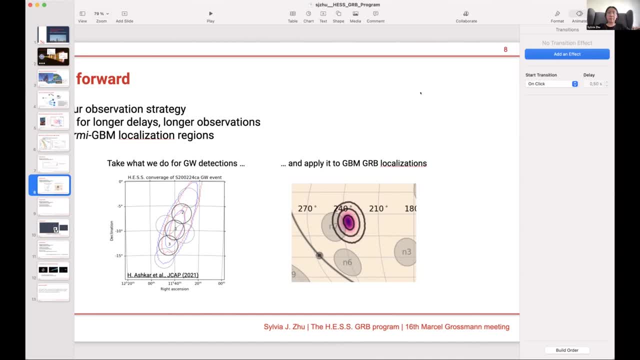 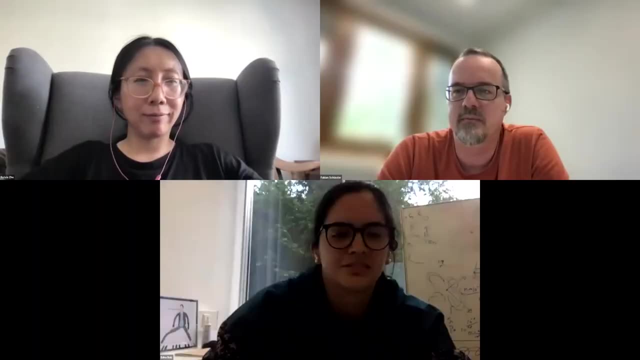 Thanks. Did I answer your question or did I talk about something else again? Okay, I guess that answered the question. Thanks a lot, Silvia. Let's move on. Thanks a lot, Edna. going to report on 1908, 29A. 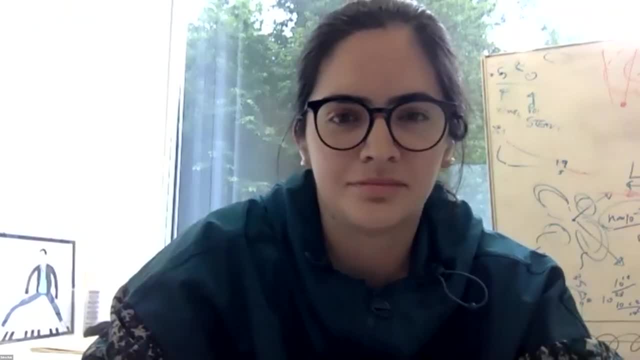 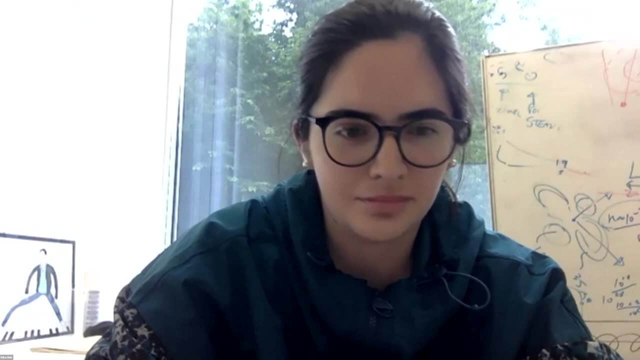 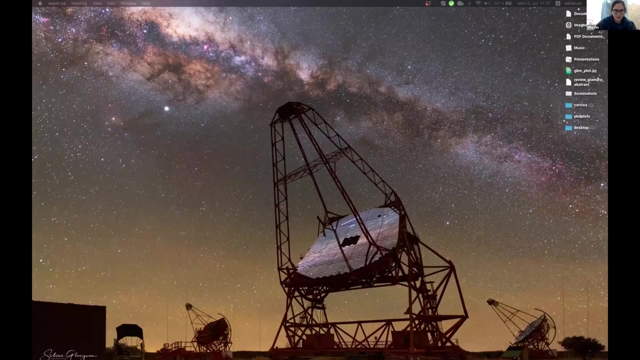 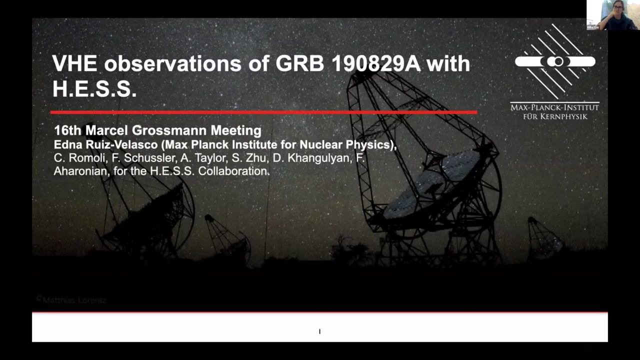 Go ahead. Sure, So share the screen And then play. Yeah, All right. So first I wanted to give a big thank you to Fabian and Franz for organizing these two sessions from today and Wednesday And also for inviting me to give this talk. 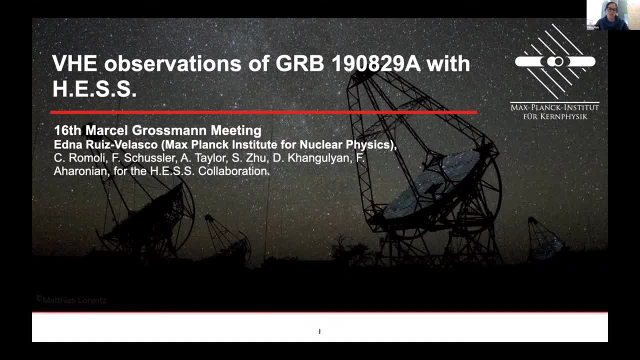 So I will talk about the observations of 1908, 29A that was detected with HESS, And while I'm giving this talk on behalf of the whole team that work on this publication, but also on behalf of the HESS collaboration, 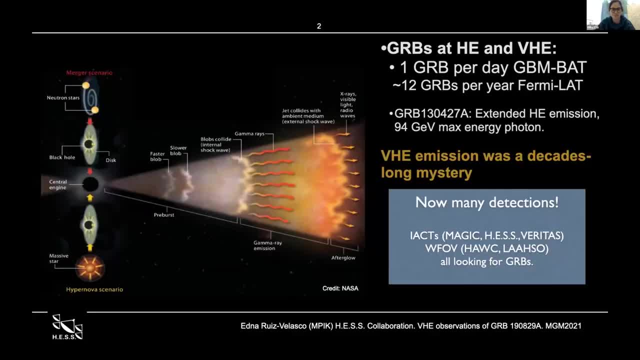 And also, well, many thanks to Alessio, Davide and Silvia for giving very nice introductions on what the rivers are. So I saved a lot of time, But I nonetheless I wanted to give a bit of an overview of where are we standing, so that we are coming to the same ground. 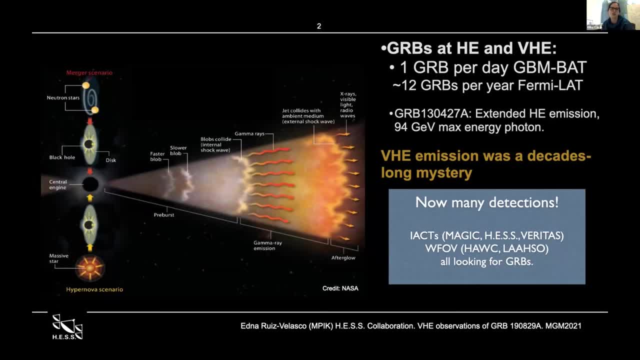 So what we basically have is we detect roughly one gamma river per day with SWIFT, BAT or Fermi GBM, And out of this amount of gamma rivers we get roughly 12 gamma rivers per year with Fermilab. So we're talking about the high energy emission in GRBs. 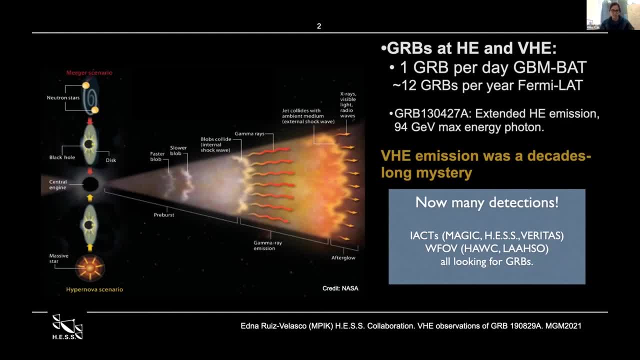 In this context, Fermilab had detected the highest maximum energy photon of 94 giga electron volts in 2015 from a gamma river, And that was roughly the end of the story. The very high energy emission of gamma rivers, given that they are very energetic, was a decade-long mystery that started- I mean, the search started since the 60s, with the very first detection of gamma rivers. 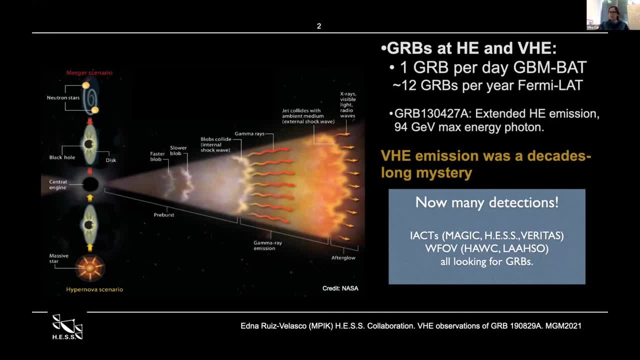 And currently 2021, we have a very high energy emission of gamma rivers And in 2021, we have many detections And these are thanks to very ambitious program of gamma rivers observation by the current instruments. So in ICTs we have MAGIC, HESS and VERITAS. 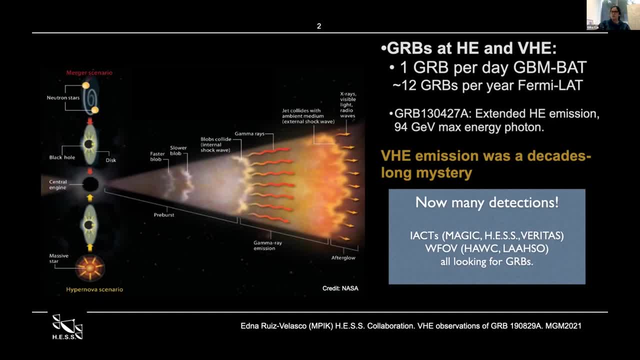 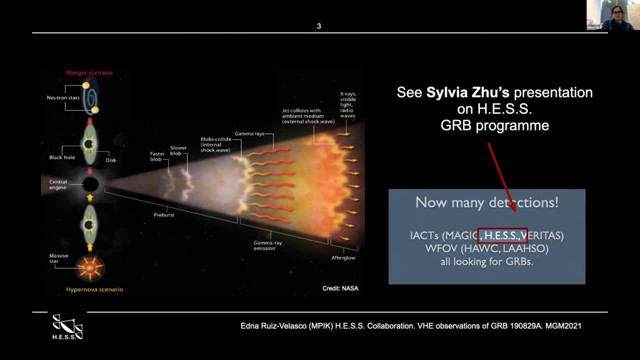 And also the wide field instruments like HOC and LASSO. we are all looking for gamma rivers and improving our GRB programs, So I'm not going to go to the details on how we observe gamma rivers with HESS, Because Silvia already summarized it. 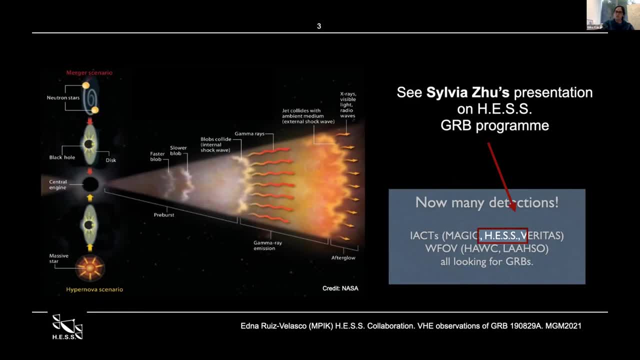 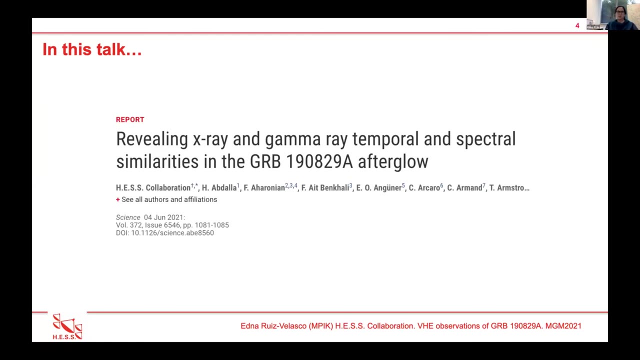 Thank you Very nicely. So I refer to the slides of Silvia if you want to know a bit more on how we do these observations, But instead I'm going to talk about the publication that we did roughly one month ago in Science. 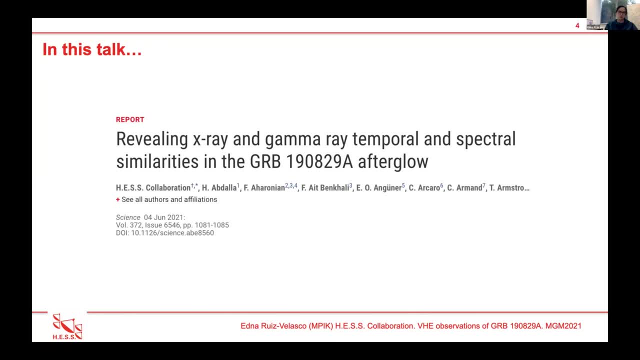 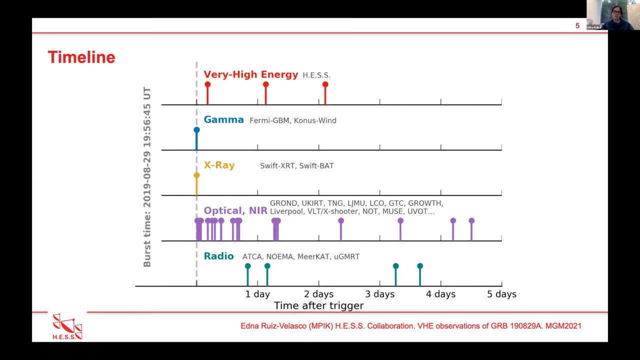 And this is about. well, the title of the paper is Revealing the X-ray and gamma-ray temporal and spectral similarities in the afterglow of TCRB, And so with this I'm going to go through how this observation happened. 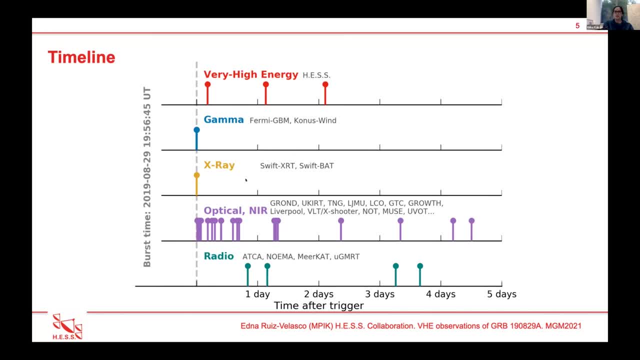 So I'm going to use a timeline. So what you're seeing here is the many instruments that detected this gamma river as a function of time, throughout the multi-wavelength range, And first we have the Fermi-GBM detection. So Fermi actually saw two peaks in the prompt emission phase of this gamma river. 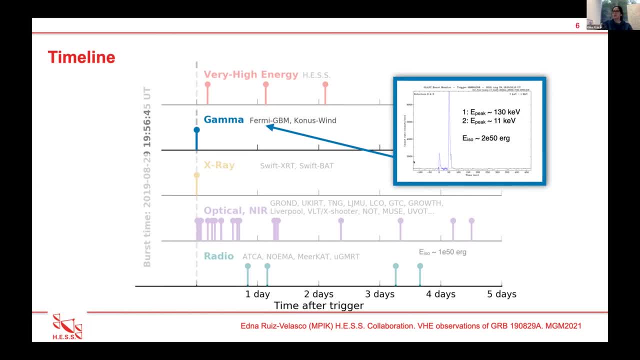 The first is very dim but has an energy peak of roughly 130 kiloelectronvolts, And it's followed by a second peak at roughly 50 seconds later that has an energy peak of 11 kiloelectronvolts And all in all, this prompt emission has an isotropic energy of roughly 2 times 10 to the 50th. 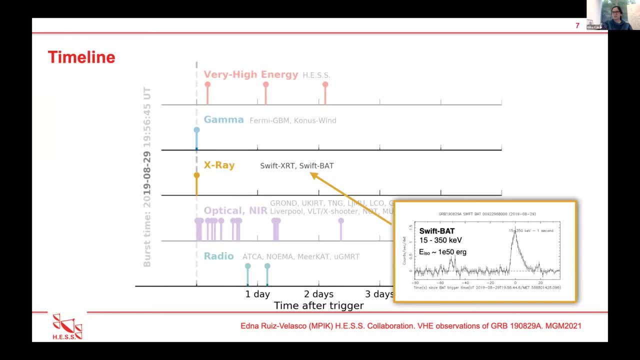 Then we have of course, Swift-BAT And Swift-BAT actually, so mostly the second peak, And this accounts for a total isotropic emission, So a total isotropic energy of roughly half of what Fermi-GBM saw. 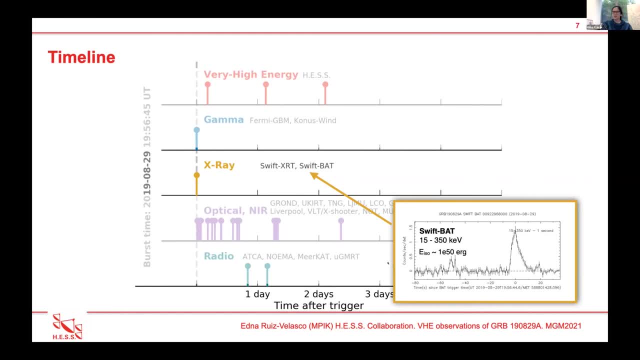 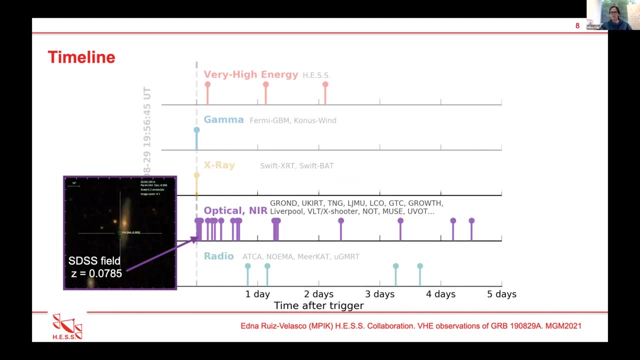 So a value of 1 times 10 to the 50th. This already having a Fermi-GBM detection, Swift-BAT detection, was a good indication of an interesting gamma river And also this was even stronger because Swift-BAT actually well, given the good localization. 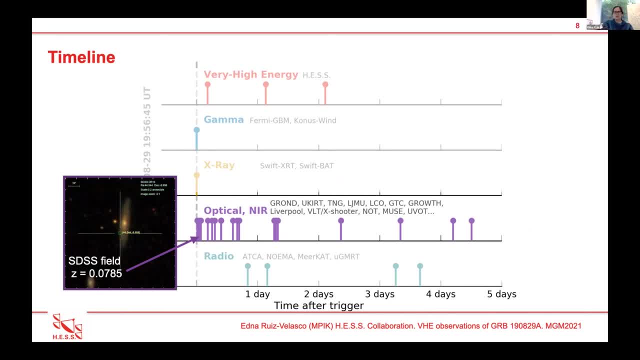 that Swift-BAT provides. we were able to link this gamma river with the host galaxy that was previously identified by the Blondie Higgs Sky Survey, And this galaxy, the host of the gamma river, is at a ratio of 0.08.. 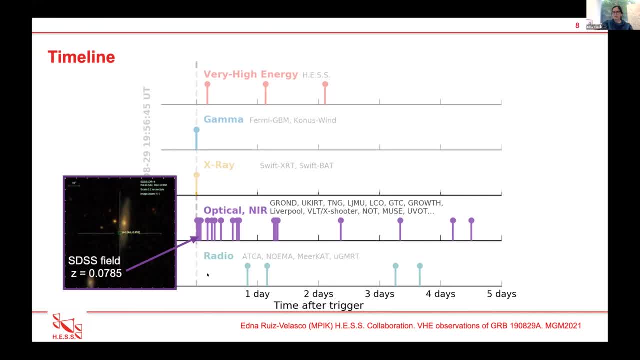 And then the ratio was then confirmed by the Grand Telescope of the Canary Islands measurements and provided this ratio of 0.078 for this gamma river. Then, all in all, given the fact that we detected this gamma river with HEF and we announced it promptly with the GCN circular and Anatel, 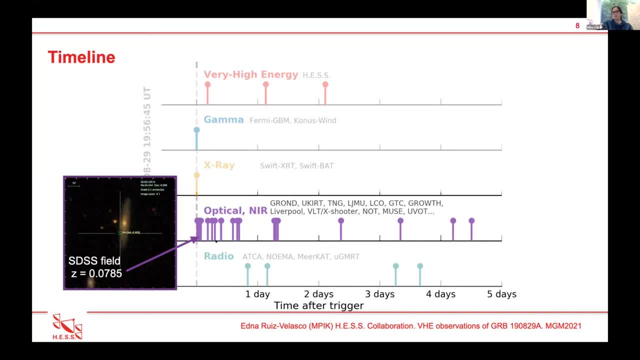 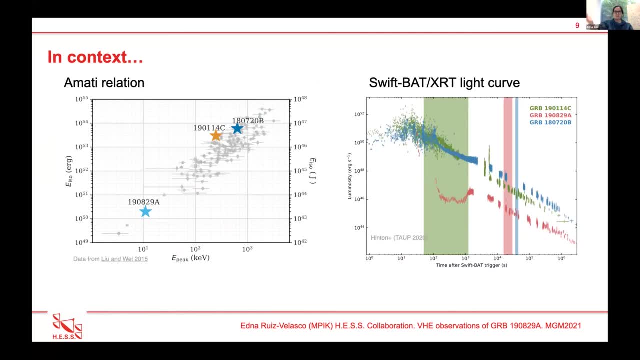 we obtained a lot of follow-up, from radio up to, well, the HEF observations in the Deep Afterglow, And I wanted to show a bit of what is the context of this gamma river. what is it standing, if it's special or not. 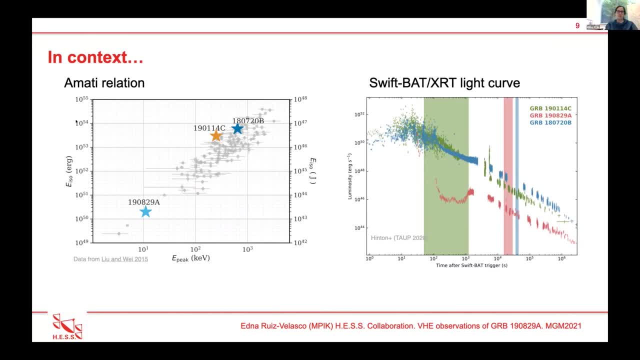 And this is well basically a dramatic relation. So we are showing the AISO value versus the energy peak for this full population of gamma rivers, of long gamma rivers, And we can see that well. GRB 190829A has a very low isotropic energy. 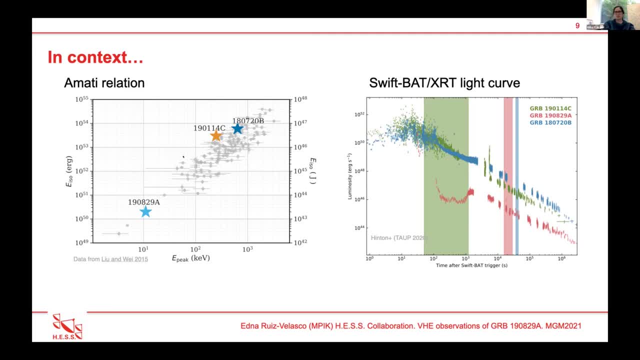 It's falling at the low end of the Amati relation And we also show here the values for 190114C, detected by MAGIC, and 180720B, detected by HEF, which are at the other end, And I like a lot this plot because it actually shows that maybe very high energy emission is nothing special in gamma rivers. 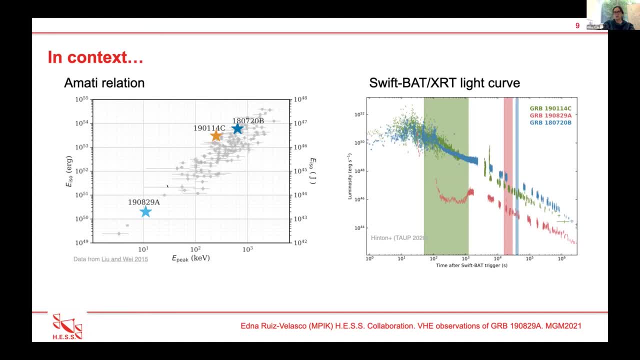 So it might be that we can also detect ones that are in the middle region of the Amati relation in the future. And then if we call the Swift light curve in the X-ray band and we show the luminosity evolution for this 3 gamma rivers, 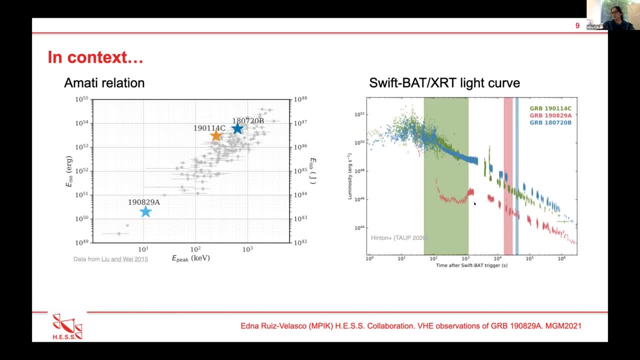 we actually see that. indeed, GRB 190829A is very low luminosity GRB, but it has a very similar behavior in the afterglow as compared to the other gamma rivers that are at very high energies. And well, just the shaded regions are indicating only the range or the interval of time that these gamma rivers are followed by the IECTs with the respective color coding. 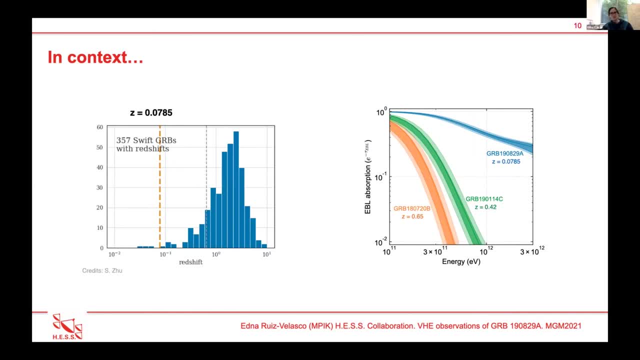 More in context On how this GRB is so nearby. this GRB is one of the nearest gamma rivers detected in X-rays And this is the distribution of the redshift of gamma rivers detected by Swift. So this totals of 357 gamma rivers. 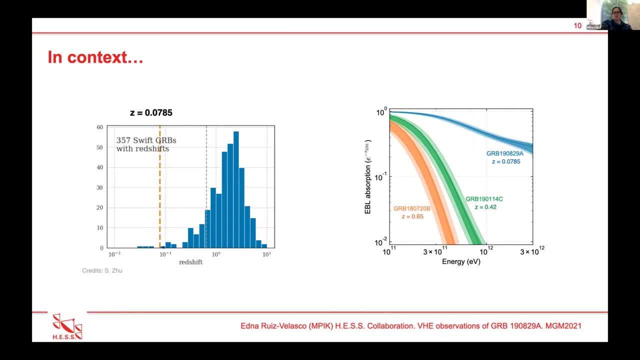 And we see that this GRB is at the very beginning of the tail of the lower values of redshift. And well, this is very important for the case of very high energy observations because of the EBL absorption. So, if we compare the 3 gamma rivers detected at very high energies that are currently published, 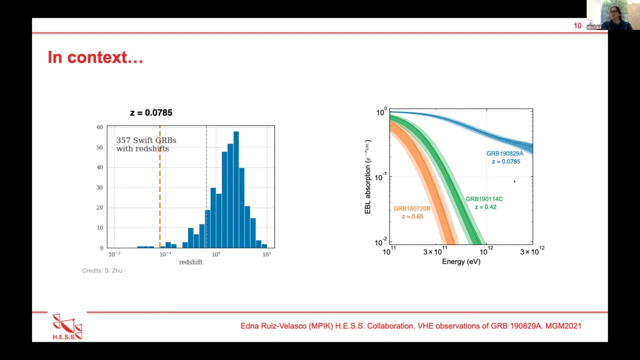 we see how GRB 190829A is providing a very, very, very small EBL absorption, And this also allowed, of course, to obtain very precise measurements on the spectrum and also the fact that we observed these gamma rivers for several nights. 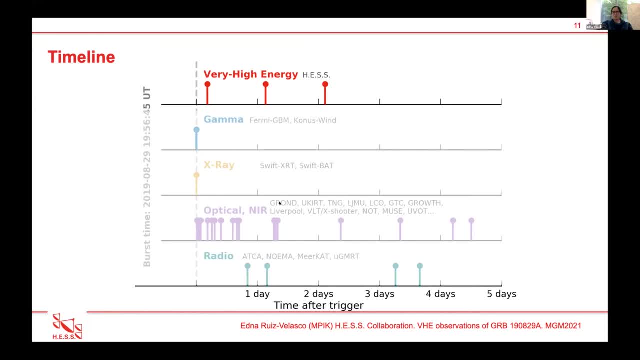 So, regarding the health observations, so we started observations at roughly 4 hours after the beginning of the prompt emission of these gamma rivers, And it is when we immediately knew, with the preliminary online analysis, that the GRB had a significant emission of very high energies. 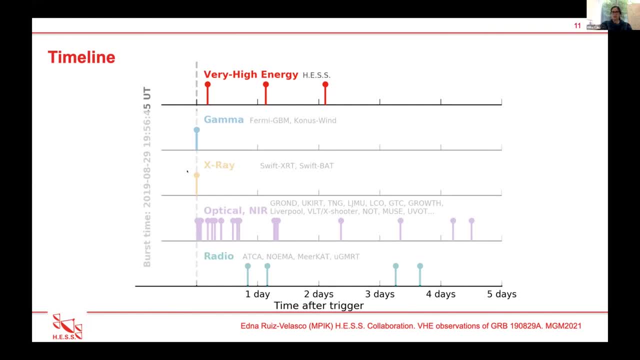 So it is when we announced the detection by the GCN and ATEL. We observed it during a second night again, when the GRB was visible, And during a third night, And this is when we actually found in the offline analysis for the first night. 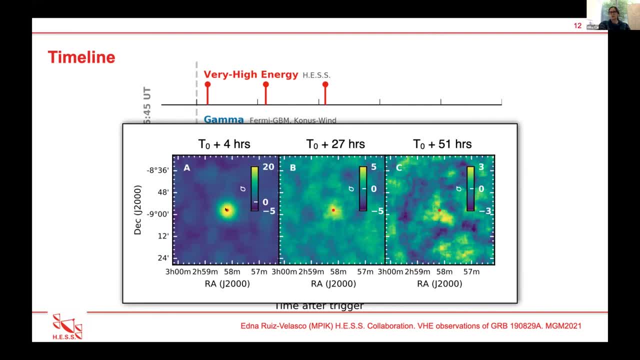 a 20-sigma detection, which is consistent with the optical position. This red dot is the optical position of the gamma rivers. During the second night we have a 5-sigma detection And this is at 27 hours after the beginning of the prompt emission. 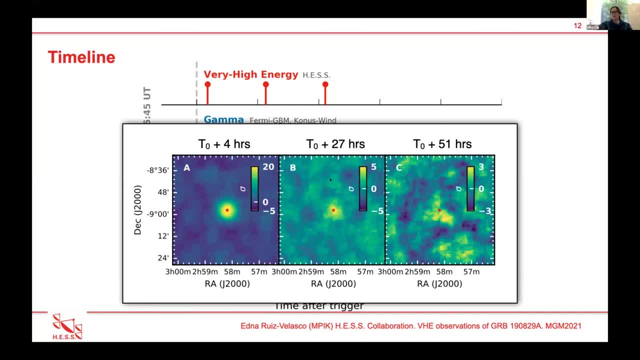 Just to put it in context. I mean GRB 180720B, which was the latest measurement, happened at 10 hours, So we are talking about 17 hours later. And then, during the third night of observation, we see again a hint of. 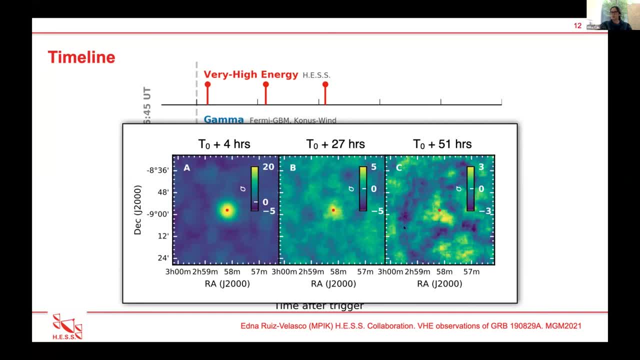 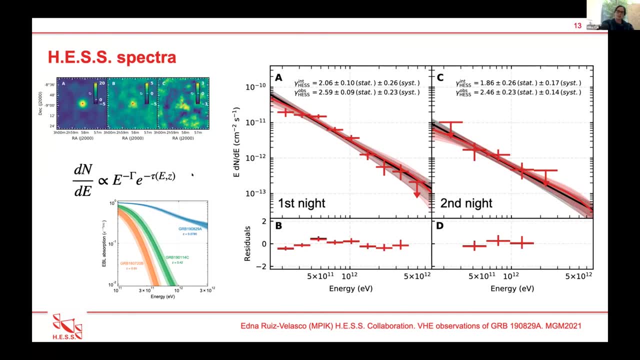 emission of excess of the level of 2.5 sigma. And so, with this data, what we can do is, of course, analyze it to obtain a spectra, And what we do is that we characterize this with a power law, So we can either measure the intrinsic or the detected. 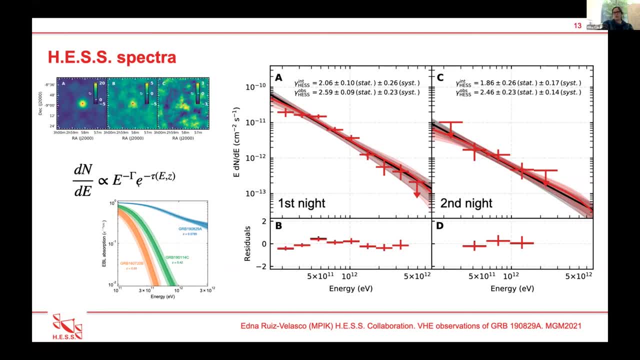 spectrum of these gamma rivers. So for the intrinsic spectrum we include the term for the EBL absorption, that the level is seen here. And for the first night we have an intrinsic photon index of the order of 2 that is going up to 3 terelectron volts. 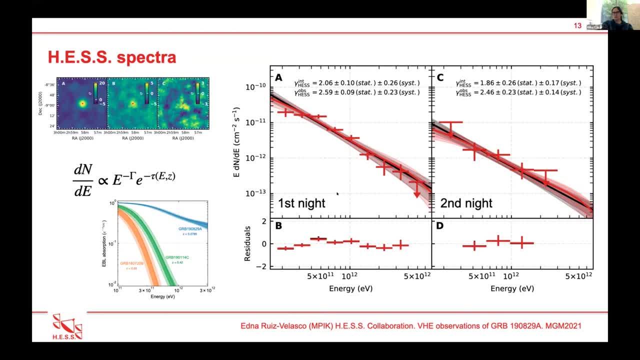 And again, these are very energetic emissions being detected, all thanks to the very high significance of the detection, but also because it's a nearby gamma river And this also allows a very good determination of the intrinsic spectrum, because then the uncertainties on the EBL are minimized. 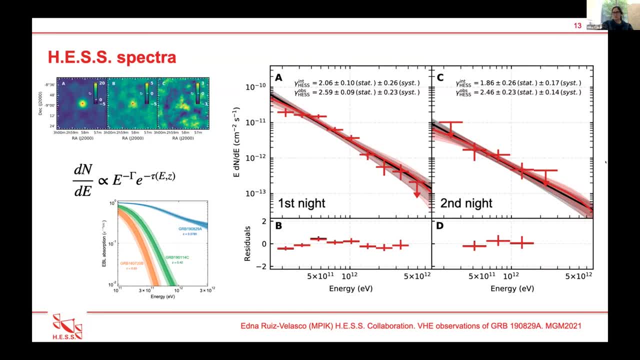 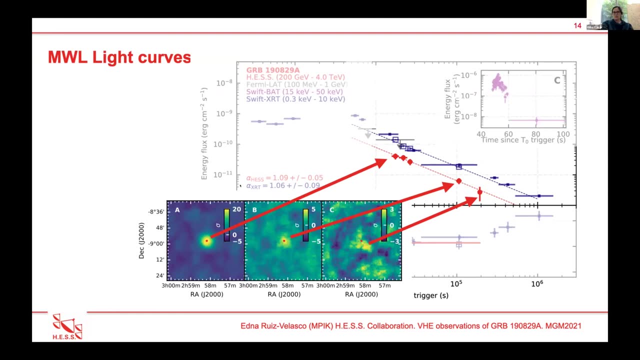 During the second night we also perform a spectral analysis. So this also results in a photon index consistent with a value of 2.0.. Then to put this GRB in context with the multi-wavelength data, so we obtain a light curve for the very high energy detection. 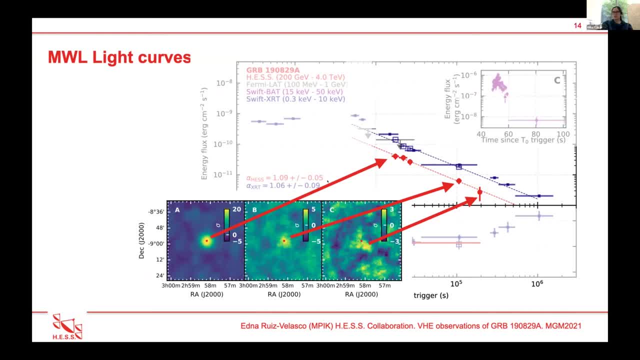 that is going from 200 giga electron volts up to 4 terelectron volts. With the first night of observations we actually split this energy flux detection in three data points because we have a 20-sigma detection. The second night we obtain another data point in the light curve. 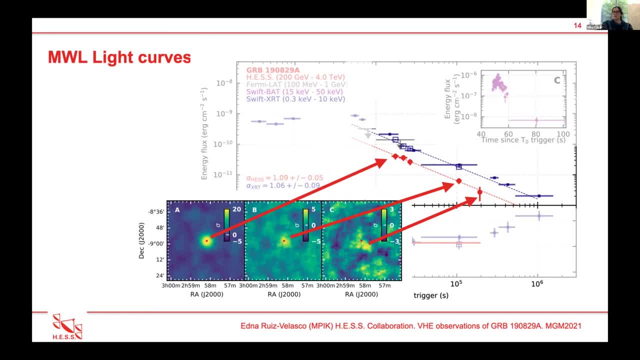 And for the third night again, the last data point. This allowed for the very first time to measure the temporal decay in the deep afterglow at very high energies from a gamma-ray burst. And well, we can of course put it in more context. 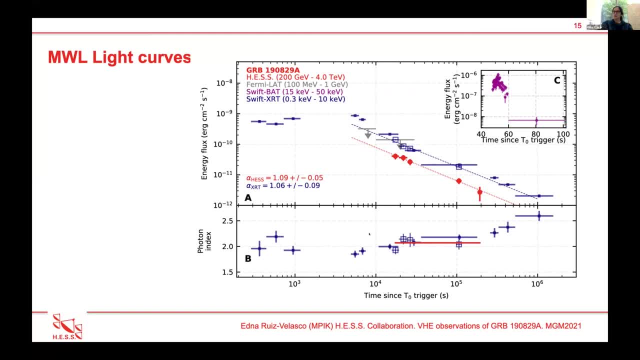 with the rest of the multi-wavelength data. So what I'm showing here is the Fermi-Latoper limits in gray are shown here that are also contemporaneous to the observations by HEF. And then we also have the SWIFT detection. 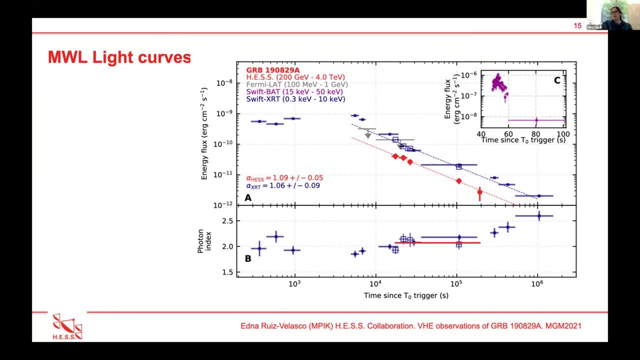 The SWIFT XRT is in blue over here with also contemporaneous observations with HEF, And the temporal decay in XRT is also compatible with a value of F1 as seen by HEF, And the other similarity between this X-ray detection and the very high energy detection is the photon index. 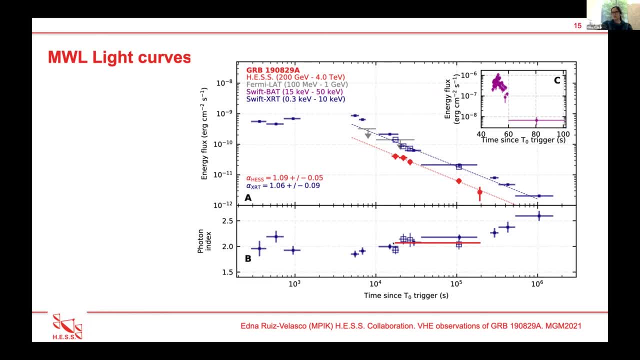 So in the case of the photon index, we see that the HEF detection throughout the whole afterglow is consistent with a value of roughly 2.. That is also consistent with what is being measured with SWIFT XRT. That is also again moving around a value of 2.0. 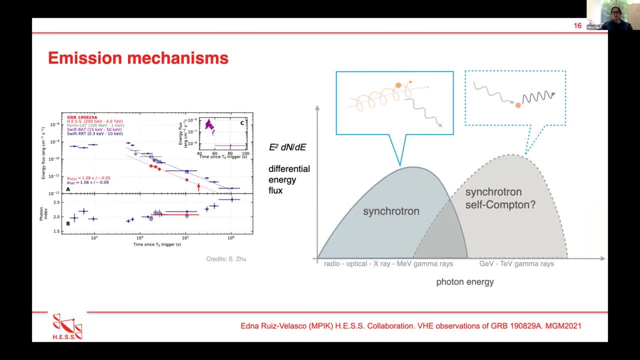 So with this I'm just going to give a bit of a peek on what are the possible emission mechanisms. So one way of interpreting or presenting our data is this light curve, Of course, if we put this data in terms of our spectral energy distribution. 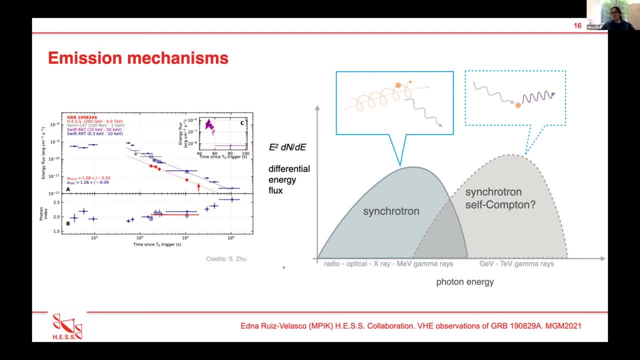 and considering the usual scenario for the emission in gamma reverse, where we have of course the synchrotron that is going from the radio up to low energy gamma rays, so electrons basically accelerated and then emitting synchrotron within the magnetic field of the forward shock in the gamma reverse afterglow. 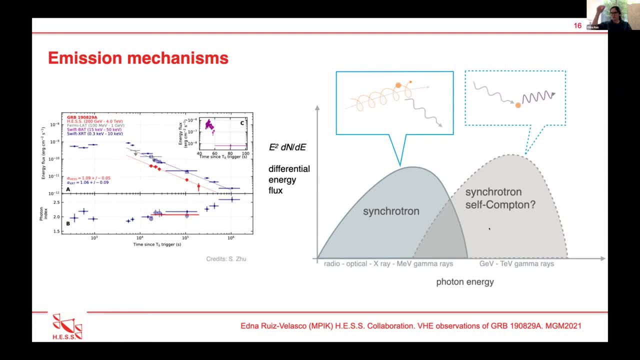 And then we might expect, for example, the very famous synchrotron component that is operating at very high energy. So in this case we have this population of electrons and photons that are being obscured in order to produce even more energetic photons. 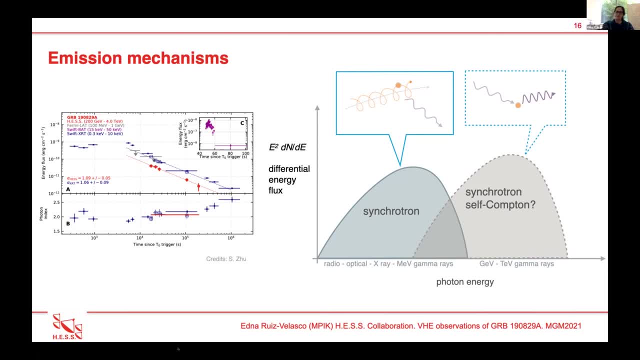 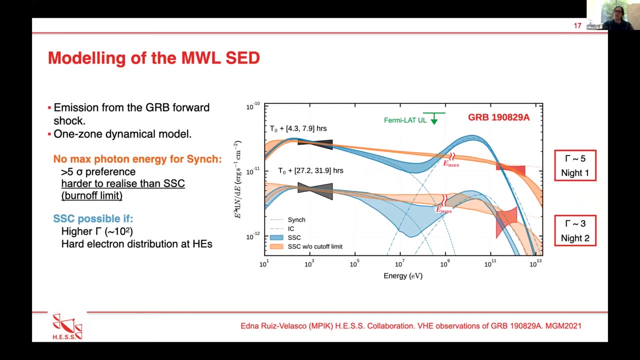 So we will see a second component in our spectral energy distribution. So we took our data from our observations in very high energies and X-rays and performed modeling of the multi-wavelength spectral energy distribution. So we are showing here E-squared DND as a function of energy. 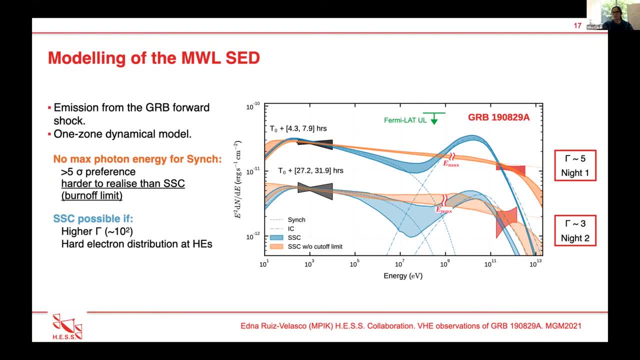 If we have a spectrum that has a value of 2, then our SED will be flat, And this is the case for the X-ray detection. So this butterfly corresponds to the swift detection during the first night of observations of HESS, And then this other one corresponds to: 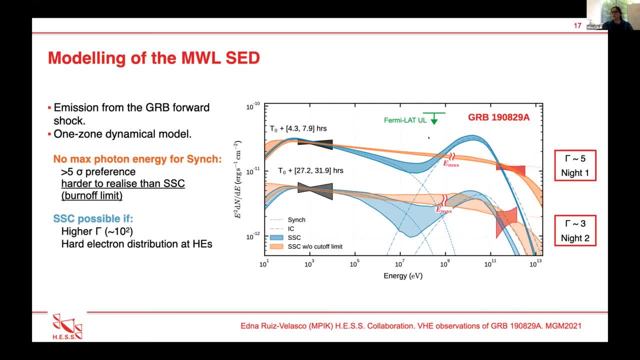 the HESS intrinsic spectrum. We have here the Fermilat upper limits that correspond only for the first night of observations that are very far away from anything closer to those levels seen between X-rays and very high energies. And so for the modeling, what we did is that we consider the GLB forward shock. 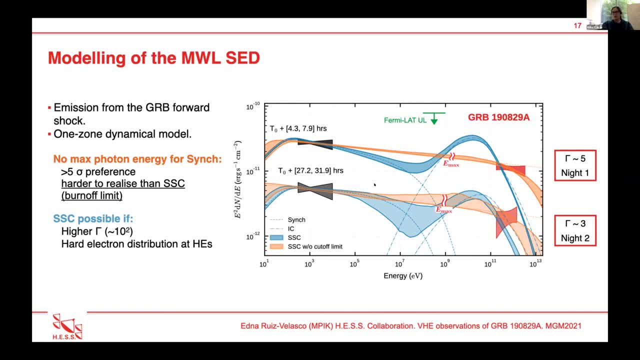 and also a once-on dynamical model. In these cases we play with two cases. So one is the synchrotron test content, the normal scenario, and then one where we remove the got-off limit that is imposed by the burn-off limit to the synchrotron. 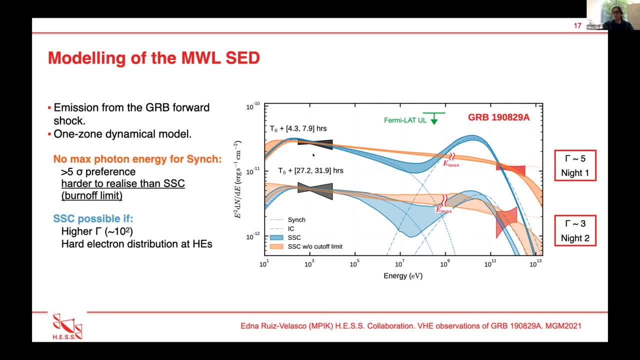 We did this for the two nights of observations. So this corresponds to these two different plots, two different LEDs in the plot, And we can also already kind of estimate what would be the bulk Lorentz factor at this corresponding time. So we're talking about a Lorentz factor. 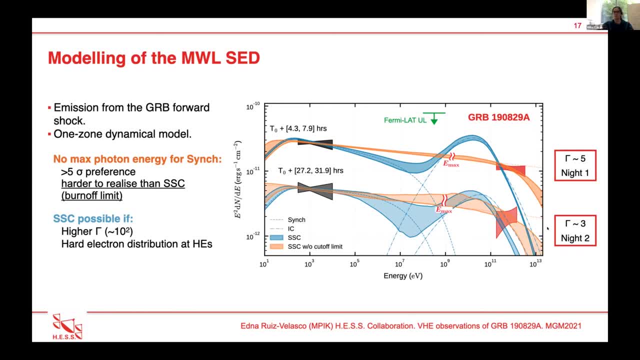 of probably five for the first night and of the order of three for the second night. What we actually found is that there's a five sigma- or more than five sigma- preference for a scenario where we allow for the synchrotron to go beyond the got-off limit. 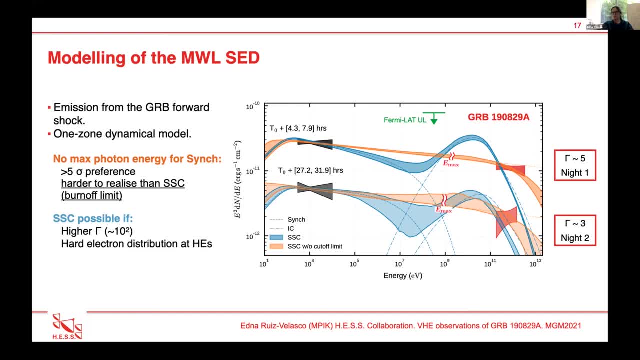 So this is the theoretical maximum energy imposed by the burn-off limit And we see that with this scenario we can nicely connect the X-ray and the very high energy detection, And these are going roughly eight order of magnitude being described by one single scenario. 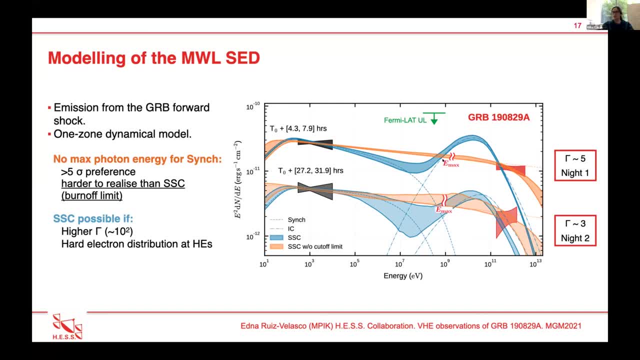 And we are going roughly three order of magnitude beyond the maximum energy imposed by the burn-off limit. Still, we discuss also a bit of how can be the synchrotron test content scenario possible, And this could be realized if we have bulk Lorentz factors of the order of 200. 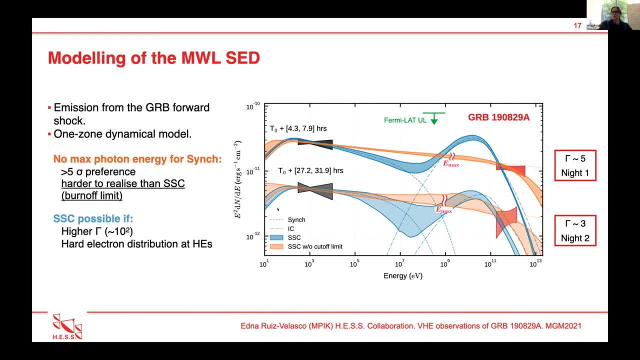 But of course it's very difficult to put this into. I mean to operate at this high bulk Lorentz factor, especially during the second night of observation, that we're talking about, an observation at 30 hours after the beginning of the burst. 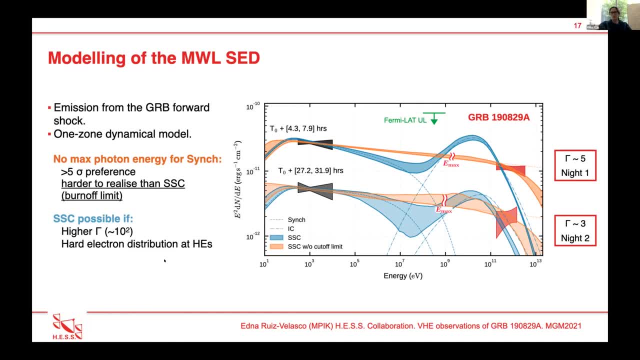 Or also we can talk about SCC if we have a different distribution of electrons that are operating at high energies. But all in all, I mean the thing is that in these simplistic scenarios, one's own scenarios, the synchrotron seems to be favored. 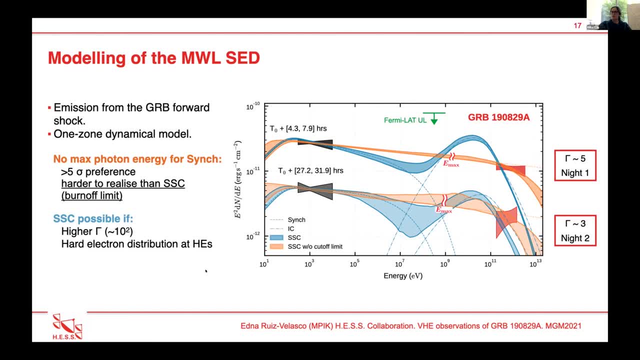 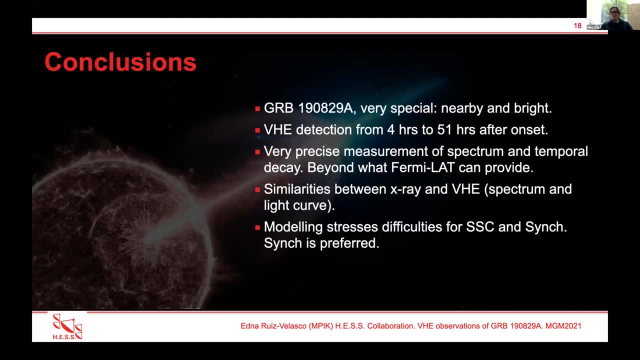 And we might. indeed, these observations are calling for more detailed analysis, for also some other new models in order to describe this data. So with this, if I can move the slide, Okay, Thank you. I come to my conclusions, So I think I hopefully motivate you. 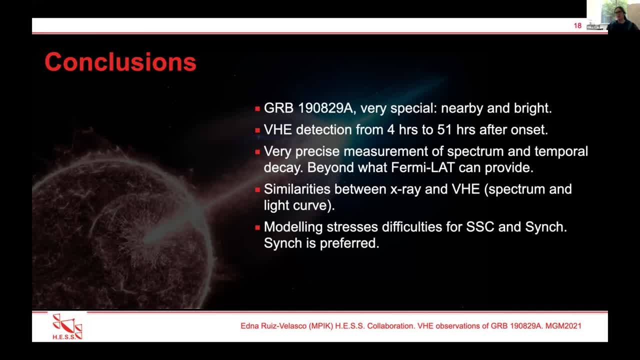 and convince you that this gamma reverse is very special, And this is because it's very nearby and it's also very bright, And also because we have a detection of very high energies that goes up to 51 hours after the onset with a very good 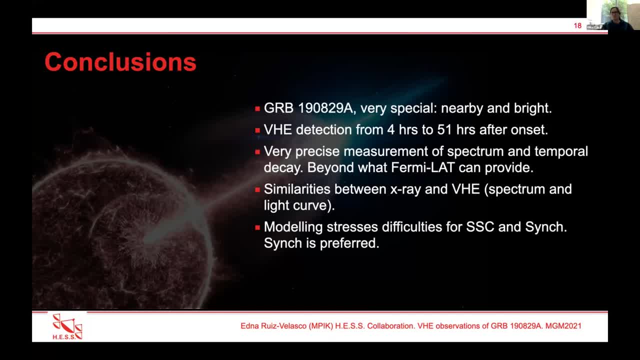 and very clean spectral determination thanks to the fact that this GRB happening in our relatively neighborhood, And so we were able to actually determine with a good precision the spectrum and the temporal decay, And this is also something that happens beyond what Fermilab can provide in terms of sensitivity. 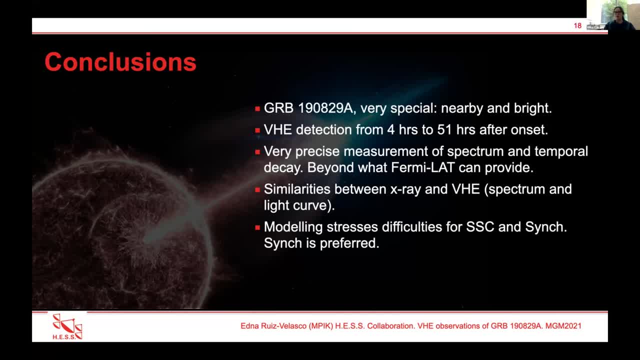 So, as you can see, this gamma reverse was not detected by Fermilab, but with this we were able to measure with good precision the afterglow, And well, I also show a lot of similarities that are arising in this gamma reverse between the X-ray and very high energy. 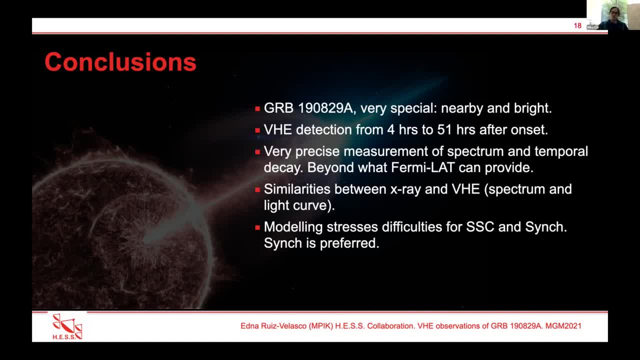 in terms of the spectrum and the light curve. And I try to also stress what are the difficulties between the synchrotrons of Compton and the pure synchrotron scenario, although the synchrotron is preferred. So this is the end. 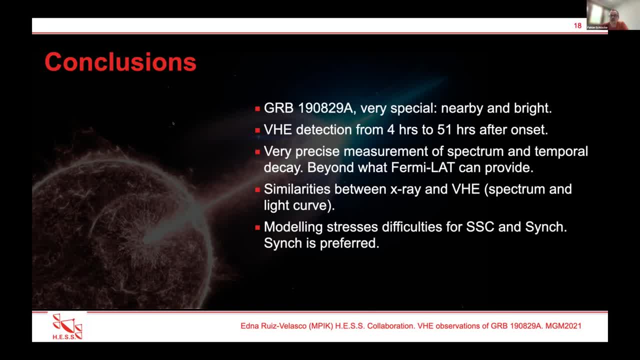 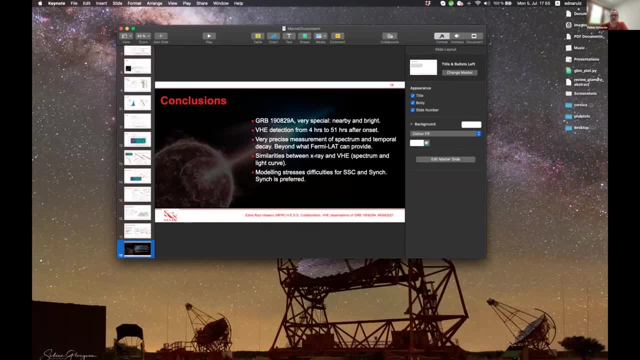 Thanks a lot, Edna. Other questions, Let's see, Edna. maybe I have one, if I can, Let's say, about the progenitor of this GRB. So what can you say? Is that something that it is important to know? 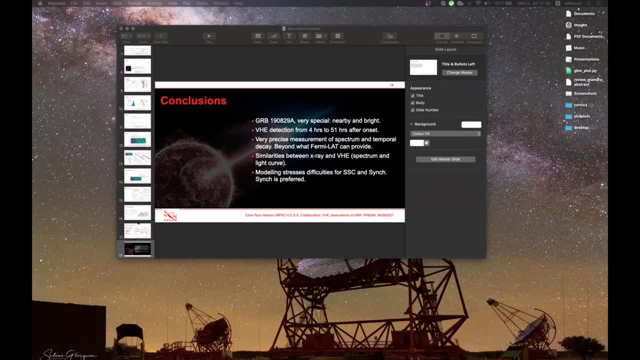 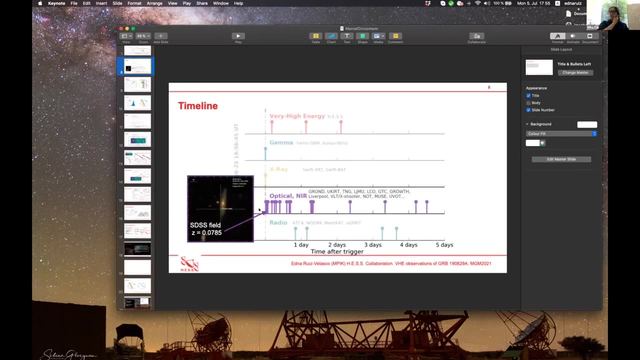 for the very high energy detection. So what could be the environment of that? I mean, I think the fact that this gamma reverse is in the outskirts of the galaxy has a role on the progenitor, And then also the fact that- well, of course, 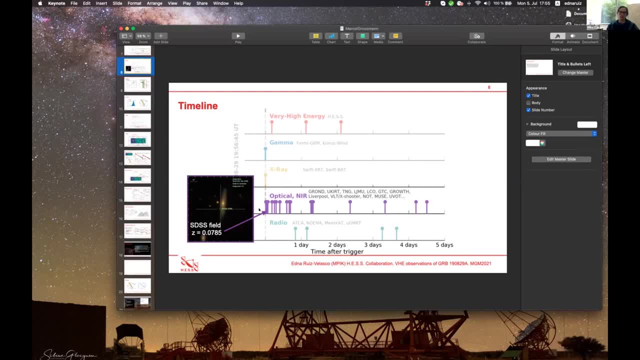 this is a long gamma reverse, so we know that it's, And we also saw the rise of the supernova a few days later. So then, for the proper modeling, I guess one needs to take into account what could be the environments. I am not an expert on anything beyond. 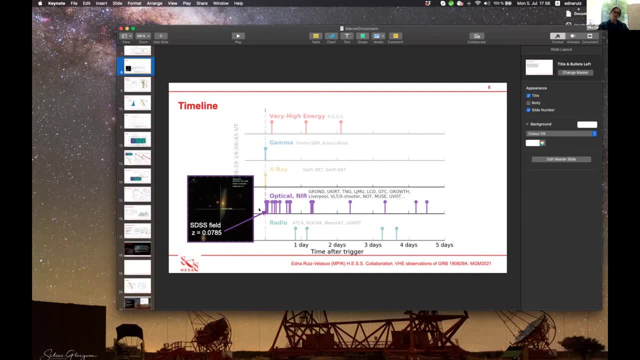 what you already mentioned. Okay, thanks. I was thinking to the X-ray aspect that Alessio mentioned, based on the paper by Sergio Campana and others. Okay, we might discuss offline also as well, by other means. Last question: Silica. 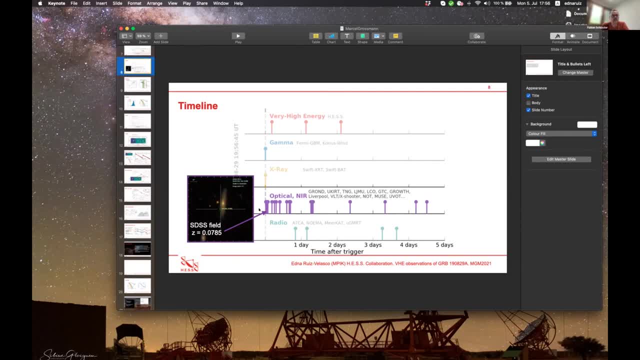 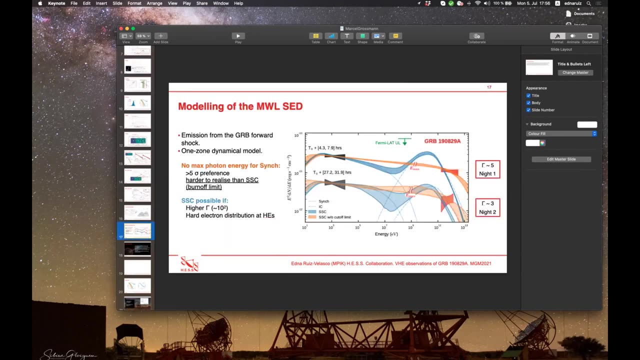 Hello, can you hear me? Yes, It's a nice talk And I just wanted to ask you something. I'm not sure if I understood correctly, So in this last but one slide- that you showed, where there is a spectrum that is dominated by a single synchrotron component. 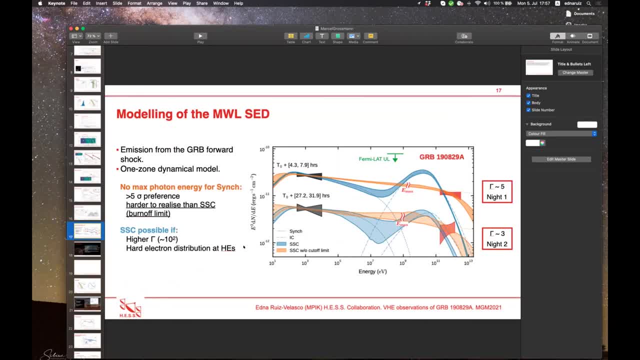 that covers this whole energy range. do you understand correctly that there was no limit placed on the maximum electron energy? Yeah, exactly. So we remove the maximum electron energy, and this is when we get this modeling in orange, And here we just indicate what would be. 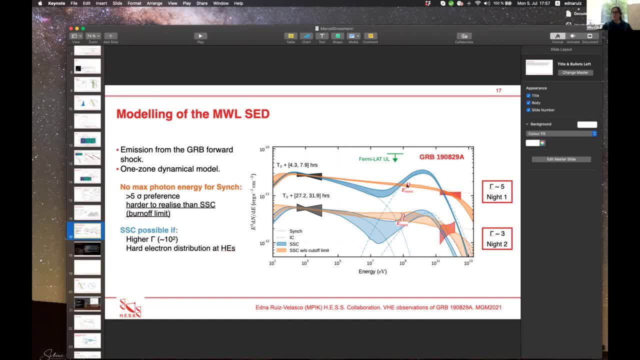 the actual maximum energy, All right, But you still call it SSC because actually inverse quantum, All right, yeah, So, exactly. So we allow for the SSC to still operate, But the thing is in the end, well, I mean, we're also showing here. 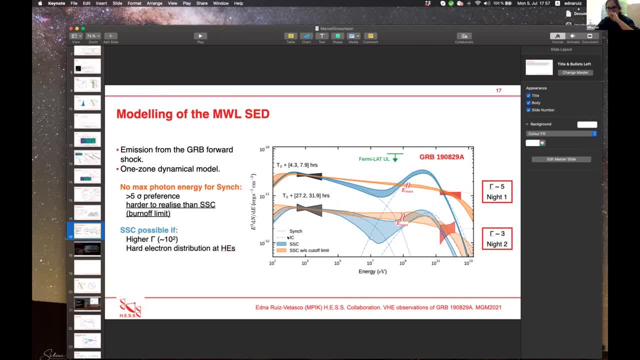 what are the contributions from the synchrotron and the inverse quantum part? So, for example, in the blue case, where we don't have the maximum, Where we have the maximum energy, in both we see here the synchrotron contribution and then the inverse quantum. 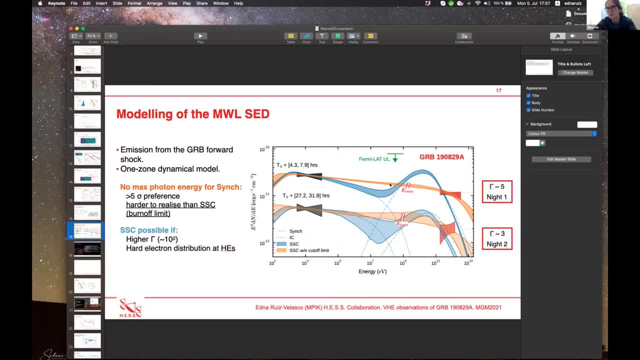 In orange we only see the synchrotron operating, And this is because, basically, the synchrotron self-quantum component is roughly three orders of magnitude lower in this case. So it's outside the plus actually, But the inverse quantum is allowed to happen. 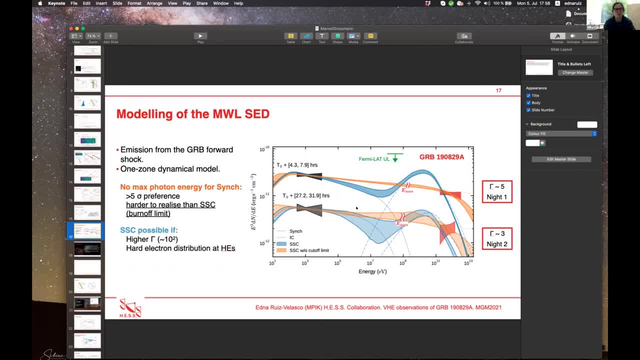 in this modeling, It's just the maximum energy that we allow it to go beyond. I mean, we don't impose it. All right, thank you, You're welcome. Thanks a lot, Edna. Thank you, Let's move on. 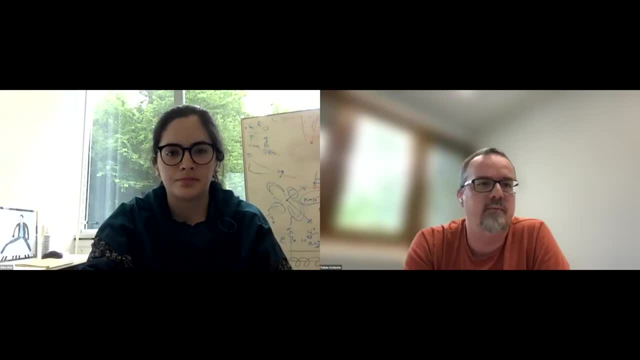 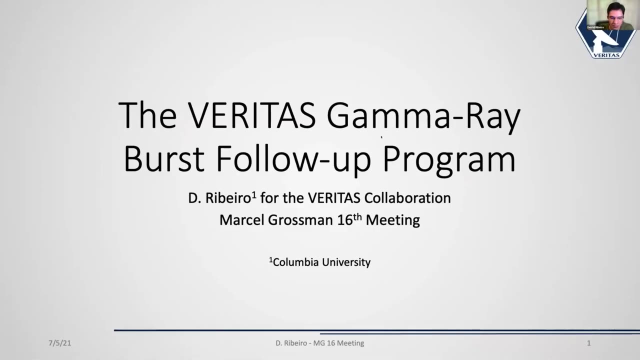 David is going to report on the Veritas program. All right, All right, hello everyone. I'm David. I'm from Columbia University, I'm a fifth-year grad student, So I'll be presenting on the Veritas gamma-ray burst follow-up program. 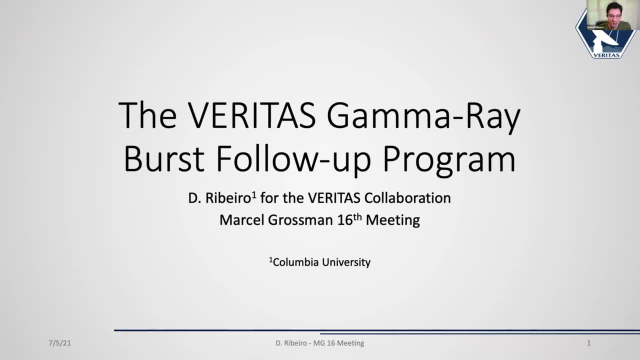 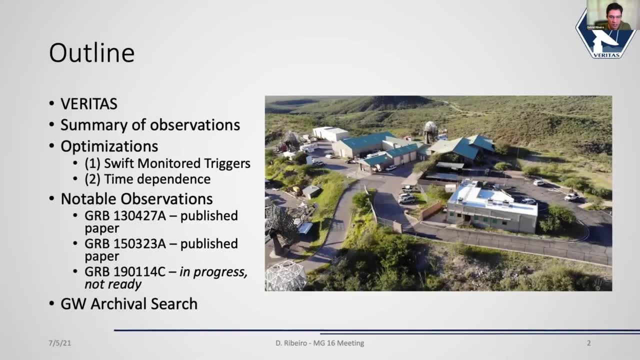 So now that I've seen the others, it's very, very similar to what we have heard before, So there'll be some nice overlap. So, to review, I'll just give a quick update on what Veritas is In a summary of our observations. 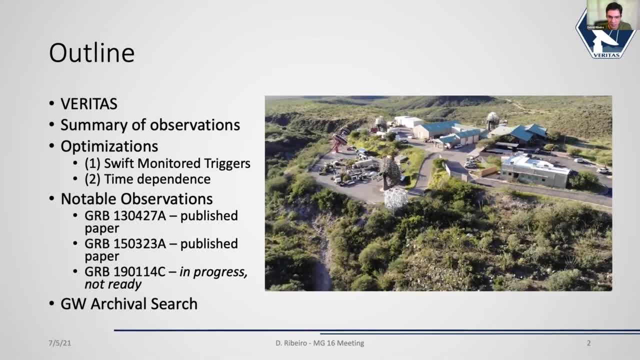 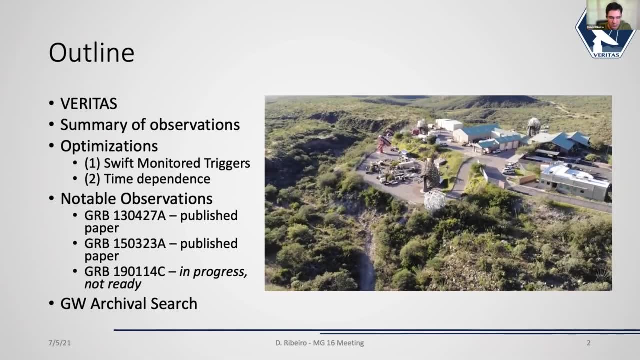 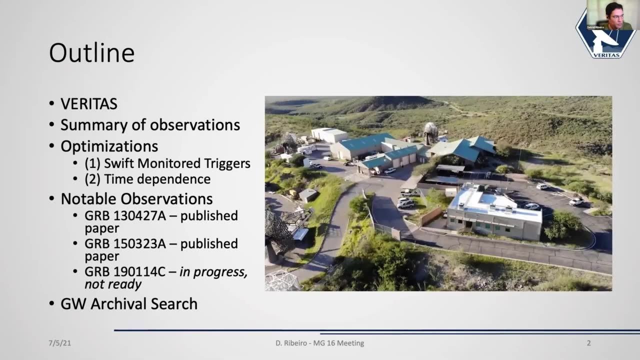 you can see here in this flyover with the drone, the Veritas base camp, We've done a few optimizations of both our ability to observe GRBs and also offline analysis of them, And I'll give a couple slides on a few published GRBs in the past. 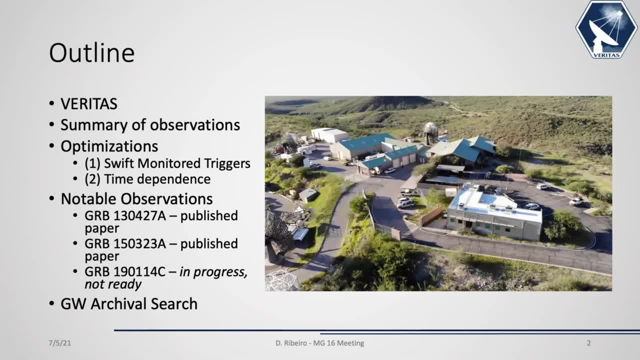 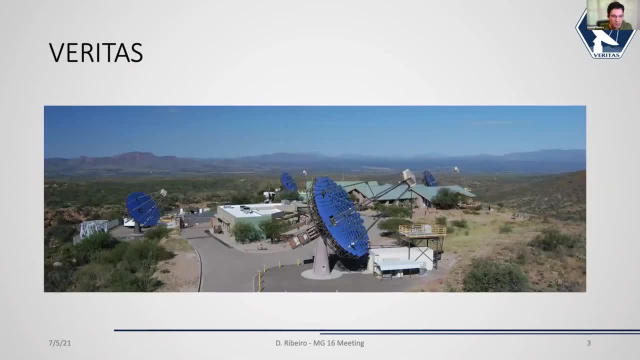 and conclude with a few slides on our gravitational wave program, which includes an archival search that has been in press right now. So, Veritas, as you can see here in this picture actually showing off the mirrors, we're a small collaboration, I think about half of. 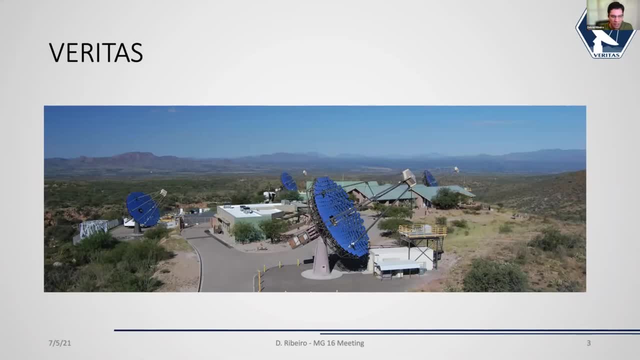 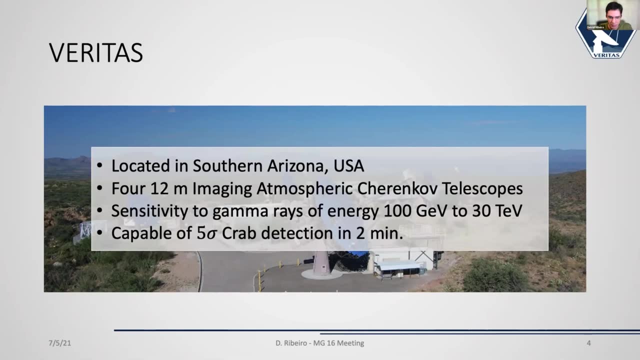 between Magic and Haspik, 80 people or so. We have four IACTs of 12 meters apiece And our sensitivity is up to energy, some 100 GeV, up to 30 TeV, So we're capable of detecting crab in about two minutes. 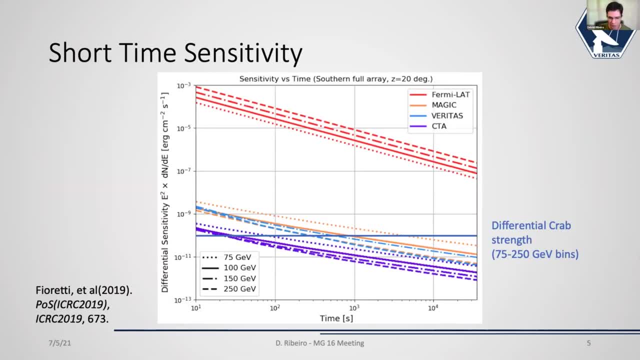 So a couple of years ago, working with Valentina, which many of you may know, we made this short time sensitivity plot showing the differential sensitivity for crab-like sources. the point source And the key thing I want to highlight here is that for a differential crab strength, 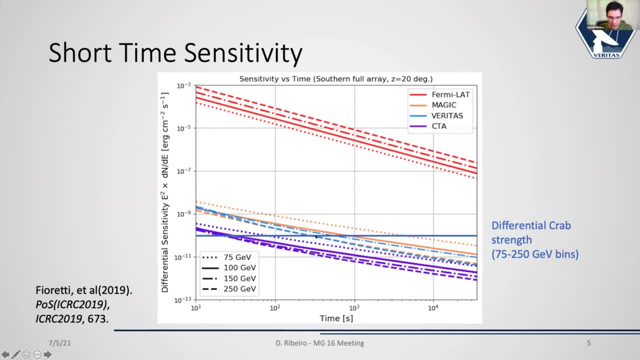 of these energies. they all overlap here. you can get a detection within a few minutes, showing both Magic and Veritas. I didn't have Hess at the time of this publication, And CTA in the future will be able to do this in just tens of seconds. 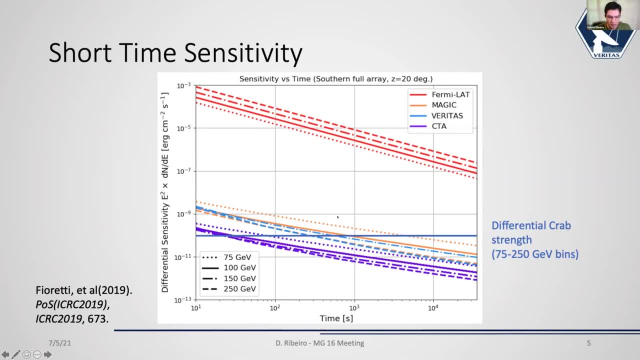 So the key thing about this is that we should be able to detect them, And now, at this point, we have several actual detections of GRBs, which is really nice. This was taken with public data to make both the Fermi and the CTA sensitivity curves. 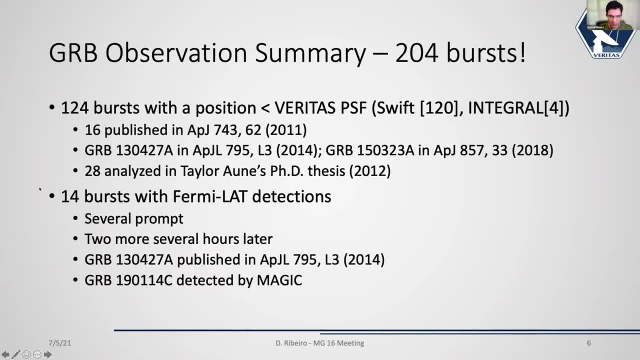 So for Veritas we've observed over 200 births, 124 of them are with positions that are smaller than the Veritas PSF. so the swift and integral births- And we've published several details about these 16- were part of this population study. 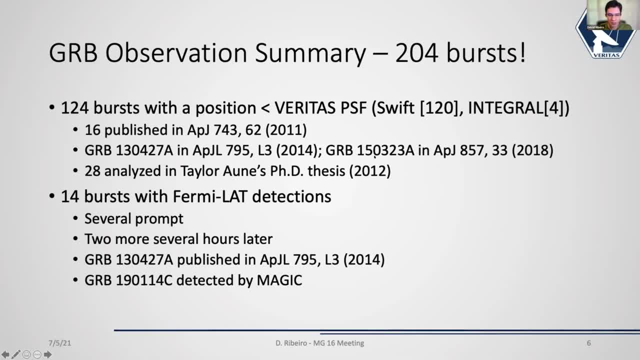 from about 10 years ago, And then two specifically 130427A- the famous one- and 150323A were published independently. We also had a graduate student who did 28 of these. It includes the 16 in his work. 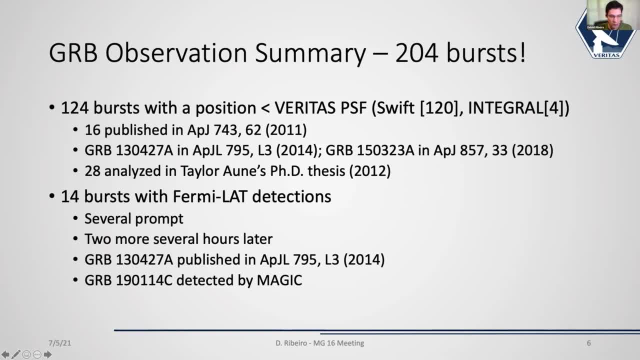 And in addition, we have followed up on the Fermilab detections, 14 of them. Several of them were following up immediately after the prompt alert, Several were several hours later. And then these two here, the one that was published, 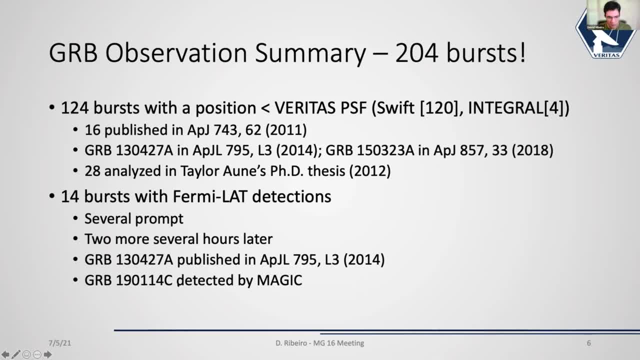 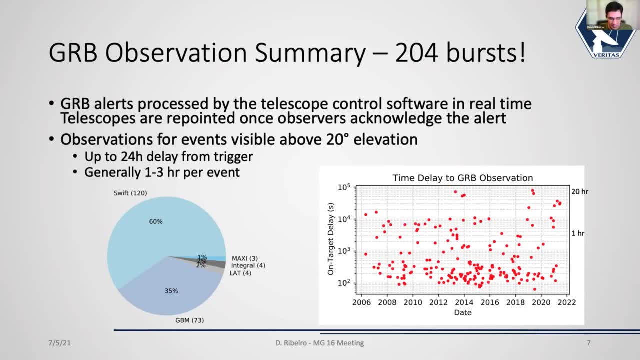 and then we also followed up on 190114C, So to give an even greater breakdown. the alerts are processed by the telescope control software, So they come in in real time. There's just a pop-up window And the observers have to acknowledge the alert. 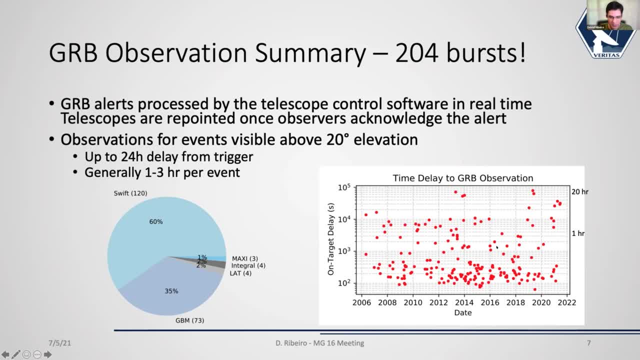 and then decide to slew, which begins automatically. So you can see in the delay plot here very similar to the others, showing over the course of the years our fastest has been around 64 or 70 seconds or so. The main thing to that is our slewing time. 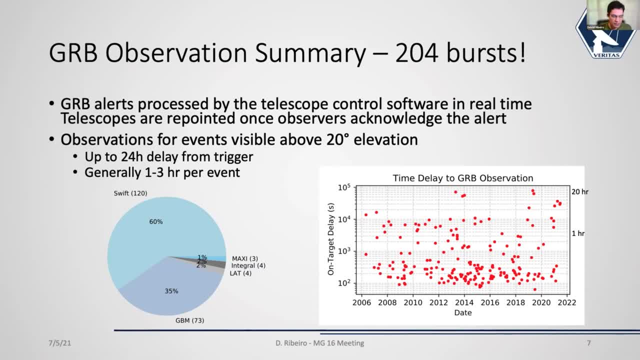 where we do about three degrees per second and per minute, excuse me, And so we generally take about two minutes to cover most of our observations And we have a standard observation time which is about three hours. So most of them between one to three hours total. 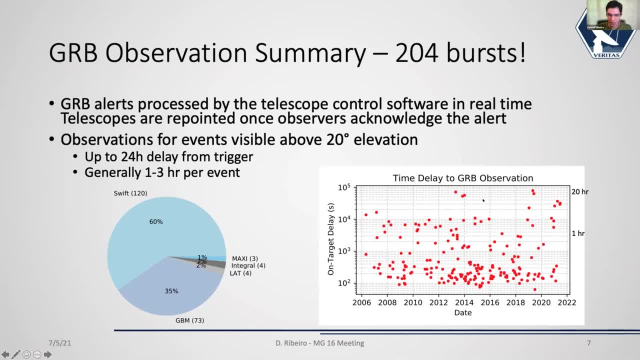 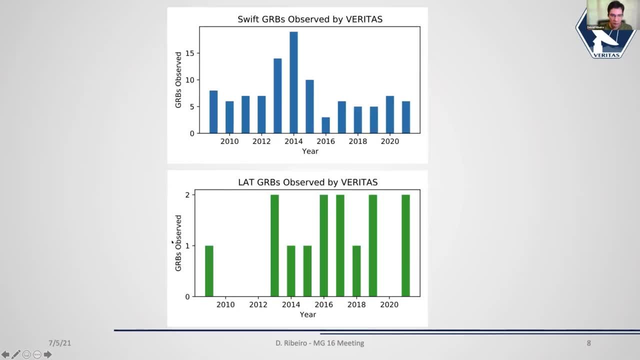 And we've observed a few that are up to 24 hours out And you can see the breakdown here: all the different telescopes that we followed up on And over the years there was a peak in 2014 that I can't explain at the moment. 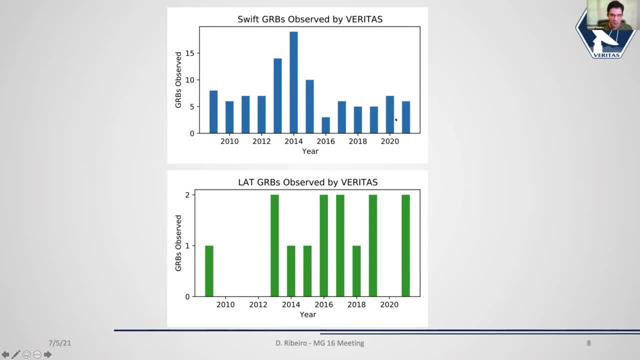 We don't understand, But we followed up on a handful of swift GRBs and also one or two lat GRBs each year, This past year, 2020,. of course, there was the COVID related shutdown, but we've continued our program. 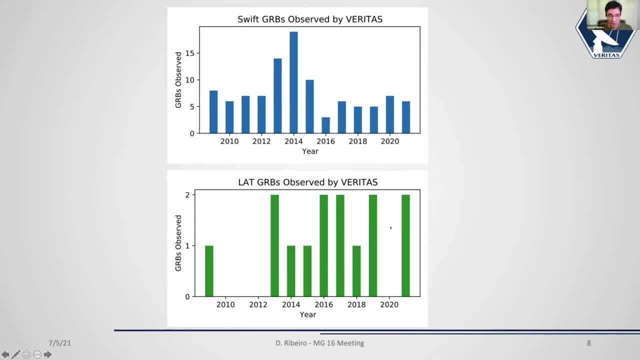 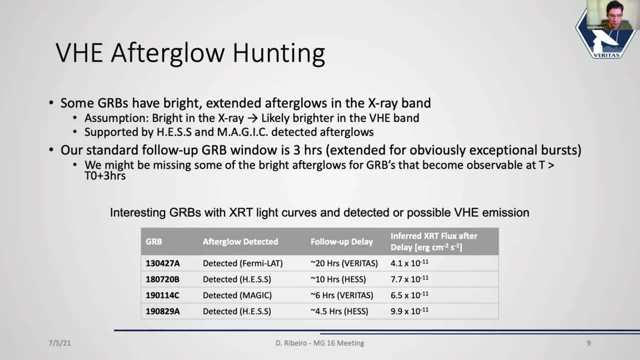 and we have been working to improve it every year- And specifically the main way we were doing that. very similar to everyone else, we're looking for the afterglow, based on the idea that the X-ray flux, if it's continued to be bright, 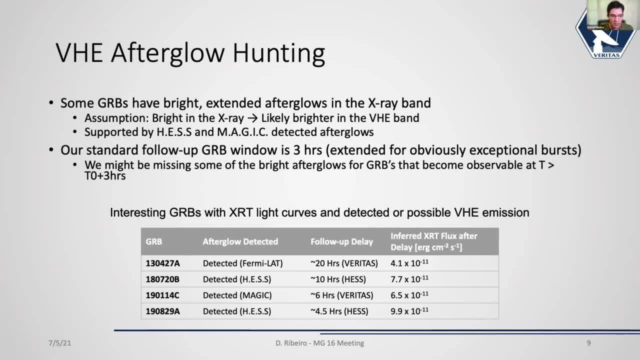 that would indicate a bright VHE afterglow as well, And so some of them, given the detections from Hess and Magic from this list down here, we use this to estimate a threshold that we can use to continue to observe. So our standard follow-up up until last year. 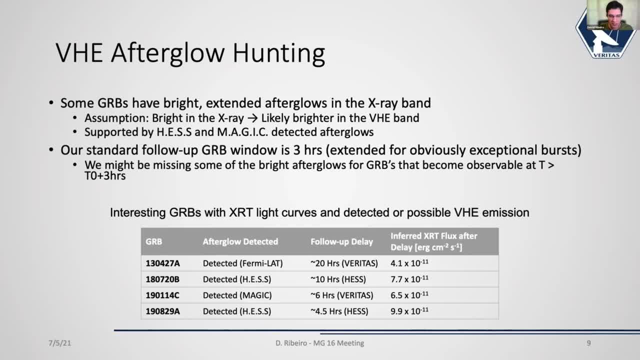 was just the three hours and then we would call it quits on that observation. But now we are monitoring. we are now monitoring with Swift XRT to follow some of the bright afterglows that we might've missed if we had continued going more than three hours. 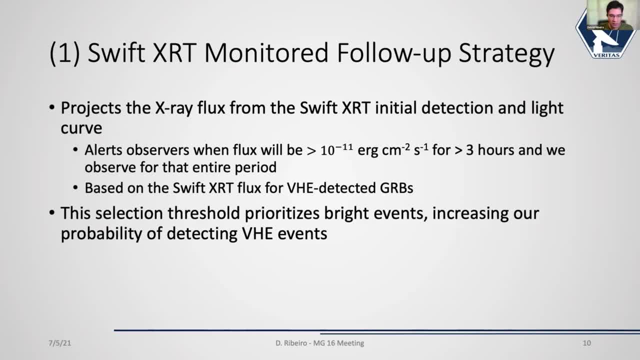 So we use the X-ray value. We have a quick look monitor and a program in our system that projects the X-ray flux from the Swift XRT initial detection and the light curve projects it over through multiple hours And then it alerts the observers via an email. 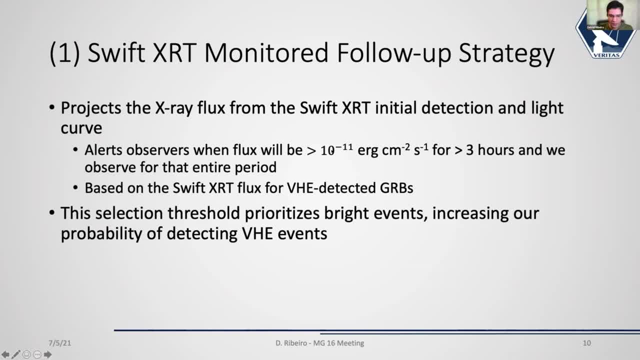 telling them how long it will be greater than this threshold of 10 to the minus 11 hertz per centimeter squared per second, how long it will be like that for us, for more than three hours, and for the rest of the time that it will stay that way. 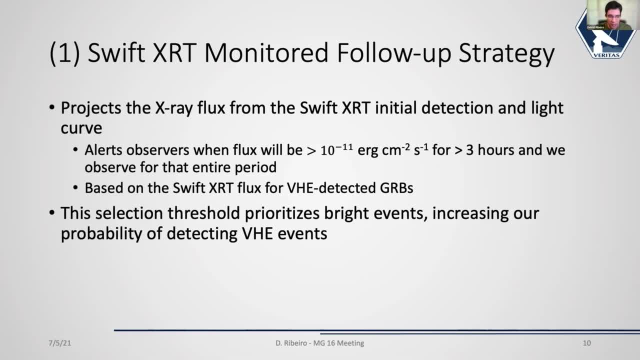 And so the main idea here, as we know, is we're gonna this selection threshold will prioritize the bright events and it will increase our probability of detecting the VHE events so that we can continue to follow up on them. So a second part of the work that we're using. 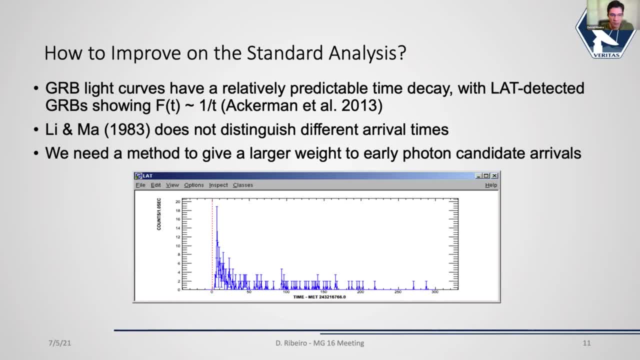 to try to improve our ability to detect is to improve our standard analysis And specifically, this is the offline analysis. So we know that the light curves fall as approximately one over T in the time domain, but Li and Ma doesn't distinguish between the arrival times. 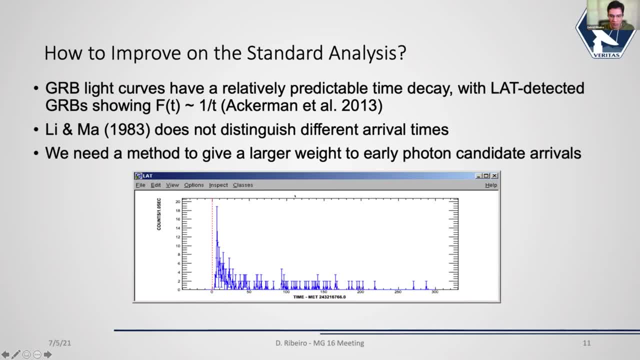 And so we need a method to give larger weight to the early photon candidate arrivals. As you can see, this is the. a lat counts as a function of time. Most of them are in the first 50 seconds and then sparingly throughout the next five minutes. 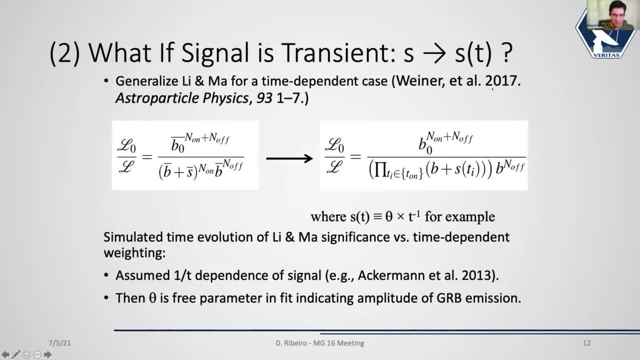 So the way to do that, we published a paper in 2017 that took the Li and Ma equation and applied the. here's the likelihood ratio using counts. ratios, counts, rates: modify the signal counts to make it a signal counts as a function of time. 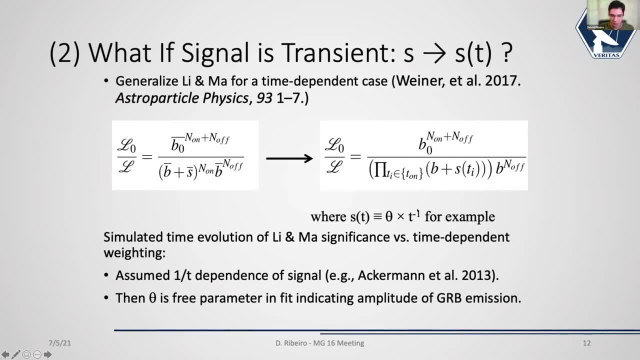 with something like a theta times T to the minus one, for example, or T to the minus beta of some kind. In this simple work he was able to rework the Li and Ma equation, And now we have that in our standard analysis pipeline. 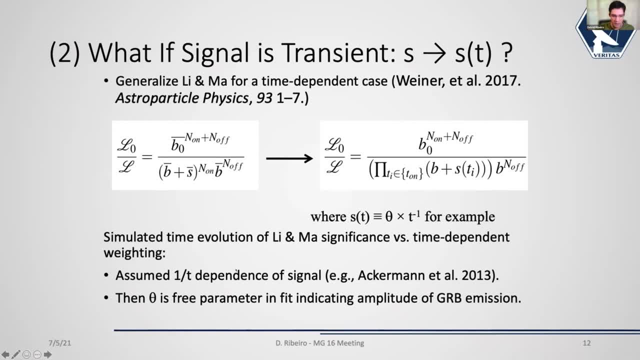 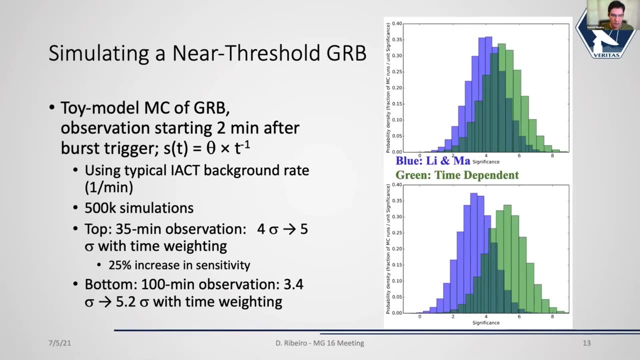 in the offline analysis, Assuming some sort of T to the beta dependence, And we can easily do some simulations to confirm that this is a proper, a proper technique to use. So we used some Monte Carlo of a GRB, starting the observation two minutes after the burst. 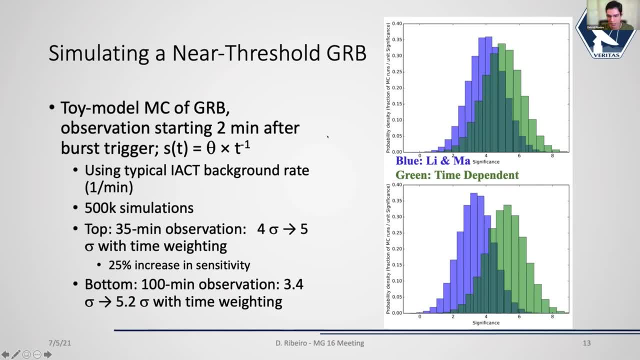 using the typical background rate of about a gamma per minute. If you do 500,000 simulations and you calculate all the significances for each of them and draw distribution, you can see that for 35 minutes. if you look on this plot on the right here: 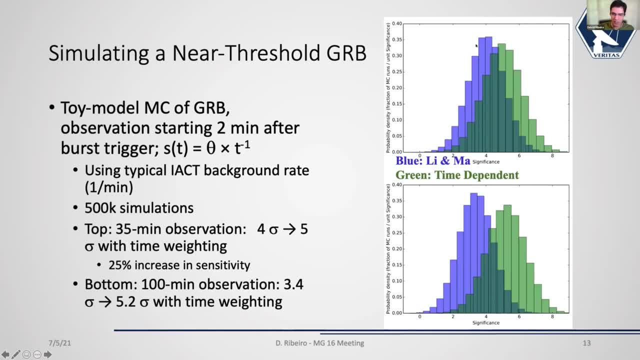 for 35 minutes without the time dependence, just the standard Li and Ma. you have a mean, a peak here of about four sigma, And then you want to supply the time dependence, that goes up to five sigma. And if you increase your observation window, 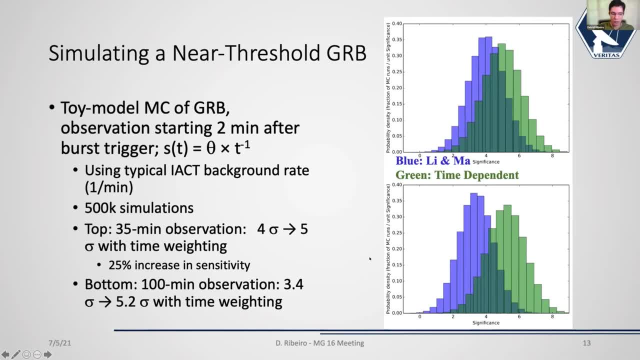 to a hundred minutes. you have a lot more data which will help with this estimation, And you can see that it the two distributions start to separate and the significance peaks at a much higher value. So the key thing to notice here is that with more data, 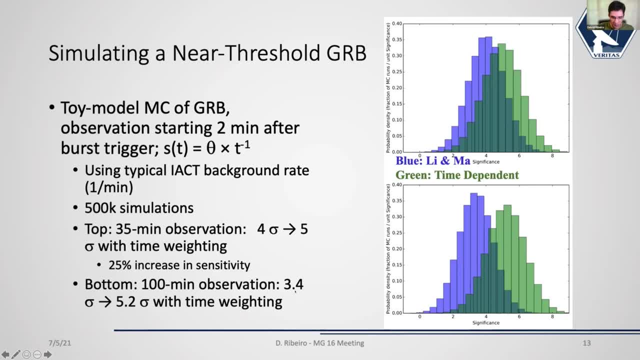 not only does the Li and Ma get worse from four to 3.4, the time dependent version goes from five to 5.2 and gets better, which makes sense if you think of how the significance varies as a function of time As you have more data. 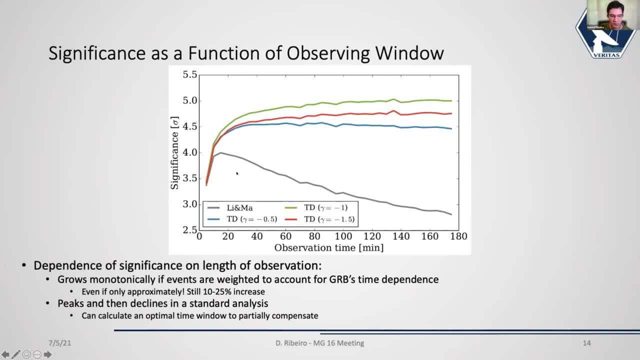 you have more backgrounds, but this is also more accounts coming into your field of view, which is going to dilute your significance. But if you use a time dependency and you weigh them properly, that significance is going to remain flat. It's going to catch the thing. 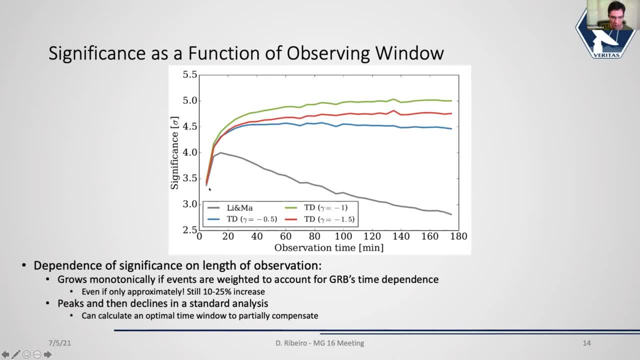 that you expect it to catch at the beginning. So we can calculate, we can estimate a good, reasonable value for the time dependence, a function of T to the minus one or 1.4.. There's also ways to get that value from contemporaneous observations at the time. 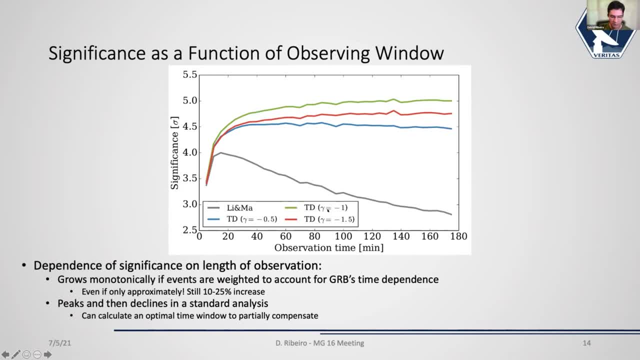 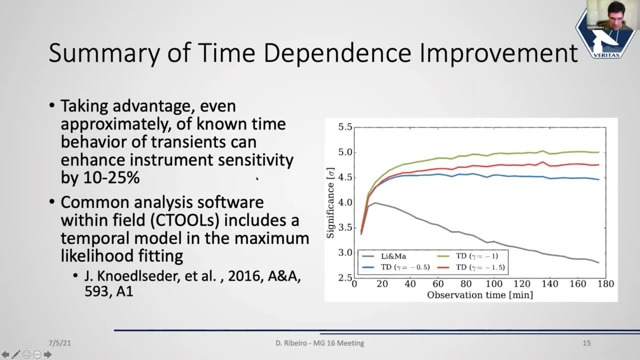 And so we can use that and the burst T- zero value- to have a good format in order to improve our time dependence. So, in summary, we can take advantage of this system. We can increase the sensitivity by 10 to 25% And you have access to this in certain analysis software. 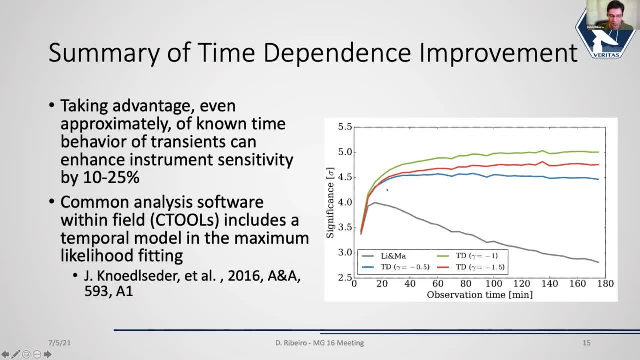 such as C tools, where you have a temporal model and the maximum likelihood fitting. So in our case, this is explicitly written into our analysis package for Veritas. So, using this, let me focus now on a couple of events that we've published. So the first one, so the famous 130427A. we followed up on this 20 hours after the Fermi observation of it. They had about 19 hours worth of detection, but they continued on. They detected it during that 19 hour period. 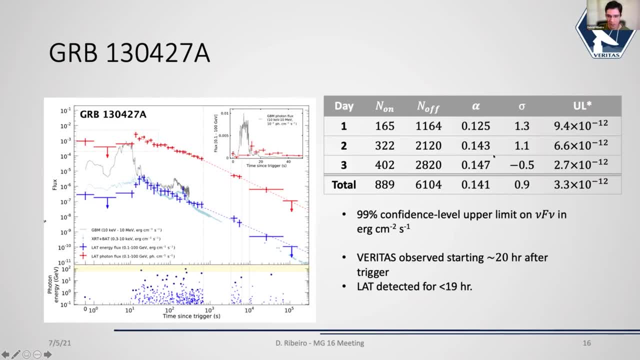 At the 20 hours we started and we did three nights worth of observations And you can see here the significance are not supremely high, They're not detections, They're simply upper limits. but these upper limits were useful. We were able to publish a paper. 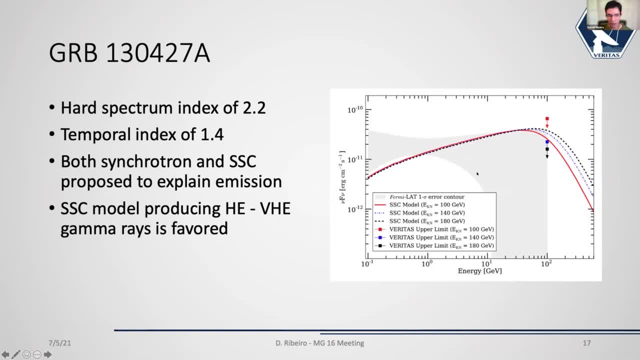 that showed in the SED here, with the heart spectrum of 2.2, temporal index of about 1.4, we can favor a synchrotron self-compton model to show that it is in the more complicated regime, as we've been seeing in the detected GRBs now. 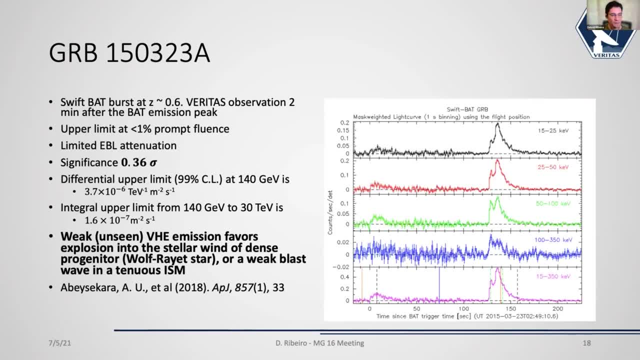 And then moving on, we also have worked on 150323A, And this was a normally distanced event, a redshift of 0.6.. And we observed two minutes after the BAT emission peak. So the key theoretical framework here we used. 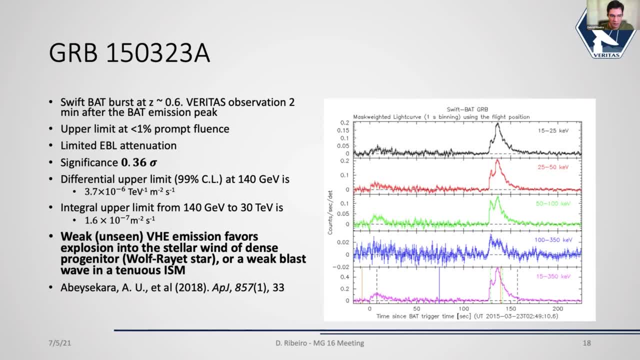 was to look at the affluence and try to constrain the affluence in comparison to the swift BAT affluence- And we were our upper limit was able- was at a 1% of the prompt affluence. So because of this redshift, 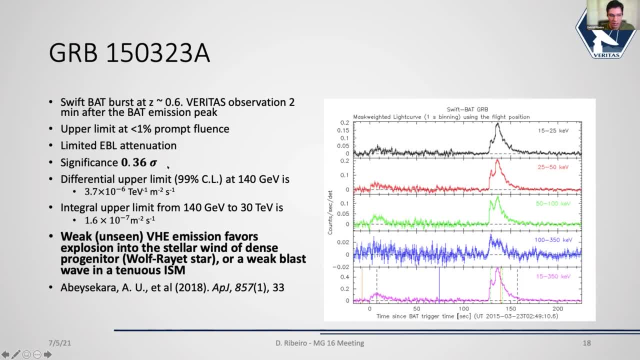 it wasn't a very strong ABL attenuation but at the end, at the end of the day, we didn't have a detection and we had a significance of about 0.36.. But even then, with this upper limit, that came out of this result. 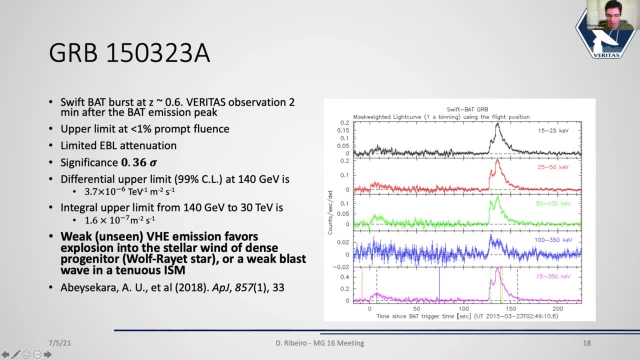 we could constrain the burst itself to some sort of explosion into a stellar wind within nearby a star or a weak blast into an interstellar medium, And you can read more about that in this paper here. This to just. I didn't mention here. 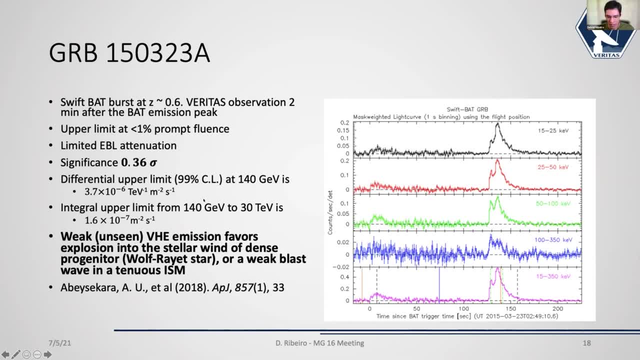 but this event was detected by looking at a population study back in 2017 to find events that were most likely to have a good constraint available to us, And so this is one of the best ones in our catalog of observed events. And then, finally, 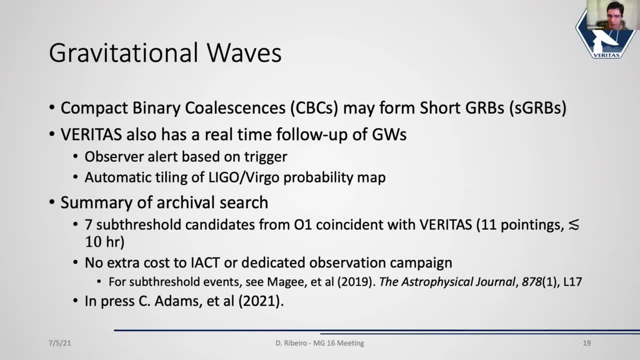 our gravitational wave program. as we know, the compact, the compact binary coalescence, the CBCs. they may form short gravitational wave, short GRD, excuse me. So we have a, so we have a real time followup when 03 was happening. 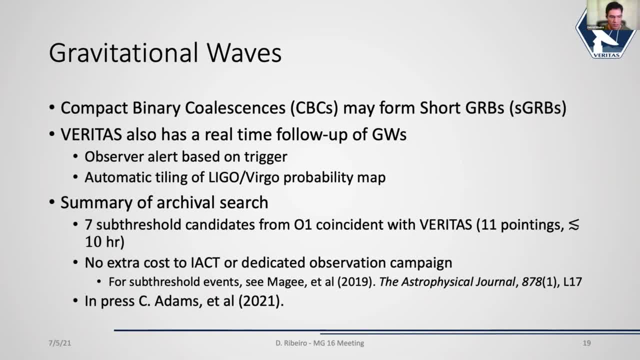 The observer would get a trigger very similar to the GRB trigger, but in the background. this program would also tile the LIGO Virgo map and give us a five minute observation positions so that we could scale through all the way. In addition to that, 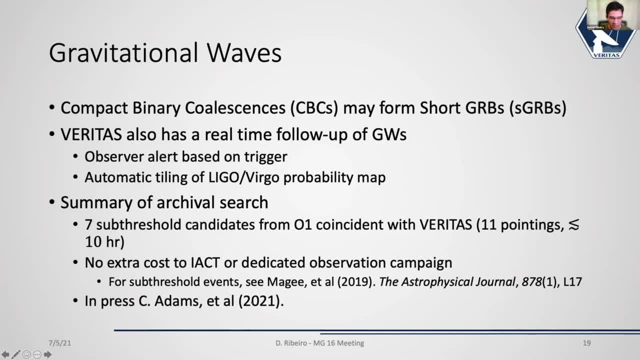 we've also- it's currently in press- CB Adams 2021 paper. we're looking at the archival search and using all of the coincident observations from Veritas during the 01 campaign So we found seven threshold candidates from that campaign, where there were 11 pointings from Veritas. 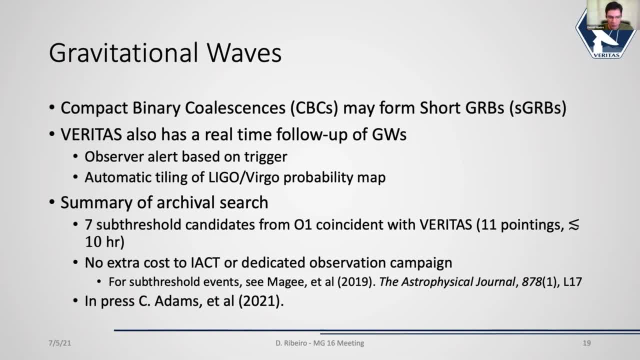 worth about 10 hours total This process, this whole, if you can check out this paper, but this whole procedure comes at no cost to our telescope, to our ACT or no dedicated observation campaign. We just need it. The list of sub-threshold events from the McGee paper. 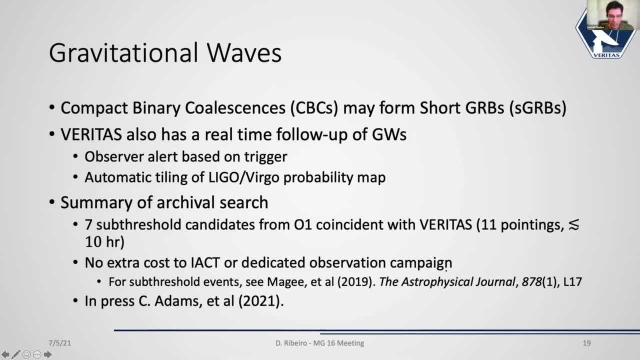 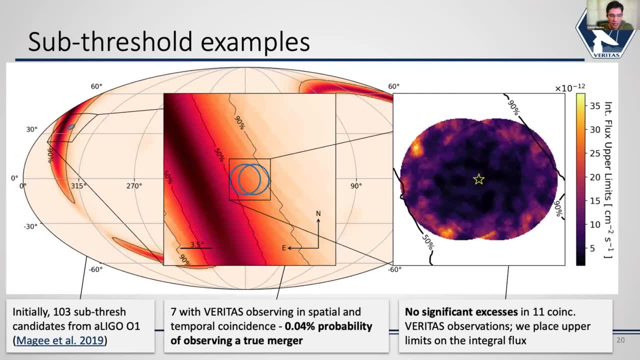 which you can get and then go back and look at your, look at your archival observations to do analysis on. So, to show an example, here's a map from one of them. You can see there were two tilings at the time in the 90% region. 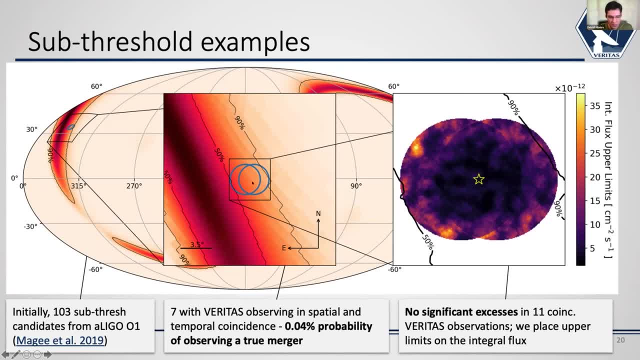 and there were no detections for any of these 11 pointings. but you can draw an upper limit map for the entire time period And with this map we can say there was no detection and the total combined probability of observing a true merger- if there had been something- was only 0.04%. 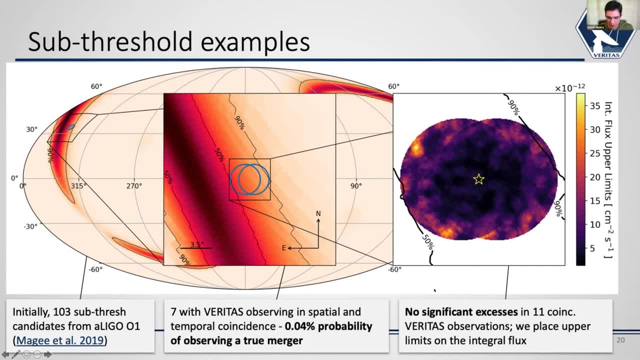 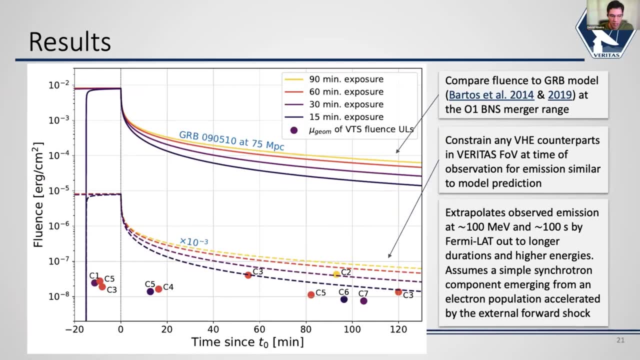 So we really ruled out our ability to see anything at the time. But you can take these upper limits and combine them with a short GRB model And you can see that for various fluences, for our observation times, there's the delays. Most of these were within a factor of a thousand. 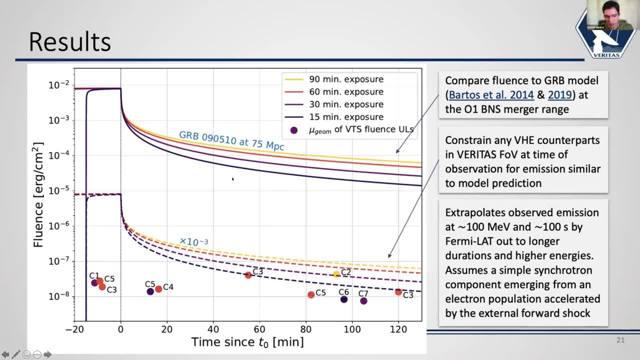 of a model of 090510,, which means that if an event like 090510 had happened, with very similar observation criteria as what LIGO Virgo can observe- these are the numbers here- we would have seen it. It would have been extremely bright. 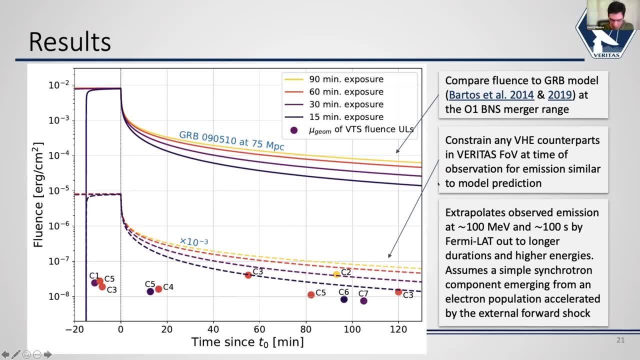 and would have been able to roll out to get a lot of details from it. So this is a great technique that you can apply to your GRB program. looking at archival data, I think LIGO Virgo will need MOUs for O2 and O3. 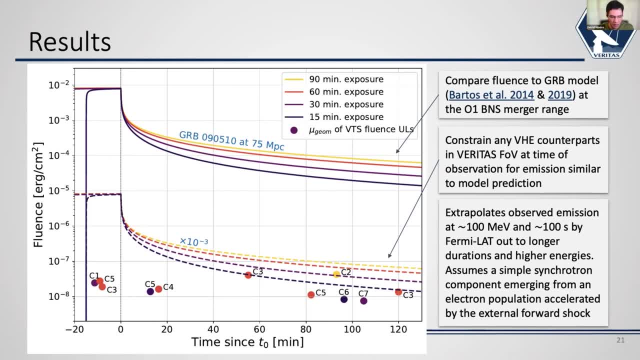 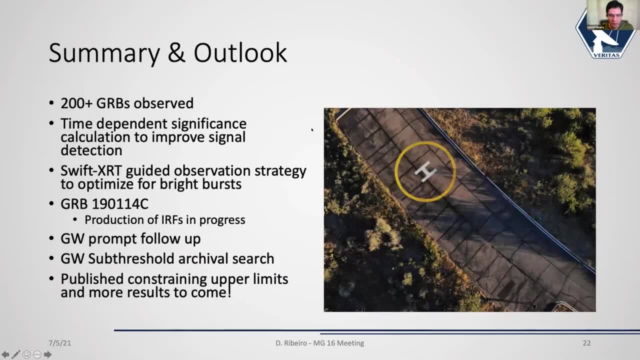 They haven't revealed yet whether they'll publish in the same way this sub-threshold catalog. So, to summarize, we have observed over 200 GRBs. We have a time-dependent significance calculation that'll help us in offline analysis for the future. We're also following up with the X-ray flux. 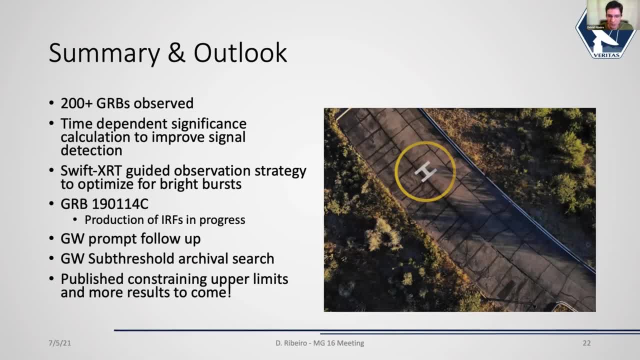 in order to help us select the brightest of the bursts For 190114C. we did observe it. It had all of the worst observational criteria that you could think of. So we've been steadily working on our IRFs. It's taking some time to make all. 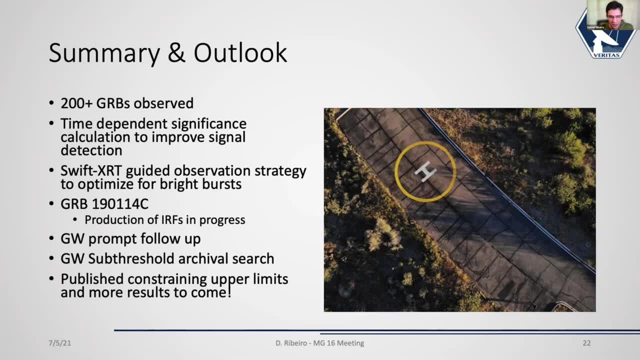 of the possible simulations to do that. We also have. I also spoke about the gravitational wave program, the prompt follow-up and the sub-threshold archival search. So we're working on more and the analysis. we're steadily going through all of our 200 observations. 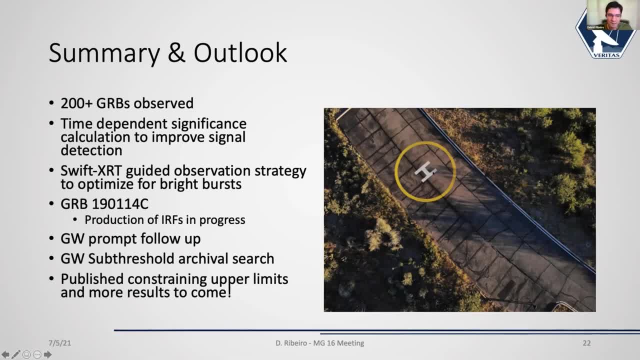 and we'll have more results to come in the near future. Thank you, Thanks a lot, Very interesting. I guess everybody agrees that you should be the next one of the IACTs to take the GRB. Yes, of course, I'm waiting for it. 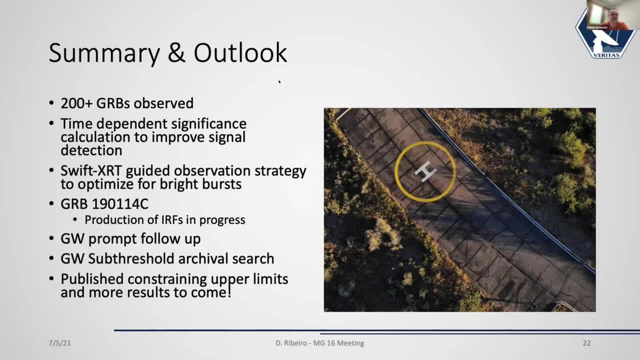 Are there other questions? Just a very basic one: What is this picture that you have in this last slide? It is the helicopter arrival. Please say what is that? Oh, we had a drone. We were at base camp and we had a lot of fun with the drone. 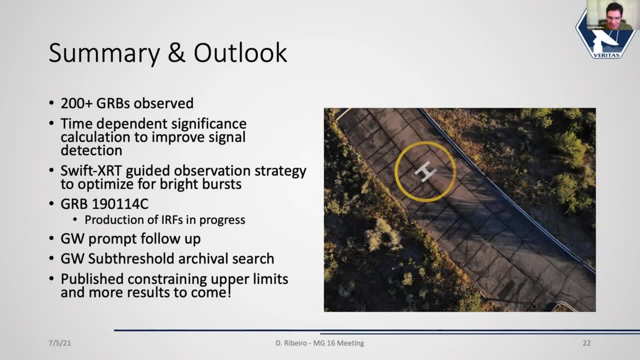 So this is at the top of the mountain, the pad that is right next to the telescopes, in case for emergencies. Okay, thanks, Bye. Very quick question on your GRB modeling for the archival search related to the gravitation wave events. 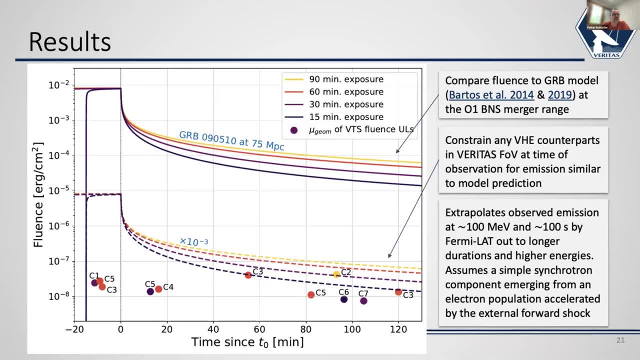 Are these assuming on-axis GRBs or do you also allow for off-axis GRBs like GW17 or 817?? We, at the point of the paper, only did on-axis. I think it would have been a little bit more challenging to do off-axis. yeah, 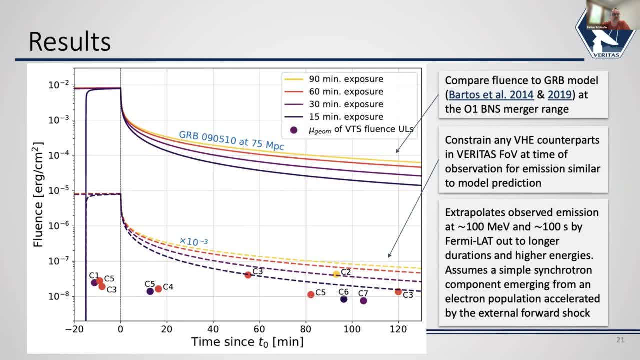 Because that might change the picture right, Because there was no, Yeah, No very high energy emission associated to GW17 or 817, which might be due to the off-axis nature of the event. so that might happen again, Which would have had also a different fluence, right. 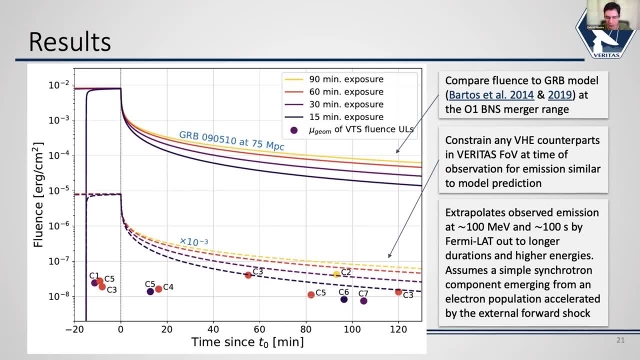 a different time. dependence off-axis. Okay, I don't see any other questions, Can you, Edna? you go ahead. I don't know how to raise my hand, so I have to just jump like a wild person. Yeah, I wanted to ask. I mean. 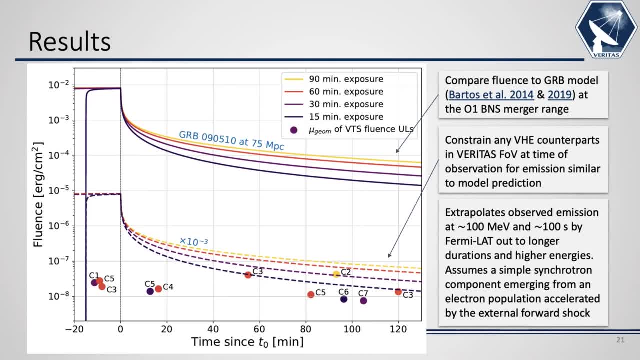 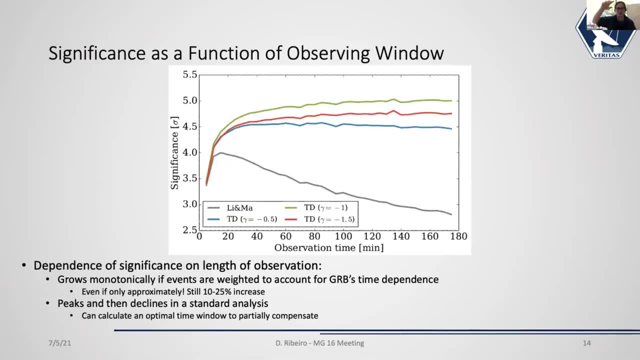 in slide. Where are we 14?? Oh, I mean this model, no Of the Exactly of the long integration time or, depending on how your observation is, Do you take into account the background rate, like the proper background rate? 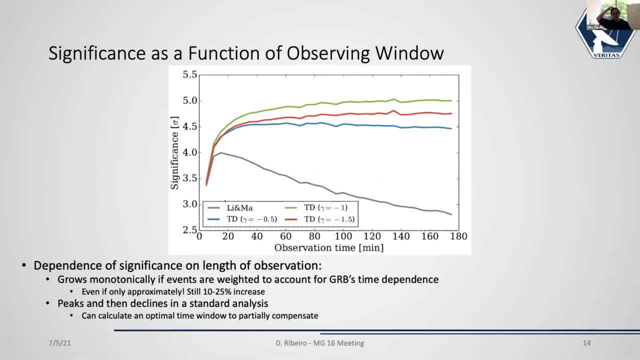 on the way that the ICT is observing through the sky. So we do. actually, I didn't mention it in these slides, but we do. That was also part of the simulation. If you could vary the background rate as well. Both have a time dependence. 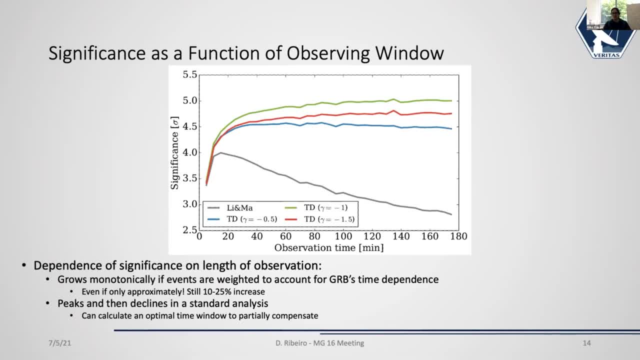 And I imagine that I mean in the end, you get an answer that this is very dependent on the way that the gamma rivers are being observed, in terms of the zenith angle of the ocean, Of course, yeah, Or how big is the impact? 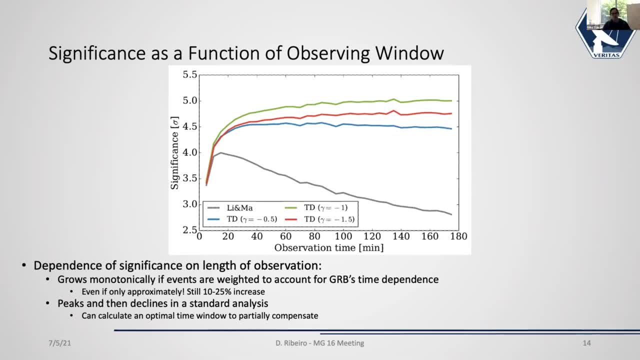 I mean, that's my question- How big is the impact of the zenith angle in terms of this optimal time of integration? I have to check It. would It could be significant, depending on how far you're going, If you're, you know. 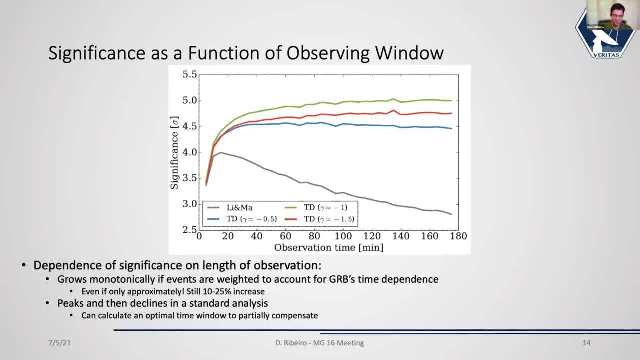 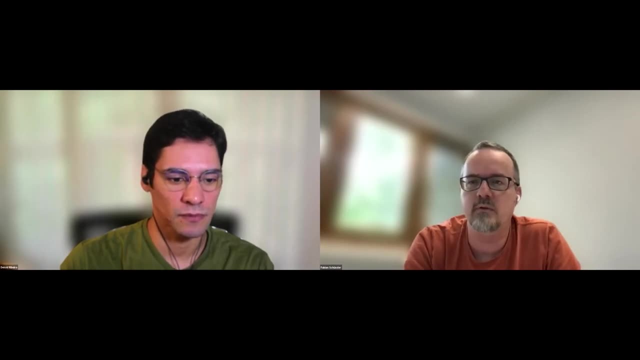 if you're swimming several tens of degrees over the course of your observation, it would be significant. Okay, thank you. Okay, Thanks again. Thanks, David. Let's move on to Christy, who will talk about the HAWC air shower array GRV program. 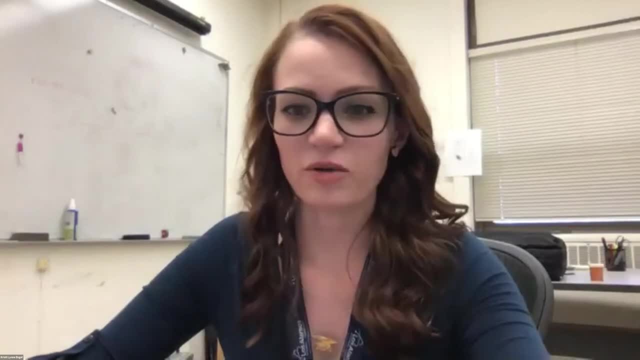 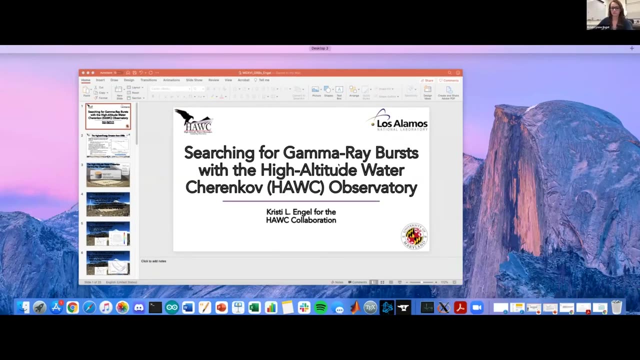 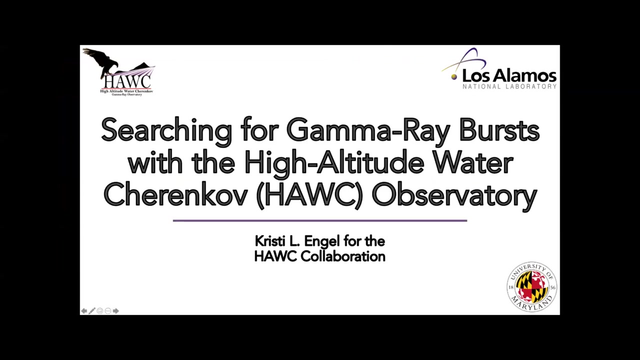 Yeah, just completely throw a wrench in everything and talk about survey instruments instead now, Good, can you see my slides? Yes, perfect, Okay, Just move you guys. So this will be looking for these very energy emissions from gamma ray bursts with HAWC. 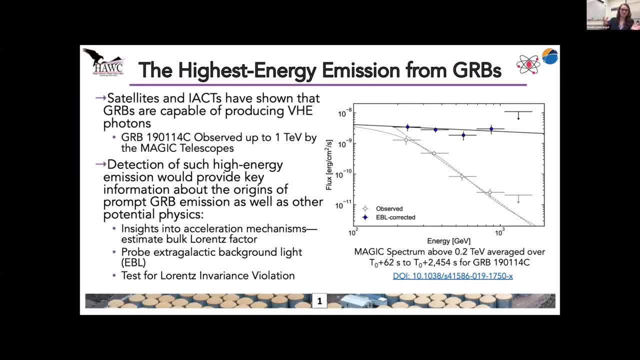 So obviously this entire session is about GRVs, so we don't need to cover too much about what they are, but satellites and ICTs have shown that GRVs are capable of producing such VHE photons. This is really motivated by the detection of GRV 19-0114 Charlie. 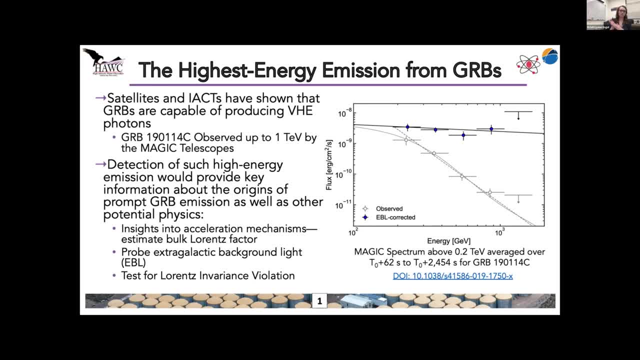 which is the long GRV observed, up to 1 TeV, by the magic telescopes in the afterglow, about one minute after triggering for BGBM and the swift bat. So the idea would be that if HAWC could see such high energy emission, 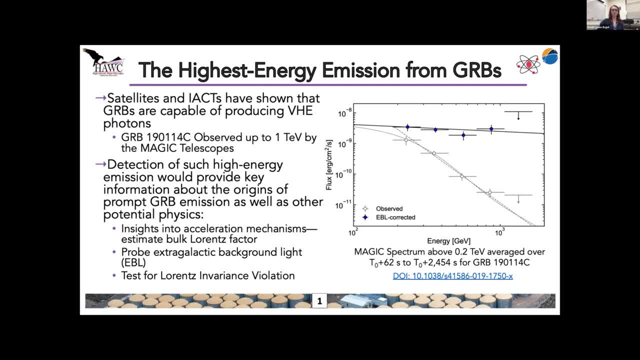 it would provide really critical information about the origins of prompt GRV emissions and a bunch of physics. We would be able to constrain or probe the extra galactic background light of the GRV, And this would be over cosmological distances. The GRV spectrum above 10 GeV can be used to constrain the Lorentz. 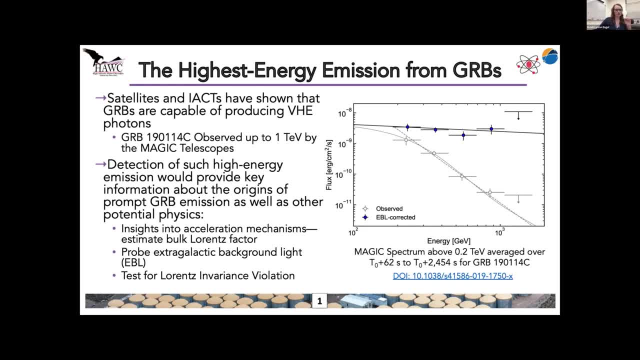 invariance violation, And we would also obviously look for insights into the acceleration mechanisms that would be estimating the bulk Lorentz factor. And really only a wide field of view observatory with a high duty cycle could place such constraints, because the key to success here is really: 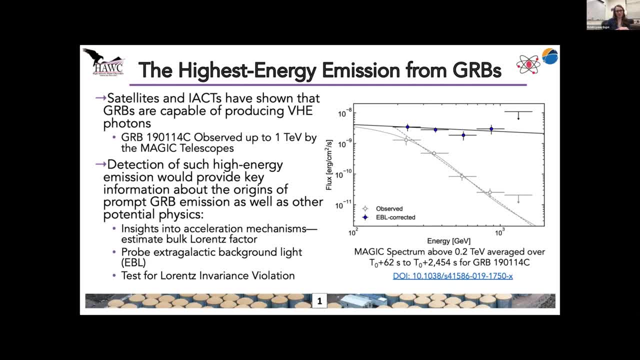 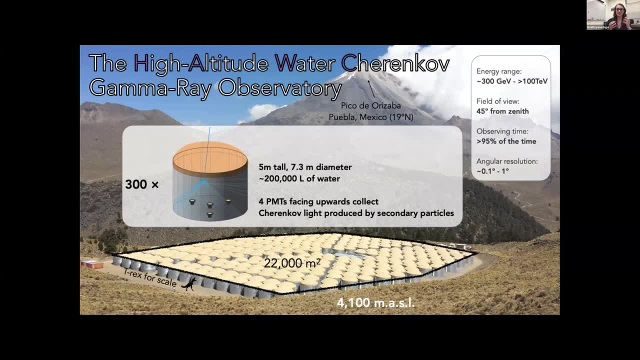 the ability to catch a burst, as it happens. So about such a wide field of view high duty cycle observatory? The High Altitude Water Cherenkov Gamma Ray Observatory, or HAWC, is a successor to the Milagro Observatory. 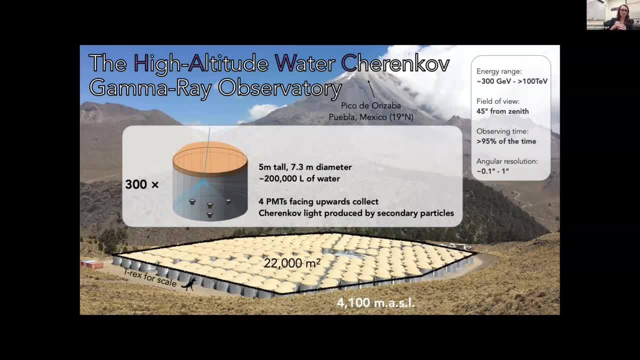 It's a ground-based air shower array inaugurated in March of 2015.. So that's when we turned on the full main array and started really taking data. It's located on the side of the Sierra Negra volcano in central Mexico. 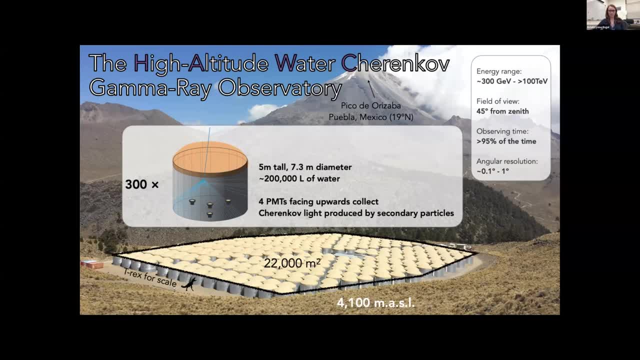 It's at an altitude of 4,100 meters above sea level. It comprises 300 water tanks. They are all instrumented with four upward-facing photomultiplier tubes, So you can see those here. There's three 8-inch PMTs and a central 10-inch PMT. 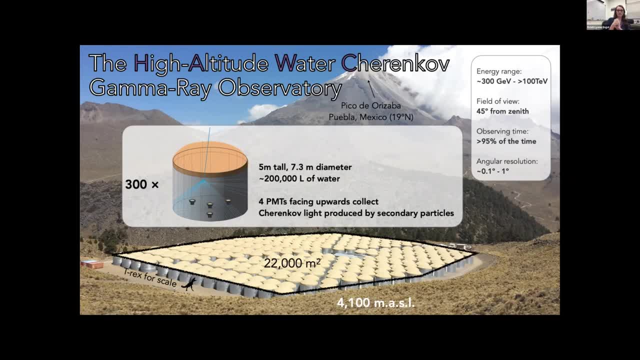 And they detect the Cherenkov light produced by secondary particles. because every one of these 5-meter tall, 7.3-meter diameter tanks, which we can genuinely use a T-Rex for scale here, is filled with about 200,000 liters of water. 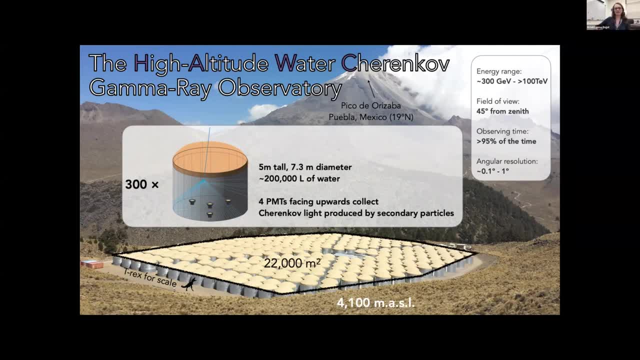 And so that's a lot. And so we detect the secondary air shadow particles at ground level from both gamma and cosmic ray primaries. We are up about 95% of the time or greater, with an energy range from about 300 GeV to above 100 TeV. 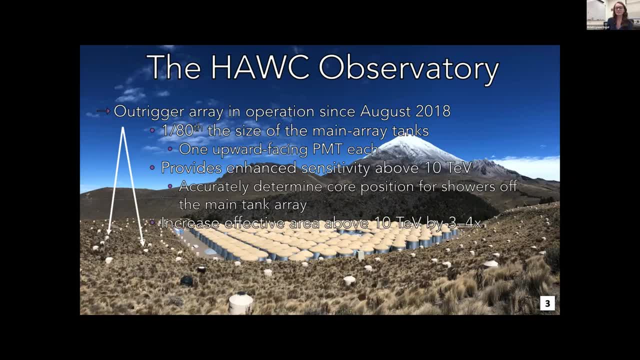 Additionally from the image that you just saw, since in 2018, we began using what we call the Outrigger Array. These are a bunch of small tanks surrounding our main array instrumentation. They're 1-80th the size of the main array tanks. 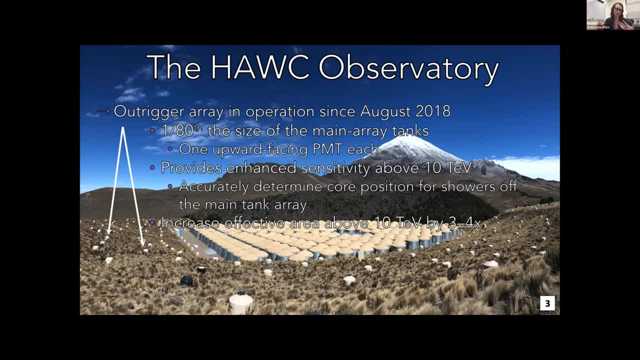 and they each contain one upward-facing PMT as well as a bunch of water, And they really provide enhanced sensitivity above 10 TeV And this allows us to accurately determine core positions for showers off of the main tank array And it increases our effective area above 10 TeV. 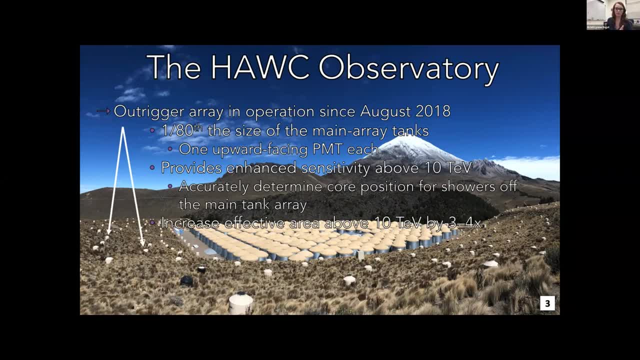 by about three to four times, which is a really significant improvement Theywe have. we've been taking data since 2018, but they'll really be analysis-ready in late 2021.. So thosethe data from these will really be upcoming results. 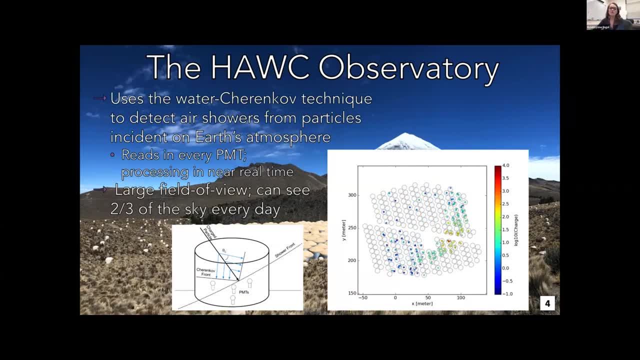 So all those combined. both the main array and the Outrigger Array use the Water-Cherankov technique to detect the air showers from particles, incidents on the Earth's atmosphere. Our system reads in every single PMT and processes this data in near real time. 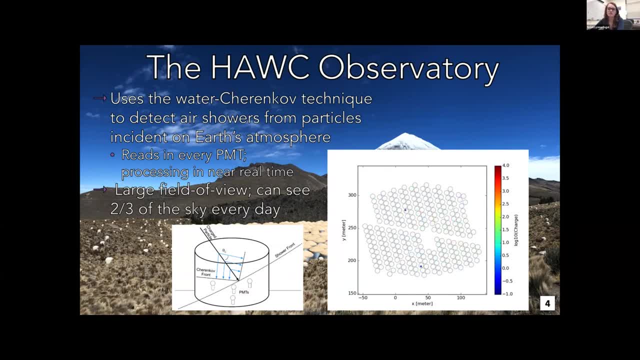 We only have about four seconds of delay to reconstruct these showers all day, every day, So this results in a really large field of view. We can see two-thirds of the sky every single day, And so what that shakes out to with our differential flux, sensitivity is. 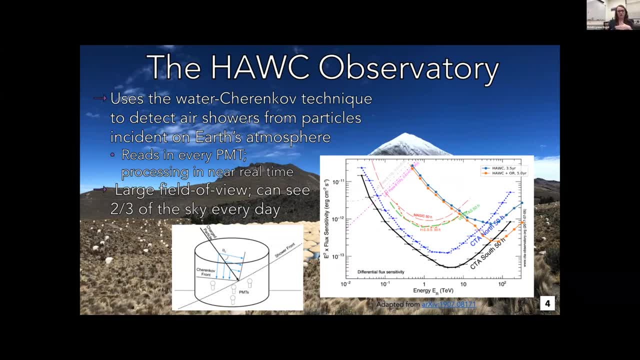 especially in the Northern Hemisphere. we're one of the most powerful high-energy detectors And you can see here in orange the really significant improvement we get at the highest energies with the Outriggers And overall. these properties allow us to search for new sources. 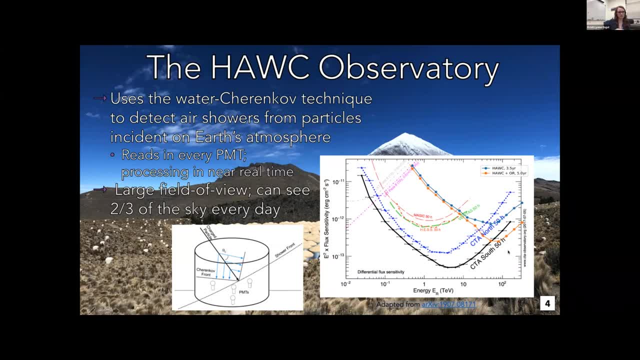 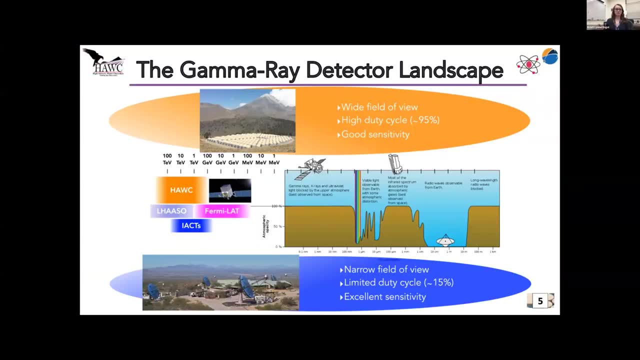 as well as go back and search archival data. So we can do both. We can look in real time and we can look in archival data as well. Especially since there's been a lot of talk about the IACTs. how do we compare in the gamma-ray detector landscape? 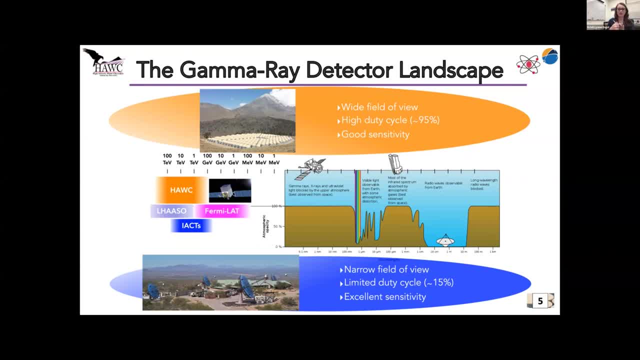 So obviously we have a wide field of view and we have a really high pointed instruments in our field of view and a much more limited duty cycle, more limited by weather than we are. We can observe day and night, no matter what. 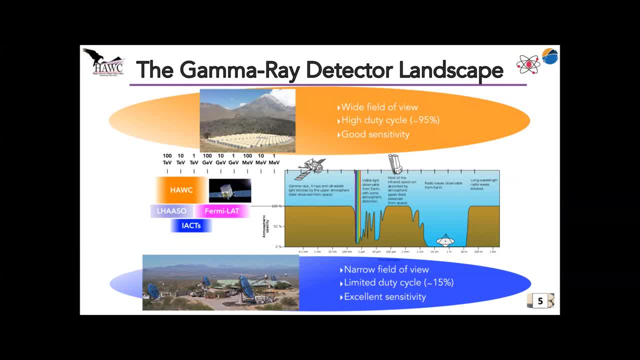 I'm going to turn off my video because it says my internet's unstable, so I apologize, But the IACTs have really excellent sensitivity, So there's really good complementarity here between the survey instruments like HAWC and the IACTs like MAGIC and HESS and VERITAS. 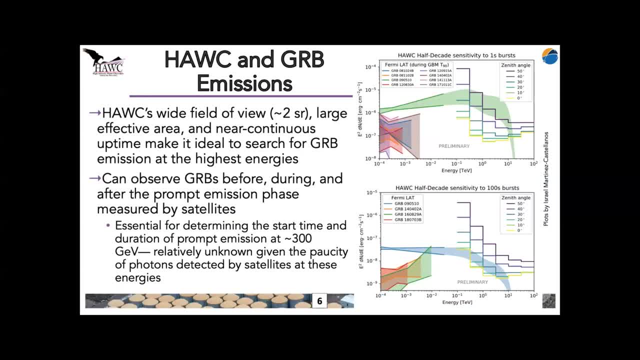 So, particularly for HAWC and these VHE gamma-ray burst emissions, our wide field of view, which is one-sixth of the sky at any given instant, is really needed to see the high-energy transients like GRBs, which typically have prompt emission durations. 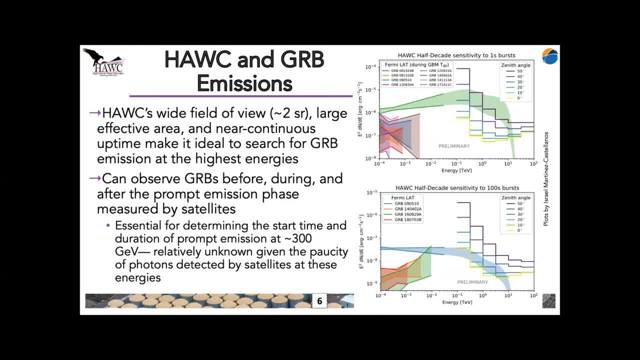 shorter than the saluting times of IACTs, Because we are a survey instrument, we do not need to point, We kind of just look up all of the time and there it is. Our effective area is also incredibly large and this is really advantageous for us. 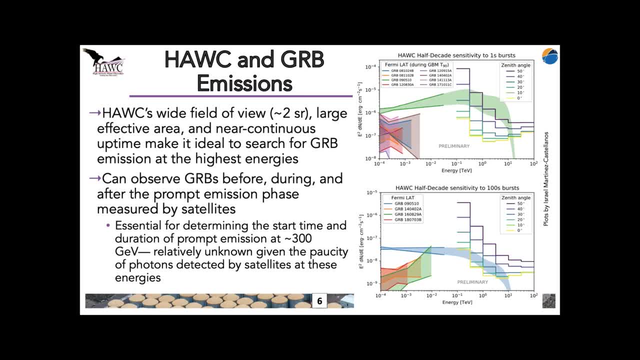 It's greater than 100 times the size of Fermi at energies greater than 100 GeV. Their limited size means that the satellites are not expected to provide useful statistics above tens of TeV, so this is where we can really shine. We can also observe GRBs before during. 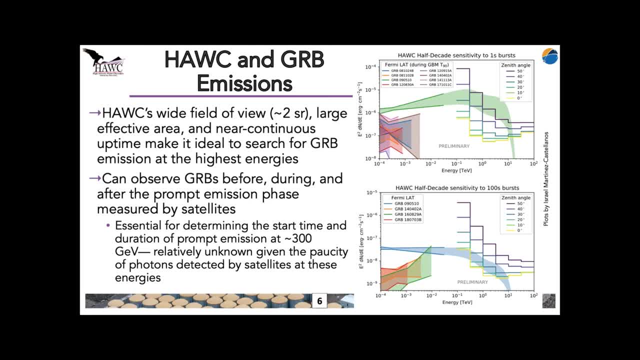 and after the prompt emission phase measured by satellites. So this is really critical for determining the start time and duration of prompt emission around 300 GeV. This is relatively unknown because the satellites don't detect a significant number of photons at these energies. so HAWC can really swoop in. 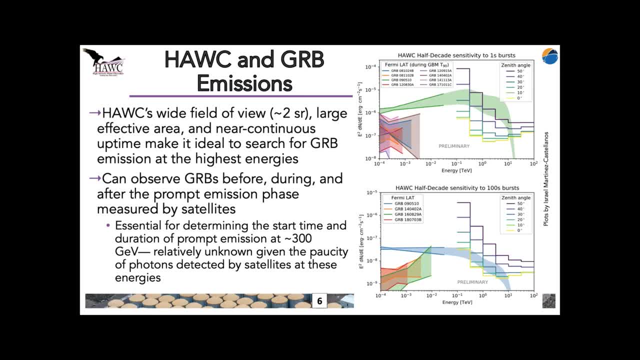 and provide information here that other detectors aren't giving. And you can see here from our sensitivity to both short and long GRBs that while HAWC is more sensitive to the long GRBs, we're really the only player in the game for survey instrument for short GRBs. 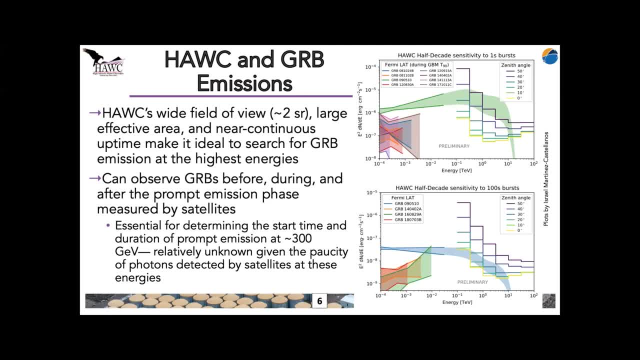 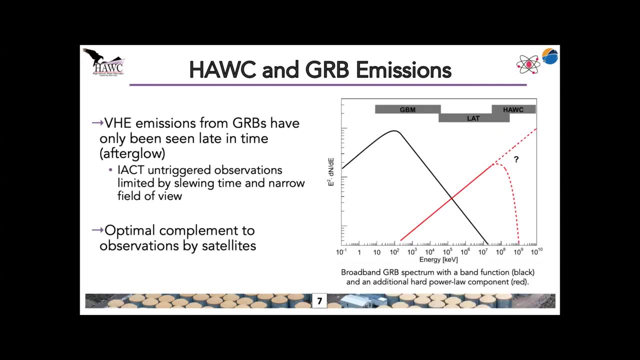 Because we have no slewing time and we have our very high energy range. So our detector is really poised as a double threat and both classes of GRBs should be prime observational and analytical targets for us. In terms of the VHE emissions, they have only so far been seen. 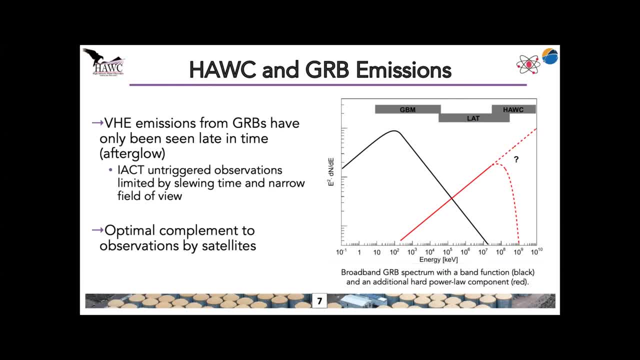 late in time in the afterglow, but this perhaps is due to the fact that the IACT untriggered observations are limited by their slewing time. This is definitely something to look into. It's unknown at this point, But really what HAWC does is: 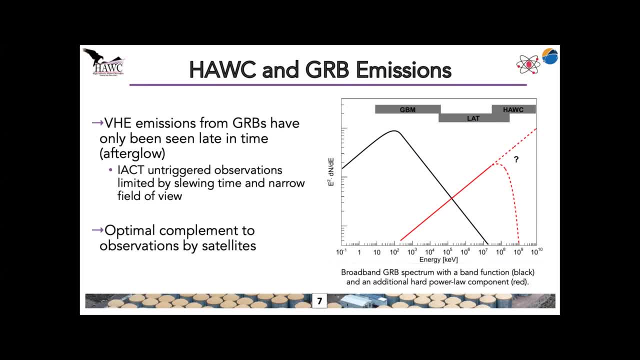 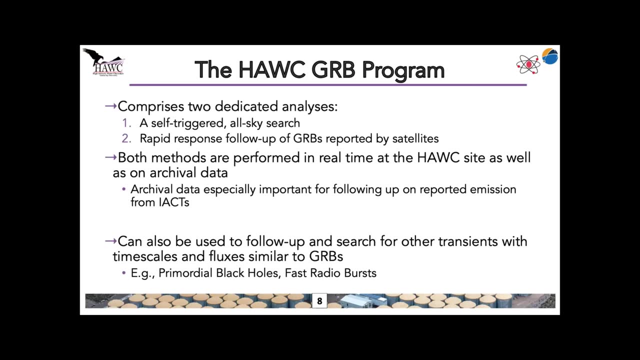 we provide an optimal complement to observations by satellites And also with our follow-up, we provide an optimal counterpart to the IACT's as well. So for our GRB program specifically, we have two dedicated analyses. We have a self-triggered all-sky search. 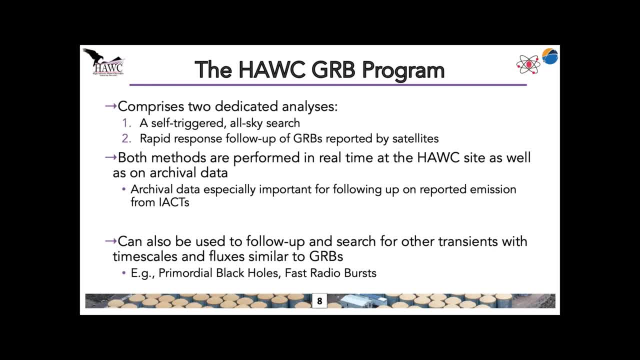 and a rapid response follow-up of GRBs reported by satellites, And both of these methods are performed both in real time at the HAWC site. so this is the four-second delay that I was talking about earlier, as well as on archival data. 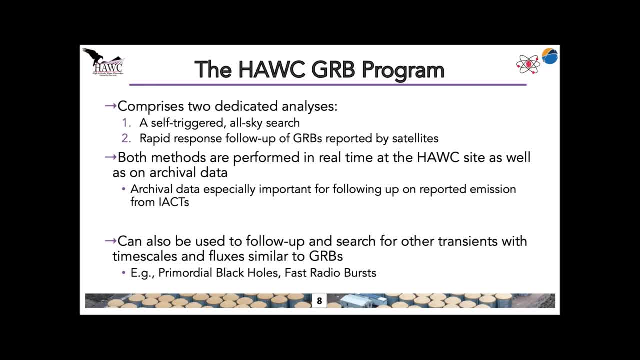 And performing these on archival data really gives us access to improved calibration and reconstruction algorithms. And then the archival data is really important for following up on reported emission from IACTs because we trigger on for the follow-up we trigger on satellite data. 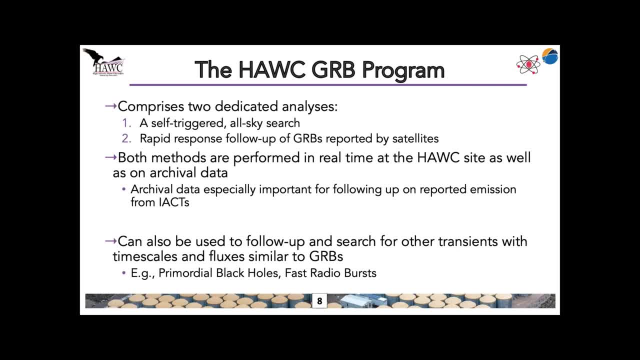 And this isn't just one-size-fits-GRBs. We use this follow-up and search for other transients with time scales and fluxes similar to GRBs, So we've already used this for primordial black holes and gravitational wave follow-ups. 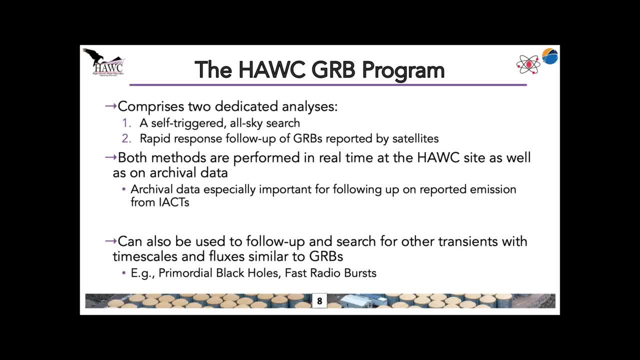 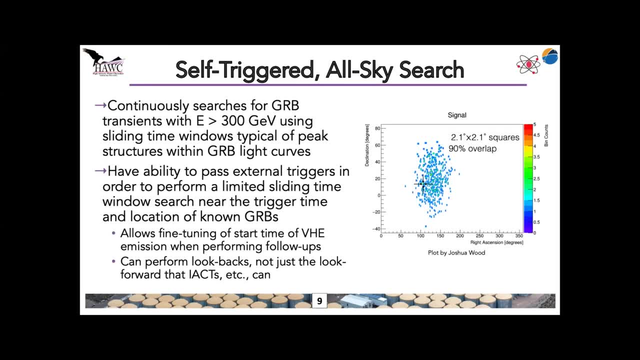 as well as in-process analyses for following up for very high emissions, for fast radio bursts, For the self-triggered all-sky search. what we do in real time is we continuously search for GRB transients above 300 GeV. We use sliding time windows. 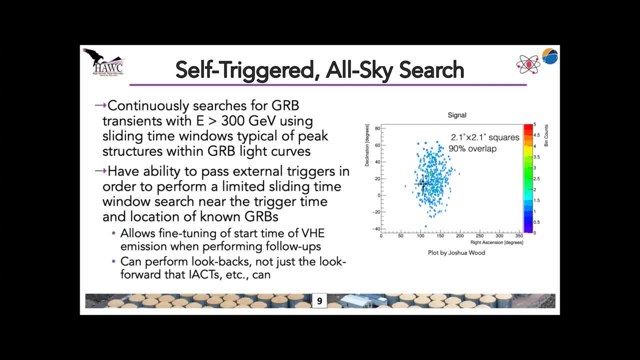 with typical sizes that correspond to typical peak structures within GRB light curves. So this is 0.2,, 1,, 10, and 100 seconds And we slide these windows in time and space by only 10% of their size per step. 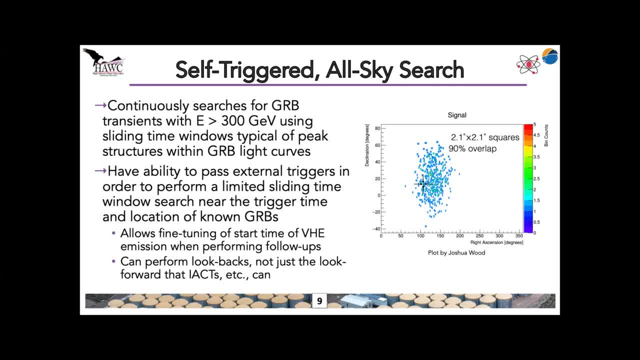 So this creates 90% overlap. So we are sure we are getting all of it And we make sure that we really work out- if it wasn't in the middle of our field of view or in the middle of that particular pixel- how to deal with that. 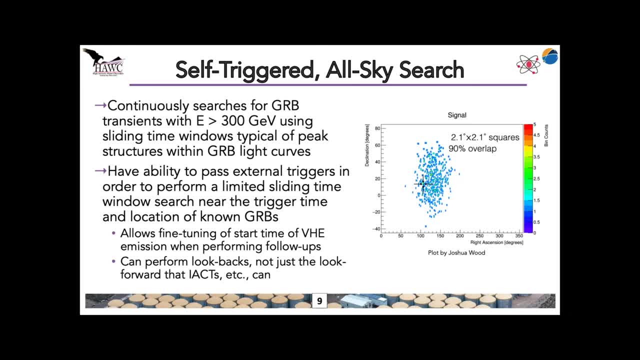 We can also pass external triggers in order to perform limited sliding time windows. So instead of searching the entire sky, we can say: just look in this one specific region, And this could be near the trigger time and location of known GRBs or not. 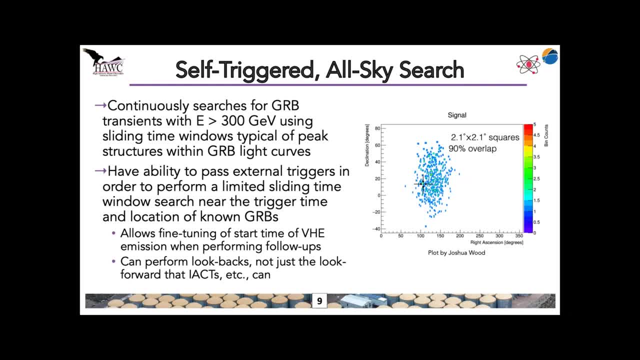 depending on the goal, And this really allows fine-tuning of the start time of VHD emission. when looking for follow-ups, And because we can perform this on archival data, this allows us to perform look-backs, not just the look-forwards that IACTs can. 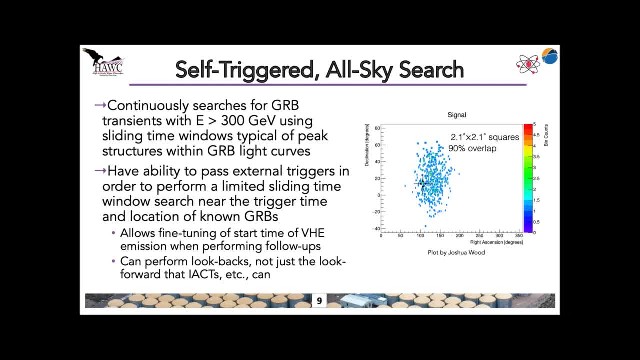 because, theoretically, we've already been looking at this part of the sky, and have been for some time now, And so we already have the data. It's there. We can go back and look at it. This program produces P-value statistics for each searched point. 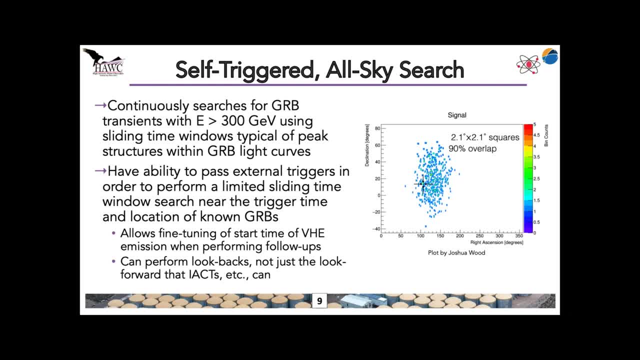 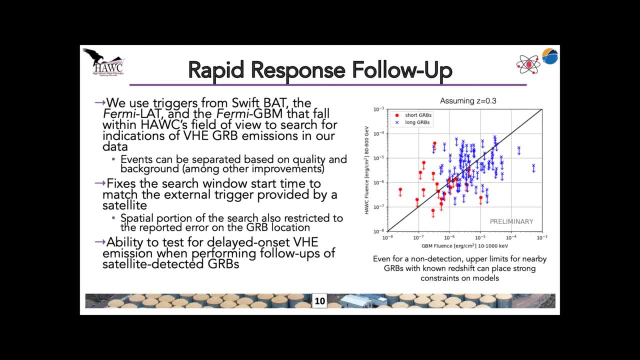 whether it's continuous or externally triggered, And we compare this to an expected, well-modeled background And we can go back and look at it and we can use the data to get those values. So, in contrast, for the rapid response follow-up, 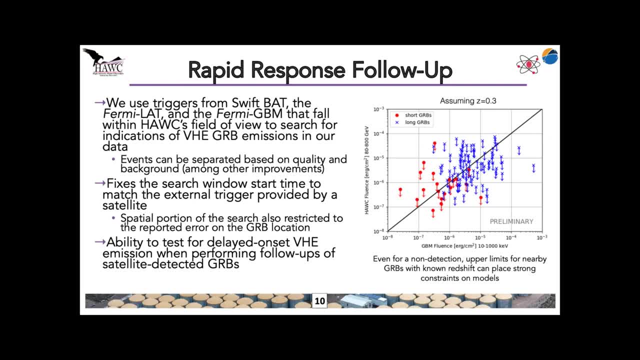 we use triggers from SWIFT, BAT Fermilab and the Fermi GBM that fall within Hawke's field of view to search for any indications of VHD gamma-ray burst emission in our data, either in real time or in archival. again, 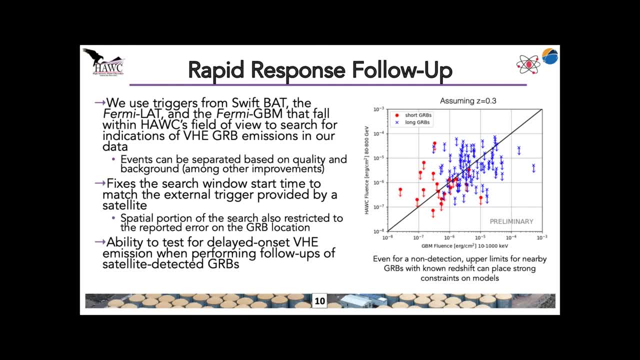 So for real time the follow-up of GCN notices for triggered searches is about 30 minutes. So we're looking at the start of the emission and a little bit before because we can search that archival data. So we fix the search window start time. 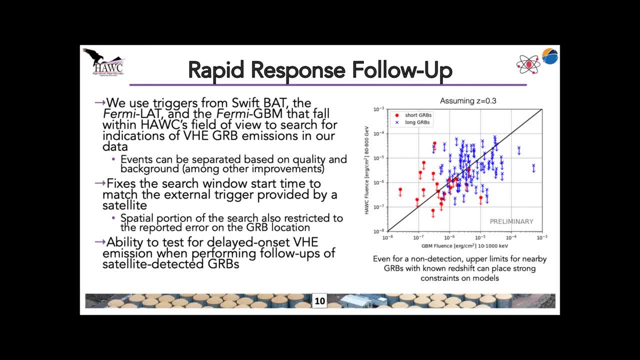 to match the external trigger provided by the satellite. And then we also restrict the spatial portion to the reported error on the known GRB location. So we don't really kill ourselves with trials or take too long to perform this test. And then we have the ability to test. 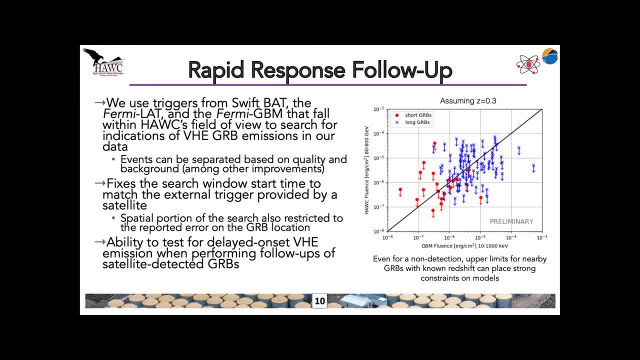 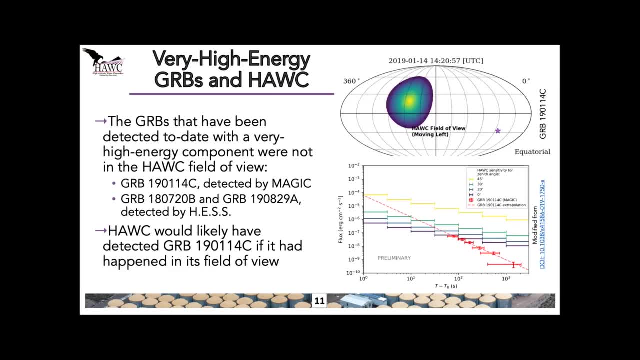 for delayed onset VHD emission when performing these follow-ups as well, because we can just continue to take data on that spot or look for it in archival data. So for the not so great news, despite how ideal Hawke is for the observation of VHD emissions of gamma-ray bursts. 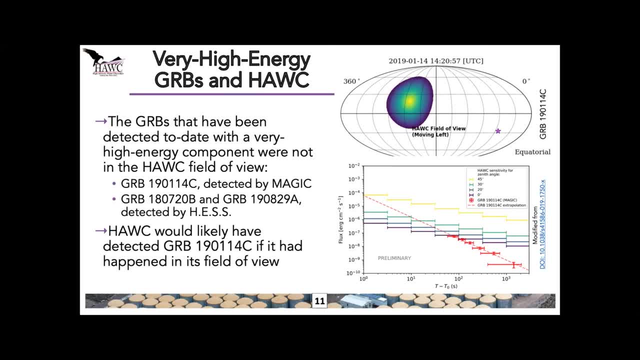 we have not yet seen one. We are obviously not the particular favorites of RNGsus, because the GRBs that have been detected to date- well, since Hawke has been turned fully on, so since 2015,- were not in the Hawke field of view. 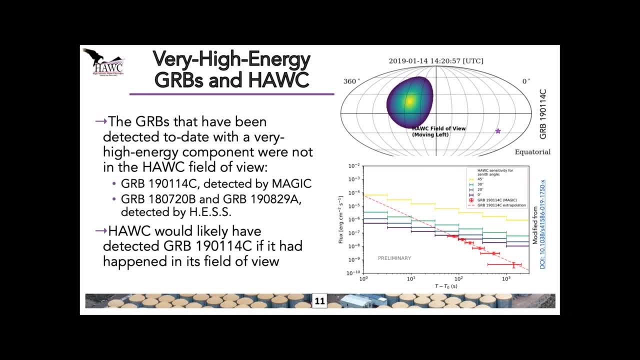 So this includes GRB 1901-14 Charlie, and then 1807-20 Bravo and 1908-29 Alpha, all of which we might have expected to see some sort of significant signal within Hawke. They were not in our field of view. 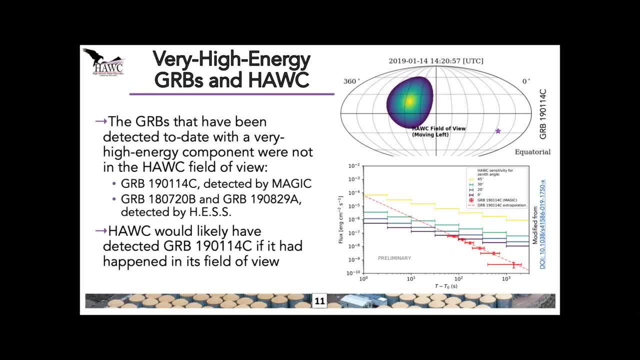 However, overlaying the Hawke sensitivity even at some pretty extended zenith angles on the flux time of the 1901-14 Charlie from MAGIC, we expect that Hawke likely would have detected if it had been in our field of view And if Hawke were to trigger on a GRB. 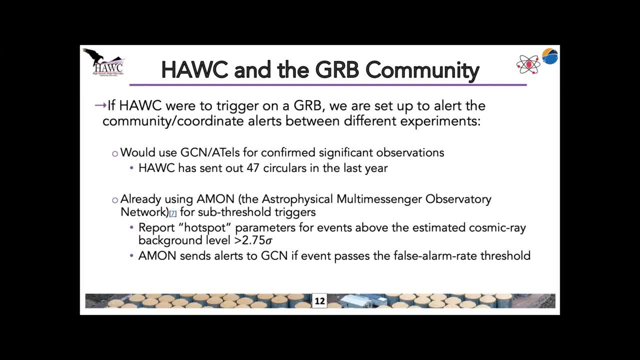 we're set up to alert the community and then coordinate alerts between different experiments fully. We would use the GCN network, obviously, and ATALS for confirmed significant observations. Hawke has already sent 47 circulars in the past year and this would be to promptly notify the community. 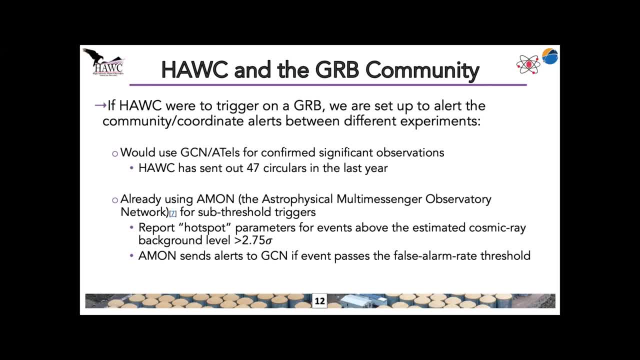 And we've already been using AMOM, which is the Astrophysical Multimessenger Observatory Network, developed in collaboration with IceCube, for subthreshold triggers, And so this has a bit of a delay. but what it does is it reports hotspot parameters for any events above an estimated background. 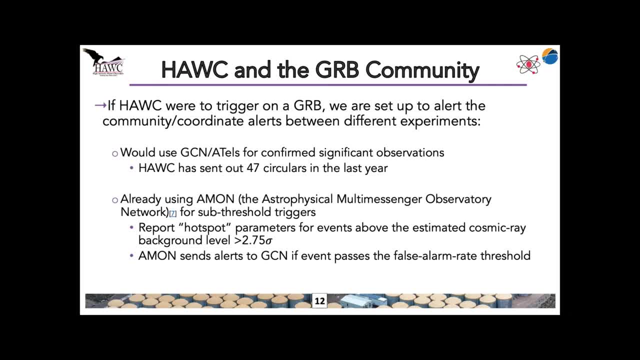 around 2.75 sigma or so, And then AMOM processes these and sends alerts to the GCN if it passes a false alarm rate threshold, which is determined to be about one event per year. So we pass all of our subthreshold triggers to AMOM anyway. 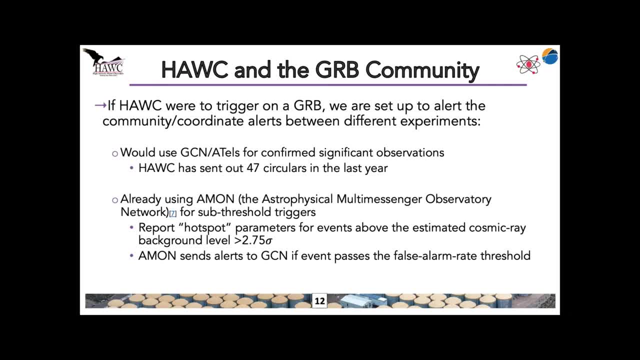 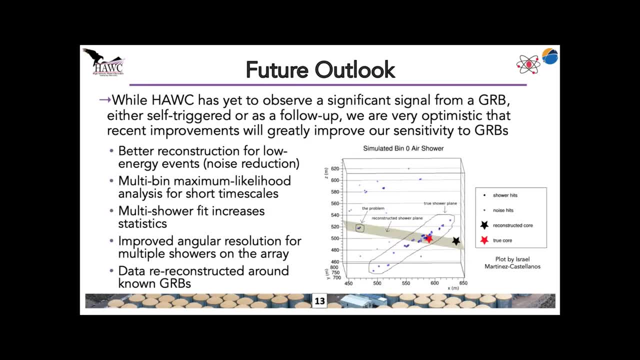 just in case, to make sure that we are really informing the community of everything that we know. So, despite the fact that we haven't seen one either in self-triggered or as a follow-up, we are really optimistic that recent improvements will greatly improve our sensitivity to GRBs. 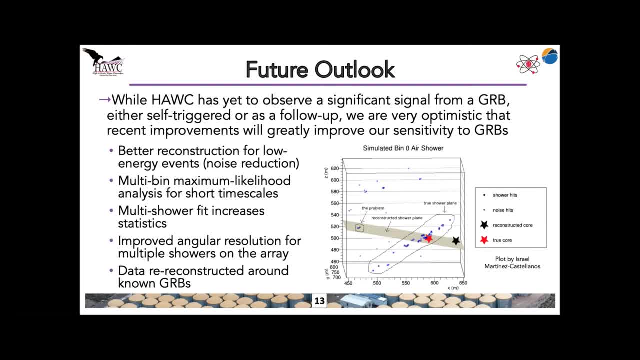 and that at the next one of these, perhaps, or maybe even sooner, we will be reporting on a detection of a GRB from Hawke. We have a project that we're working on right now that's looking at upcoming better reconstruction for low energy events. 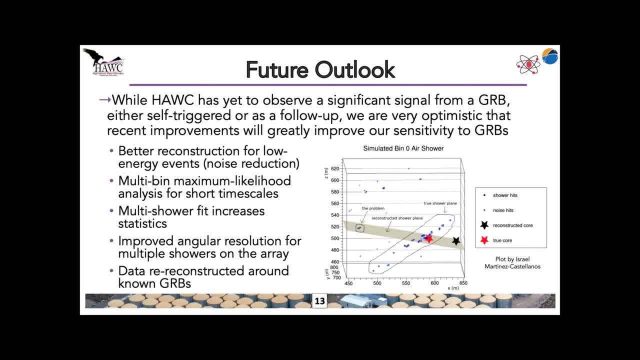 So this really reduces the noise in our signal. We have multi-bin maximum likelihood analysis improves our ability for short time scales. So before I showed that we are better for long GRBs, but we're really improving our ability to look for short GRBs as well here. 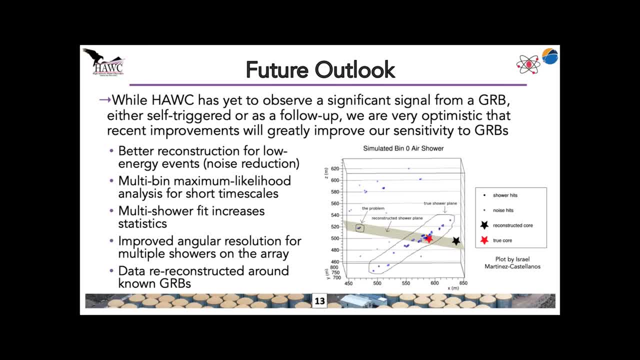 And our multi-shower fit really increases our statistics. We've also improved some corrections to our shower planes so that our reconstructed core can be more accurate. We have improved angular resolutions when multiple showers occur on the array, so we aren't quite as limited. 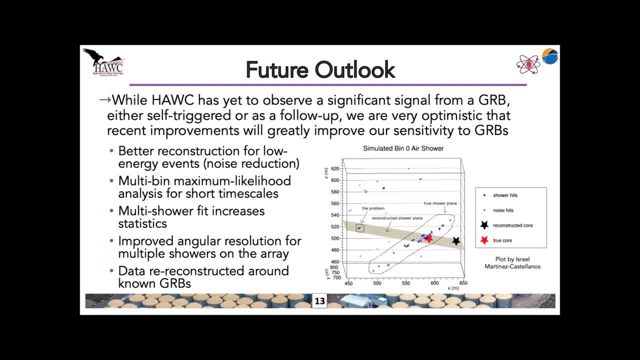 to search for only single showers. And then we have data that has been re-reconstructed around known GRBs. So we have ongoing analyses utilizing these upgrades, including both a targeted revisiting of known GRBs in reconstructed archival data as well as updates to the blind search. 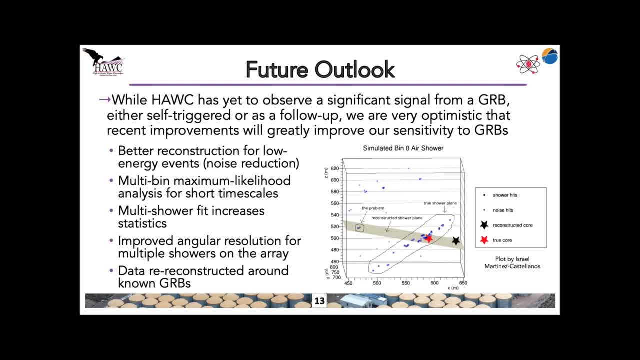 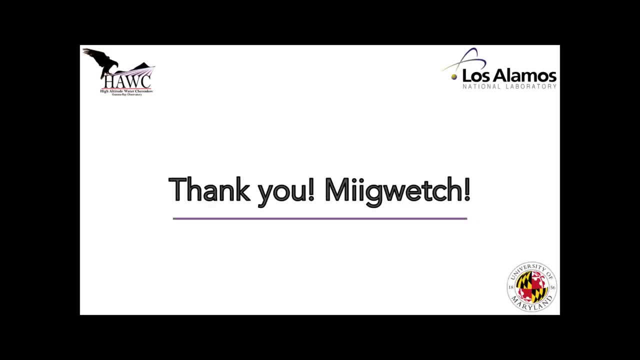 to make full use of these improvements. We expect that the full data set with these improvements will be ready in the upcoming months and hopefully these results will be coming out to you soon. And thank you so much, Miigwech. This should put us a little back on time. 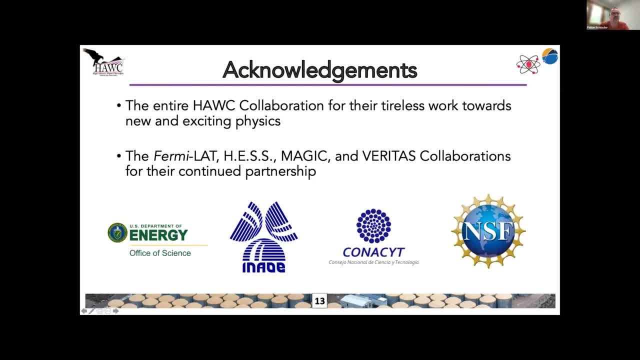 Thanks a lot, Yeah, and I guess everybody's looking forward to these forthcoming results. hopefully Other questions. I might have missed it myself. You mentioned the archival searches, but what timescales are you using for these? Are these similar timescales to the online searches? 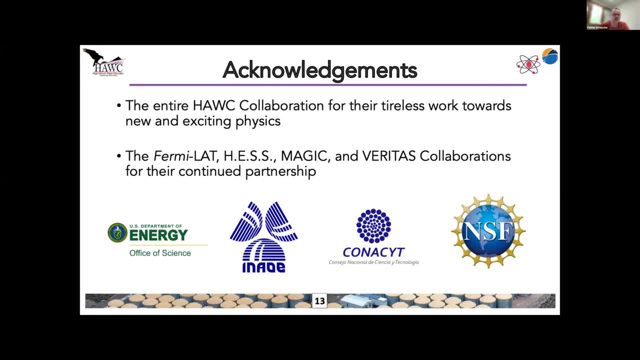 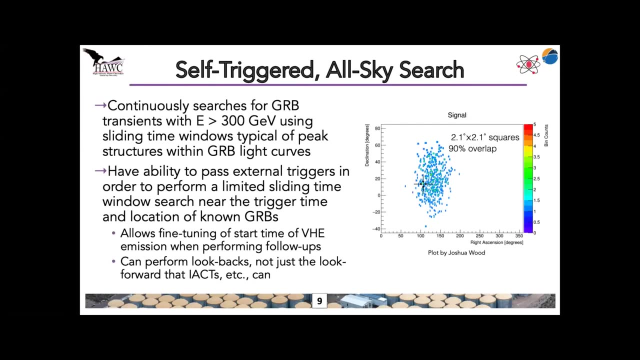 like going for the prompt emission or also integrating full transits to go for the afterglow emission. So both. One of the benefits of the self-triggered search- so when we can go back and perform on archival data- is that we can really fine-tune the start time. 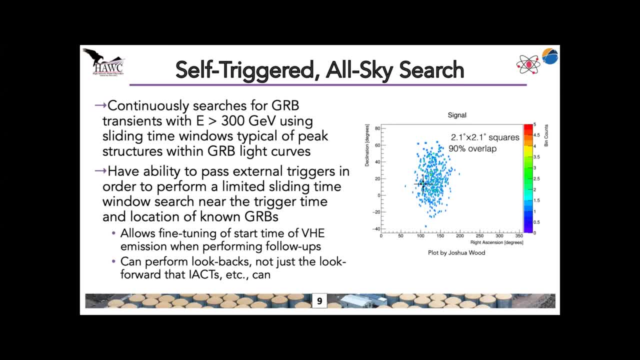 And so between the search and the search we use actually different time windows so we can look for that afterglow emission as well as just the different peak emission timescales. So we've been working on implementing longer timescales within this as well. 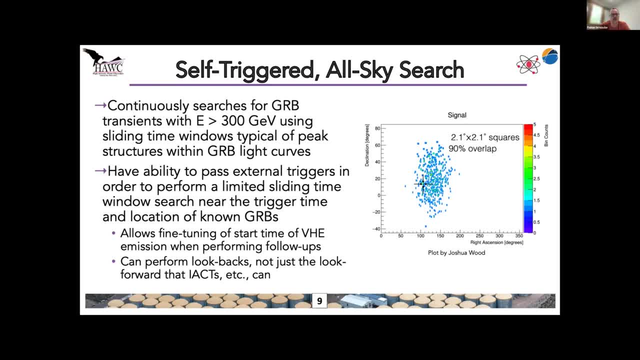 Because from the, as we discussed earlier, the deep afterglow observations by the IACTs probably hint to a chance to get a chance to get HAWK detection if you integrate over longer timescales. Yes, and we have been working on optimizing. 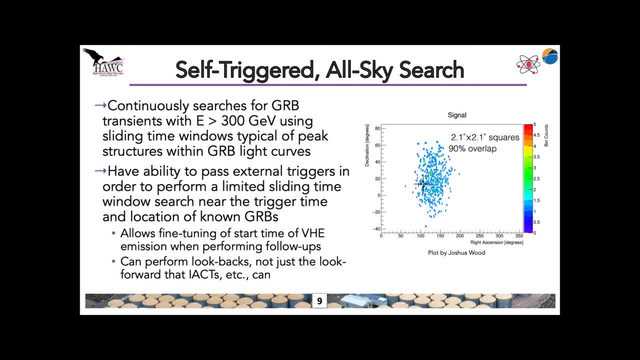 one of our analyses for such afterglow emissions. Perfect Franz, you have a question? Yes, I have one. Thanks, Christy for the nice talk. And they say sometimes HAWK delivered some burst GCN or notices. 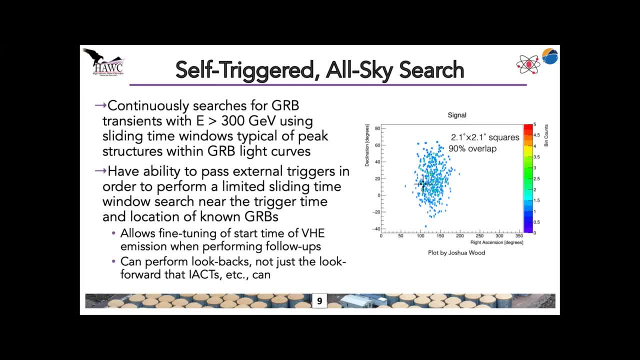 So how they are created right now. So are there school use events or can you comment on them? How we create GCN notices? So which are the because none of them were confirmed as GRBs so far We have not. I just meant. 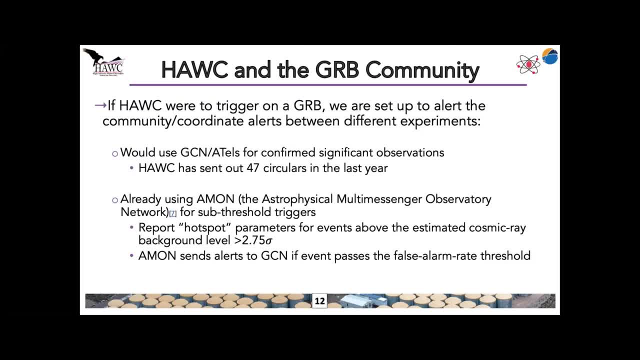 we've sent out 47 GCNs about anything We but because our system is set up for automatic GCN circulation for any significant observations, if we were to confirm a GCN, a GRB at very high energy with a significant signal. 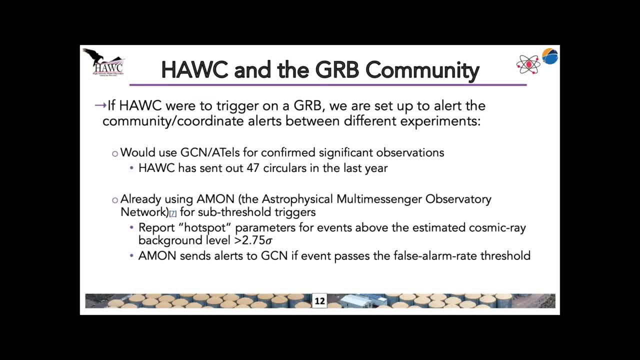 we would be. we're already set up to inform the community promptly about it. Now I was asking whether you are going to do somehow a comprehensive analysis of these alerts. try to understand what they were caused by. Oh, my apologies. Yes, I believe that is the plan. 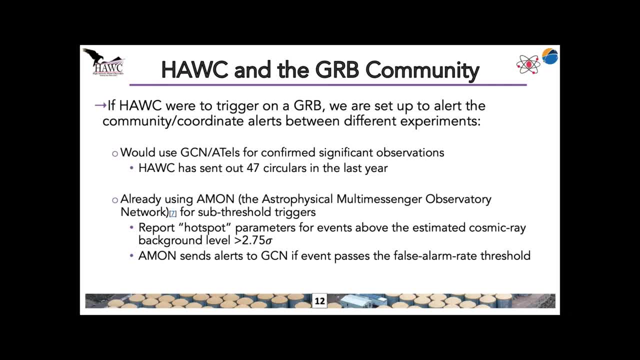 To go back in. you're asking about going back through the ones that we've received alerts for and really trying to figure out what caused their high energy emission. Yes, yes, indeed, Yes, yes, We planned one of the analyses. 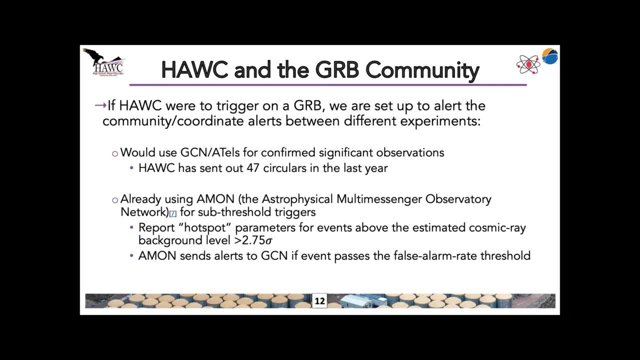 and this is also the one for that we're trying to implement longer time scales for- would really try to throw several different models at each of these follow-ups on archival data and try to place constraints on what caused them and what caused that very high energy emission. 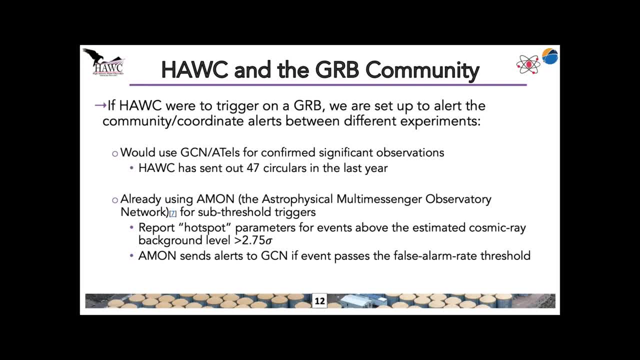 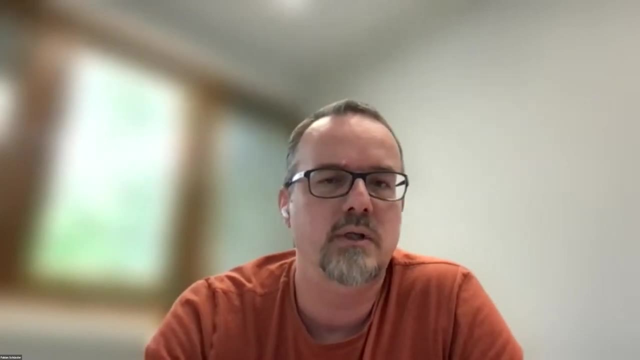 Based off of our results and, hopefully, our observation of them. Okay, thanks. Are there other questions? I don't see any. Okay, thanks, Christine. Then let's move to Jagdish, who has the job of trying to tie all this together. 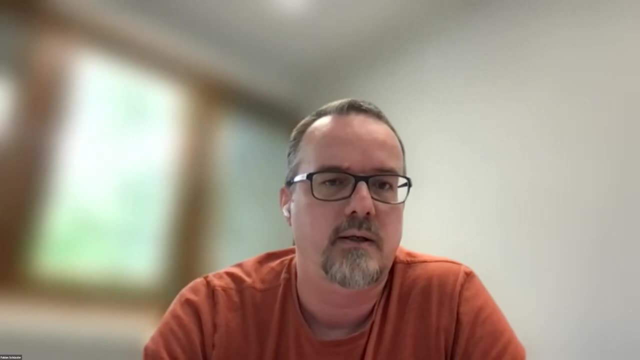 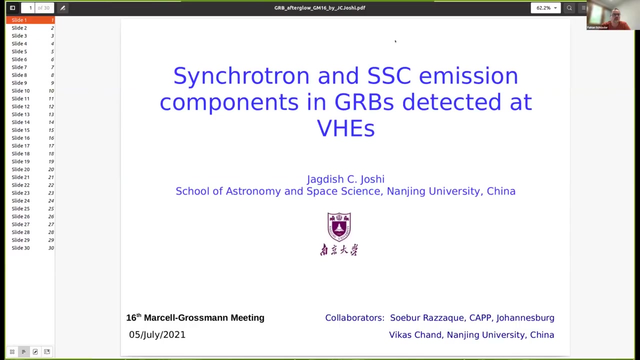 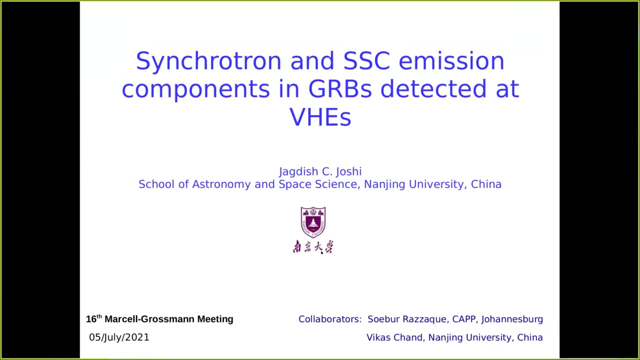 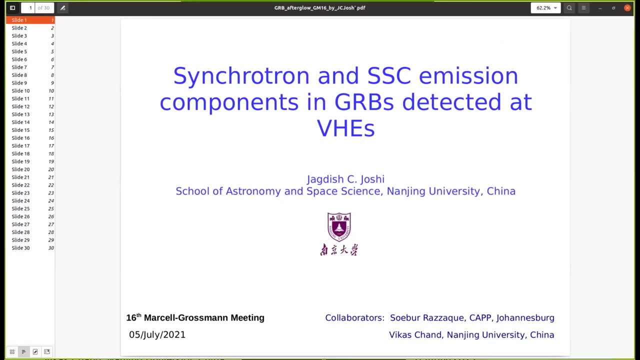 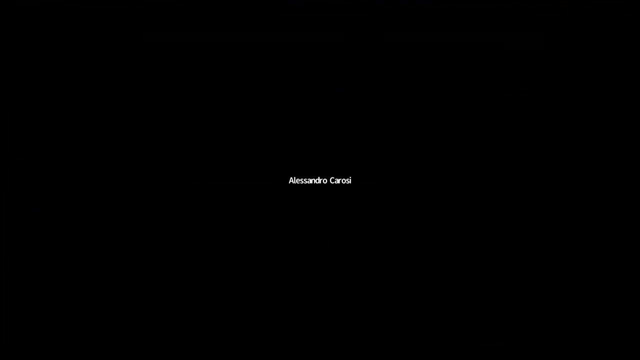 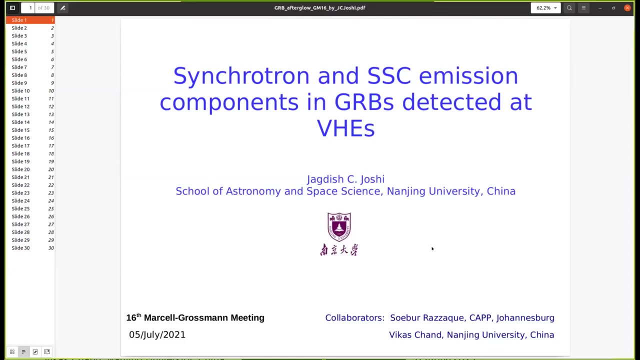 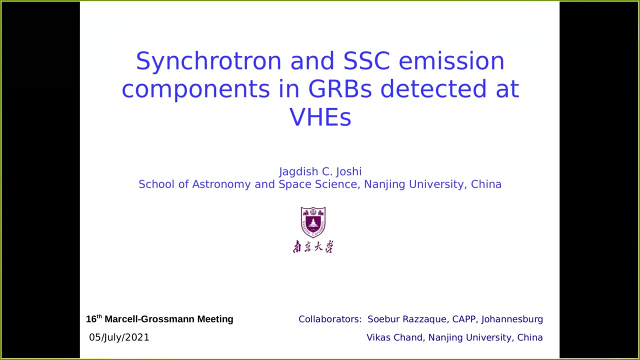 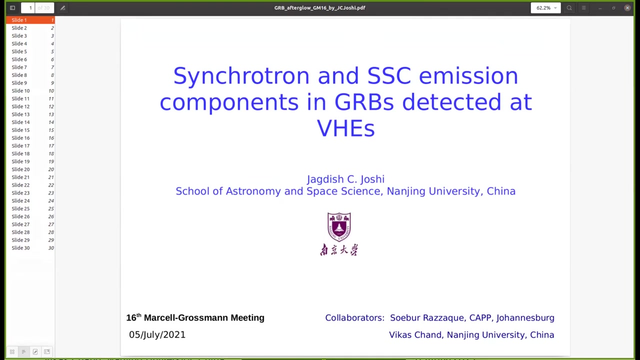 in a theoretical framework. We can't see your screen anymore. Okay, we see your screen, But for the moment we don't hear you. Your mic seems to be on, but we can't hear you, And we see your screen. 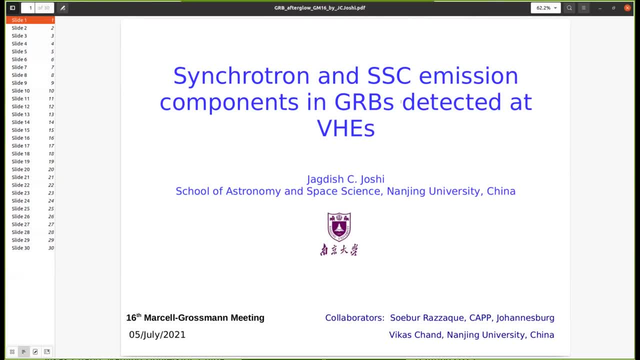 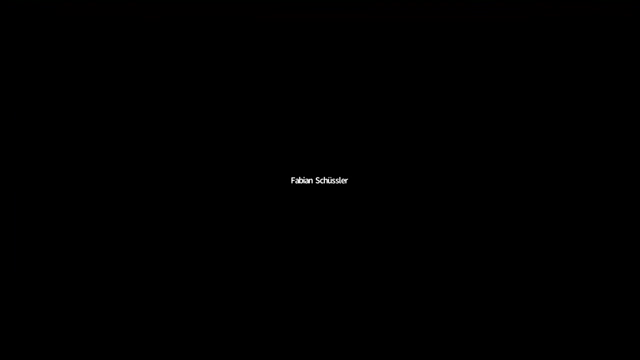 Okay, we see your screen, That's fine, but we have no sound. That's fine, but we have no sound. Maybe you have to reconnect. I don't know if you have another idea what you can try. Otherwise, we could probably change the order of the last two talks. 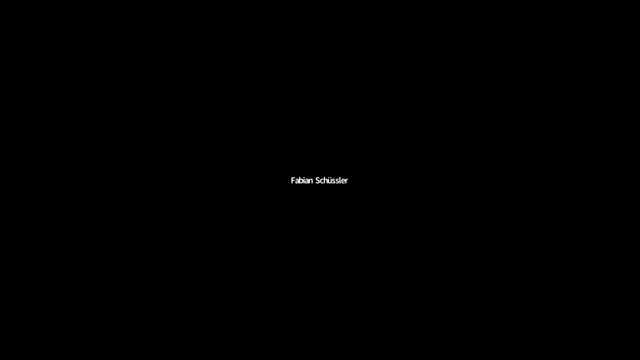 If, Monica, are you ready You could jump in and then we Can. we come back to the active later on. Yeah, yeah, yeah, Okay, Okay, Hi, Then please go ahead. Perfect, So let me share my screen. 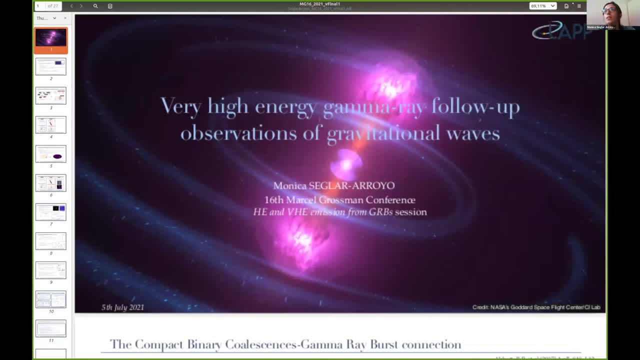 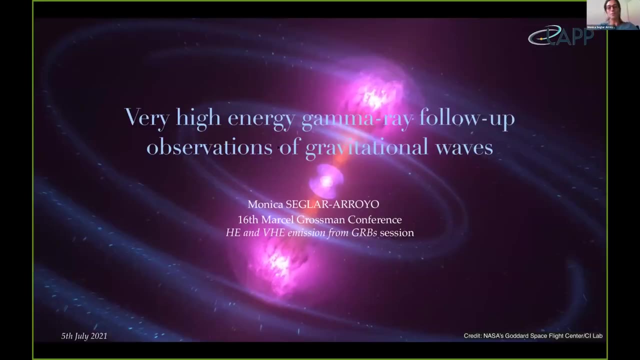 Okay, Sorry, Tag, always a problem, I don't see the continuous No. Okay, so if you hear me well and you see me well too. so now I will slightly switch topic, because now I'm going to give an overview of what has been done during the last observing rounds of LIGO-Virgo in the terms of follow up of very high energy gamma ray emission. 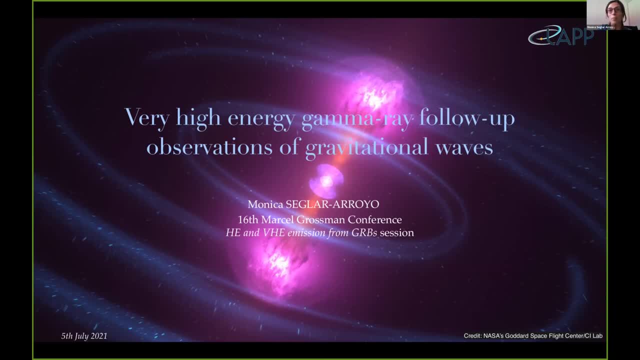 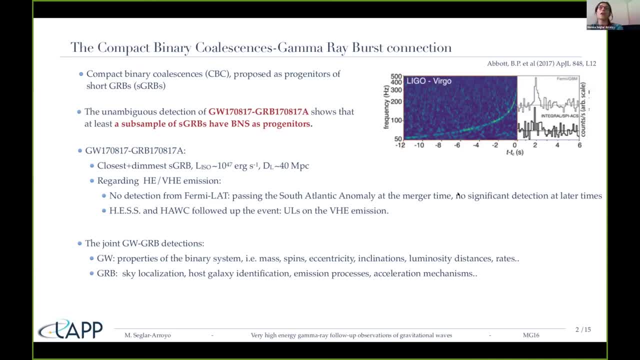 So just let me know. So, okay, We are interested in these connection because, while, as you may know, of course, compact binary coalescence, and particularly the ones, including neutron stars, so which are starting to start a black hole, 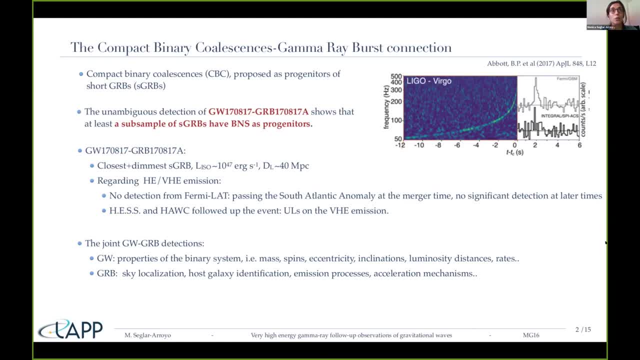 They have been proposed as the project of short GVs. So there was, there was an ambiguously program for at least a subsample of short GRVs in the case of gravitational waves in DnCO817, where here we see the inspiral phase and then we see here the Fermi GBM and 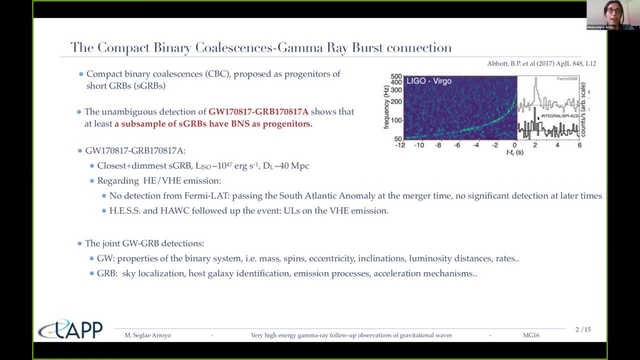 the integral detection of GRV DnCO817a. So some interesting things about this event is that this is the closest short GRV and the dimmest observed. so it was really close, at 40 megaparsecs, and really dim, so 10 to the 47 hertz per second. Regarding what I was observing: high energy and 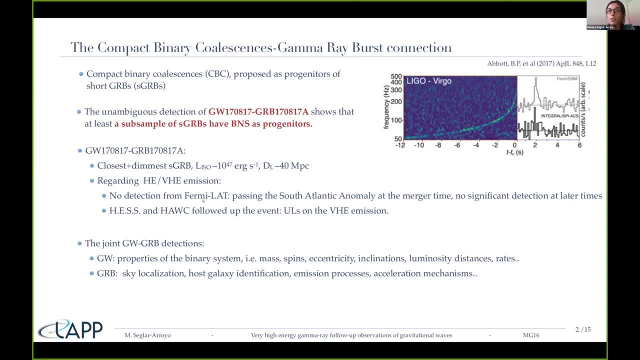 very high energy Fermilab was unfortunately passing the South Atlantic anomaly at the mature time and then there was not this significant detection at later times And regarding Hess and Hawke, no significant detection was observed. So we are basically interested in this because you guys have discussed all the GRV. 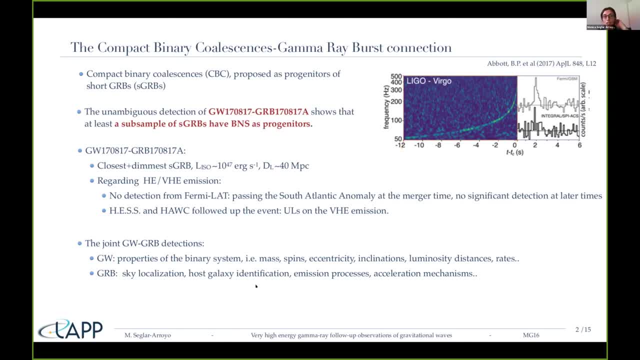 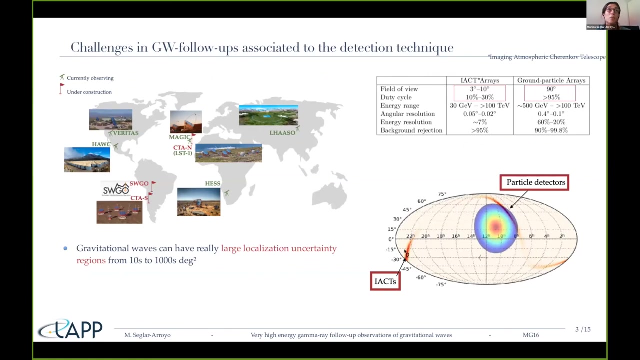 nice results that one can get. but then it's really interesting to connect it to the properties of the binary system, so the mass, the spins, inclination and luminosity and of course the rate for this type of event. So now the challenges. I'm going to go into the challenges, which is the main problem with these. 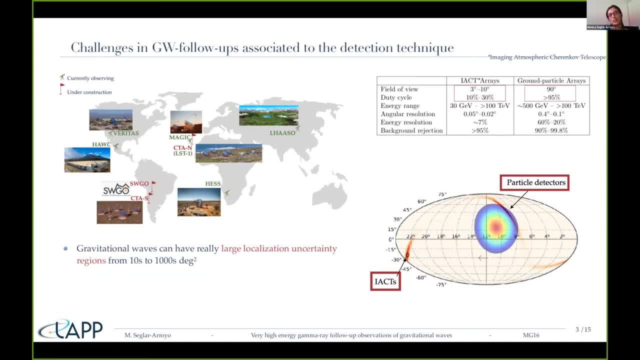 follow-ups, So no matter. I mean, basically it is challenging for all of the very high energy technique instruments. so here you see the particle detectors. so, as Christy introduced before, so you see which is the region in the sky that particle detectors have access to. and then this is for AGCT, that is. 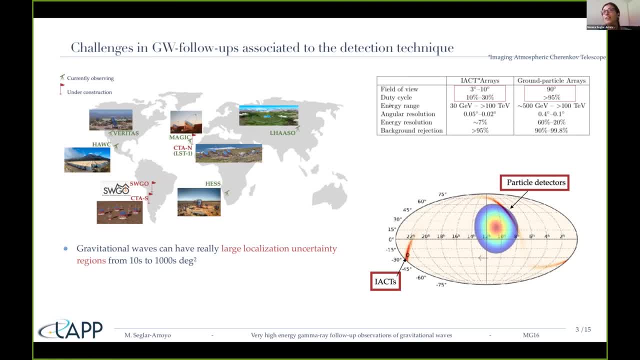 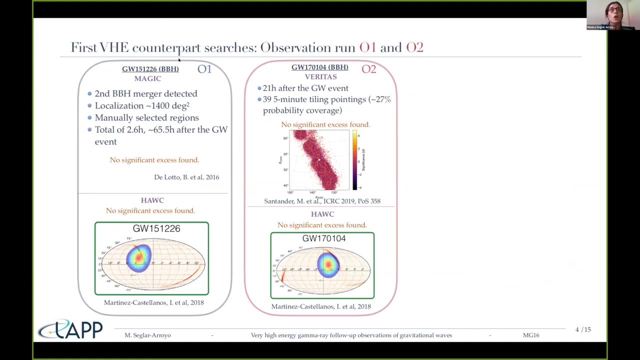 way smaller, of course, so it's important. the complementarity between these two types of detection techniques is really interesting, since we can have access to complementary results. So I will focus now on the first searches, So during 01 and 02, so first going to 01, so the first event that was followed up was this: 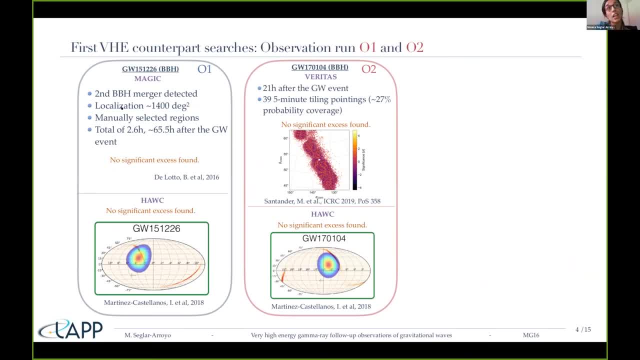 second binary black hole merger which showed a really large localization uncertainty due to basically having only the two LIGO detectors. so for this one, MAGIC did select some manually regions and, well, took about like 2.5, like 2.6 hours of data but no significant access was found. 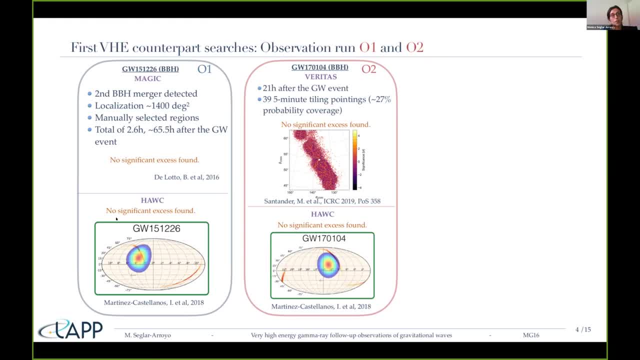 Same for these other events. well, these same events. no significant access was found for Hock, And then we moved directly to 02, so for 02, the first searches included VERITAS, with this 39 five minute styling pointings. no significant access found and with their observations they could cover 26 hours. 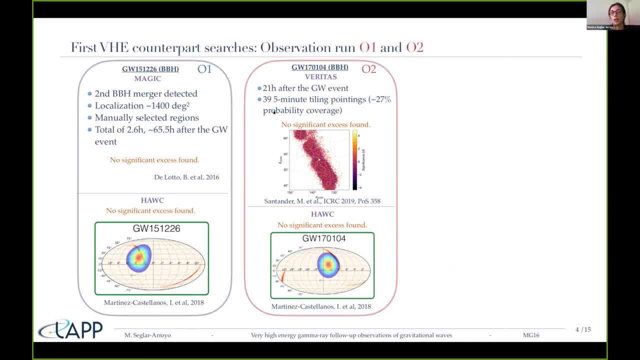 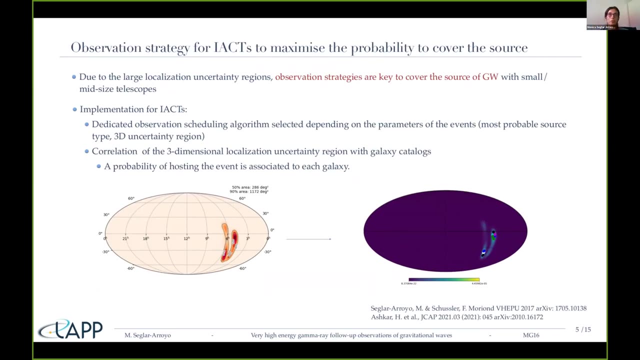 27% of the probability of a priority region. And then Hawk reported no significant results also on this one. And then- well, this is not only for ASTTs, but then for other small and mid-sized telescope. there's some serration strategies in place. 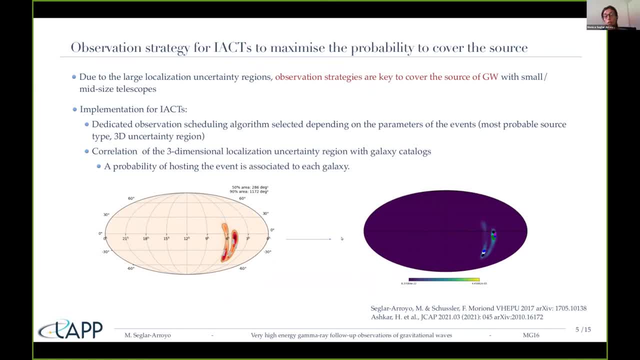 in order to cover larger regions in the sky. So there's been efforts to implement this strategy for ASTTs, as they have this small field of views. So one could have- and this is what Hess did- to have dedicated observation scheduling algorithms which take into account the parameters of the event. 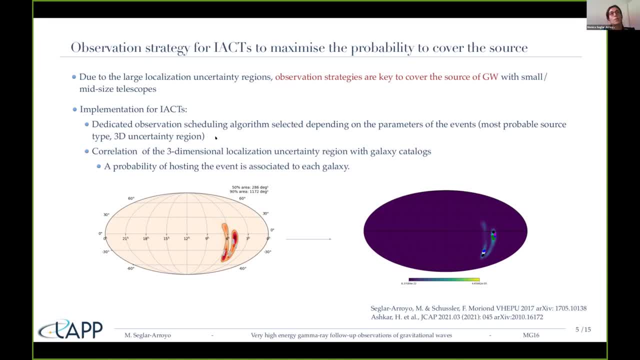 and also the 3D uncertainty region. And then one could correlate also that 3D uncertainty region with the Galaxy catalog. So in the end one ends up having a probability of hosting the event for each galaxy right. So in this way one can pass from this uncertainty region. 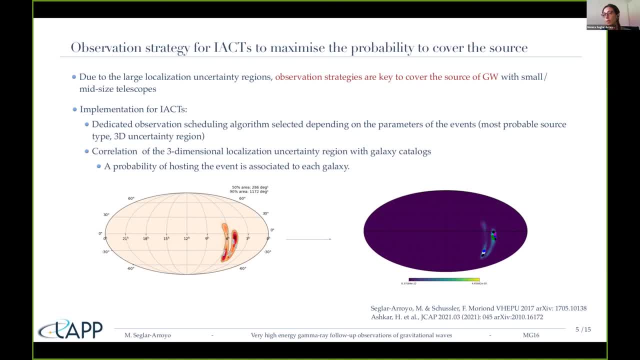 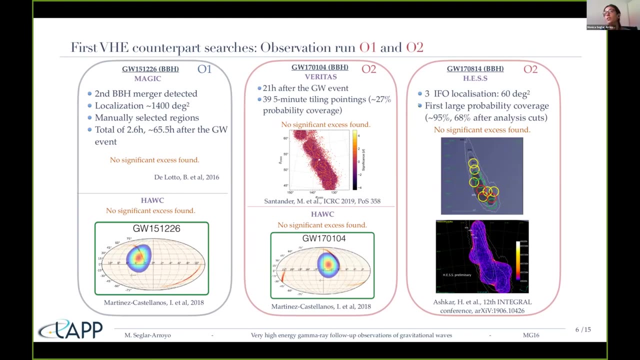 for the localization to this pointing, which will cover a large region in the sky. So this has been presenting in these two papers, first in 2017 and then 2021.. So thanks to these strategies, we've, like the first large probability coverage. 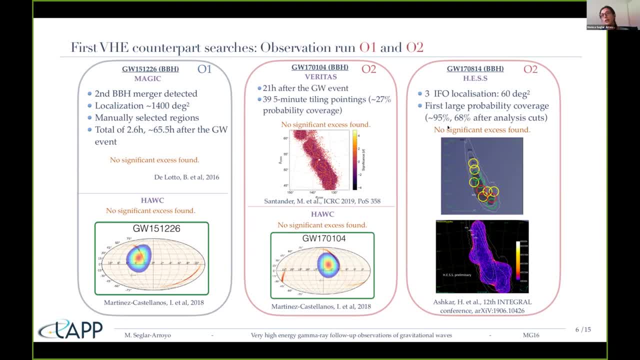 Here you can see the different pointings and different colors. And after analysis cuts there was a priority region of 68% covered. So here we see that there was no signal detected for this one, but it was a binary black hole. 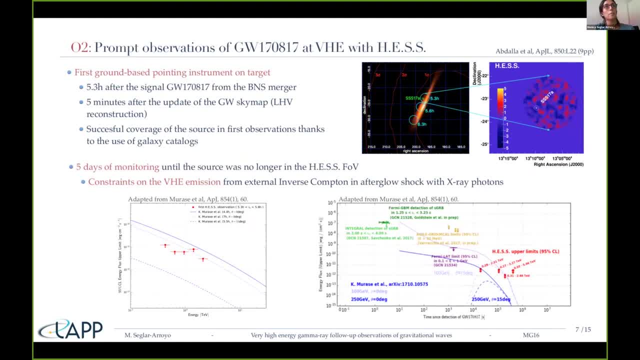 so it was somehow expected. And then going to the interesting, the interesting part, which is that it's very interesting for the followers of gravitational waves. So for this event, which is the first binary neutron star detection which is gravitational waves, since 2017.. 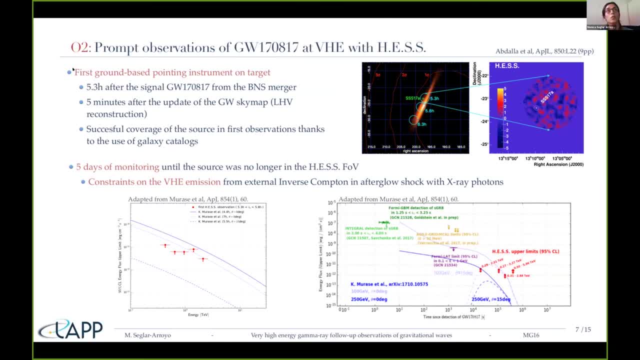 So HESS was the first ground-based pointing instrument on target, thanks to the uses of these strategies. So here you can see where the source was actually. So by the time HESS was, I think, about 10 years old. so by the time HESS pointed on this region. 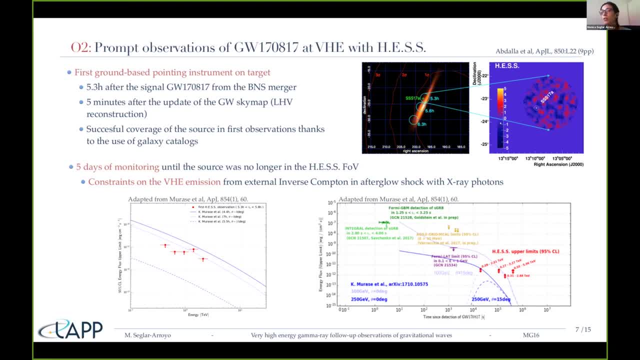 the location was not known. So this was the first pointing of this scan. You see that no signal has been detected for this one, but at least the observation strategy worked. HESS was covering this region five minutes after the gravitational waves sky map was sent. 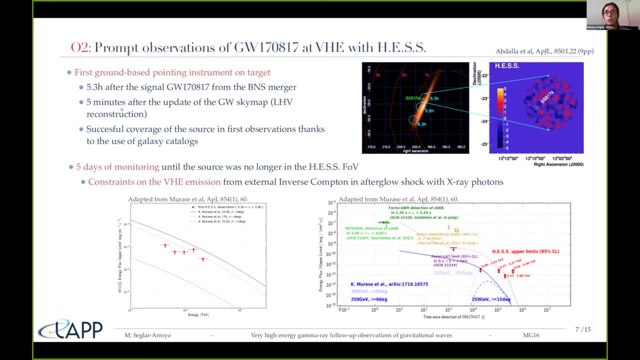 considering the three interferometer, the reconstruction. So after these three first pointings, during the first night the source was identified and HESS continued covering the source for five days. In this way, HESS put constraints on the very high energy emission. 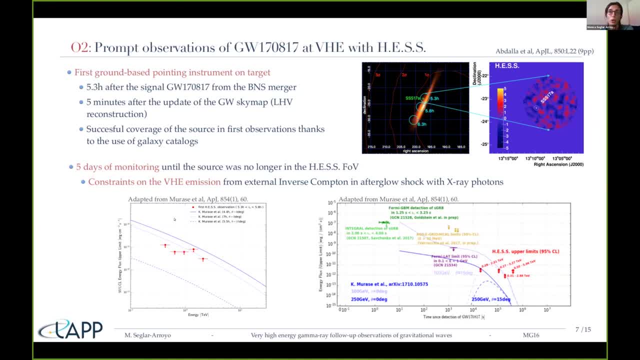 from an external inverse quantum in the afterglow shall we X-ray photon? So here you see the upper limits of HESS which constrain the satisfy energy emission of this type of pattern for 5.3 hours to the 5.8 hours after the merger. 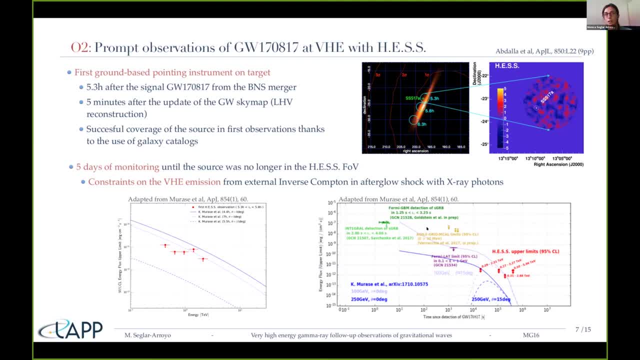 And you see how these can constrain the emission expected, expected for this with this model for zero degrees and then also for 15 degrees and different energies. So you see that it could have been constraining. So, in the case of having this super great scenario has would have detect the event, Now staying still. 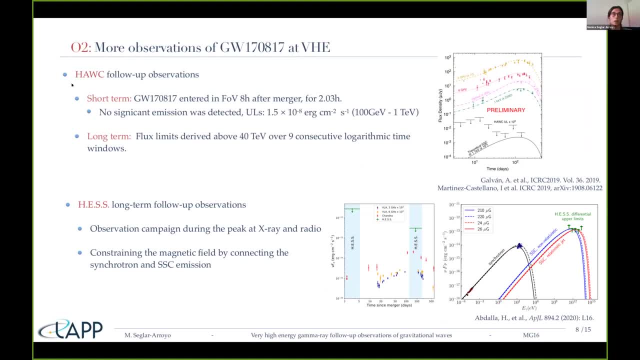 in gravitational wave 17 08 17.. Now I will. the other short term for what happened was by Hawk. This event entry in the field of view. a field of view eight hours after the merger and he stayed for two hours. So no significant detection was detected. but have 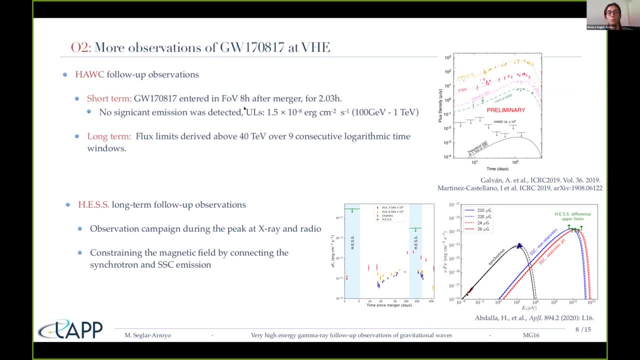 the upper limits for for the emission. And then not only there was a short term, but thanks to be how? capabilities, how could you a long term observation campaign? We're here, we see all the different logarithmic time windows and these put some limits on the 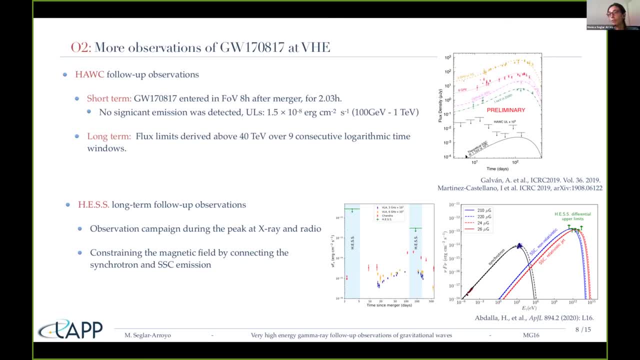 theoretical SSC at one TV that we that we can see here and that have been reported in ICRC 2019.. Now moving back to hers, but now in the long term, there was an observation campaign For the That here you see, for the peak at x rays and radio. So thanks to this campaign, there's 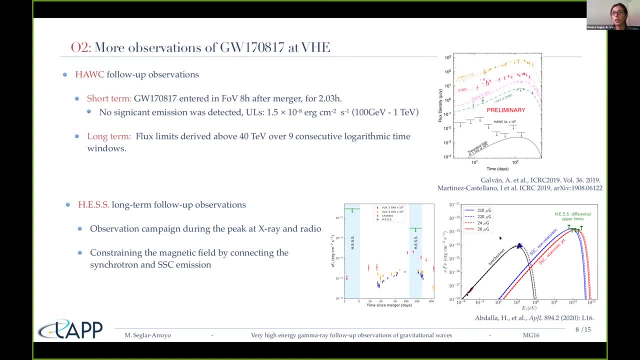 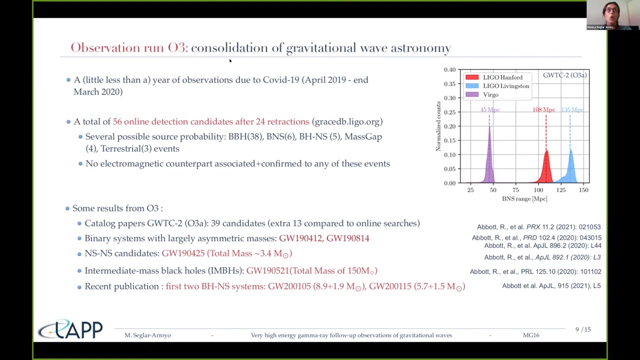 been some constraints on the magnetic field that have been derived by connecting the sequence on emission and and the SSC for different models taken into account: relativistic, jet, non relativistic, and different different magnetic fields. Okay, now, this was a very. this was all. this was for oh two, and now moving to O three also was really like the. 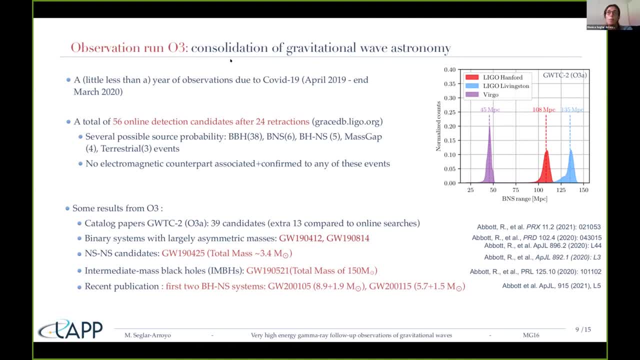 consolidation of the greatest way: astronomy. Here I report The binary neutron star range for the different interferometers of the network And- and this was this was a year around the lasted for for about a year, 11 months, due to COVID, but there was a total of 56 online detections that were not retracted. 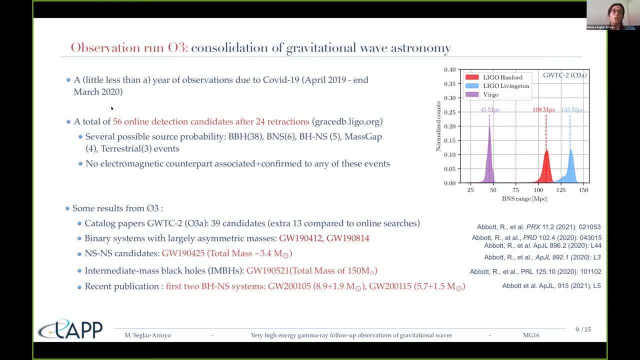 24 of them. they were So, out of these 56 detections, the largest probability associated to each event makes that we can say that 38% are most probably binary black holes, mergers, 6% bineutron star. then we have some black hole, neutron star and other types. 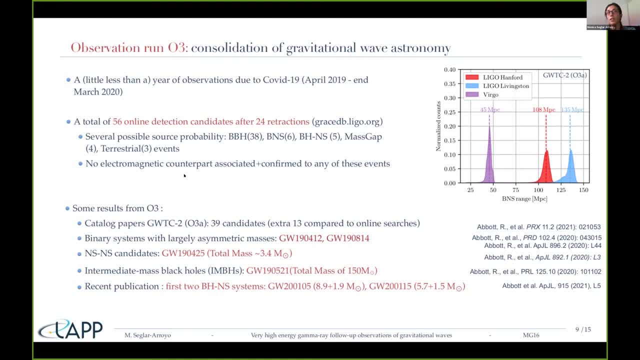 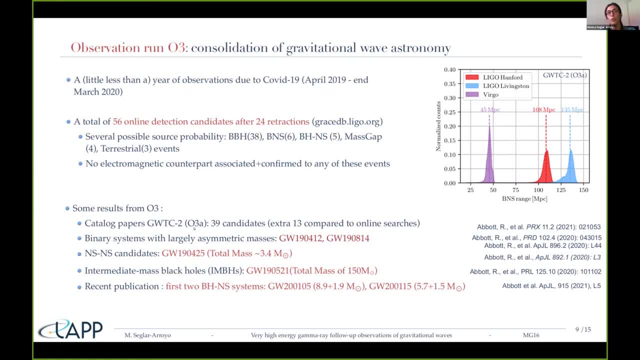 There's the O3A paper out, There's the O3A paper out, There's the O3A paper out, And soon there will be the transient catalog 3, 403B. Some of the results include binary systems with large asymmetric masses and neutron star. 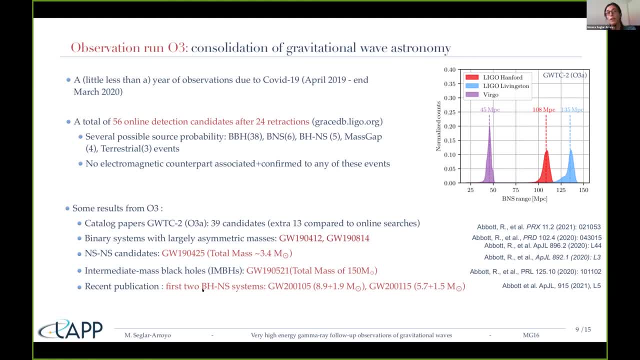 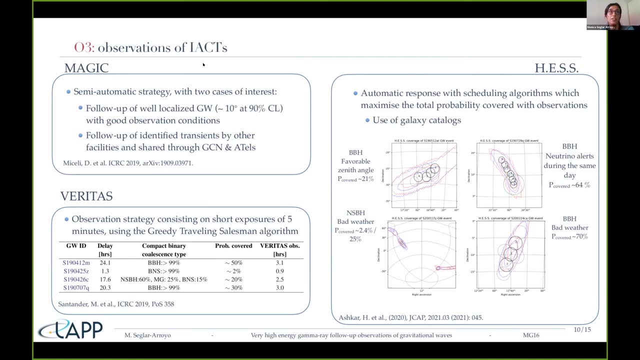 neutron star candidates Also. first, two binary black hole neutron star systems with the masses that I quoted here. that was presented last week. Now moving to the observations during O3 by the different IECTs. So you already gave the details on this, but just to see the picture for the three IECTs: 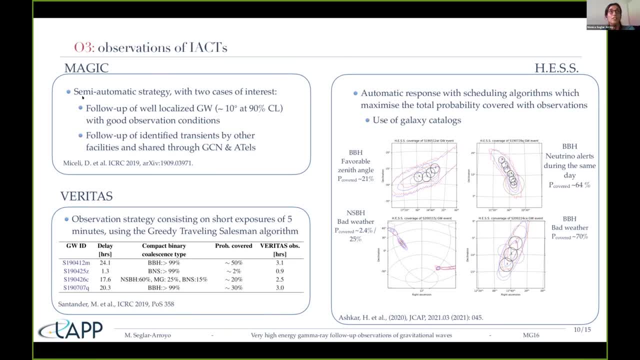 currently taking data. MAGIC has a semi-osmotic strategy with two cases of interest. One is well-localized gravitational waves and the other one is to follow up and identify transients which may come through GCN and ATOS. In the case of VERITAS, their strategy is to follow up and 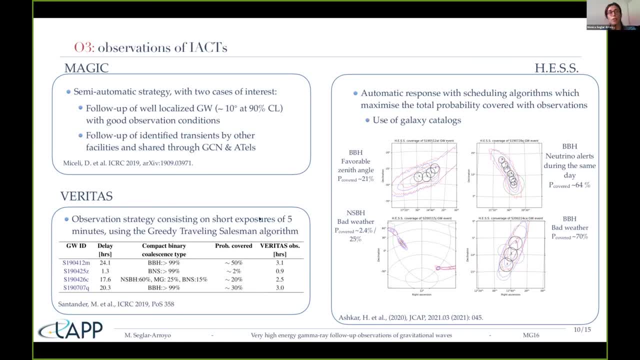 identify transients, which may come through GCN and ATOS. In the case of VERITAS, their strategy is to do a short exposure, so five minutes, using this greedy traveling salesman algorithm according to the ICRC 2019.. So in these proceedings there's different events that 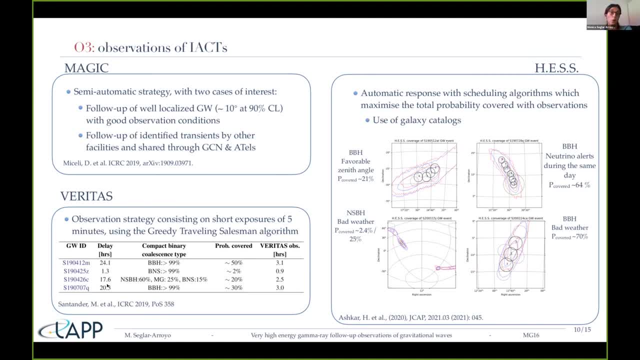 were followed up during the first, during O3A. We see here that there's this one where the probability of the binary neutron star was pretty high, was 99%. Nevertheless, they could only take a 2%. They could only cover 2% of the uncertainty region. Then, regarding HESS, they have this: 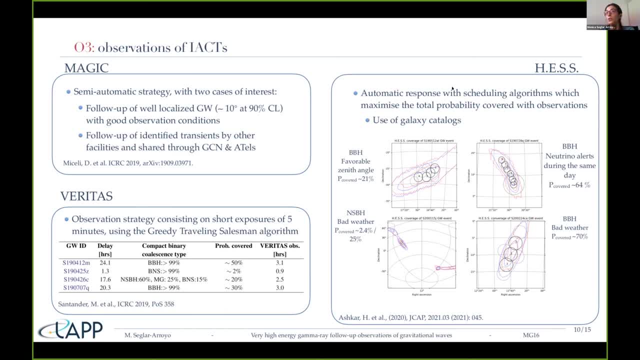 automatic response and they use scheduling algorithms in order to maximize the probability covered. And there's this use of galaxy catalogs included. So in this paper we summarize the different follow-up observations. these three are binary black hole mergers for which we have the largest probability coverage. 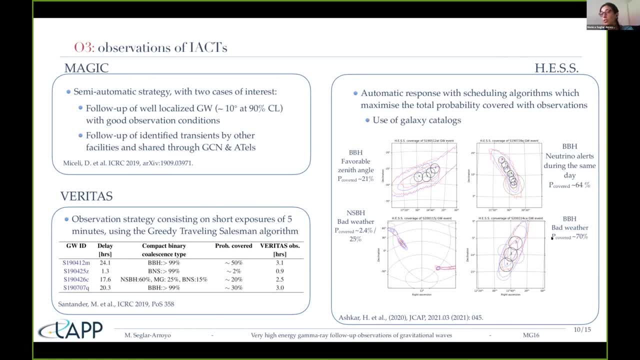 We see that in this case the probability was actually pretty high- was 70% of the uncertainty region. Then the only neutron star black hole merger that was observed is this one, which is the same that I mentioned before. Nevertheless, for this one there was bad weather, So only a 2.4%. 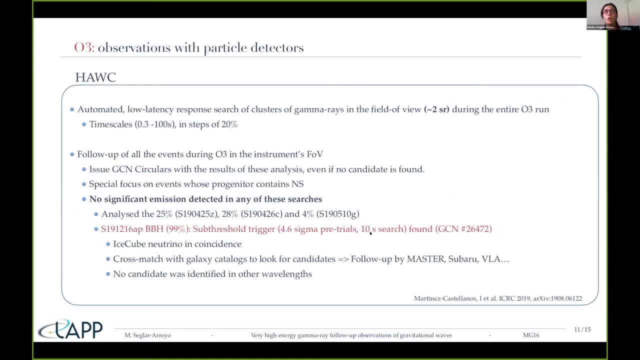 of the uncertainty region. Now, regarding HOG, there's been a really nice explanation on how this is done. I will just mention that they were issuing GCN circulars with the result of their analysis, even if no candidate is found, And there was this interesting discussion about this sub-stratio trigger that was 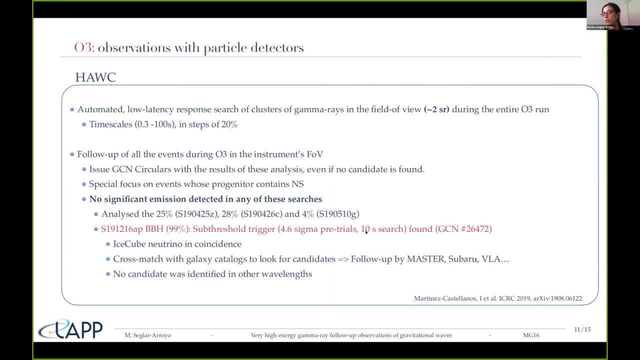 seen at 4.6 sigma protohylose with a 10-second search And there was an ice cube neutrino in constant. So there was this discussion. People cross-matched with galaxy catalogs to look for candidates And it was this follow-up campaign of the different candidates identified by 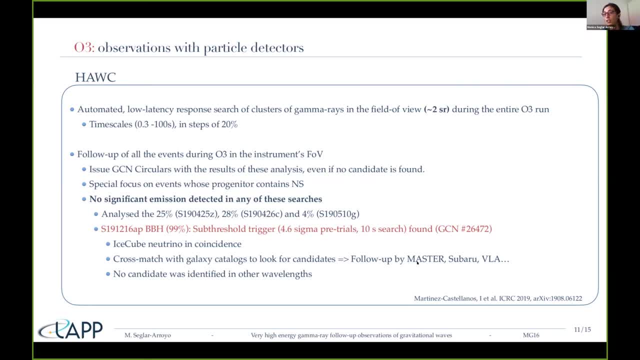 using galaxy catalogs by different instruments at different wavelengths. Nevertheless, no candidate was identified in other wavelengths in the end. So this is a very interesting study. So this is a very sometime-llor window. distillation for워ilding or coaching or5F speed sampling at MC. 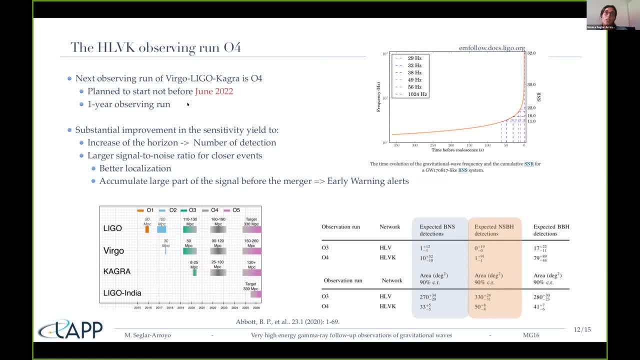 Now moving to свор. this is the next smart observing run that will start not before June 2022, next year- and it will be a one-year observe run with 4 interferometers, four in the network. These kind of have a big impact because each interferometers are improving their sensitivity. 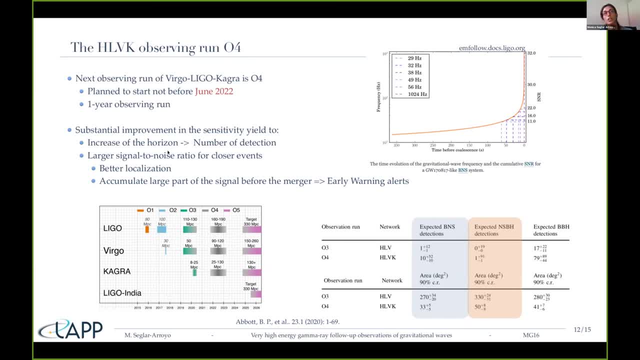 As well. this is eeP pessoal, Gorodong boubeom recstatabaay jeb we преfer excel story desim, including otherEND won causing of existence, reproducibe of는 we tactical. a increase on the number of detection, of course, and also larger signal to noise ratio for closer. 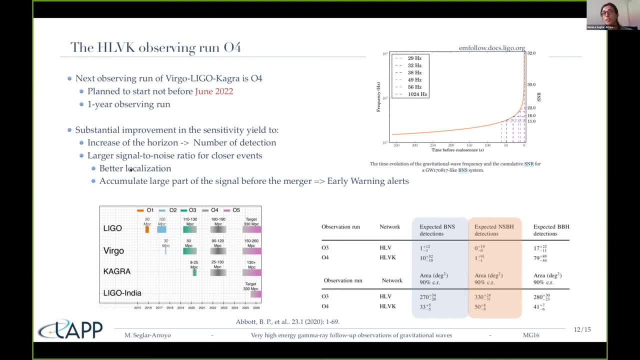 events. So in the end we will have better localization for the events. I quoted here some numbers for what is expected for the 90% uncertainty region in the case of 04, where we see an important improvement compared to 03.. And then the other feature. 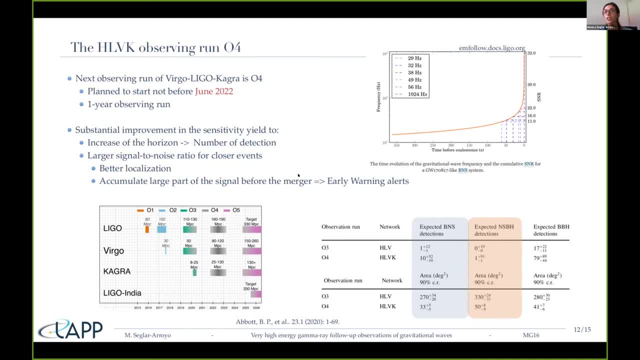 is these early warning alerts. So there's an effort in order to issue the alert. So first have the detection of the event and then issue the alert as soon as possible, So one could accumulate enough signal to noise ratio before the actual merger. So in this way we would like to try to. 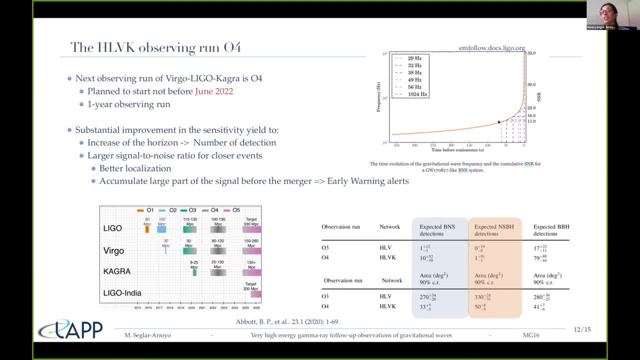 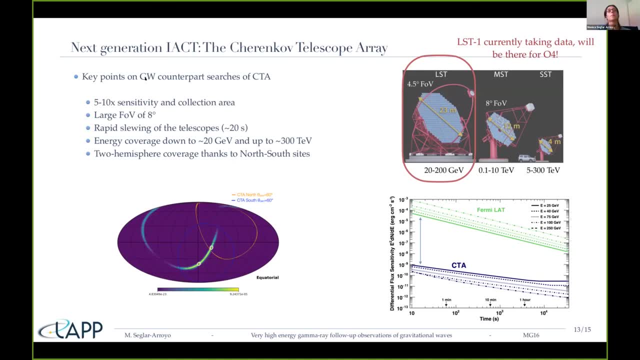 decrease the latency between the detection and the follow-up as much as possible. So now in 04, the first LSTs are already is already taking data, But probably next year maybe will be another one, But yeah, the next generation of ASTTs are going to are showing they have. 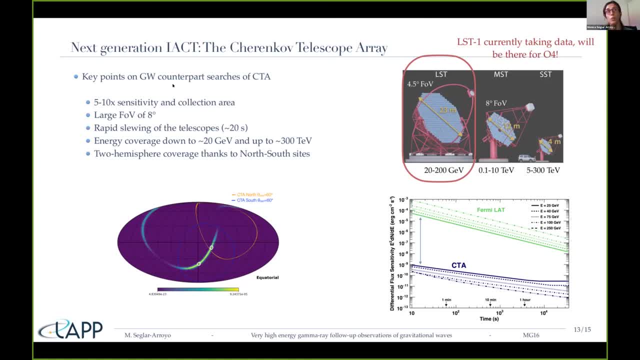 important features in order to look for gravitational counterparts. So these include the sensitivity, but also an increase of the field of view, also the rapid slewing which is really important for transients, as you know, but also the energy coverage down to lower energies Here. 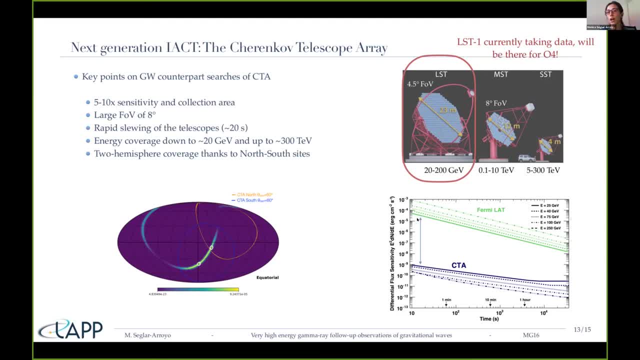 we see a comparison with Fermilat where we see how big these, the orders of magnitude are different for these short exposures. So these, together with the 2-emisphere coverage, it's really interesting and we are going to see probably interesting results in the future. 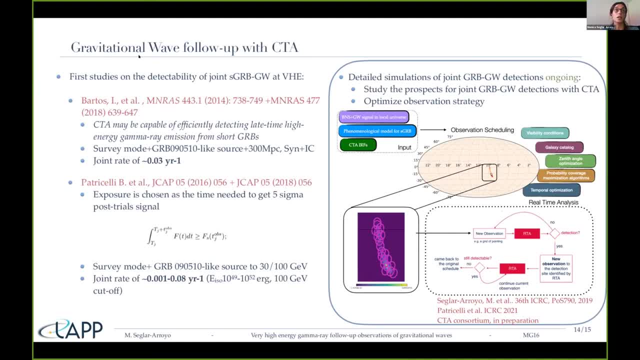 And regarding what is the prospect for this joint surgery, gravitational wave detection with CTA. there's been some studies, but by Bartosz already in 2014,- where they for a certain modeling and in a certain strategy which included a survey mode. 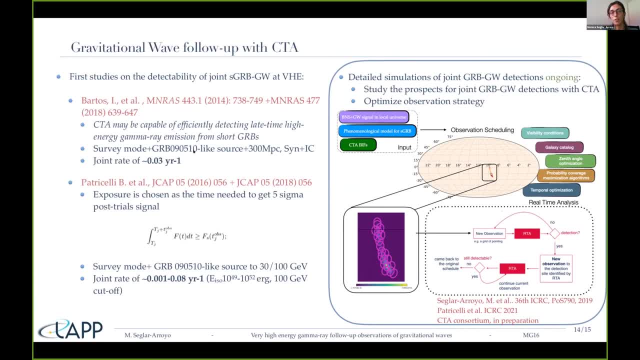 and included also well this gravitational wave 090510-like source, a place at a closer distance, and then considering synchrotron inverse content emission, et cetera, they were already saying that the CTA may be capable of efficiently detecting late-time high-energy gamma-ray emission from 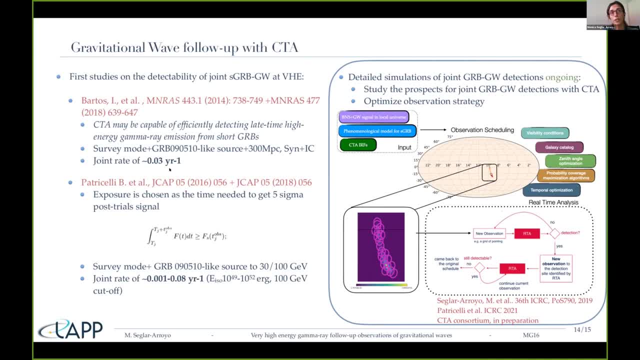 short GVs and, in the end, the newspaper. the joint rate that they're paying is around 0.03 events per year. for these assumptions, Then there was this other paper by Patricialli et al, where and study was done not only in the joint rate but also on the improvement coming from the fact of 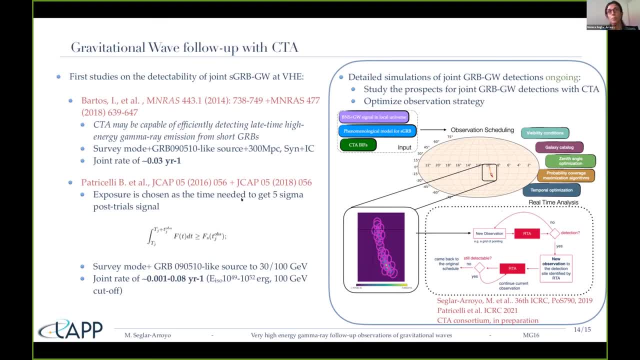 having an exposure. that is the time needed to get five sigma post-trials. So in this case and for these assumptions, the joint rate was of about 0.001% to 0.08, sorry, 0.08 events per year for these assumptions. 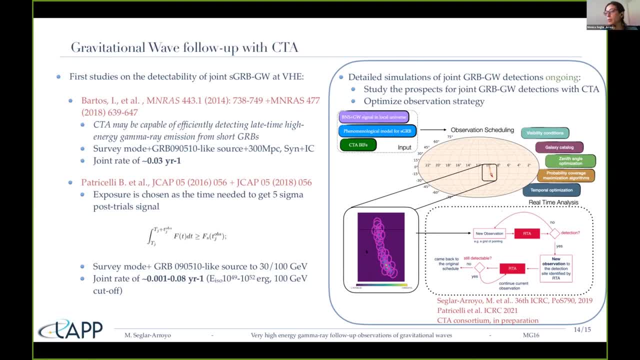 So now, results will be presented in ICRC next week, but already in ICRC 2019, we are going to be presenting this work which aims to study the prospect, with taking into account the recent TORB detections, for the phenomenological model and then an optimized 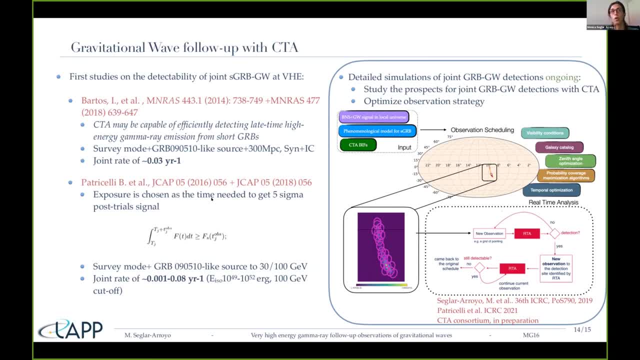 observational strategy in order to also study these prospects, which takes into account all these phenomenological models, also the last CTA-IRFs, The observation scheduling which takes into account the visibility conditions, standard angle optimization, et cetera, and then derives an algorithm and an observation. 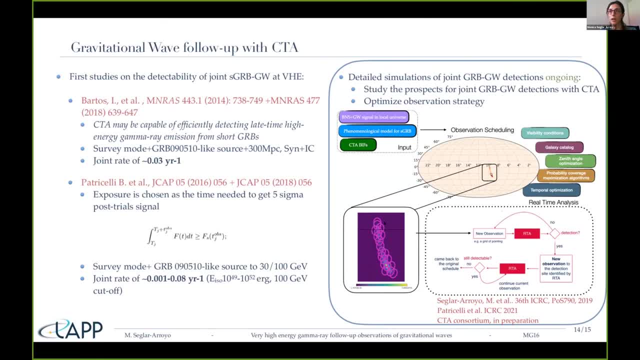 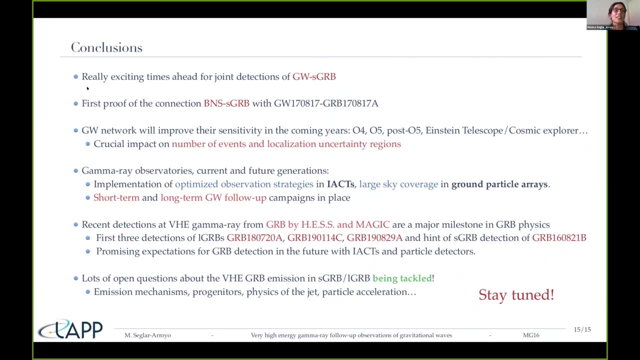 scheduling that looks like this, which would be connected to the real-time analysis and would be changing the observing region also depending on the results of the real-time analysis. So let me conclude with this: These are really exciting times ahead For joint detections of gravitational event, for GRB events. the first proof of the connection we saw it in 2017.. The gravitational network will keep improving their sensitivity and in coming years, not only with 04.05 and post-05, but also with future instruments as Einstein Telescope. So this is going to have a crucial impact. So I think we should keep pushing. 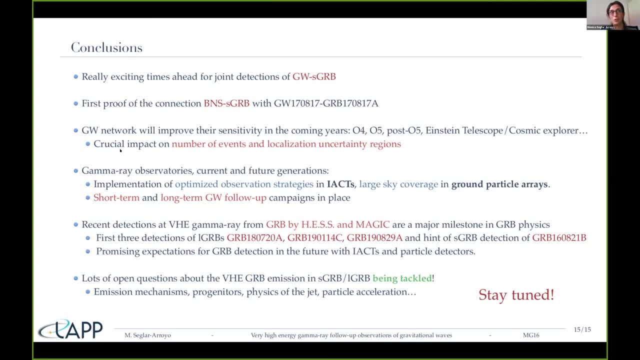 to find the short GRB counter Part of the gravitational detection. regarding gamma-ray observatories, there's different strategies for different instruments And it's really important this feedback between the ground particle arrays and the IDCTs, which also have their strategies. 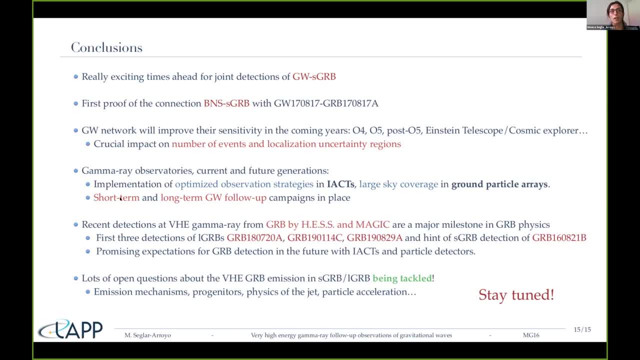 as I mentioned before. Then there's these campaigns in place, not only short-term but long-term, in order to study the afterglow for these events. And yeah, I won't give any. I won't say anything about these GRB detections. We already said everything, but I just 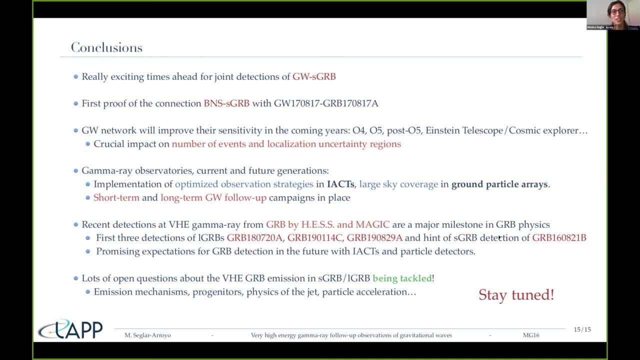 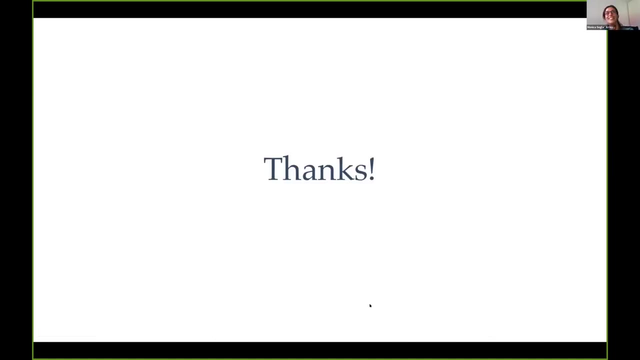 these are really a major milestone in GRB physics. This is promising times to study GRBs, including initial mechanisms, progenitors, fixes of jets and particle exteriors. So stay tuned, I guess. Thanks, Thanks, Monika. I don't know whether Fabian is still here. Thanks for the nice talk. 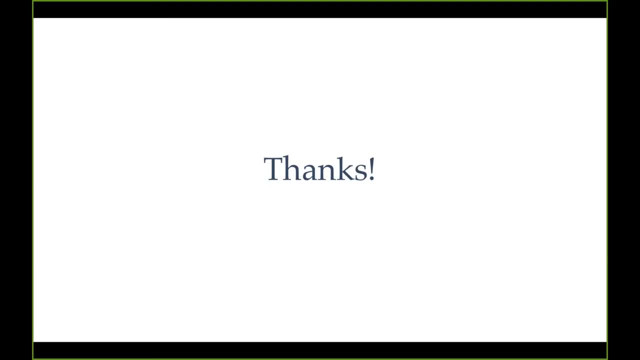 Are there questions to Monika? Thanks a lot. Can you hear me? I have some Some kind of connection problems. Yeah, Okay, I can hear you. Well, not now, I cannot hear you. So are there any questions to Monika? in the meantime that Fabian tried to, 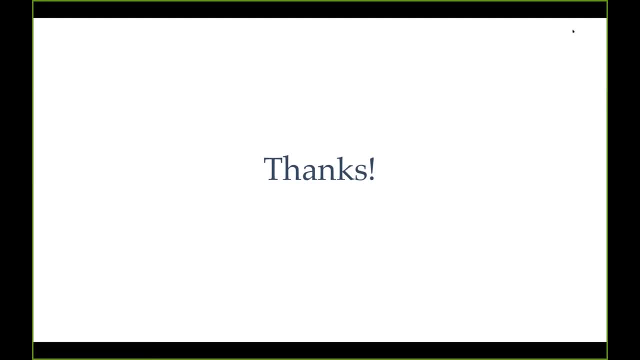 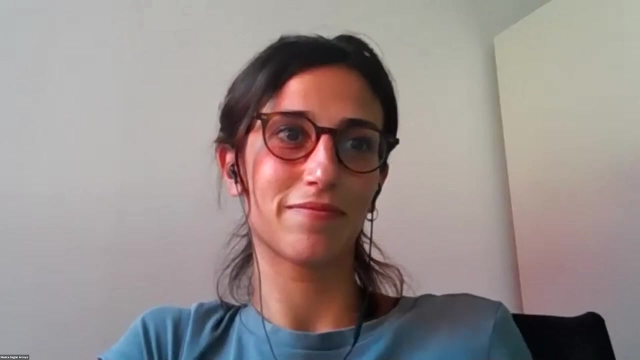 To unmute himself. Otherwise you can write it on the chat and I will answer. Okay, so I don't see any raise hand. So we thank Monika again for the nice talk. Now we try to go and thanks the speaker for the nice introduction to this very nice topic. 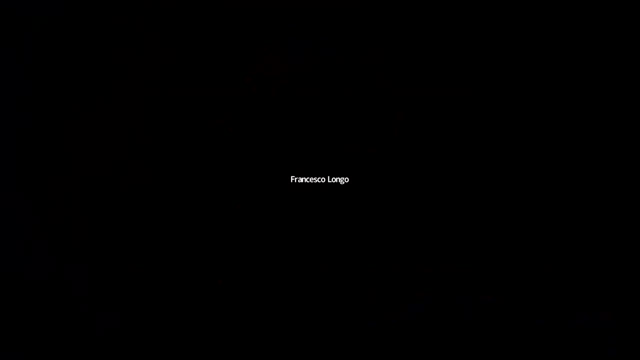 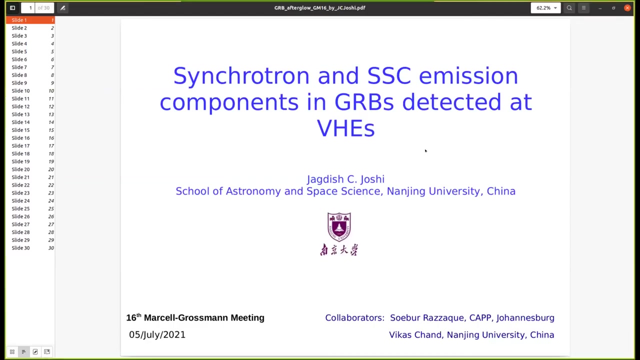 and now we shall go to the last talk of the of the session by Yagdig Yoshi, and he might try to share again the screen and try to talk. can you try to talk now? yes, so, can you hear me now? yes, perfectly, so go ahead. can you see my screen? yes, okay, thank you. thank you for the presence and 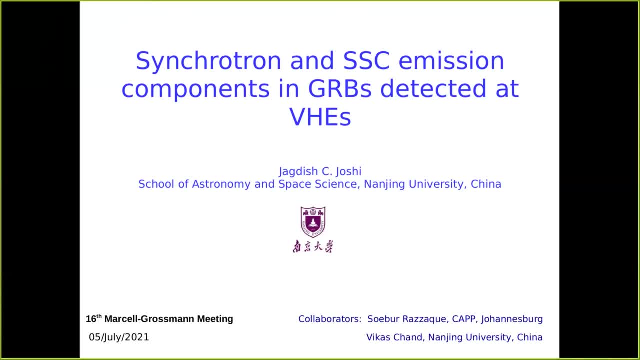 it was some issue with my network actually, so it so from the talk in the session it is very clear that this very high energy component is very important. we know from the modeling of GRBs that at lower part of the spectrum in the x-ray on radio, the synchrotron is the dominant mechanism. 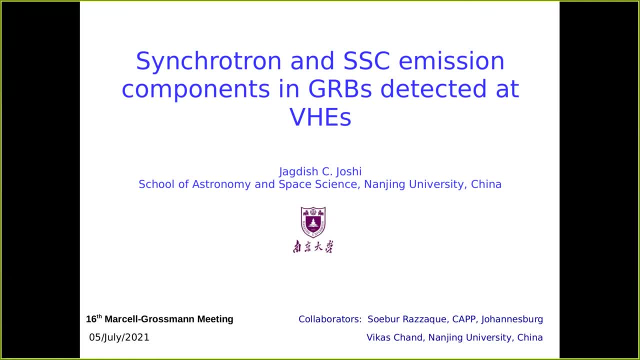 it produces the afterglow well. but when we go in the high energy and very high energy, there are competing channels like the synchrotron ssc and the high energy and very high energy, there are competing channels like the synchrotron ssc and. 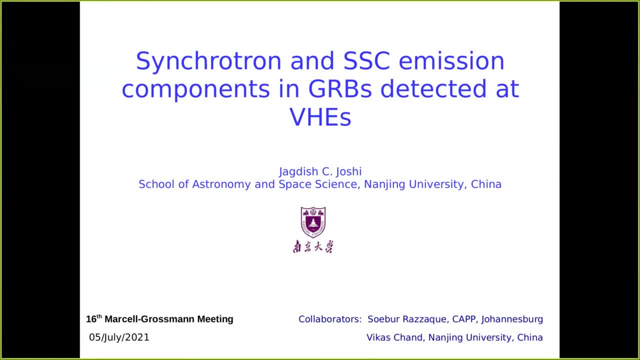 the high energy and very high energy. there are competing channels like the synchrotron, ssc and external competent, so this is very good time to study all these processes. so this work has been done with soy at university of johannesburg and vikas, who is. 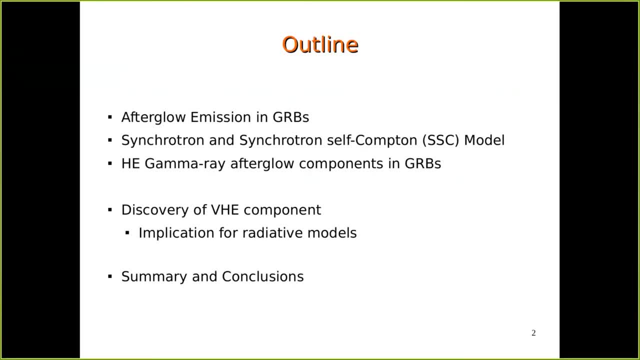 a postdoc at nanji. so my talk will give some view about ssc model and then i will discuss about this high energy in the fermi era, how it, how it was important to understand these composition in the blast way, and then i will discuss the radiative models already. 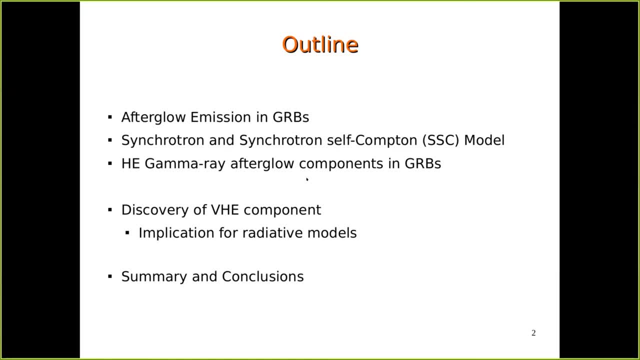 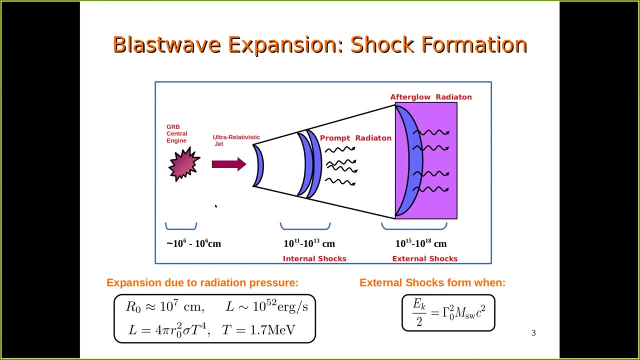 we have a lot of good discussion about the discovery of very high energy component in GRBs. so in the schematic picture of GRB we know we have the central source around 10 k or 6 to 10 k or 7 centimeter size and then it leads to ultra-radiated jet and makes the prompt. 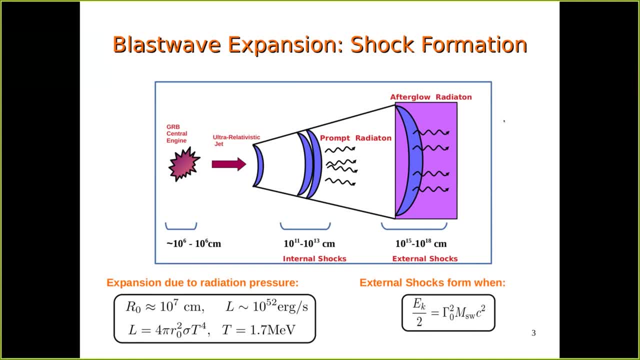 radiation. here, part of the jet energy interacts with the surrounding medium and it leads to the afterglow radiation. so most of the afterglow radiation it comes from distances around this. at these distances, what happens? that some of the afterglow parameters, or for certain set of 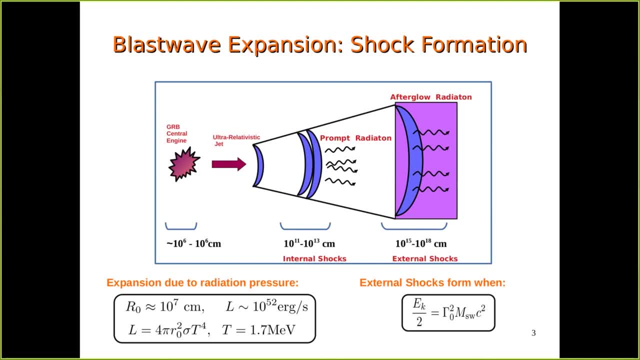 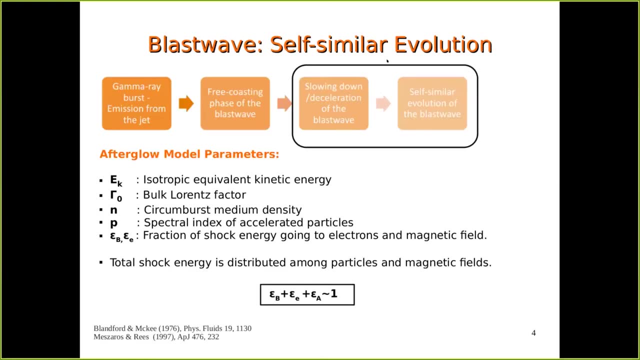 afterglow parameters. very high energy gamma ray do escape and they they don't go gamma gamma pair production. so optical radiation is actually one of the one of the zone where a very high energy gamma ray can escape to the observer. so the afterglow models generally, what they based on, 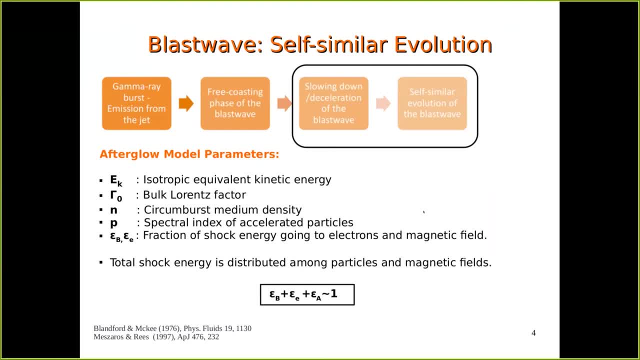 are is self-similar evolution. what happens that you have this blast wave going to the surrounding, a circumcised medium, and where, and the orange factor, as well as the radius of the blast wave, can be written as a function of time and based on that one can drive. 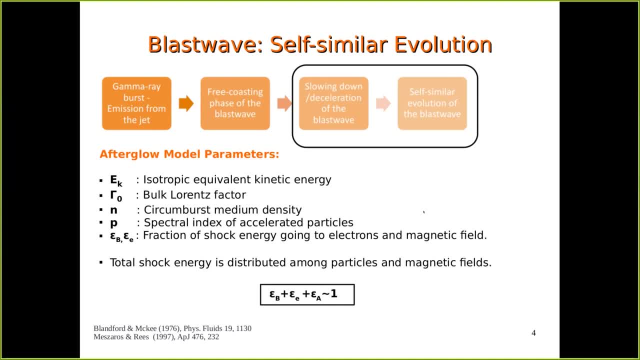 the blast wave dynamics and, as well as the radius and channels, the model parameters. what already discussed in the earlier talks are basically these: the initial kinetic energy, the bulk orange factors and from this, density and the relativistic electron index, as well as the energy distributed in the particles. 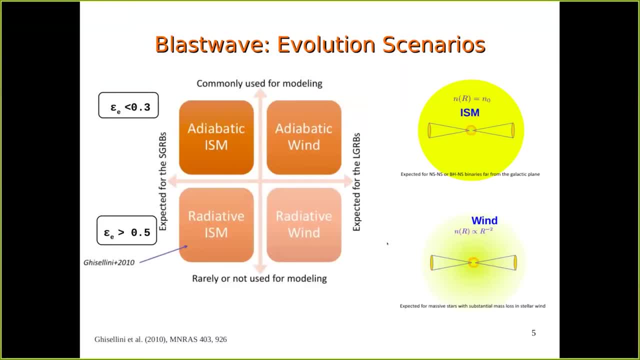 so in generally considering the electrons and particles in the blast wave we have either the adiabatic case and the radiative case. in the community generally these two cases- adiabatic blast in the ism and wind- are very popular and generally used. the reason is the amount of energy. 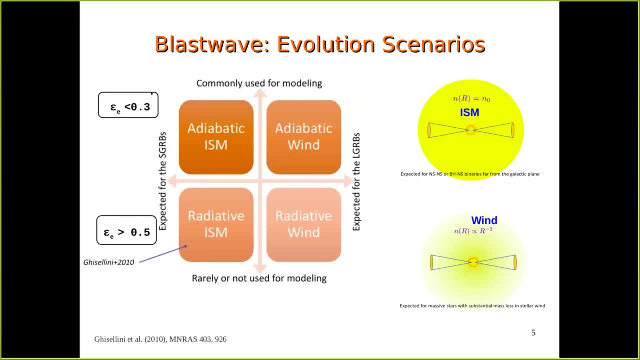 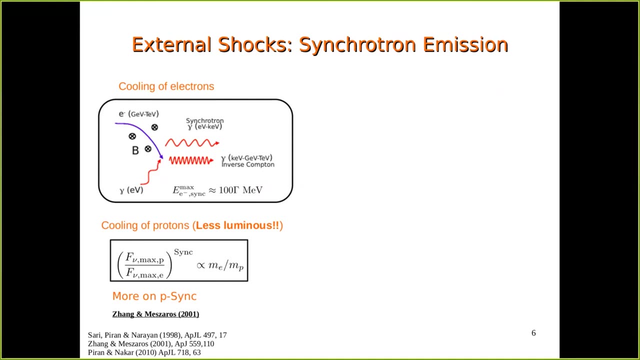 in the electrons needed, less so compared to the radiative case. so with respect to the power budget, these two cases are favorable and generally used in the blast wave in the modeling. so we know for the synchrotron radiation, the particles accelerate at the shock region and they undergo this cooling. synchrotron cooling produces the 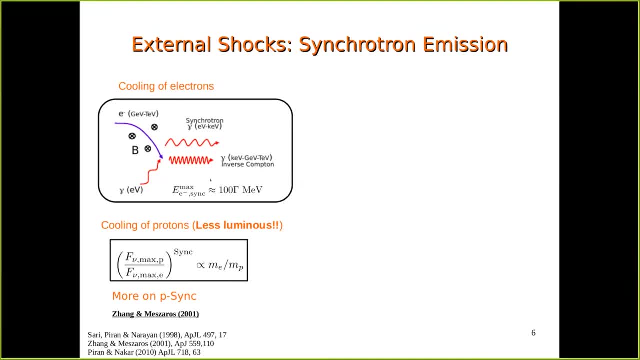 radiation, the maximum energy. this is the challenging task now because in the fermi era we know the energy can be around 100 times bulk orange factor and the bulk orange factor is around 500 or maximum maybe thousand. so it can go about up to tens of gb. 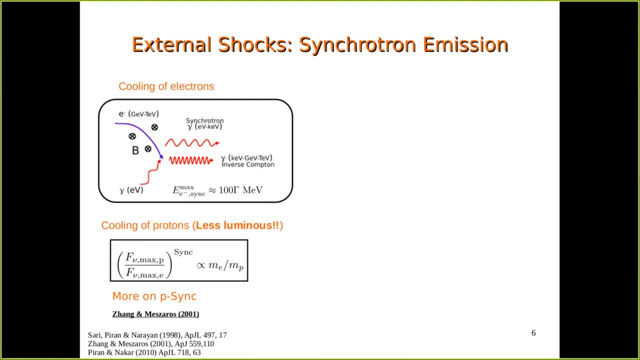 so this? this is an interesting point, like with the very high energy component discovering grh, whether this channel is still very important or not, which is already we have seen in the discussion of 190829a- that what can be the physical motivation for synchrotron to continue up to very 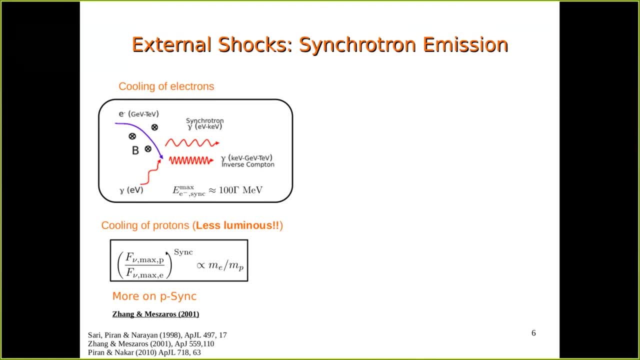 high energy other than synchrotron radiation. what we have is proton synchrotron of so this process. what happens? if you compare the ratio of maximum flux, it is the proton synchrotron is 1000 times lower in flux compared to the electron synchrotron, so electron synchrotron is dominant. 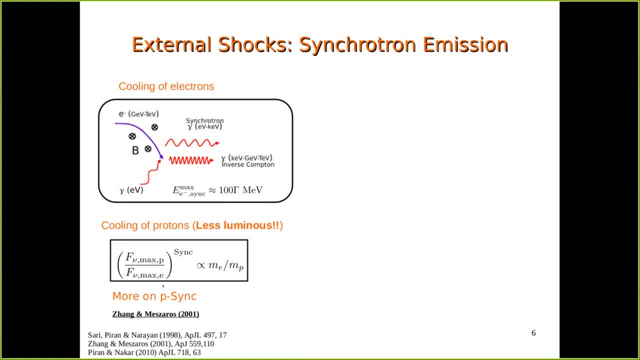 but if you want to check when proton synchrotron can be important above some energy range, so please see this paper by jahan in measures 2001.. so this is the general picture of synchrotron radiation shown as the cd in the analytical spectrum of sari and piran 1998 paper. early in the time the 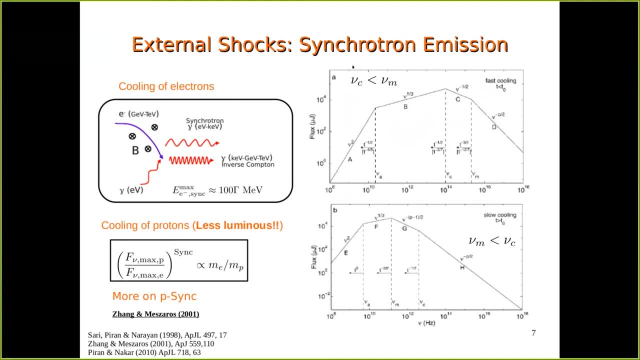 electrons cool very fast in the blast wave and they follow this frequency order. the cooling frequency is less than the frequency corresponding to minimum lawrence factor. have a certain time at t naught, the. when there is a transition between um and uc, the order changes and the system goes to. 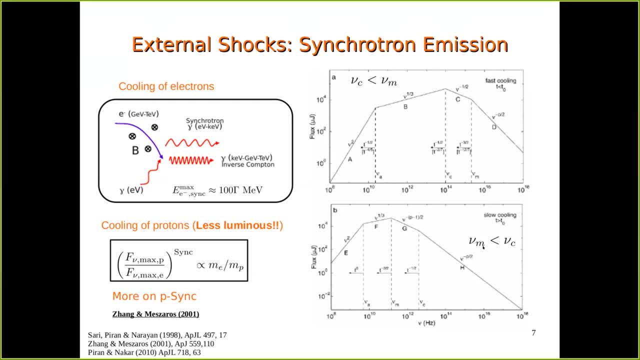 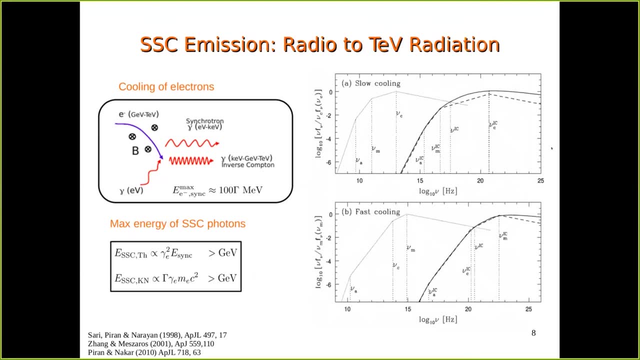 the slow cooling. in the slow cooling the electrons have mostly about new c. they are cooled. in the fast cooling most of the electrons are cooled within the dynamic time of the last wave. so other mechanism which is a natural process, like because we have the electrons in the system, 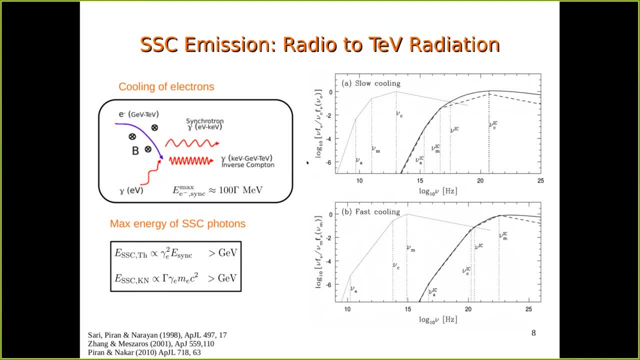 in the blast wave and we have the building platforms. uh, these electrons, basically these photons can be upscaled by the electrons and can produce this mirror copy of the supertron emission. again, the same two important, the two channels which are very important, like the slow cooling and the fast cooling, can be discussed in this scenario. the ssc can be either in the thompson, 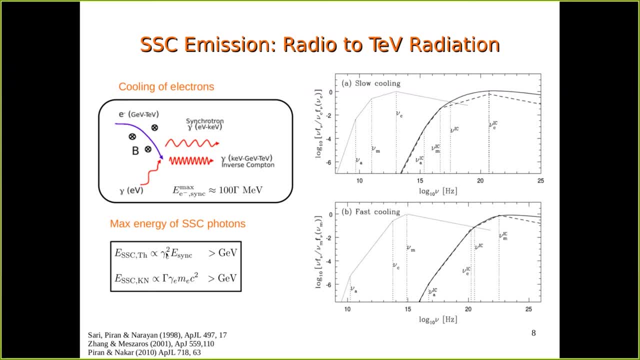 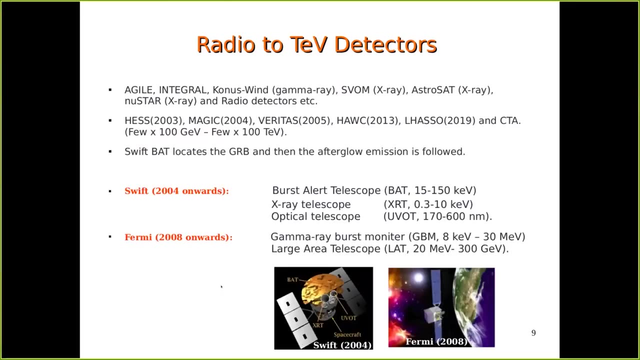 regime where the opportunity photon energy is vaulted square times the single photon energy, or it can be in the clean trust regime where the this is proportional to the linearly proportional to the electron allowance factor. I will just skip this slide, because we have already very nice discussion about how multi-wavelength 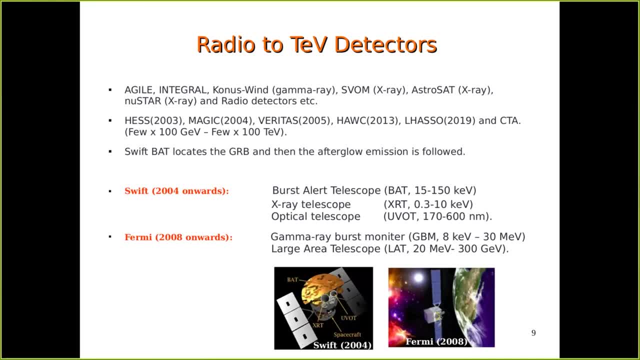 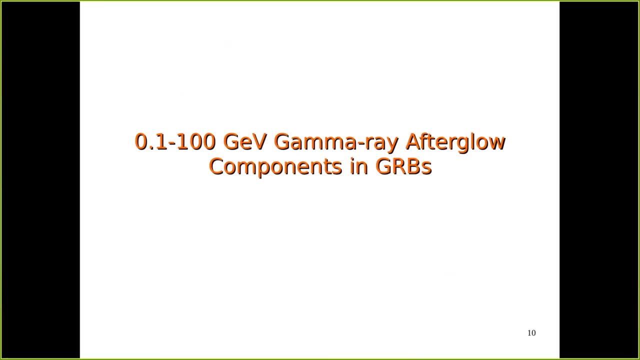 radiation is giving us the afterglow picture and giving us sources in lower wavelength, high energy to very, very high energy. So here I will just give two examples: in the Fermi era, which we had the bright GRBs, where this component discovery had been used to understand the jet composition. 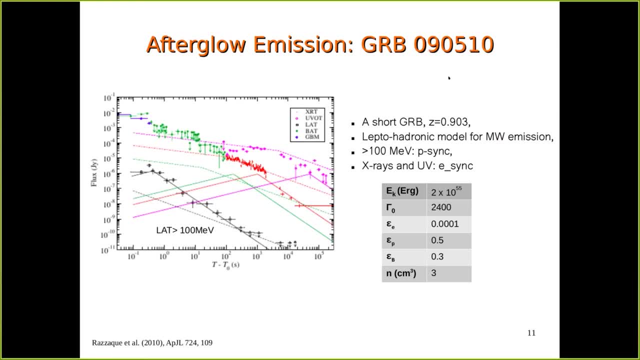 So, for example, if one considered GRB 090510, what happened? that that detected this component above 100 MeV and this, this flux with time, has you see evidence, basically, of a break in the in the component. So the, so this, this component was the studied and the origin of this component was was found to be consistent with the proton. 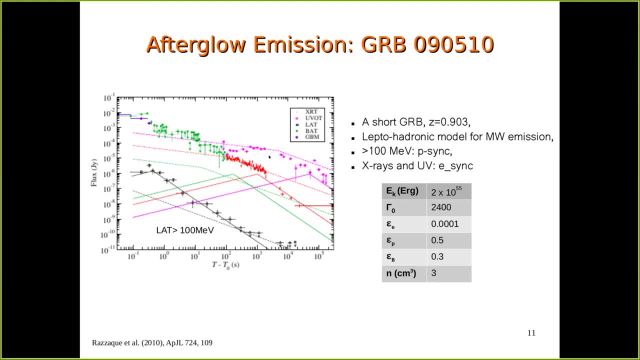 synchrotron model. However, these radiation, in the x-ray and when optical, were dominant by the electron synchrotron radiation. However, to do this, one has to make sure that the fraction of energy going to protons is thousand times larger than the fraction of energy going to 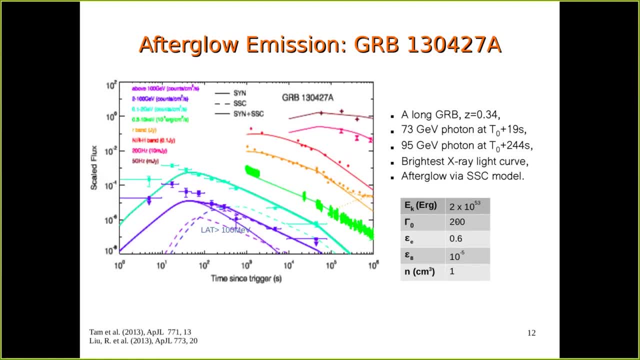 electrons. So, other than the short GRB, we have another example of long, GRB 1304-27a. It was one of the brightest GRB before the very high energy era and we had photons of energy 95 gV in the upper globe, very close to the boundary where the high 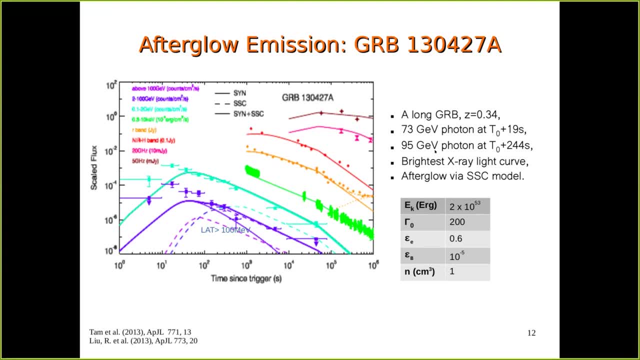 energy gets transitioned to the very high energy. So Tamm and Liu at all discuss the origin of this component, of this LED component, and they found that its superimposed- as I previously salt give this 晶- andστial component is high, higher At this point, for example, in light, in light light, using this. 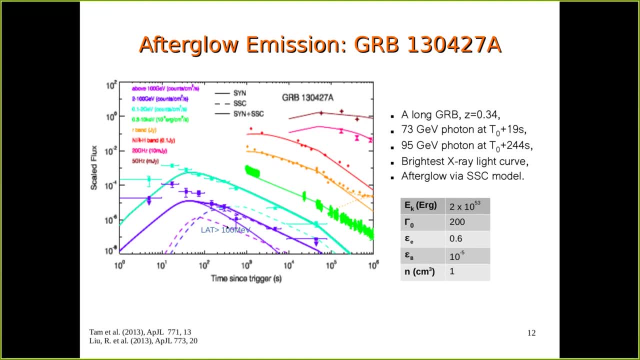 Now the order is very similar, because many curry would normally be dedicated because energy has been found that this can be explained with a SSC component. So this was the first indication that SSC component may exist in GRBs, but after 2013 it took a few years, like 2006 years, to really 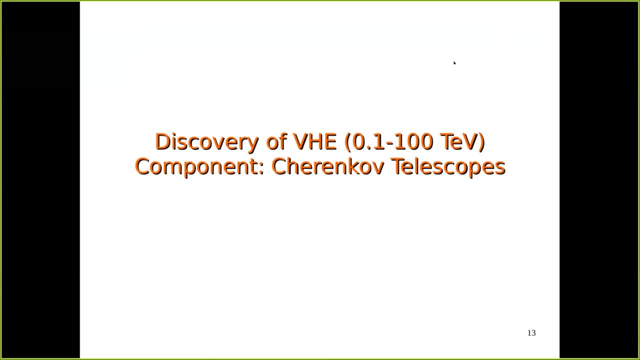 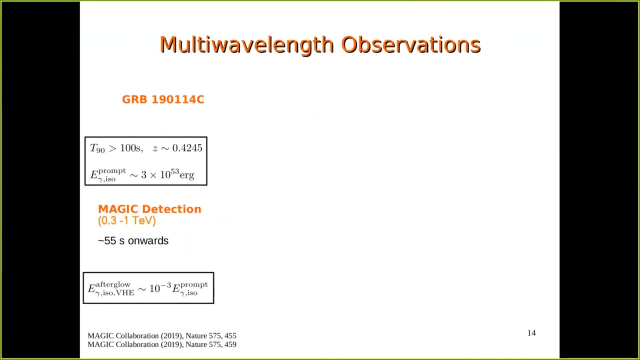 discover some component which is very hard in very high energy and can be, can be, can be explained with something like SSC or EC without any challenge from the synchrotron component. So here I will just discuss. I will actually skip because already there is really good discussion. 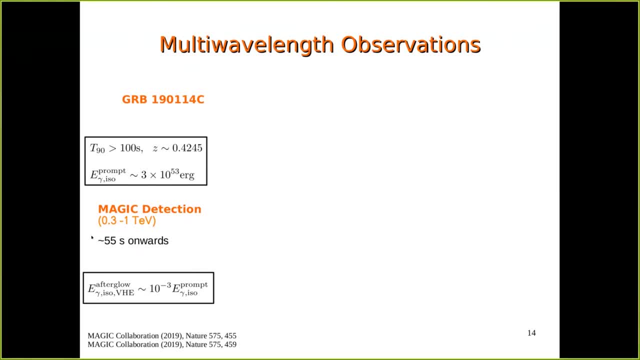 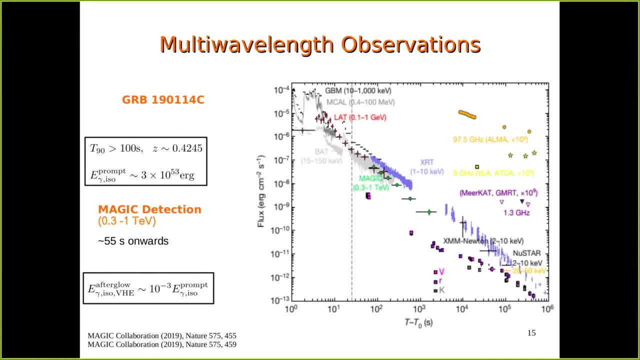 about this magic GRB, and we know this magic detection starts somewhere above 55 second and if one consider the emission in the upper globe, they follow power law, nice power law. they are the prediction of the fireball model and the emission in the, in the magic he starts here, which is approximately having isotropic energy 10 to the power minus three. 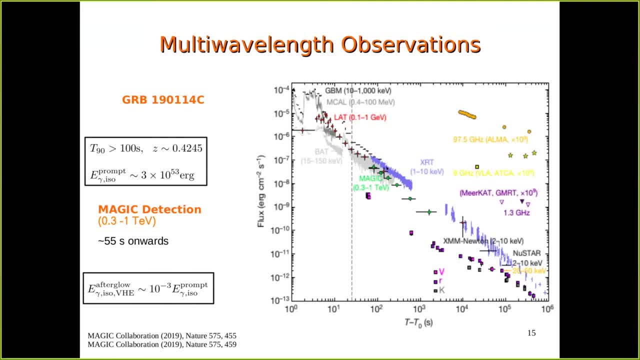 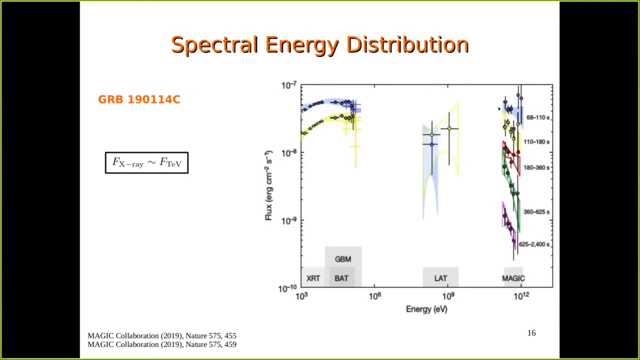 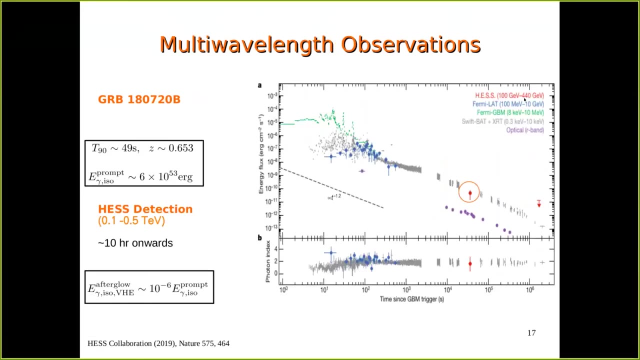 times the isotropic energy in the prompt emission. So these were the first signals and in the very high energy and if one consider the X-ray flux they follow, having they have very similar flux levels in X-ray and at TV. The second GRB, the HES one, have been a component detected. 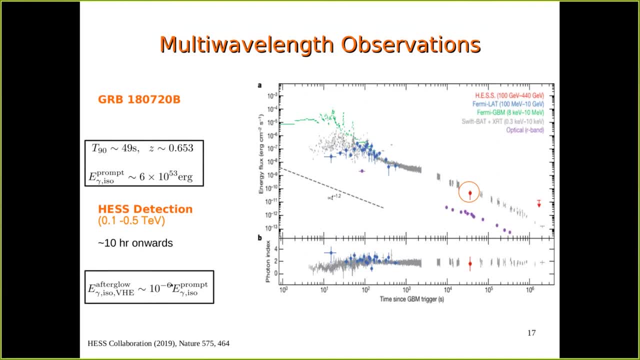 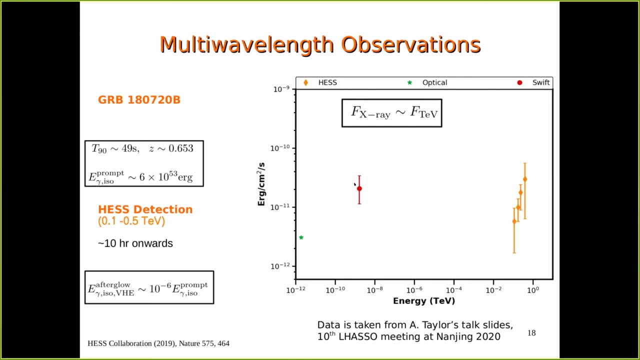 hours was very, very deep because the flux levels and the isotropic energy were like 10 to the power, minus six times the isotropic energy in the prompt emission. So it was again another long GRP and it was having the flux levels very similar in the x-ray as well as in the in the TV band. 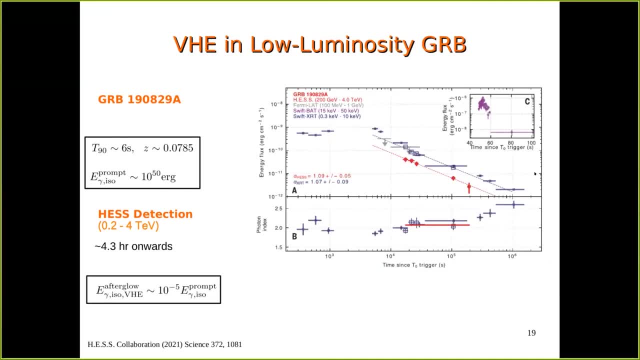 So, as discussed by the the talk earlier by Adina, that these light curves are very well detected by Hess after like first night, second night and third night, and there was, the signal was very strong here and then the significance goes down. It was the example of a low-limiting GRP. 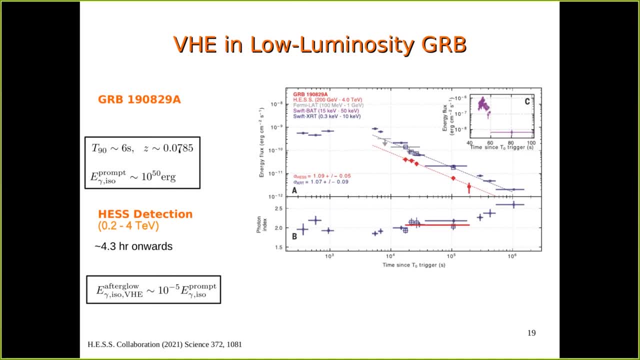 where the luminosity is around anywhere 50R and it was very local source. So this means the eBL attenuations are not very important, as well as, because of very low luminosity of this source, the internal attenuation are also less effective. Again, this 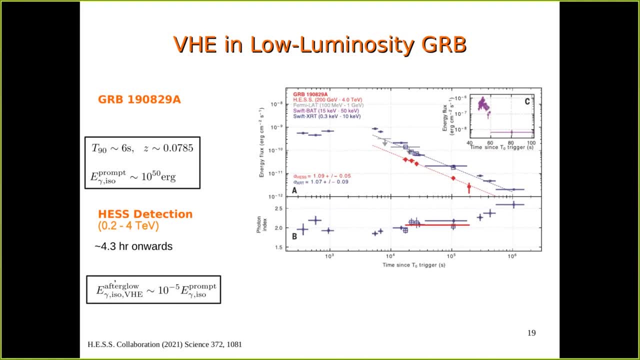 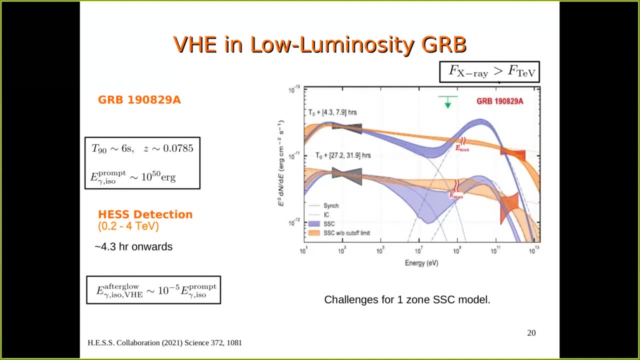 was a deep signal around ngr, minus five times energy in the afterglow compared to the prompt emission Here already discussed. like, as in this GRP, we have x-ray flux levels greater than TV flux level. So the extrapolar radiation of synchrotron can explain this very high energy regime. but the question again comes. 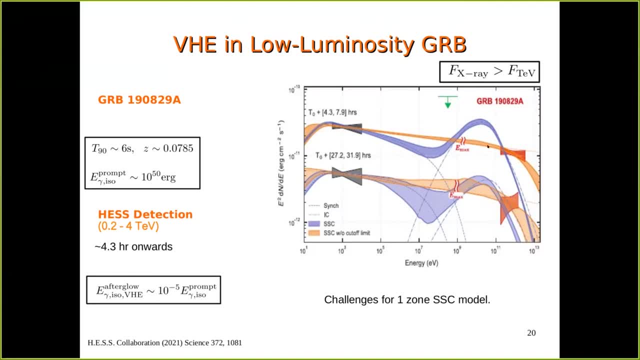 like physical challenges in the sense how one can achieve these energies in the synchrotron model. So this GRP already opens this question, whether synchrotron radiation can reach to this energy or not. However, there are future. so again they tried to explain the source with the SSC. 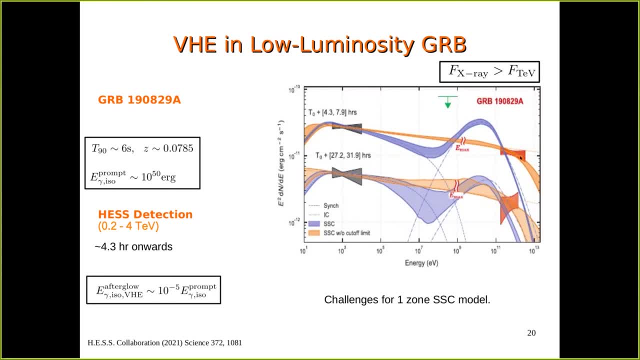 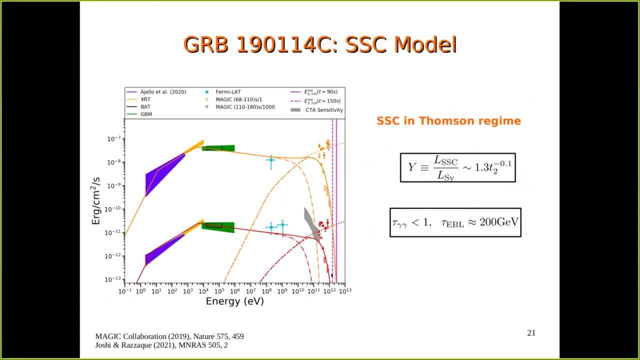 and it was not very, very well created compared to synchrotron. So I will discuss here our modeling of this GRP190114C using an SSC model and we found that the SSC process takes place. these photons basically takes place in the Thomson scattering. 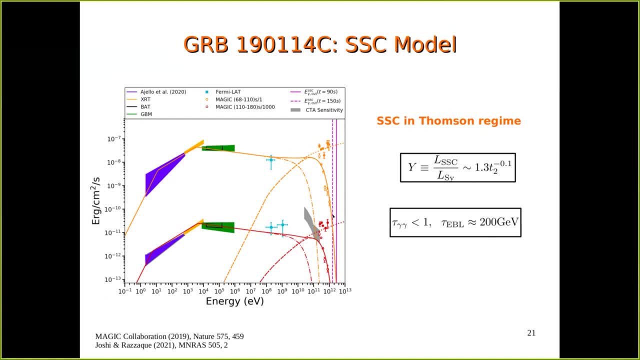 regime. These vertical lines here they show the Thomson maximum energy at 90 second and 150 second. So with time the Thomson scattered maximum energy of photons in the SSC goes to lower energy. So late in time the process would definitely go to planation. 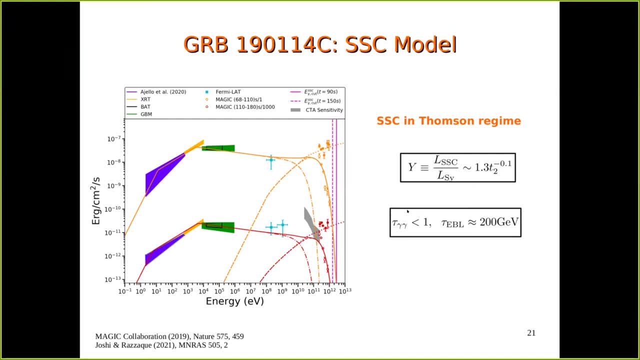 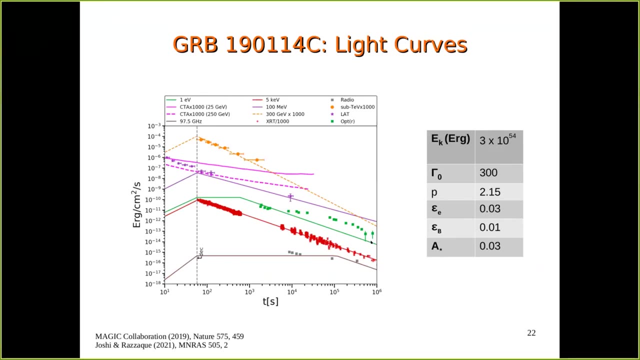 regime. Here we found the internal attenuations are not very important and the EBL starts to be effective at 200 Gb, using the Finke et al model and consistent with the attenuation shown here. Using the same, using the same, yeah, using the same set of. 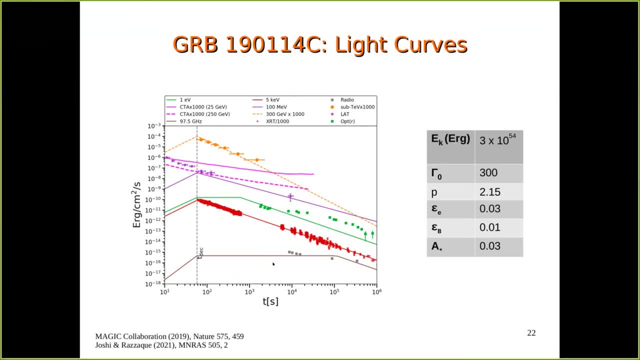 parameters. can you hear me? sorry? just to confirm: yes, go ahead. okay, sorry, okay. so, using the same set of parameters, we also plotted the light curves and we found that consistently we can explain most of the light curve but not the optical ones, because in the optical we found there is this: 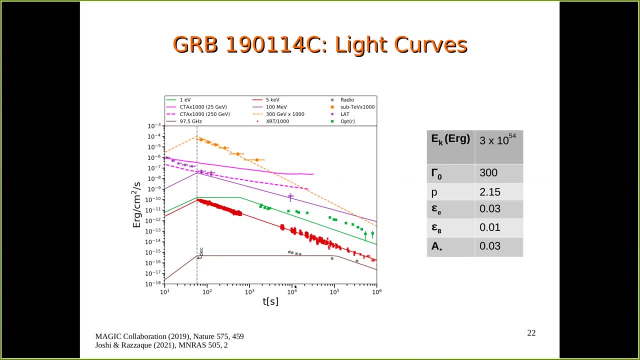 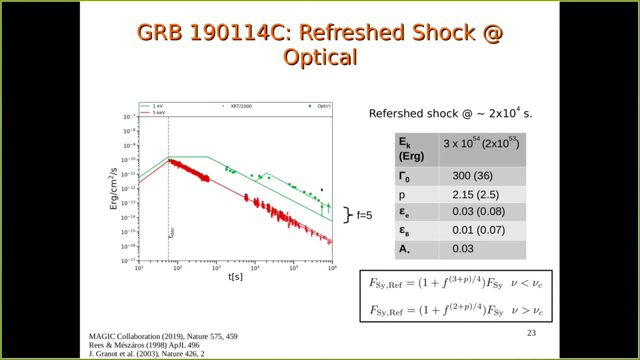 hardness seen after around approximately 10 to the power 4 seconds. So we exclude the origin of this optical hardness using a slower moving cell which takes energy from the internal shock and then later hits this forward decelerating cell. So what happens that using this? so we found that we need energy like approximately 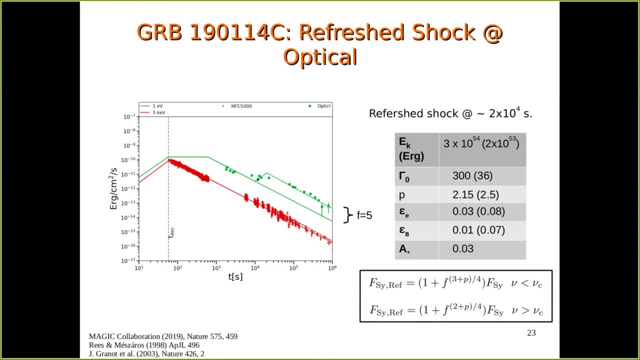 10 times lower in this slow moving cell and at this onset it got the Lorentz factor around 36 and more or less the these parameters are in the equipartisan. So we this this level of hardness is around like in the ratio of 5 and using the refresh shock scenario we can calculate how the 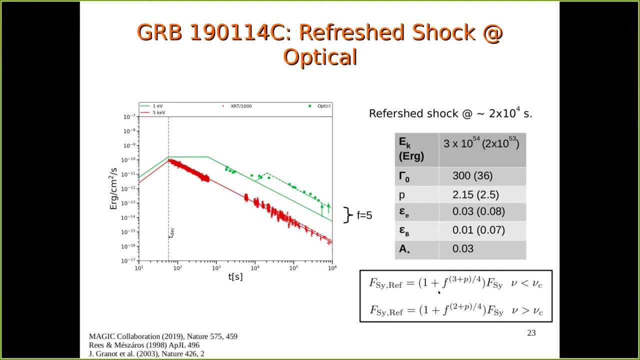 flux will be affected and so it affects the below the cooling frequency mostly and above the cooling frequency. So we get this hardness explained here and, corresponding to this hardness, we do get some effect in the x-ray also, but they are consistent within the data. However, these refresh shock has some of the signature in the in the reverse shock, but 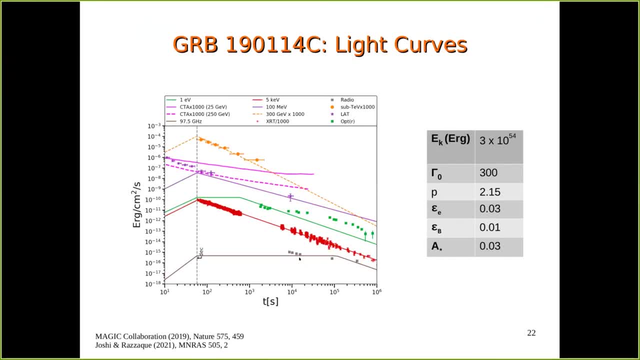 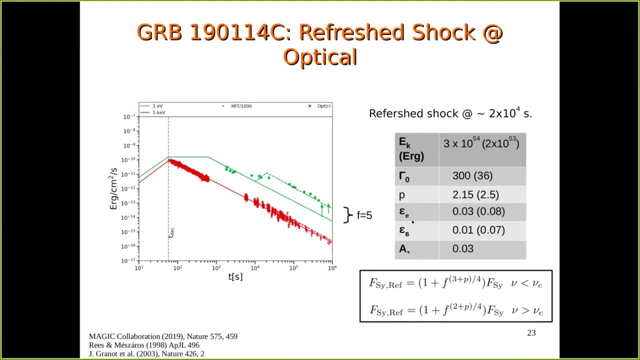 in this source, more or less the radio, etc. can be explained with the forward shock model. However, what we think, that these micro physical parameters like epsilon e and epsilon b can be different from for the reverse shock and can have less significant signal as we don't see a 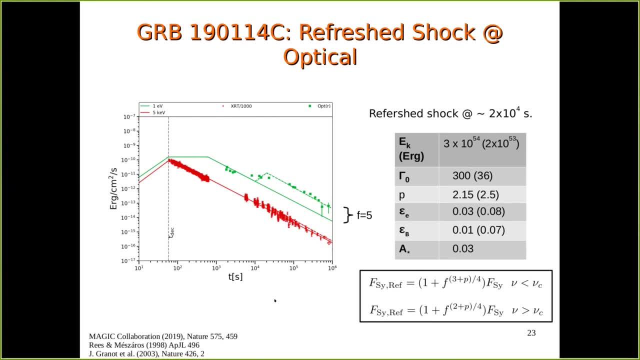 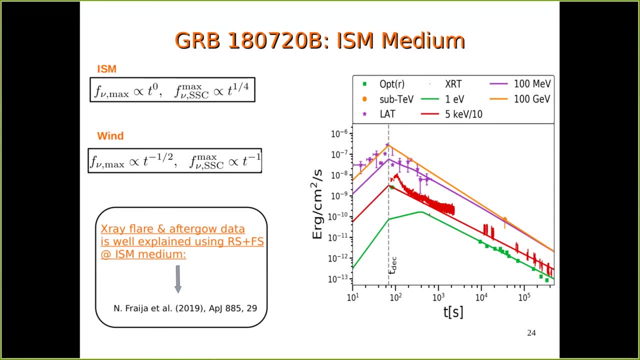 significant radio and IR signal in this source. Then we also studied this GRB 1807-20B, which is which is like detected by HESS late in time. One of the one of the question is like the late time detection means there should be. 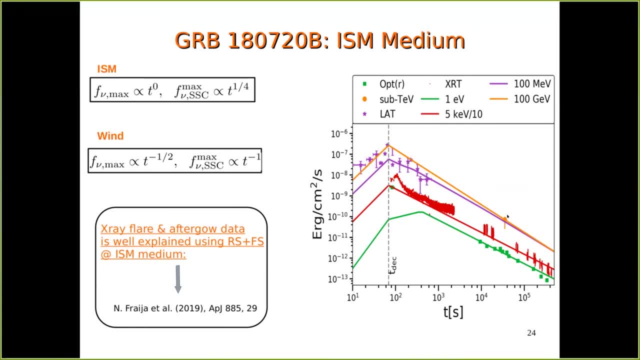 a good amount of flux in the late of late time as well as as well as the detector sensitivity. So if one consider the ISM and wind blast wave models, the ISM has maximum SSC flux which increases with time, and the wind has the flux maximum SSC plus, which goes t minus one with time. So there, 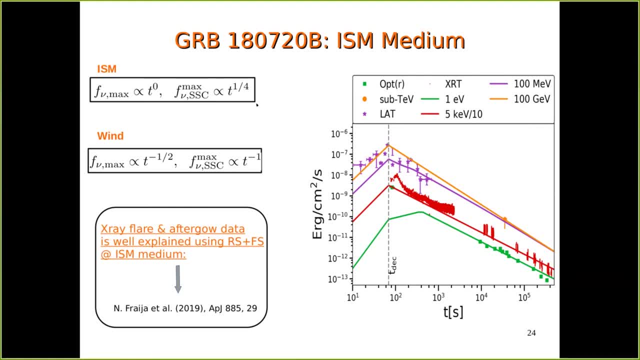 is slight bias around for the ISM medium to explain the late time, these observations in very high energy. Also, if one consider- we have one check the paper by Frey et al. they have discussed that the closure relation of x-ray light curve infers that ISM model would be a better one for. 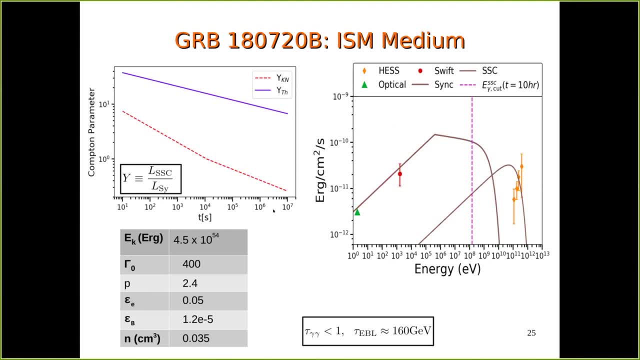 this source. So here we. we found that these photons again, because this is the magnet, this vertical line here shows the maximum energy due to Thomson scattering. So these photons are definitely in the Klemensina regime. So then one has to consider this Klemensina y-parameter, which 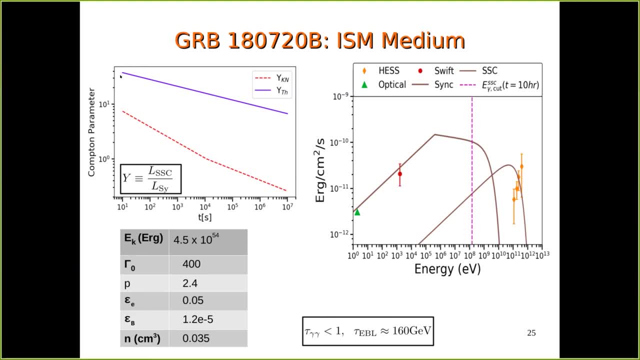 significantly reduces around like a factor of four, the y-parameter and based on that, what we found, that the Klemensina regime required in this to explain the late time observations here and the internet, innovation is not important and this EBL, I think, starts around 160 GB based on Finke et al model. 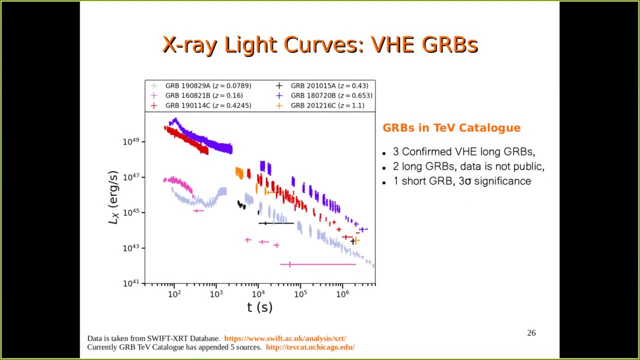 So, based on this, the sample of GRBs which are available in TEB catalog for now we have three confirmed sources and all of them are long GRBs. One is low luminosity GRBs, so this shows that the diversity in the luminosity is large. So that is a good news, because 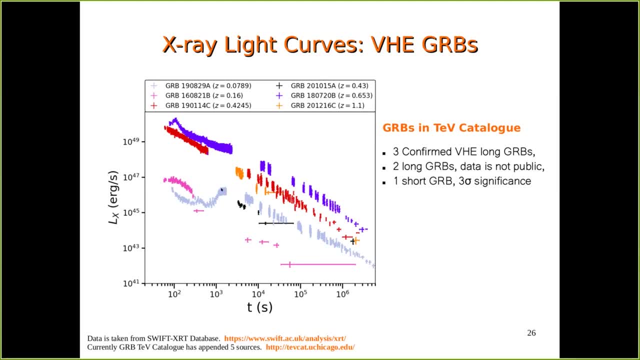 this means that the very high energy component is available in the low luminosity GRB as well as in a standard GRB. So that will enhance the detection of GRB in very high energy regime by the upcoming CTA and LASSO and already well active take down based telescopes. There is another. 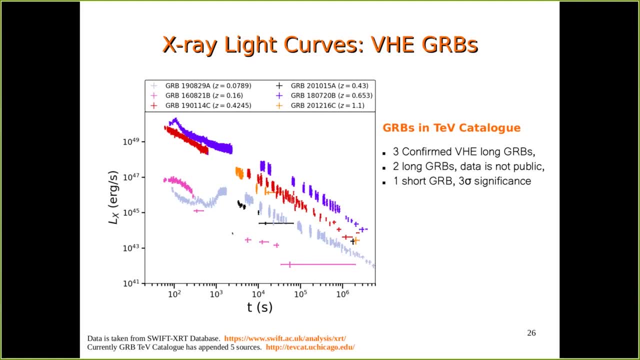 short GRV with three sigma significance. already discussed about it in the in the previous session talks, so I will just skip it. So currently, if you check the modeling of these samples, either SSC or external inverse Compton, where the target photons for scattering of where the target photons 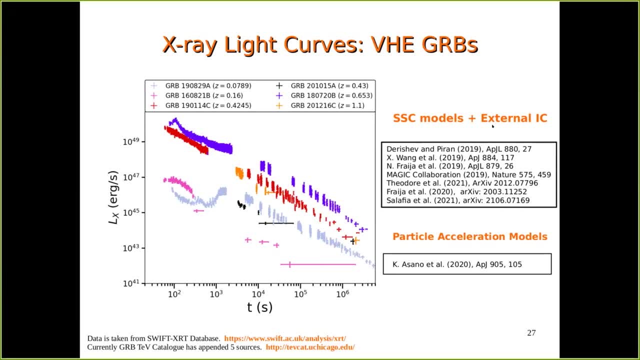 are not from the blast wave, from the zone one, but can be somewhere in the other region of the source or of the galaxy. mostly it's in in the flare region. for example, a recent paper by by this, Theodore et al. They estimate that this low luminosity GRV has these X-ray flares and 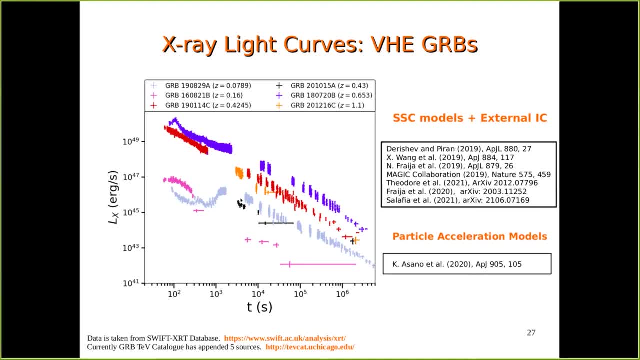 they can be very important for the external Compton. to explain the, the multi-wavelength emission in GRV 190829a, which helps because when SSC model doesn't work, there is a chance that the ISEE- external ISEE is very important- can work. Also, there is another paper about the same source by Salafi et al which discusses that. 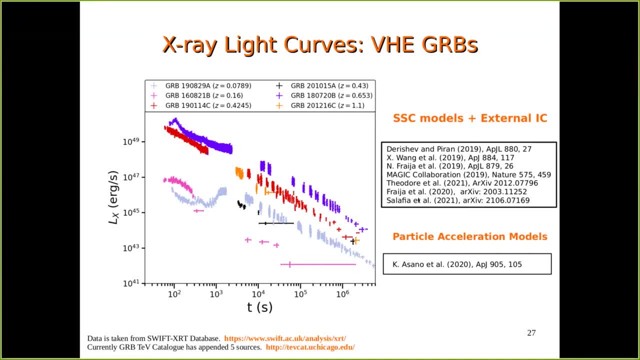 the SSC can more or less work for GRB190829A. So, other than that, using these very high energy observations in gamma rays, Asano et al has discussed recently the implications for studying the electron acceleration at the shock region. So, more or less, we are reaching to a regime where 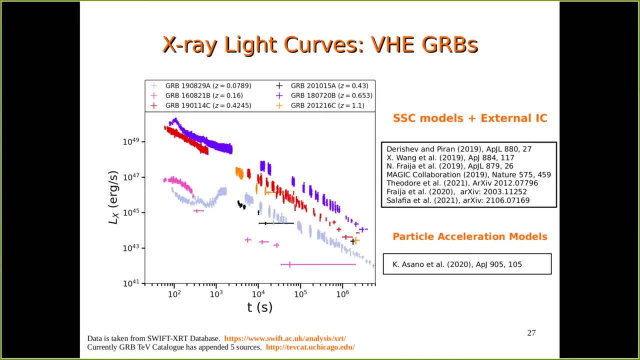 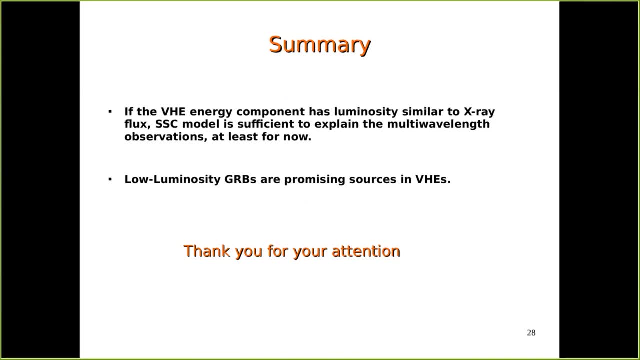 in the transients we have very high energy gamma ray observations and we can study the relativistic shock physics also for these time zones. So with this I will just come to my summary that at least if the X-ray and TEV flux are of the same level, then SSC models. 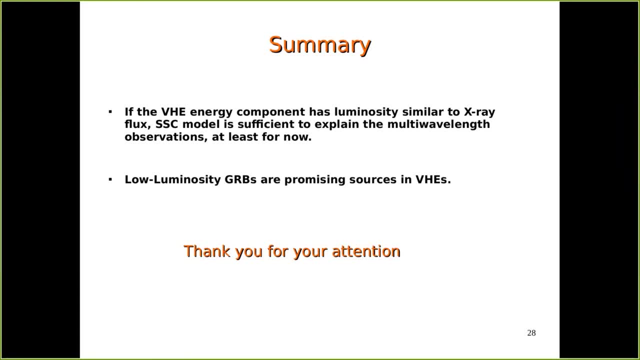 are look sufficient. If not, then there are, like for example, for GRB190829A- there are three competing models, either electron cyclotron or SSC or external content. So it would be interesting to see that in future, if more low luminosity GRBs detected, then how the modeling goes and what we understand in future. So it's very low luminosity. 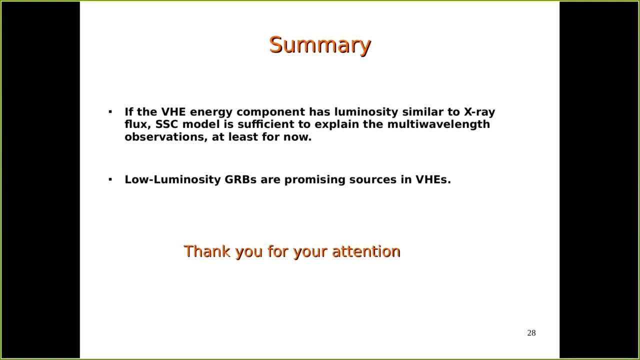 GRB in particular, their frequency is higher and they are nearby, so they can give more intrinsic information about the very high energy spectrum of gamma rays bus. So it will be interesting. Thanks for your attention. Thanks a lot. Thanks, sir. Are there other questions? 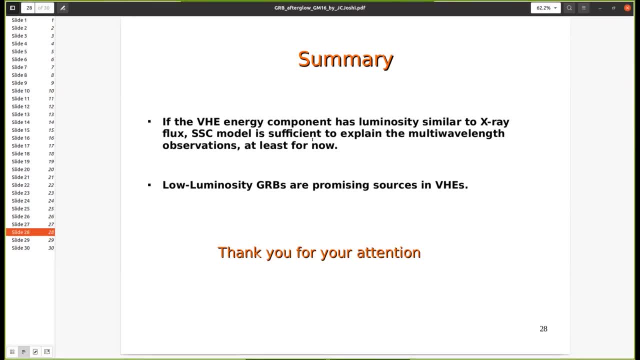 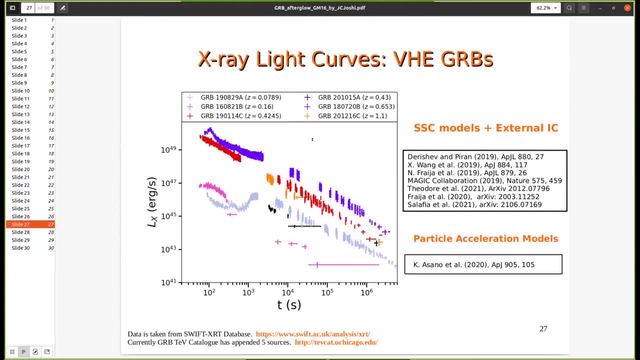 I have one that I, because the connection with X-ray also points out that the GV stuff, so the prompt or the component measured by LUT, is somehow, if it is self-synchrotron, Compton, is not in the best reason of the region of the spectrum to be connected to the X-ray. So it's not in the best reason of the region of the spectrum to be connected to the X-ray, So it's not in the best reason of the region of the spectrum to be connected with the very high energy. 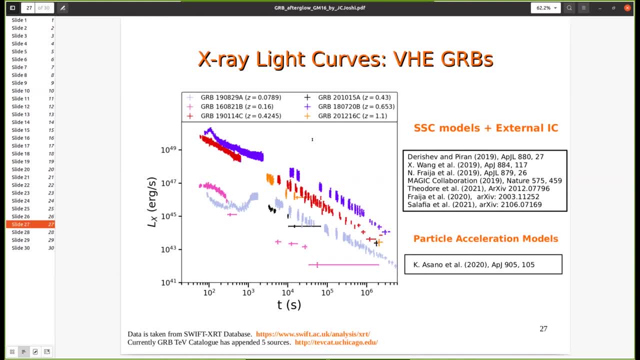 So do you think that we need to change something? let's say, having for the future, more sensitive X-ray instruments instead of, let's say, having, let's say, hard gamma ray instruments of space. Okay, so, for example, like if we see the very high energy signature, 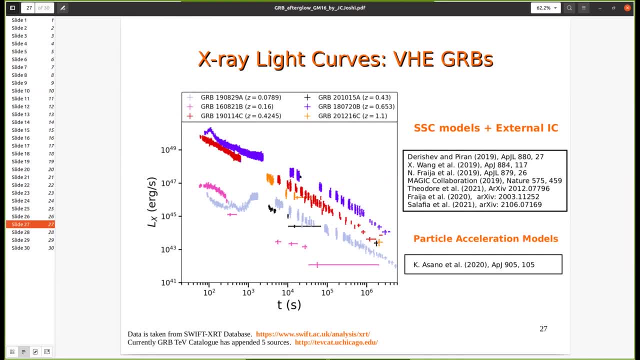 of gamma ray burst. they are independent of X-ray luminosity because the X-ray luminosity have very diverse range for the detection. The second option is like, for example, in: more or less the SSC or external Compton models are working very well for interpretation of the multi-wave length. 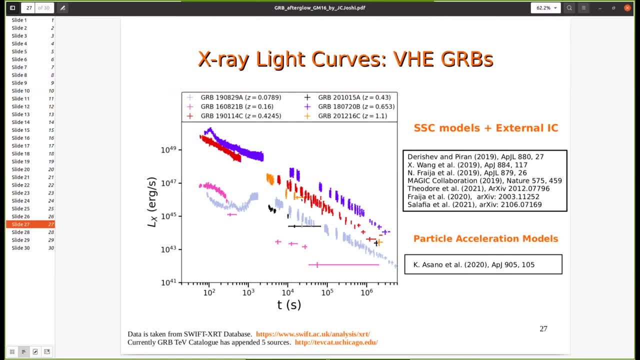 observations. However, if we have, we have like. for example, like at least for now, we have good observation in X-ray. So I'm not very sure, in my opinion particular, which wavelength can be good for for the detection, because definitely the X-ray is correlated with the TEV. So if there are more sensitive detectors it's always good to have. 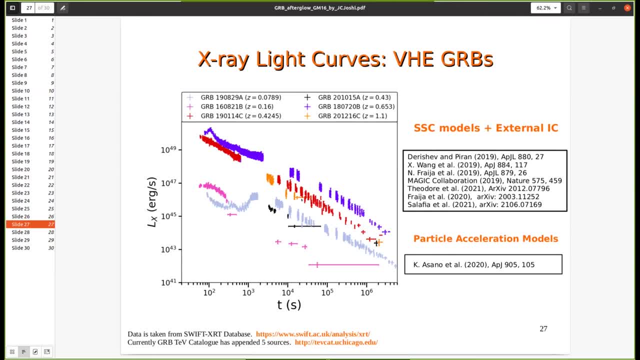 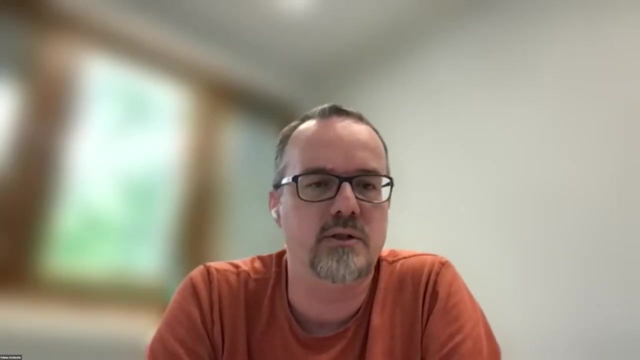 better X-ray fluxes. Thanks, a lot Thanks. Does it answer your question like, yeah, that's what? yes, yes, yes, perfect. Another question? I don't see any, So let me thank all all the speakers of this session. Thanks a lot. Was very interesting run through the very high energy detections and modeling of GRVs. 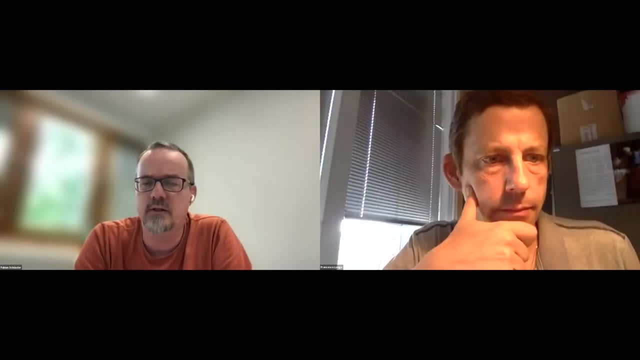 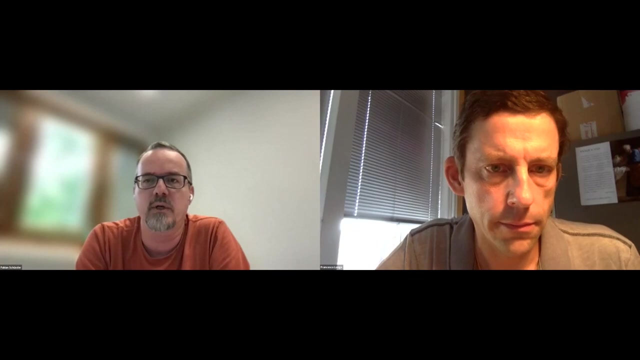 As I mentioned early on, it's not the end of the story because that was only part one of our session. So we reconvene on Wednesday at 9: 30 central european time and complete the. the picture also on the on the low energy. so the the high energy part. 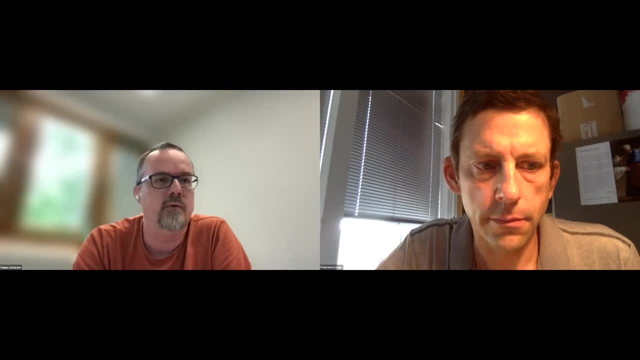 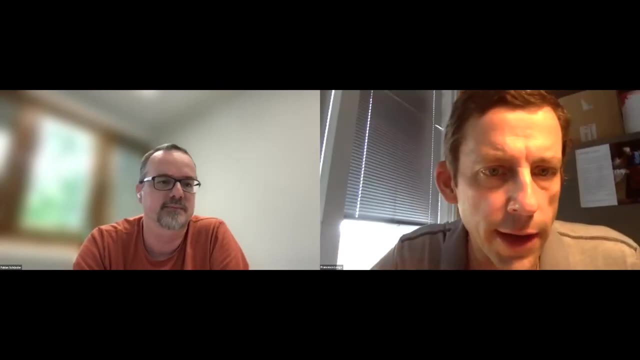 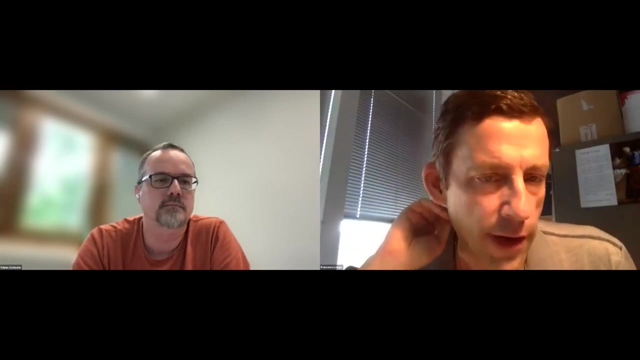 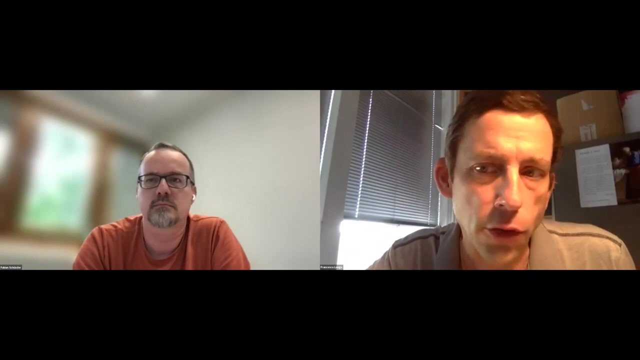 and yeah, Franz, any last words? Yes, Yes, I will circulate the direct zoom link for the meeting tomorrow for so that you will get immediately the. the connection on monday morning, and something that we have not used today, is that if any of you want to, let's say, continue the discussion with one of the speaker, please ask myself, or 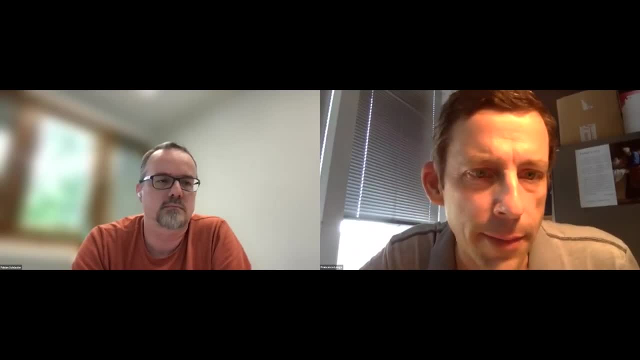 fabian, which are the host, and we can create a breakout room in zoom so that you can continue the discussion there. of course, you will miss the remaining talks, so this is why we didn't advertise, but it might happen that you need to discuss more in detail what was presented. 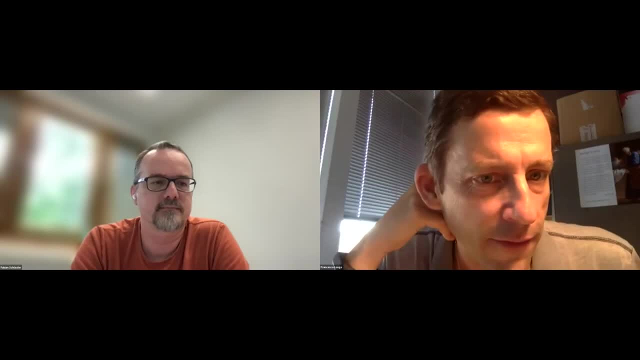 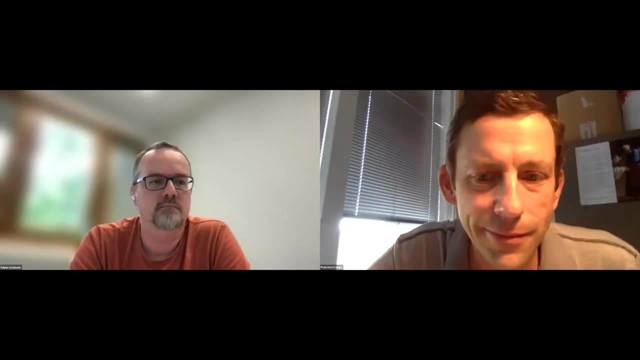 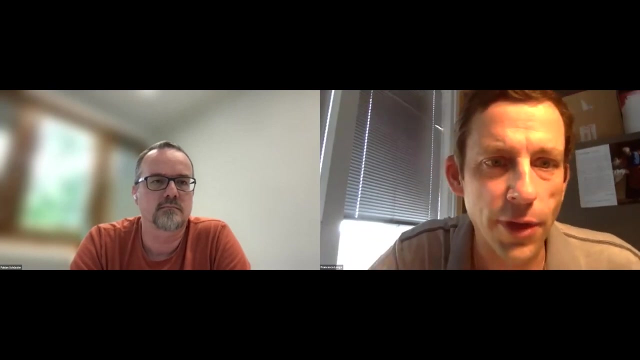 and that the organization make available this, made available this opportunity, so let us know, if you need that, that on wednesday, okay. this france, these breakout rooms are available at all times, right, like 24 hours. no, no, no, these are breakout rooms for our meeting today, okay. 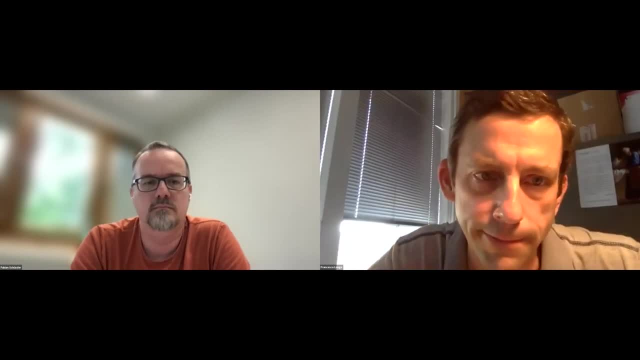 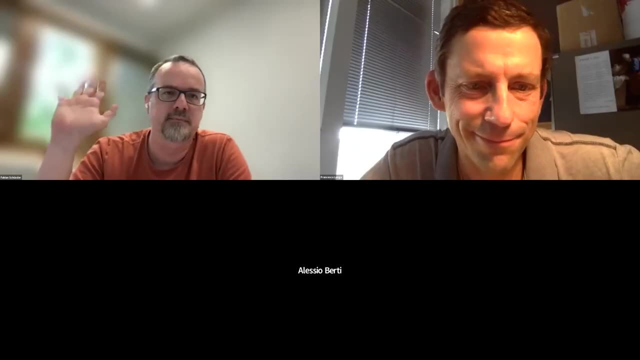 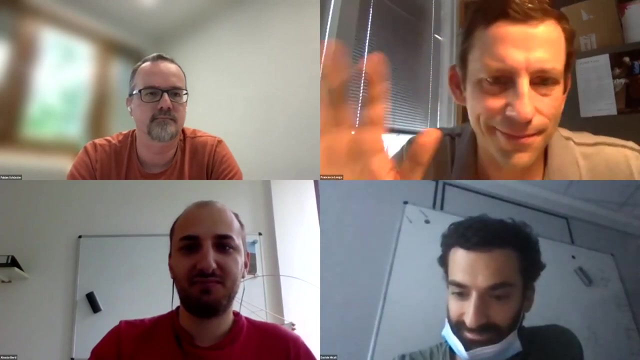 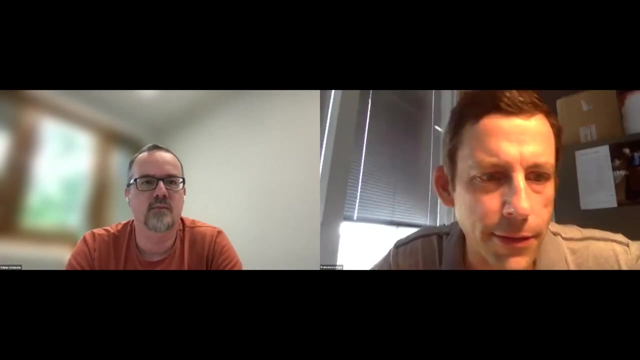 that i have to create today, while let's say we are talking: okay, i see, okay, okay, thanks, thanks everybody. bye, have a nice day, thank you, bye-bye. okay, i close so. 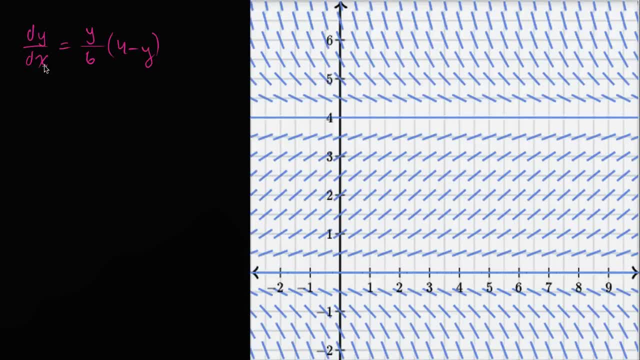 So we have the differential equation. the derivative of y with respect to x is equal to y over six times four minus y, And what we have plotted right over here is the slope field, or a slope field, for this differential equation, And we can verify that this indeed, 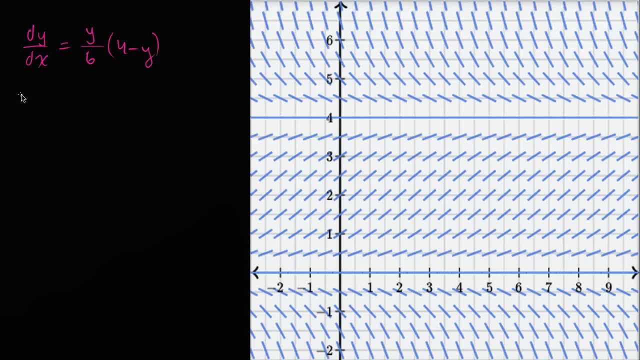 is a slope field for this differential equation. Let's draw a little table here. So let's just verify a few points. So let's say x, y and dy, dx. So let's say we start with I don't know. 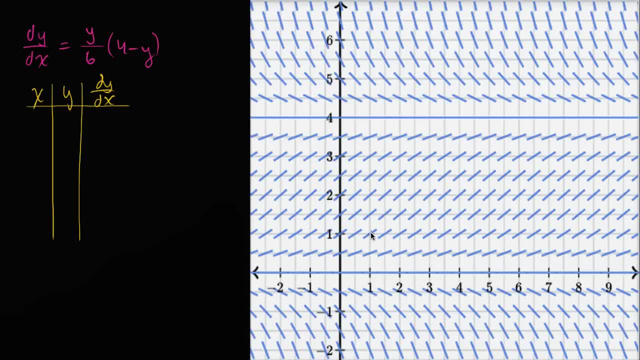 let's start with this point right over here: One comma one, When x is one and y is one. well, when I look at the differential equation, one sixth times four minus one, So it's one sixth times three, which is three sixths, which is one half. 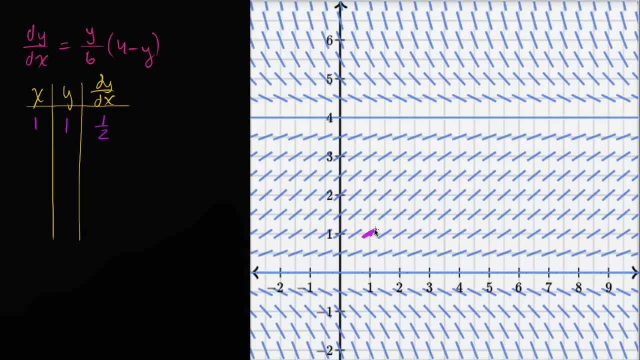 And we see, indeed, on this slope field, they depicted the slope there. If a solution goes to that point, right at that point, its slope would be one half And, as you see, it's actually only dependent on the y value. It doesn't matter what x is. 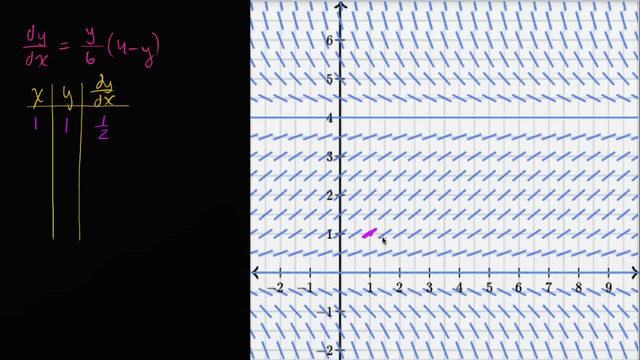 As long as y is one, dy dx is going to be one half, And you see, that's why when x is one and a half and y is one, you still have a slope of one half, And as long as y is one,